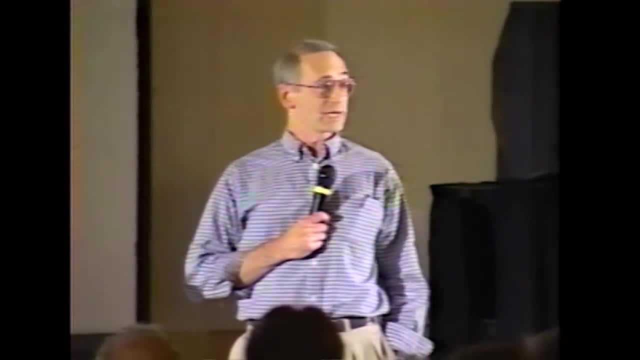 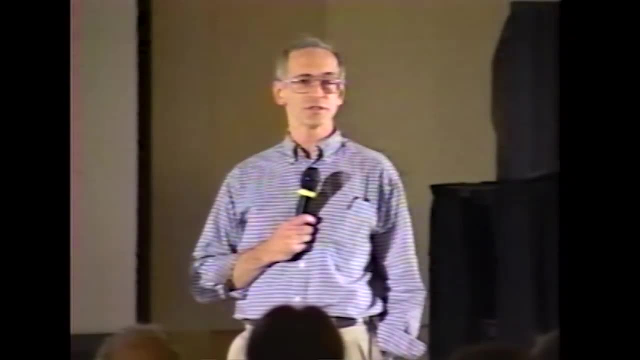 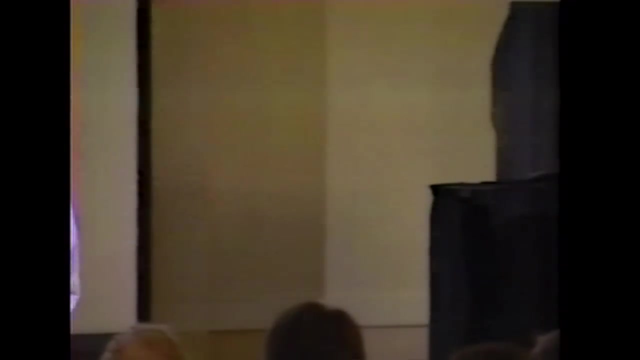 and documents and books and so forth. we're inviting people to help us with this project by doing lots of things. we have weekend volunteer days when people come and help us work on the collection. we'd like as many people as can to become members of the museum and you can do that in several ways. one program if. 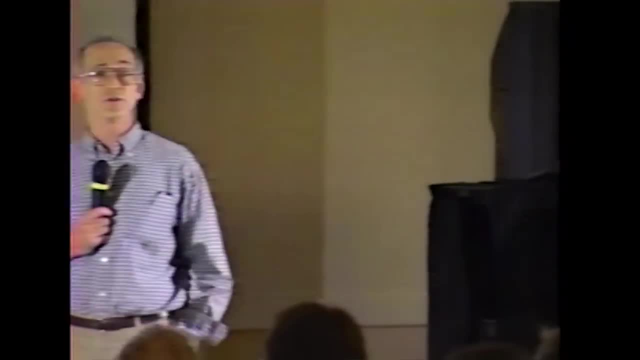 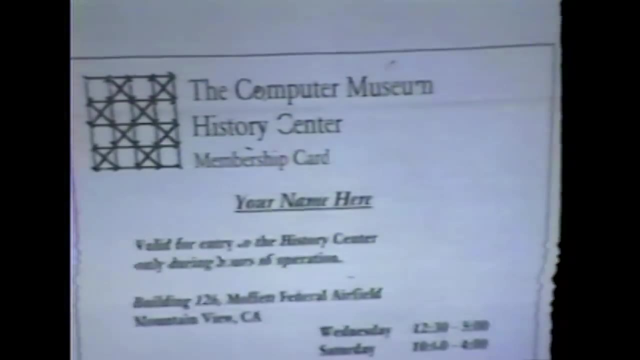 we just started is that you can become a member for a hundred dollars and get a card that gives you access to the History Center and also gets you access to Moffat Field. so on Wednesdays and Saturdays you can, without going through the process you went through today, get on to the field and to have access to 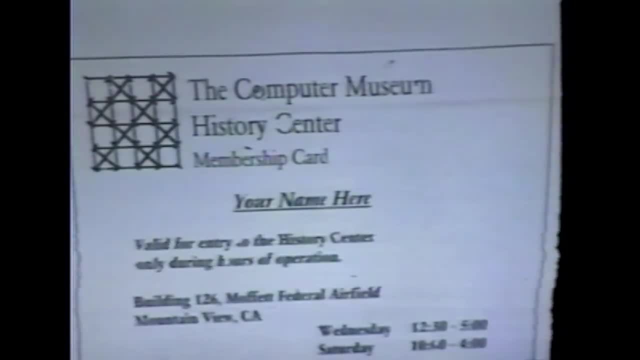 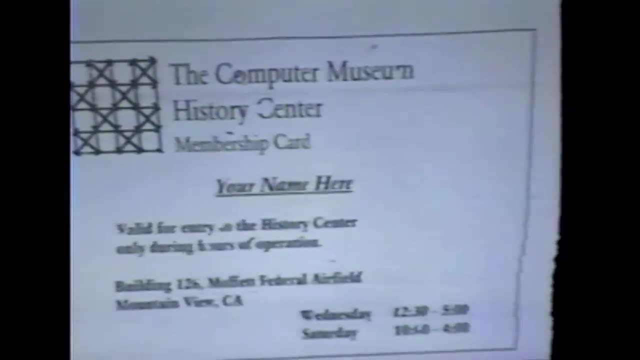 our visible storage location. in addition, for the next- I guess about six months, you have an opportunity, one time only, to become a founding member of the Computer History Center by donating a thousand dollars or more and be promoted to the Museum of History. I was permanently enshrined as one of the founders of the Computer History. 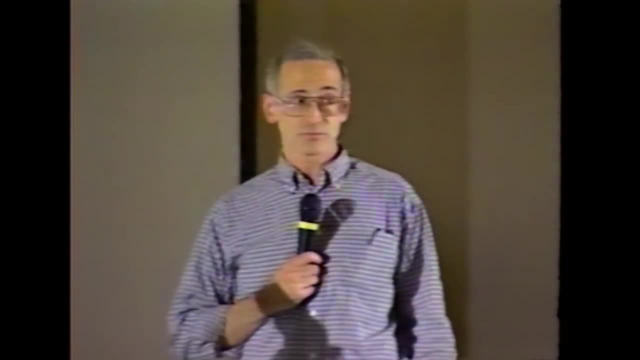 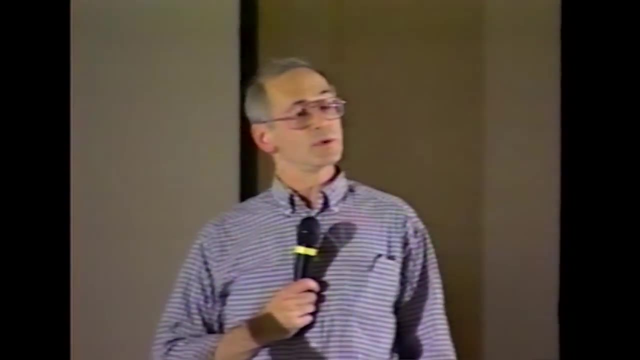 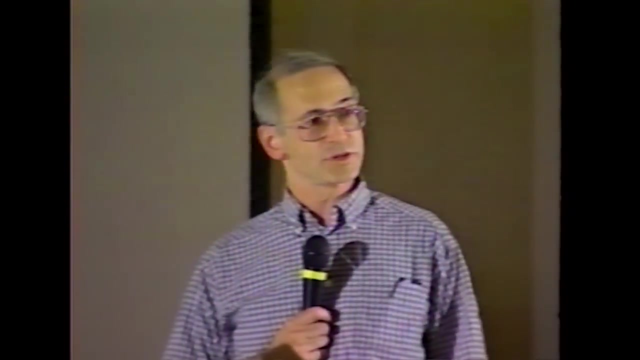 Center. it's the same kind of program that was done by the Computer Museum 10 or 12 years ago when it was in its founding stages. what else are we doing? we're, we're having a. we are mounting a bunch of expert of exhibitions in various places. we've done several at trade shows and conferences. we've got 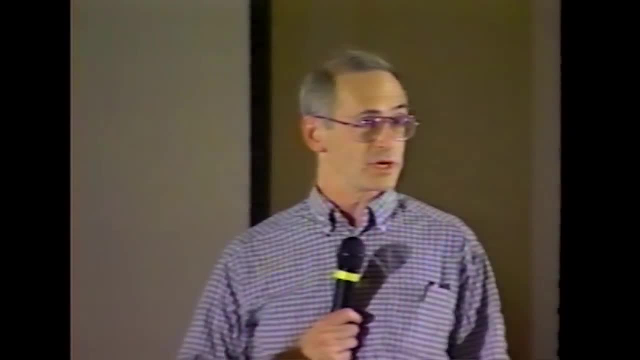 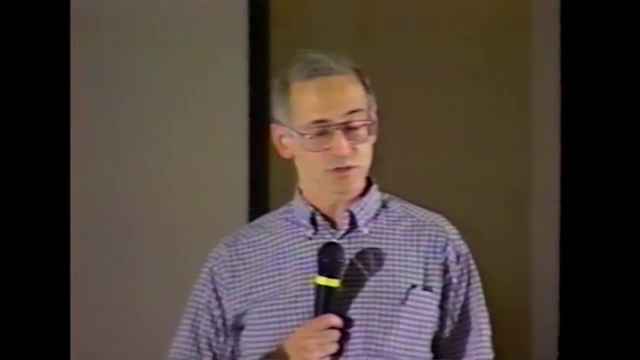 one that's going to be opening next week at the new gates computer science building at Stanford, where we're taking part of our collection and and showing it off, and until we have our own permanent space, that's a good way to show off some of our wares. we've got more stuff coming as we speak. there are four tractors. 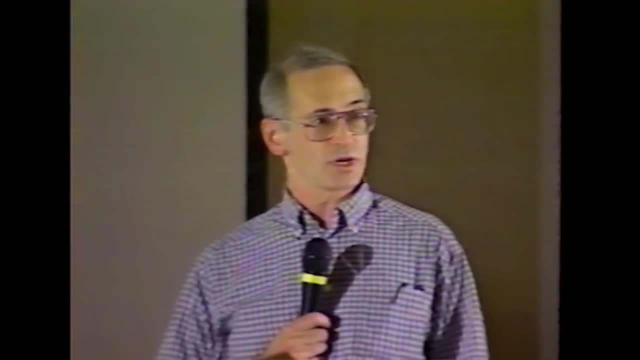 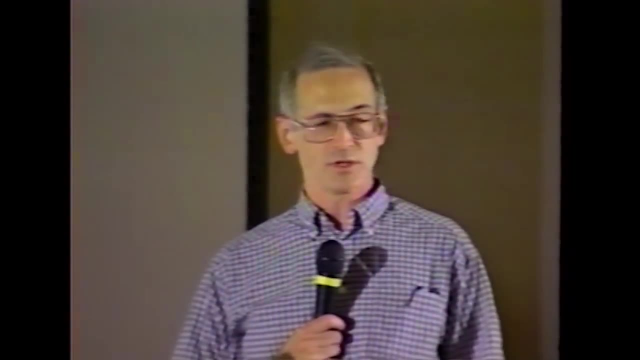 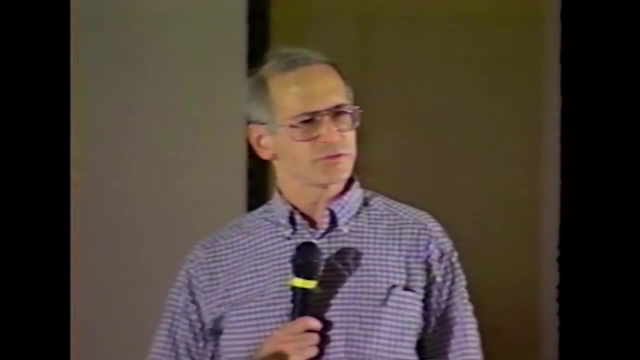 loaded, being loaded in Boston and heading across the country with the next installment of the machines and and the part of the artifacts from Boston, and included in there is what the Johnny act and cm5 thinking machine that we just got from MIT and a whole bunch of other very valuable artifacts, if you want to. 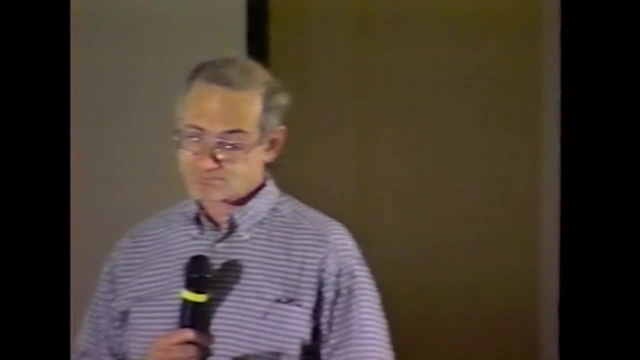 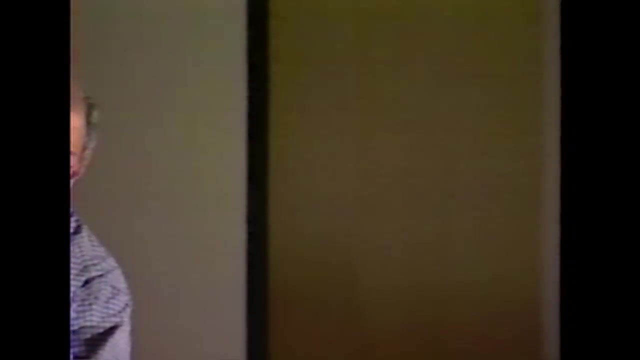 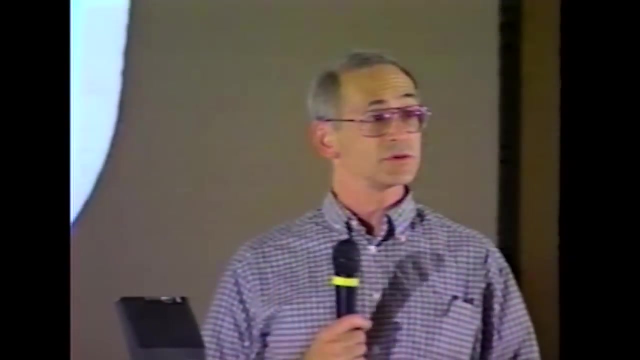 get more information about the Computer History Center, talk to me or Gwen Bell or Zoe or Dag or any of the other people who are on staff. we'd like to thank the people at NASA Ames here for their hospitality, both in the use of this conference center but also in the use of the warehouse space, for which we're very. 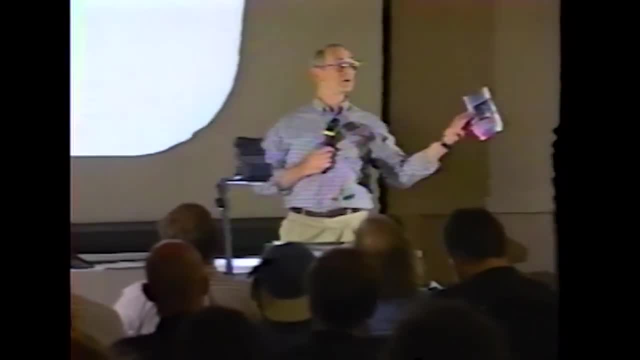 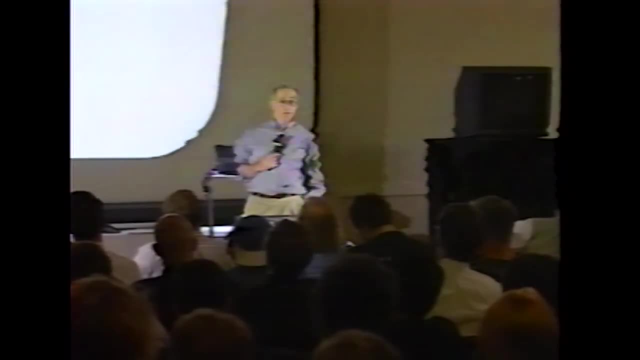 much in debt to them. there are some fliers in the back that you can pick up that describe what's going on here, both NASA and generally in their center for excellence in information technology. this is one of a series of talks that we've been giving in cooperation with the 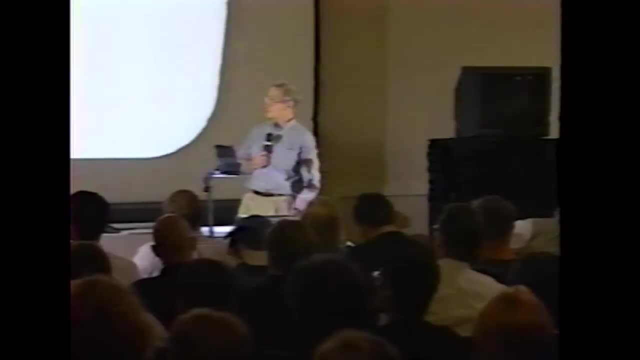 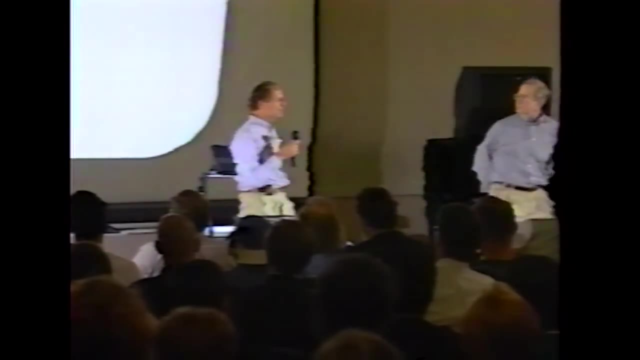 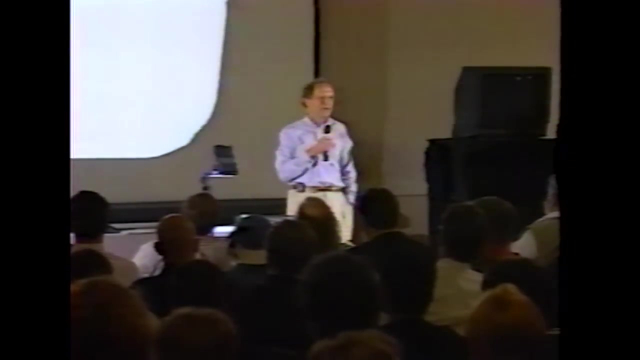 Bay Area computer history perspectives. Peter Nersky runs that and he will introduce tonight speakers. thank you, Len. I don't really run Bay Area computer history perspective. it's more a joint venture between myself- I work at Sun Microsystems- and Jeannie Trichle also works at Sun Microsystems and Jeannie was. 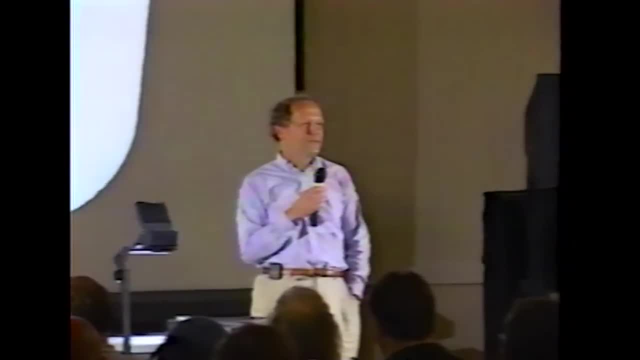 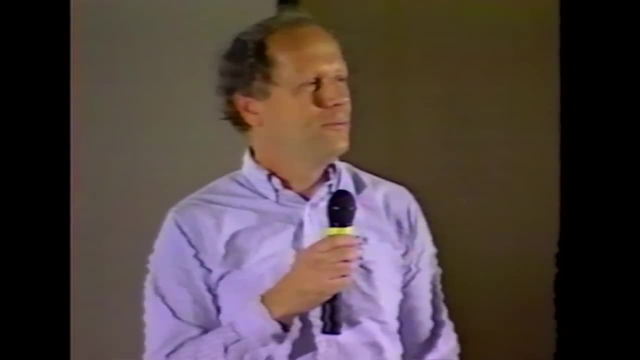 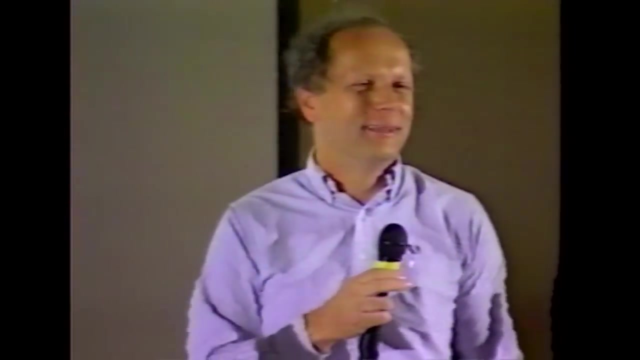 at Xerox PARC many years ago. as part of history itself, we started this computer talk series over four years ago, like 1973, and two of our speakers at the first program here in the front row, Norm Hardy and George Michael from Livermore, and so a lot of people have been coming back over. 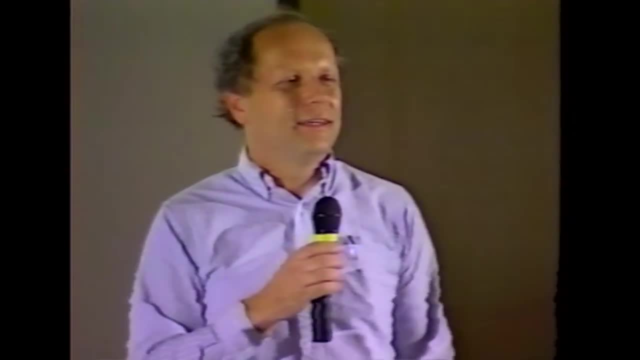 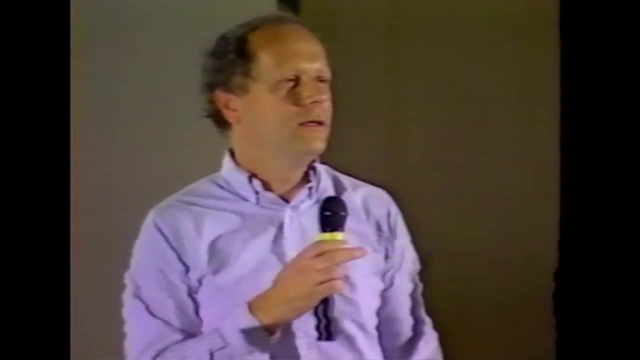 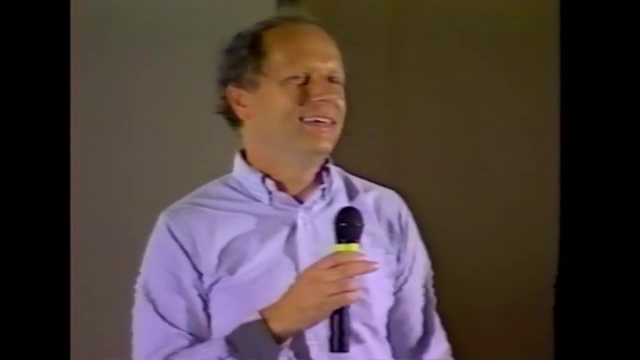 the years from one program to another, and Larry Tesler, who's one of our two speakers tonight, himself did a program, along with Bob Harriet, Larry Breed, Don Wise, over three years ago on the Stanford card stunts, which I wrote up in the description was the largest bitmap display ever. 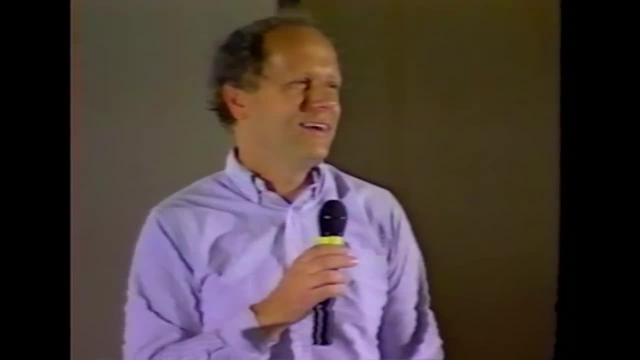 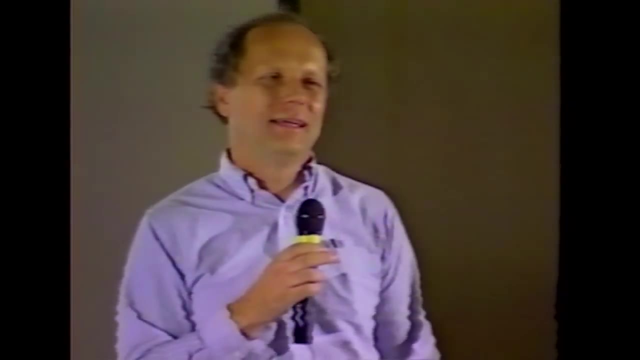 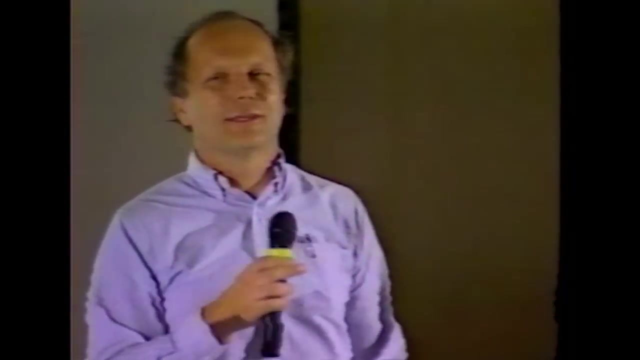 You know it was like several thousand students holding up colored cards in sequence. That was a feat itself to do the programming of the instructions back then at that time. And Larry has also been coming to many of the programs before and since then. So it's like this history talk series has developed a history of its own. 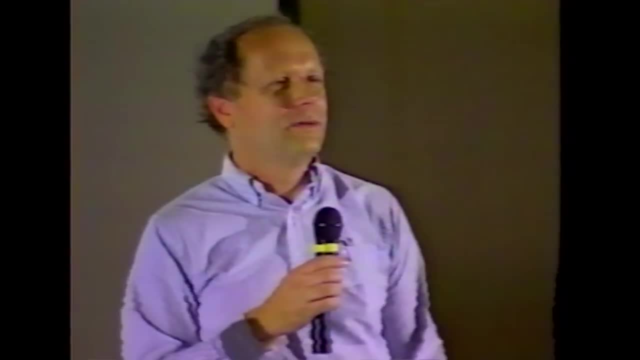 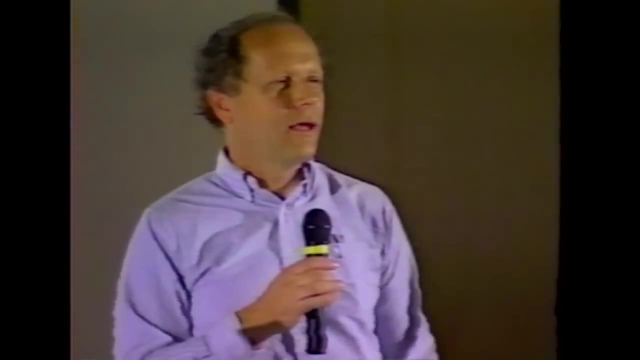 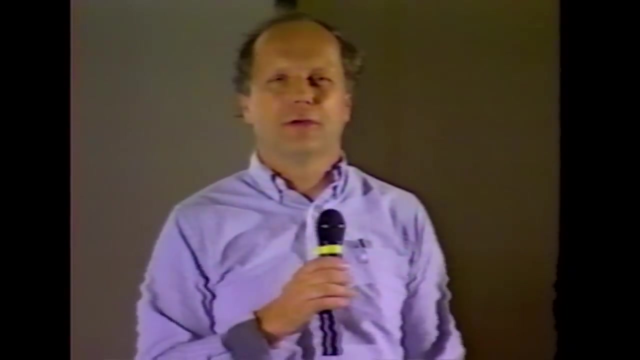 So tonight we have Larry and Chris Espinoza from Apple talking about the early Apple user interfaces And I think, as you may have heard, Larry came to Apple from Xerox PARC back in 1980, and he figured he was bringing a lot of user interface knowledge with him. 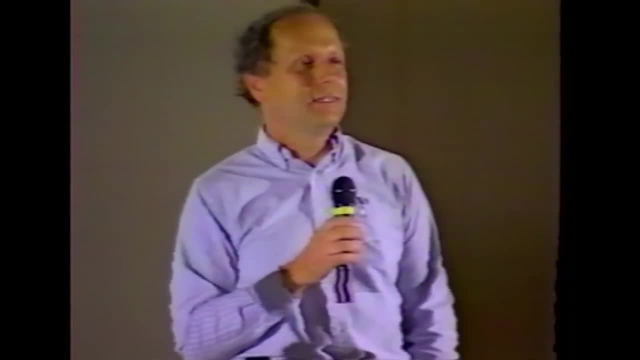 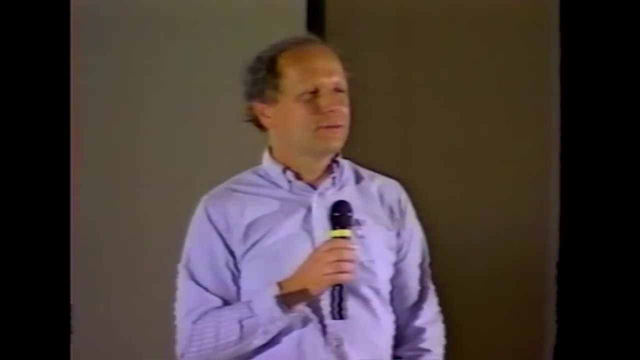 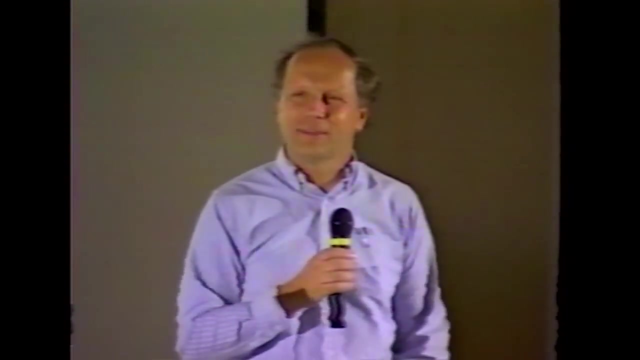 only he's found out recently that user interface testing and development existed at Apple before 1980, and Chris had a part in that. Chris, I think it's correct, was probably the youngest Apple employee ever did demos at Apple while a high school student. 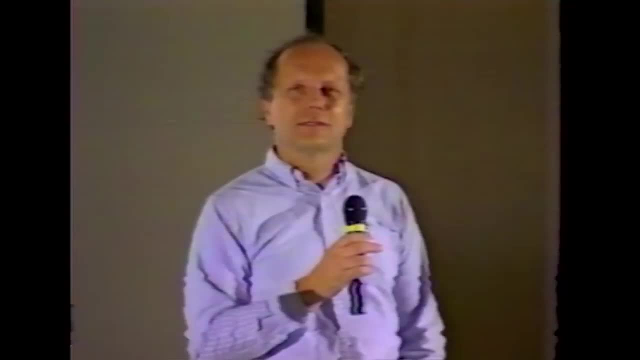 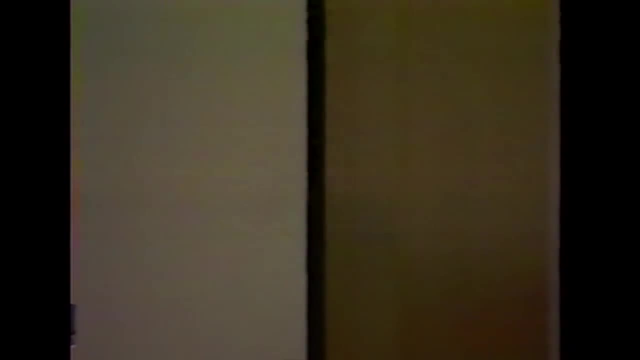 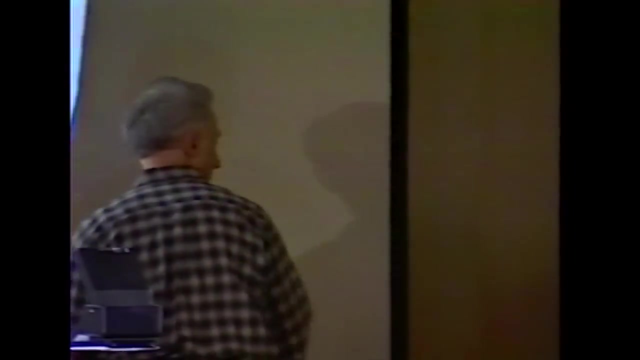 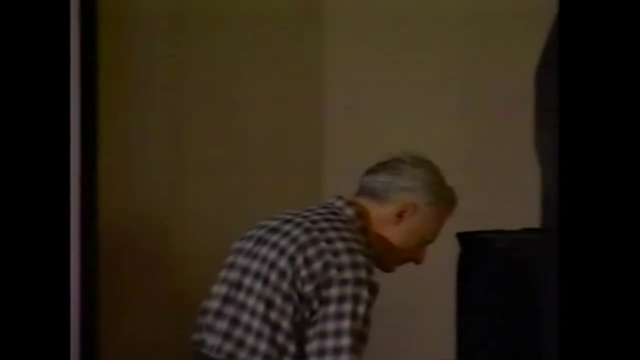 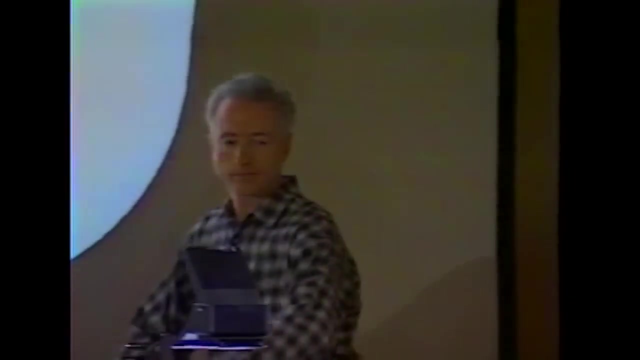 So, Larry, pass the mic. Where's Larry? There you are. Okay, I already have one. Is your tape in there, Chris, Or out? Okay, fine, Good, Put mine in here. Okay, well, glad to be here. 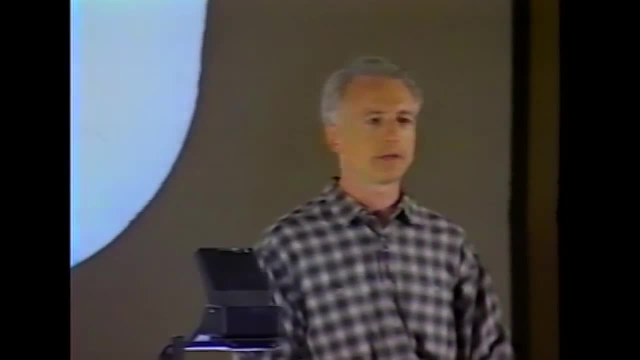 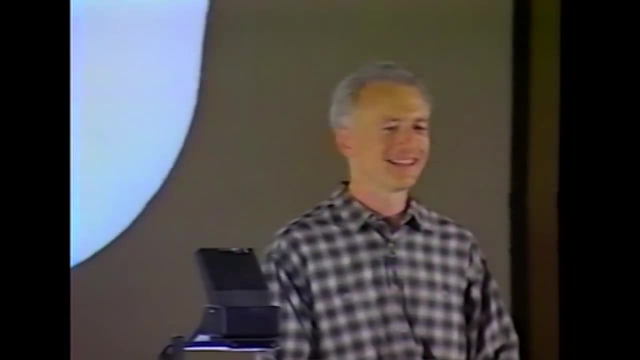 This is a talk, actually, that's based on one that Chris and I gave at Apple Back in July, And we got clearance, thankfully, from the Apple lawyers, which came about two or three weeks ago, So we could give it here just in time to announce it. 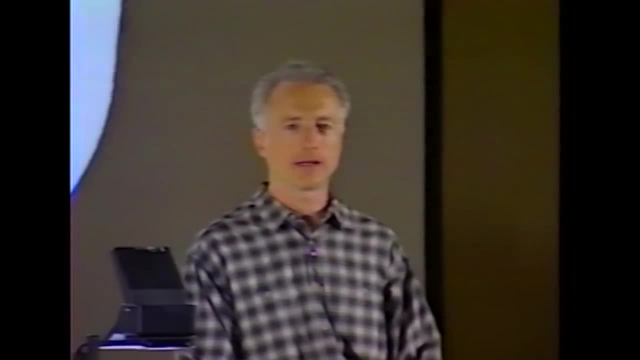 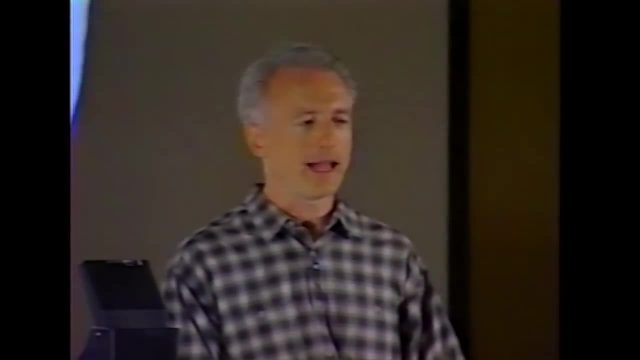 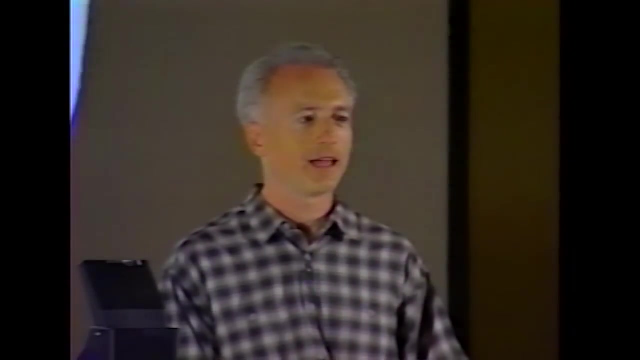 And we're grateful to Apple to release this for public disclosure because we think it's of general interest. Asking about what was early user interface design at Apple is kind of like asking about early engine design at Mercedes-Benz or something Everybody was doing it. 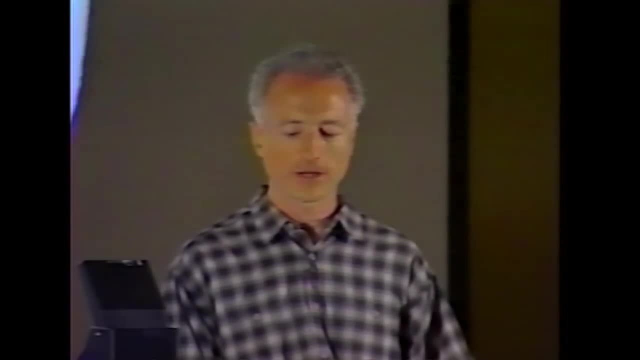 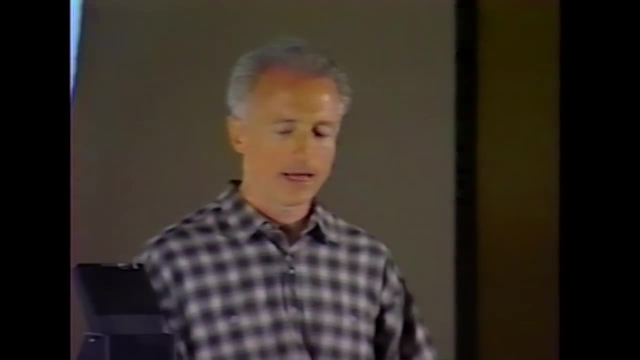 So, depending on who you, You could have gotten a lot of people up here to give a talk and you'd get different perspectives on the same things that happened. So today you're going to get the perspective of a couple of us, To get it to be a little more grounded in something more closer to fact. 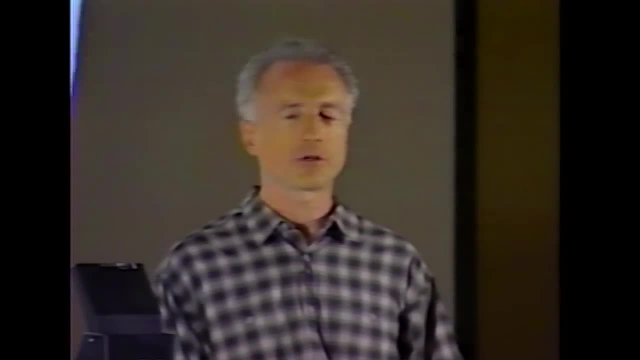 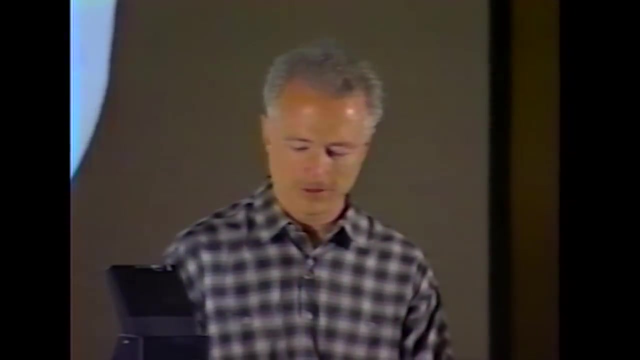 than opinion or perspective. we're trying to use as much as possible actual, original documents that were created at the time, so you see actual, contemporaneous thinking as it was going on, instead of just our memories, which fade over time and tend to aggrandize over time and so on. 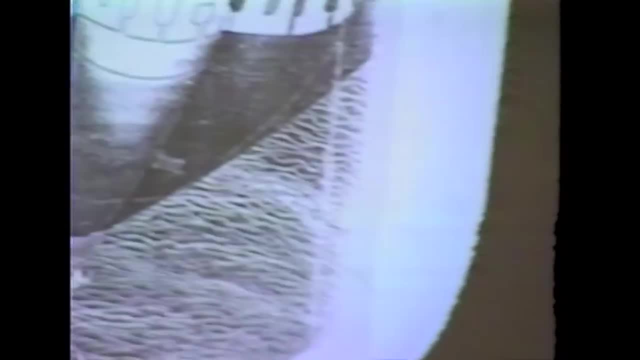 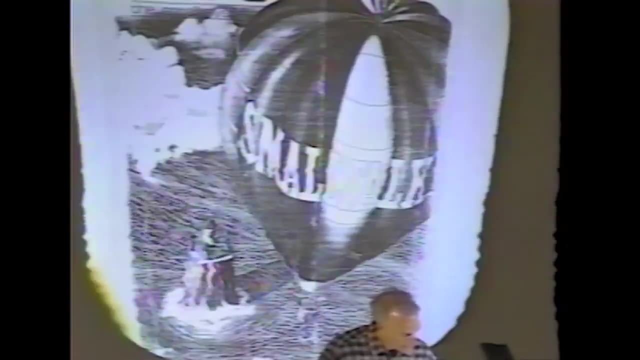 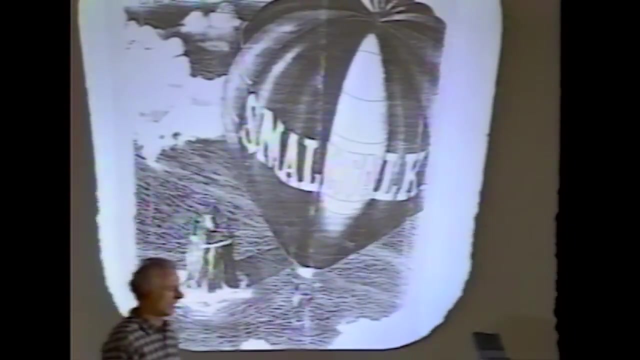 So here's something which is not from Apple. This is the cover of Byte from August 81. that was the small talk issue. This one doesn't have color, but it's a very colorful balloon, And the reason I show it is that there was a lot of influence from Xerox, obviously. 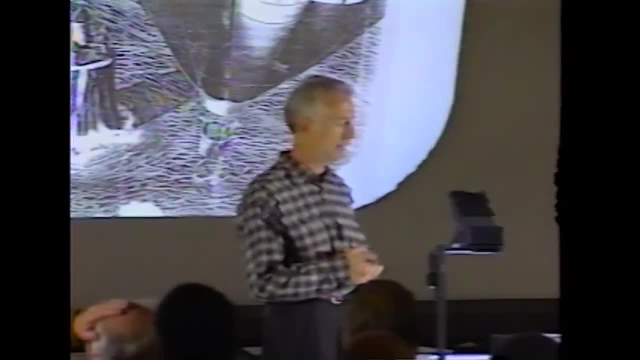 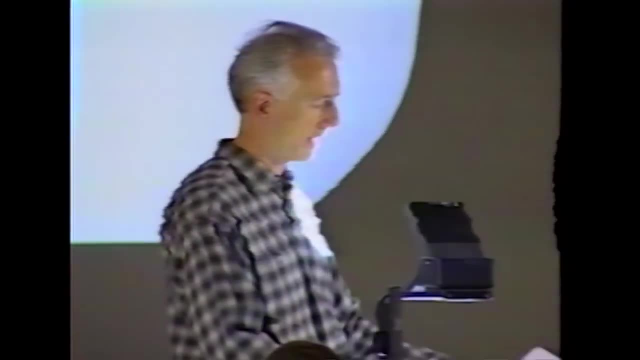 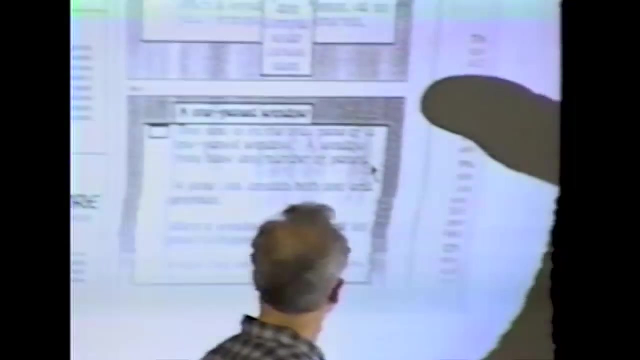 on the user interfaces that were done on the Lisa and the Macintosh, But maybe not as much as some people think. Media tends to just say, oh, they just copied it. So I'm going to show you what it looked like to be working on from that article which I wrote. 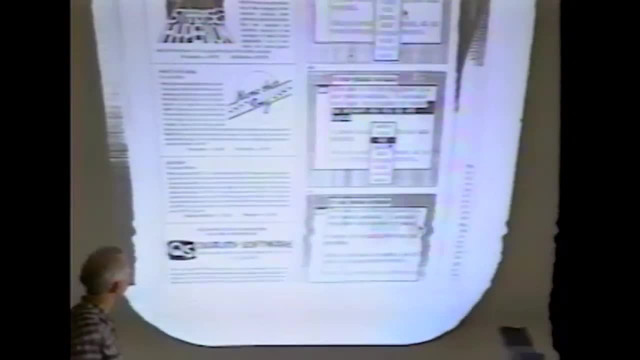 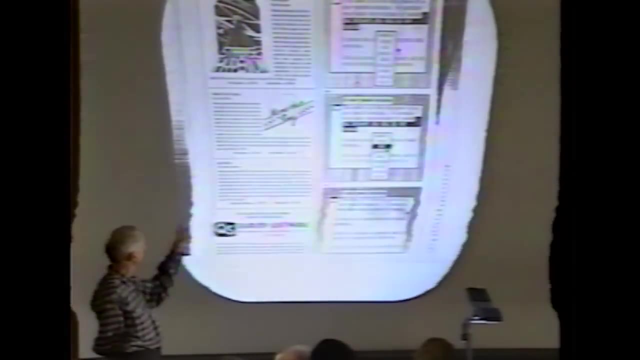 to be working on a small talk at that time, 1981.. And you see what the windows looked like: kind of a little rectangular title scroll bar without any arrows and a little pop-up menu. There were two pop-up menus that you could use for each window. 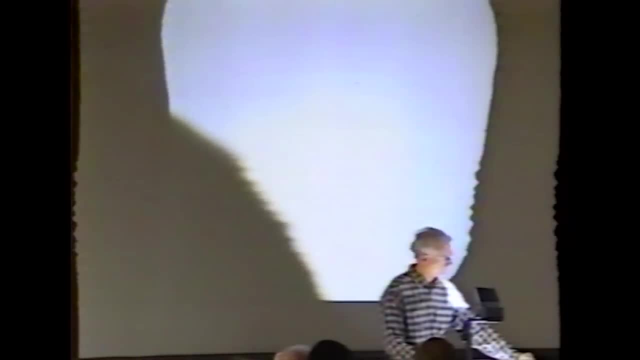 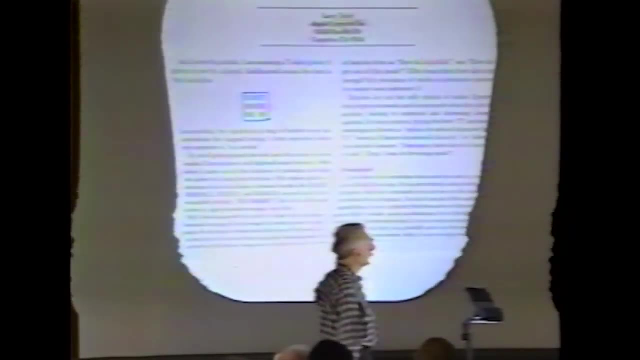 So it was a pretty different looking interface, And one of the principles- though that was in the small talk environment- was to have no modes, And there was actually a photograph of a T-shirt that was made for me by a friend that said: don't mode me in. 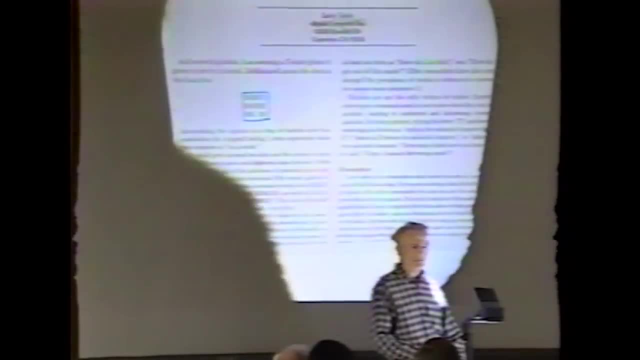 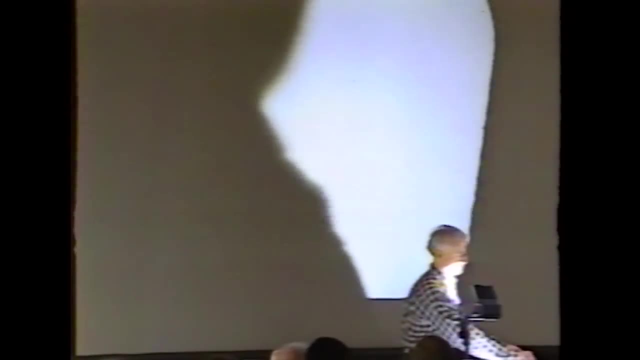 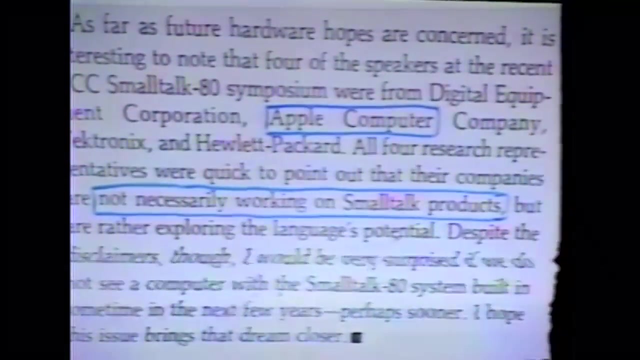 that represented sort of this mission I was on to try to eliminate all modes from user interfaces, Which isn't necessarily a good idea, but it was definitely the mission I was on. And at the end of that article it mentioned that Apple Computer had gotten a license to small talk. 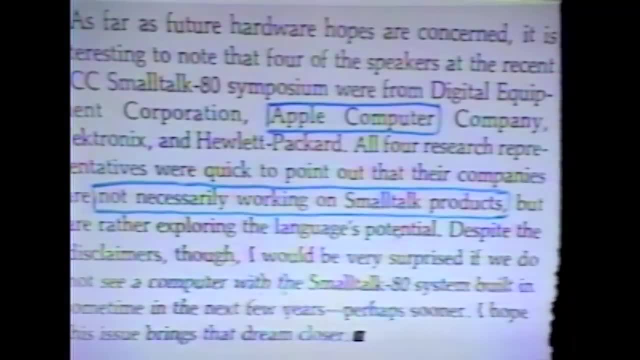 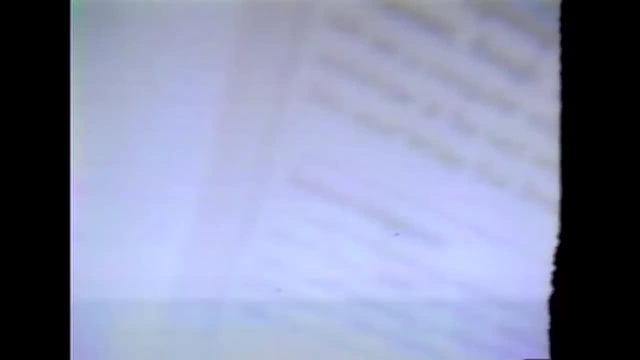 and was maybe going to do something with it but maybe not going to do anything with it, And in fact Apple and Yorke Packard, Digital Equipment and Tektronix all did do various amounts of small talk development after that. 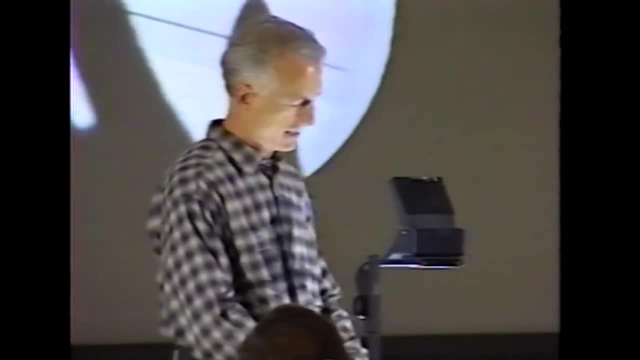 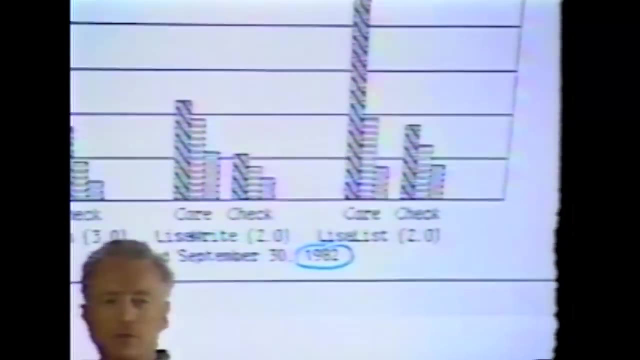 but it was really independent companies that managed to make small talk somewhat of a success. I'm jumping to the end here before I go to the beginning, just to let people know what the Lisa was. The idea of the Lisa was to have something that was very, very easy to use. 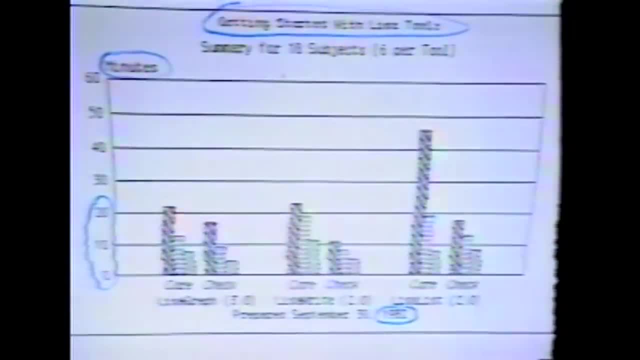 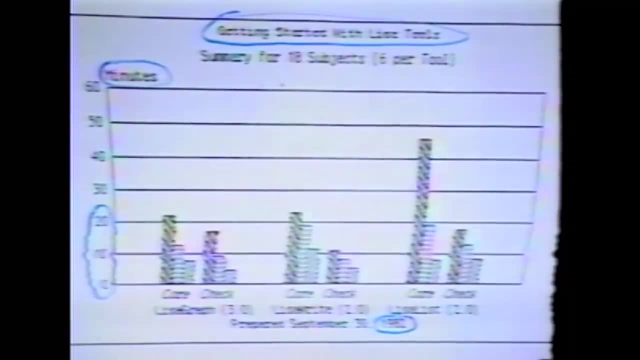 People loved the Apple II, which was what we had at the time at Apple, but it took a long time to learn how to use it, And what we wanted to end up with was something that was easy to learn, And just to show you that we did do that, 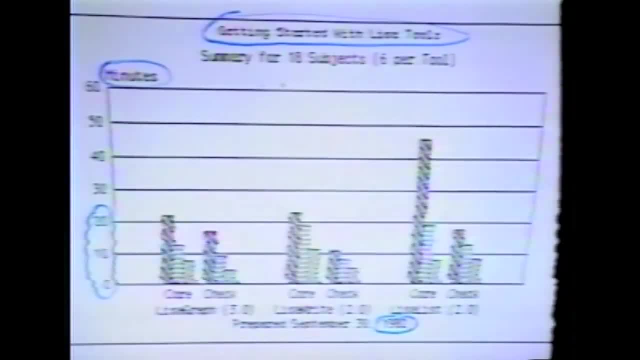 this is a study done at the end, where there were 18 subjects, six using Lisa Graph, six using LisaWrite. LisaList- Lisa Graph- was a business graphics program. LisaList was a list manager kind of flat file database. LisaWrite was a word processor. 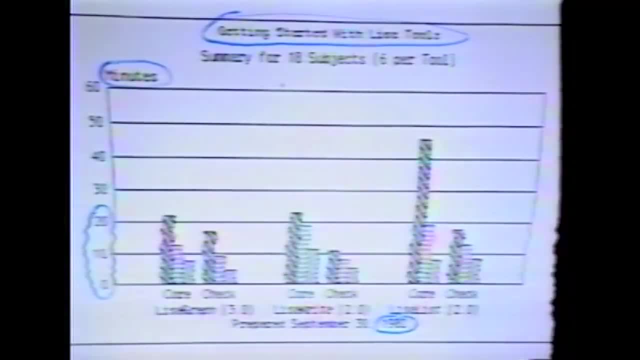 And, as you see, for all but one user using LisaList, it was under 20 minutes to get through the core competency to use the application And if you ever had a chance to use a Lisa- and I hope to be one operating here someday- 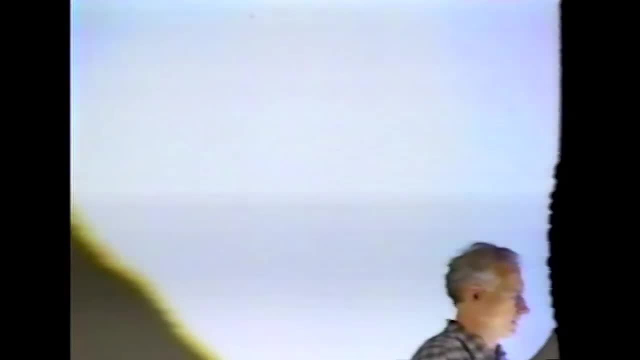 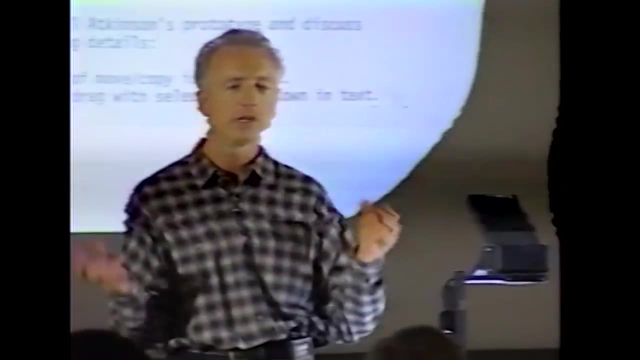 then you'll see that it was extremely easy and in many ways more bulletproof, I'd say, than the Mac, Not simpler than the Mac, actually, but we loaded a lot of things into it to try to make it so people couldn't get themselves in trouble. 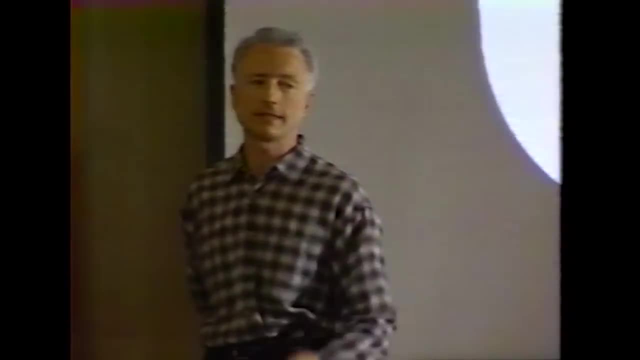 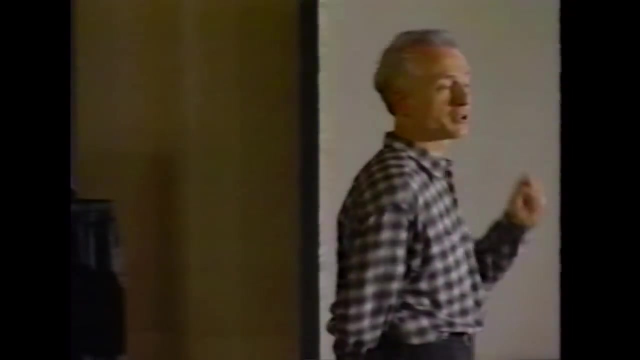 Okay, so let's start at the beginning. I started at Apple on July 17th 1980, and I just left there a few months ago. I was there for 17 years And this memo was written on July 18th 1980.. 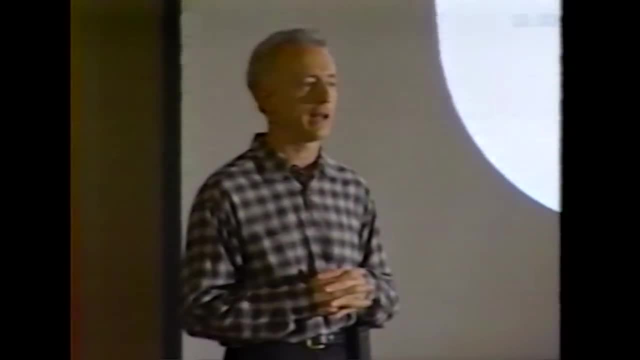 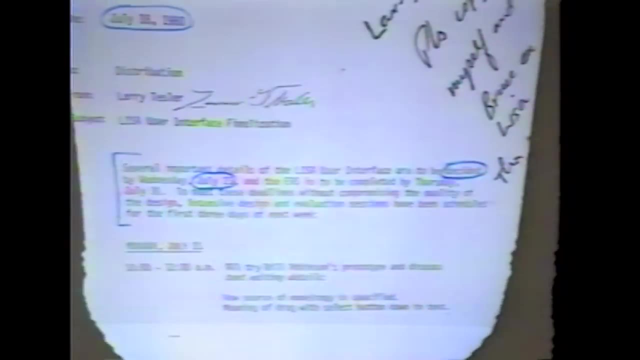 So one thing I discovered when I left Big Xerox Corporation and went to this little Apple startup was that you just really get engaged immediately and they put you right to work. And one thing I was told the day I got there was that the user interface design. 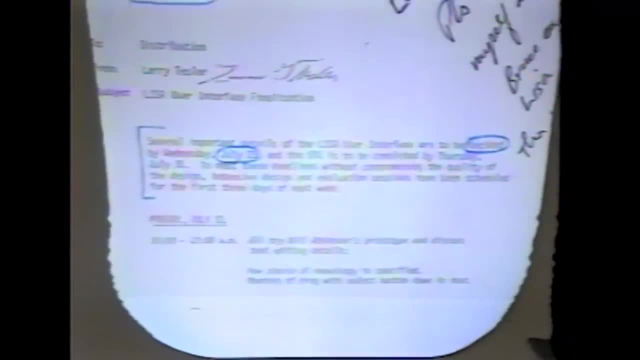 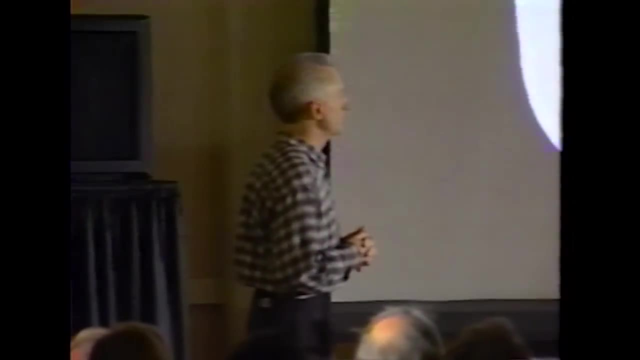 was basically done and they were just going to write it up and finalize it and implement it and that was the end of it And it was too bad. I took so long to show up at the office because they were hoping I could have contributed to it. 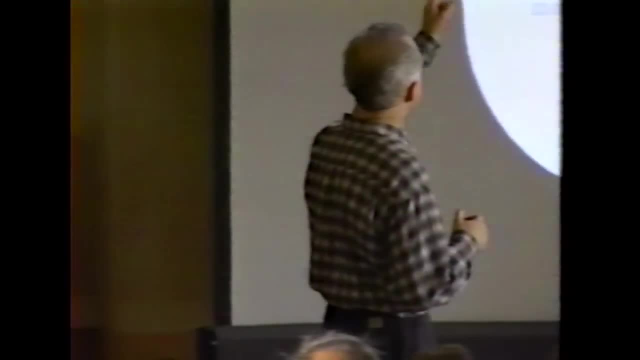 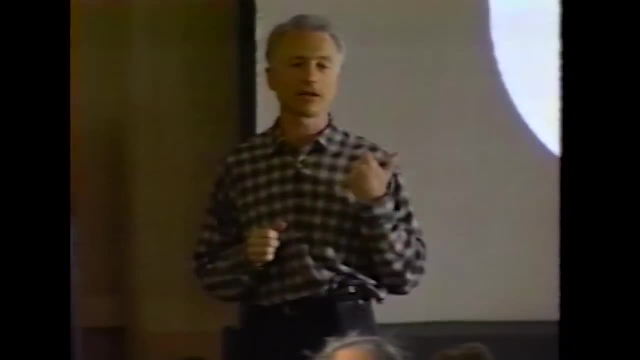 but now there was no time left to do that, And this was the 18th, and they told me that all the decisions had to be made by the 23rd and by one week later the external reference specification had to be done. 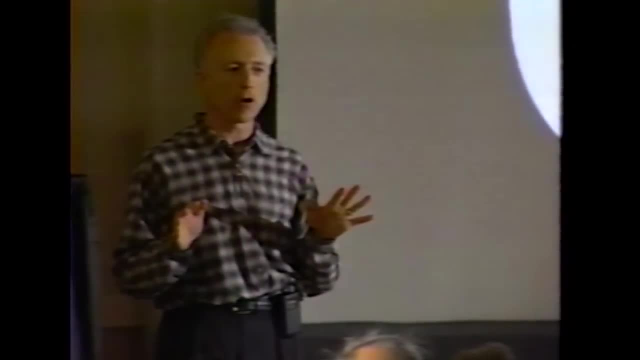 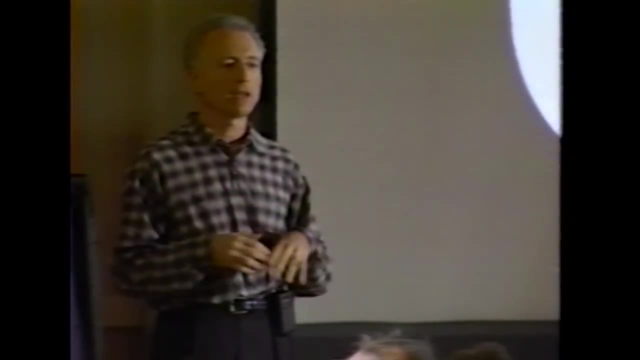 which was the complete spec, but we couldn't compromise quality at all, and so what could I do between the 18th and the 23rd to make sure we made all the right decisions? So I started explaining how it was really necessary to do months of user testing and careful iteration. 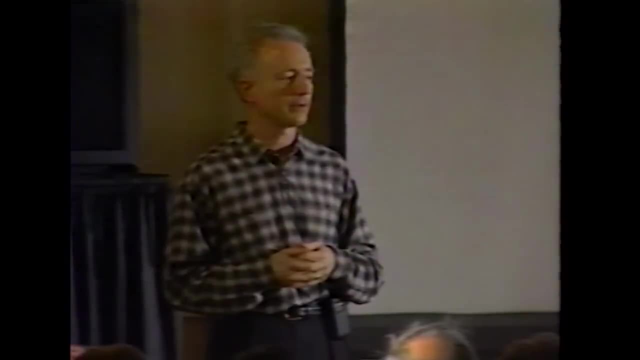 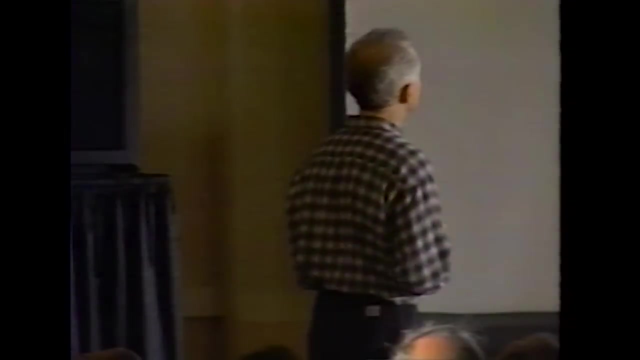 and I gave them a whole spiel about the right way to design software and they said: well, sorry, we only have five days and there's a weekend in there. So we got together and we came up with a compromise, which was to lay out a schedule that was very aggressive. 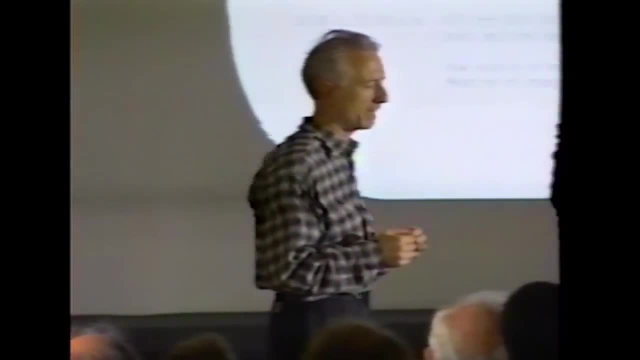 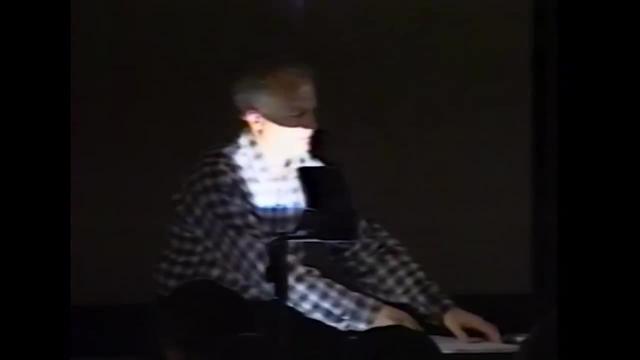 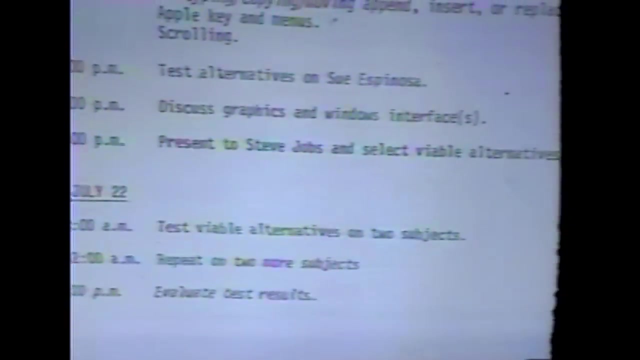 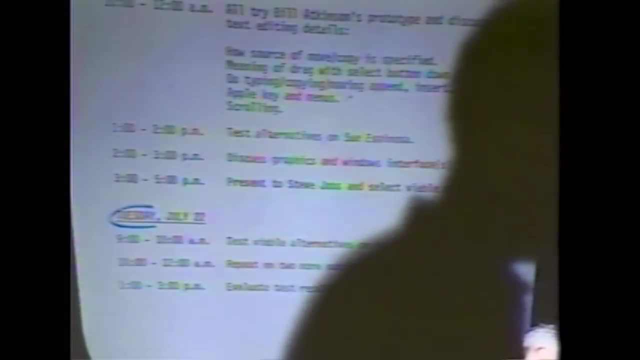 and people promised that they would meet their part, So let's go through the schedule. This was the 18th Turn. this make it a little easier to get at This. No, It is Pull. Oh, that kind of pointer. 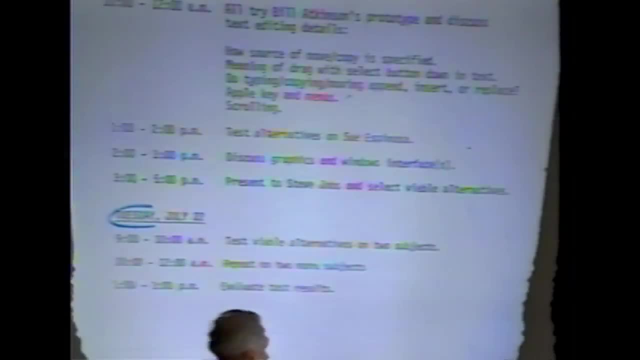 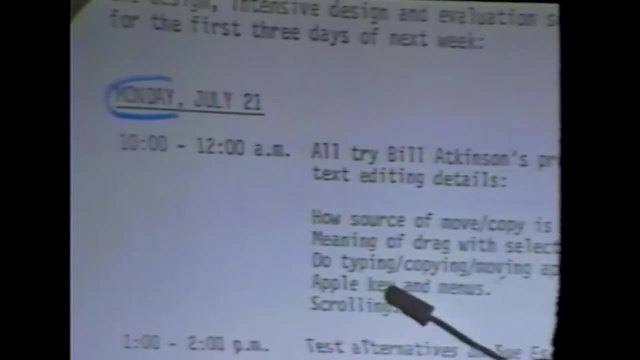 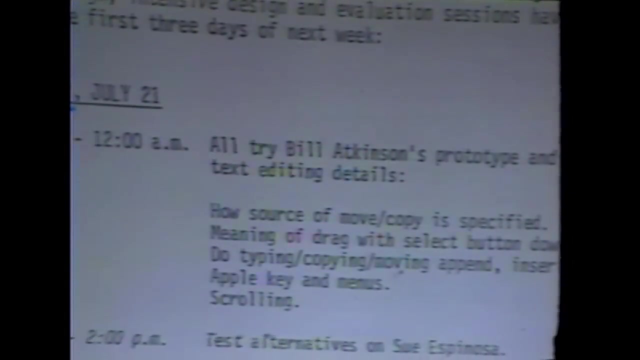 You're the one with the laser. Ooh, Okay, So here was the schedule. Monday we're going to run user tests, So we're all going to try it ourselves. Everybody's going to try Bill Atkinson's prototype. 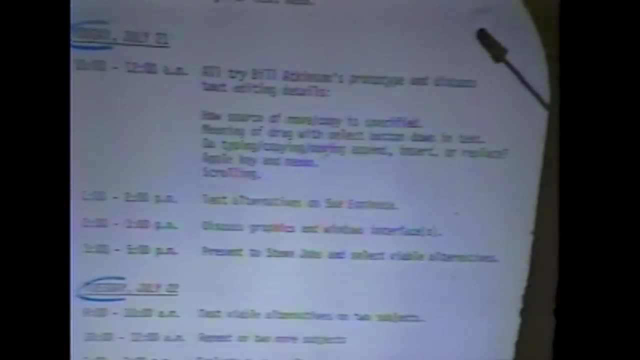 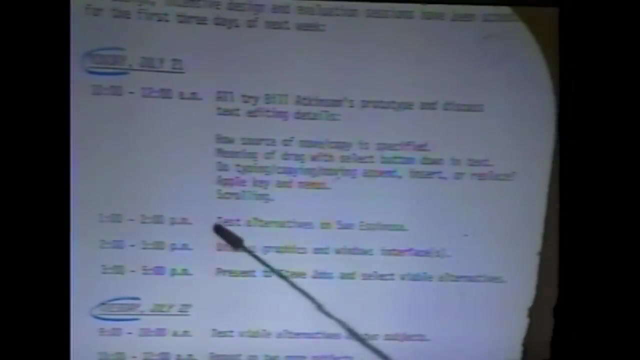 Bill Atkinson was the person building the prototypes at that time and thinking up a lot of the ideas, And we were going to evaluate several issues that were going on. Then we were going to bring in. after two hours of that, we were going to take a break for lunch. 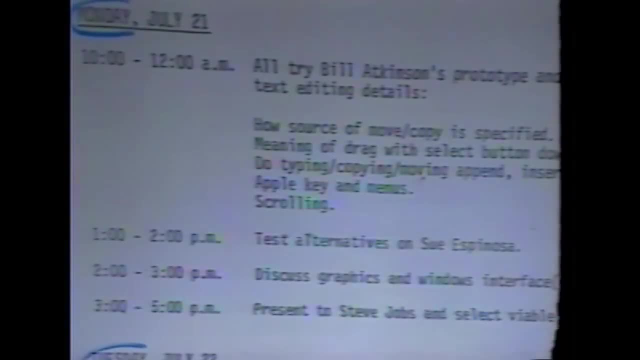 Then at 1 o'clock, we were going to bring in Sue Espinoza, who was in charge of training and also, coincidentally, is Chris Espinoza's mother, And then she was going to give her opinions about that and maybe help us decide. 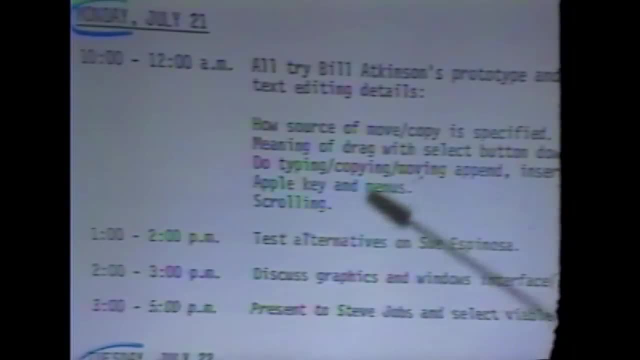 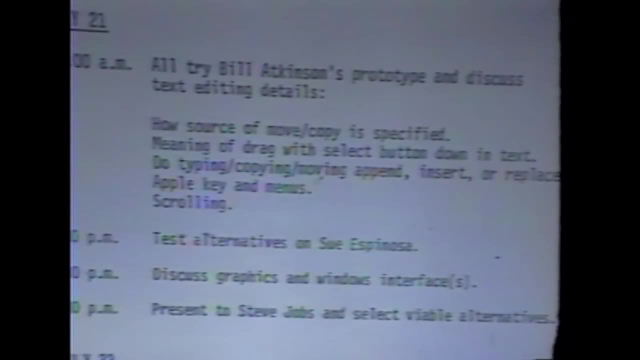 on what would be easiest to train in her opinion, And then at 2 o'clock we were going to discuss for an hour a couple of more issues, And now we would be done. We will have discussed all the issues, And then between 3 and 5 o'clock, 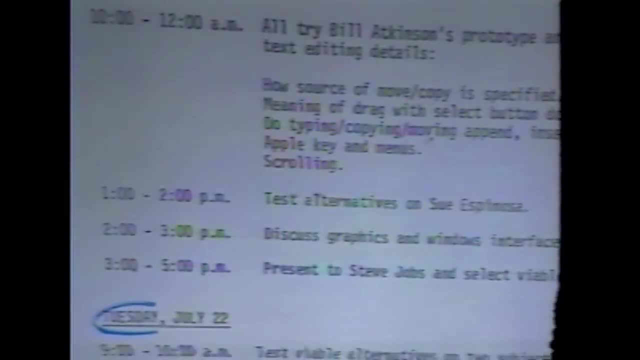 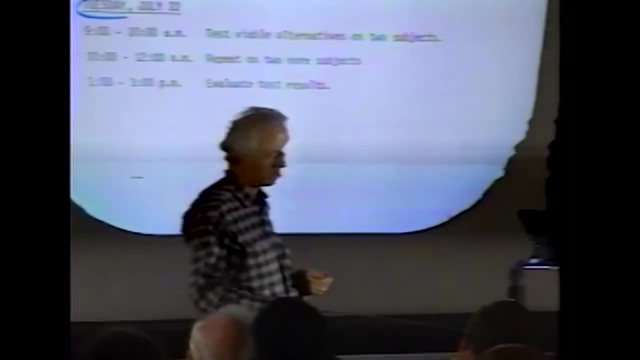 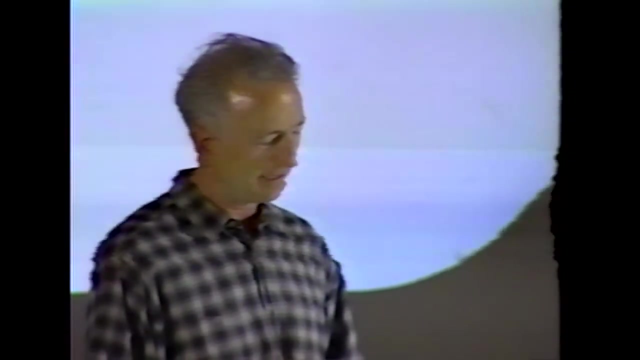 we would present this all to Steve Jobs and Steve would make the decision, which we knew would be definitely forthcoming. And then, on Tuesday, we were going to take the things that Steve liked and we were going to test them on subjects from 9 to 10.. 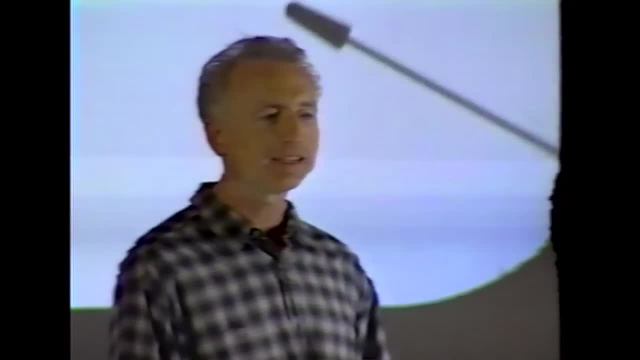 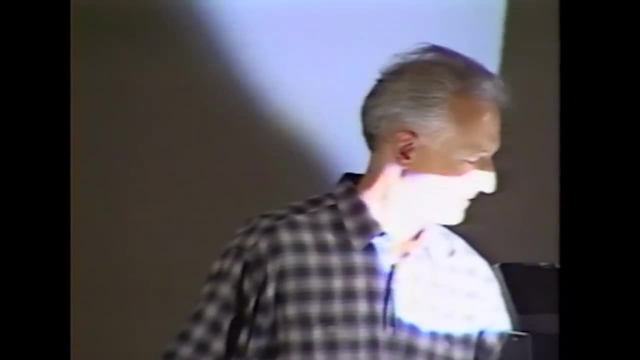 Two subjects, Two more subjects, from 10 to 12. We must have figured we would be slowing down by then. 1 to 3, we would evaluate the test results. So that was it Okay. so remember that was supposed to be July 22nd. 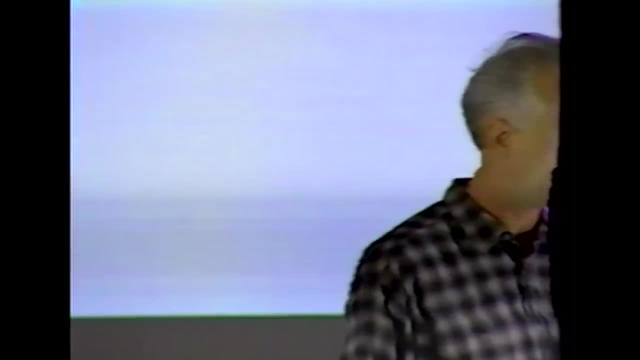 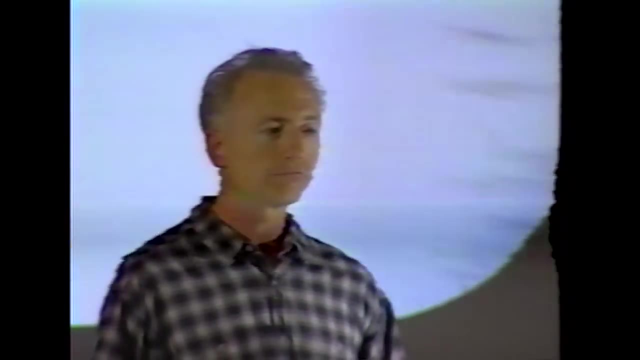 Okay, so now the rest of the, for the next 15 minutes or so. keep in mind that that was the schedule for July 21st and 22nd. Okay, well, we actually did that. We did all those tests. 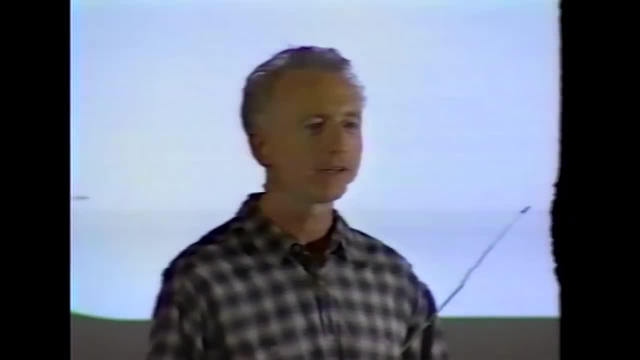 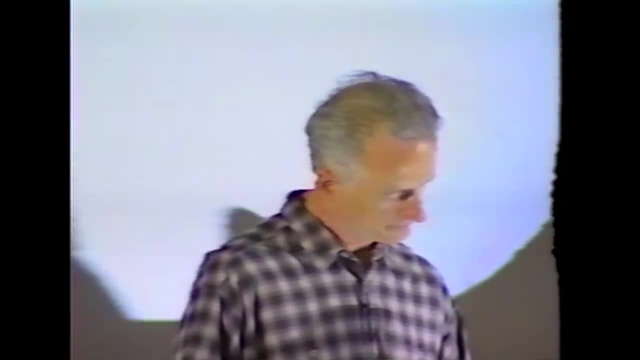 We did talk to Steve Jobs. He gave his opinions, We did some more testing And then Bill went to write up a user interface specification- external reference specification. I was a little worried because we hadn't really done extensive testing, but we tested a couple things. 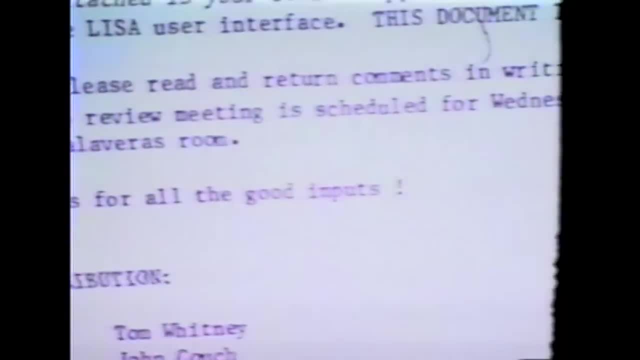 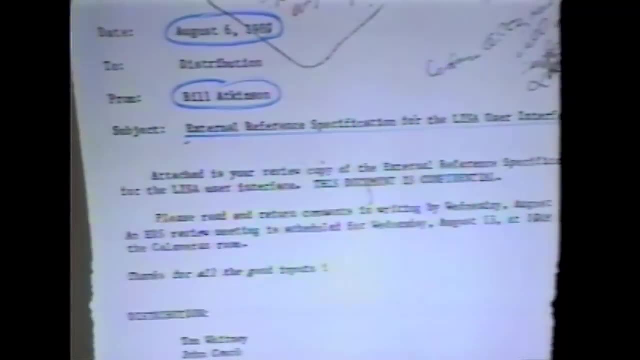 So this is dated August 6th, which was, as you may notice, a few days later than the deadline date that we had provided, but it took a while, And it said that you had one week to review and return your comments. 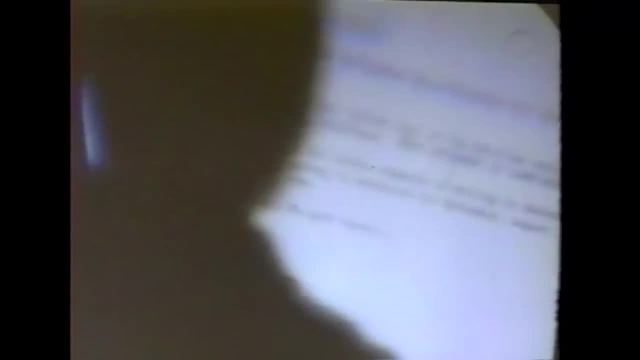 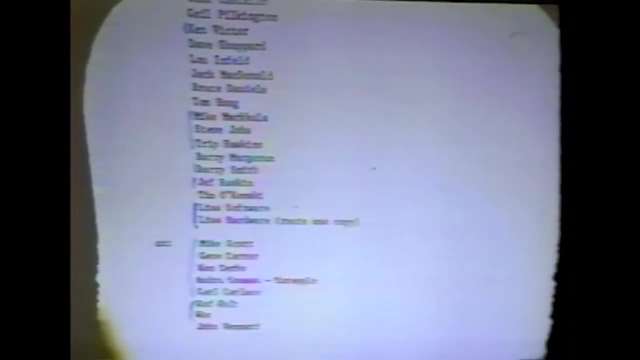 So we were already starting to slow down a little bit here, And let's look at some of the names of the people who got this memo, because it'll turn up to be important later in the story or just interesting right now. Ken Victor. 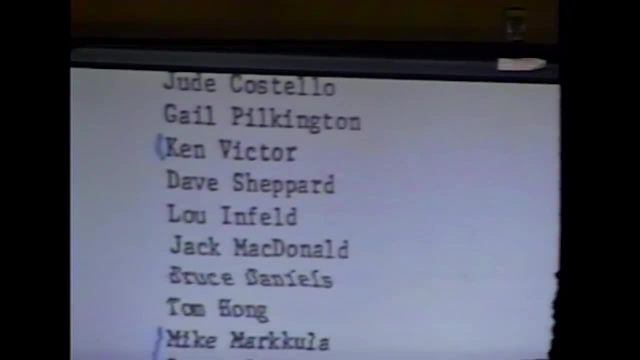 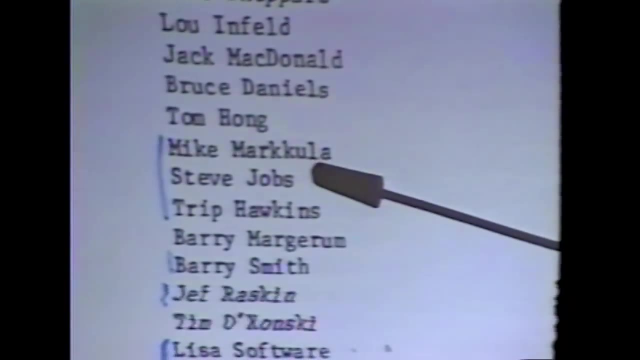 who is going to respond to it later, and Jeff Raskin. also Barry Smith. In addition to that notice, we sent it to Mike Markla, who is one of the founders of the company, and Steve Jobs, Trip Hawkins, who is the head of product marketing. 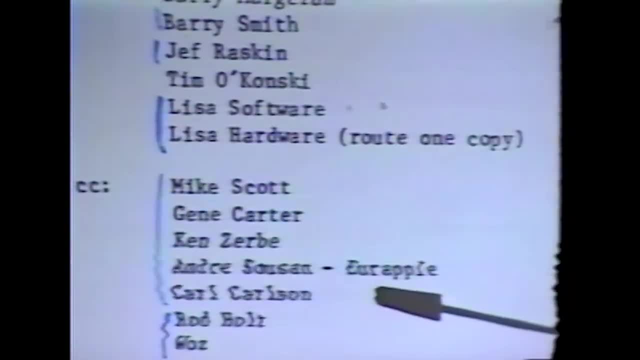 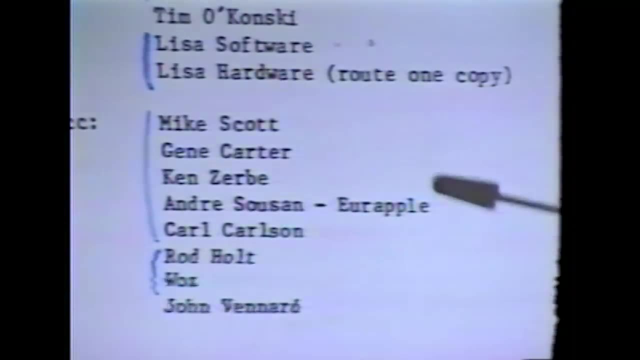 We sent it to everybody in Lisa's software group. We only sent one copy to Lisa Hardware. They get to share. We sent it to every vice president we could think of and to our two people who became Apple Fellows somewhat later, Rod Holt and Steve Wozniak. 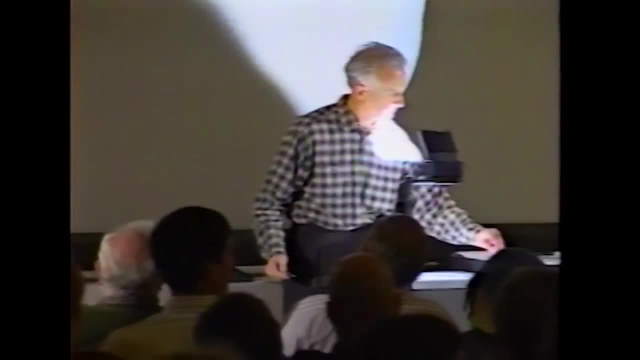 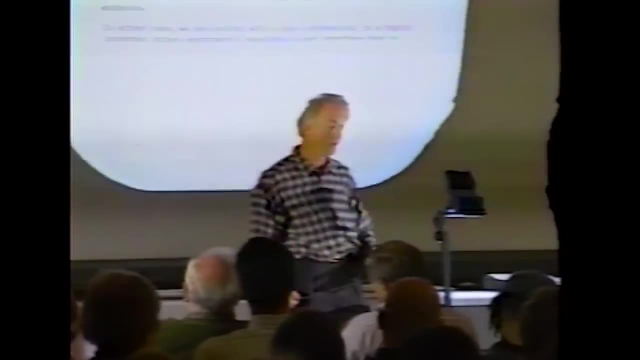 who's here in the back today. I don't know if he remembers receiving this memo, But he probably does. It was pretty dramatic, Okay, So we did some. I think we did some things right. Bill started out by talking about who is the customer. 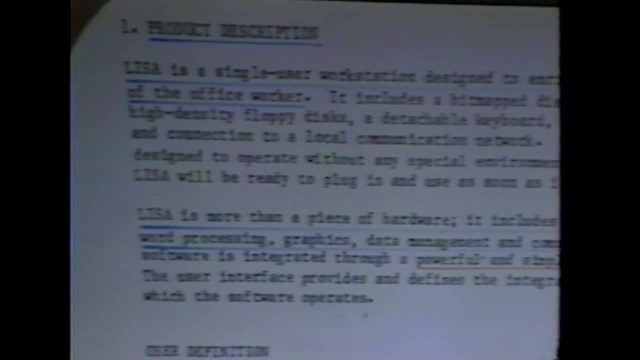 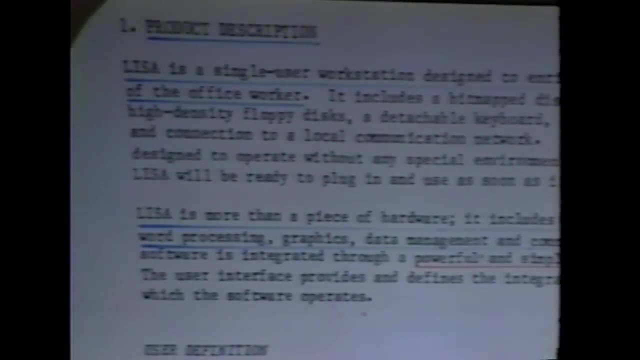 So it wasn't just some easy to use computer. It was an easy to use computer for specific people. So what was it? First of all, it's a single user workstation. That was an important point in those days. Well, still an important point. 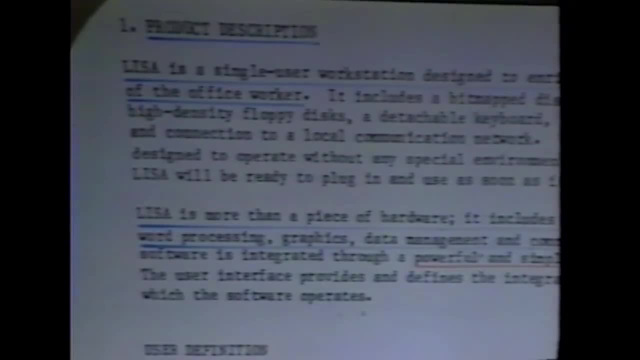 if you work at Sun or something- And designed to enrich the productivity of the office worker. So our market was office workers And it went on and talked about the hardware and so on. It's more than a piece of hardware, though. It includes major software. 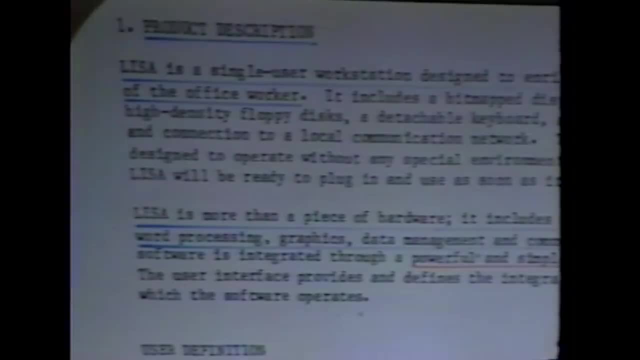 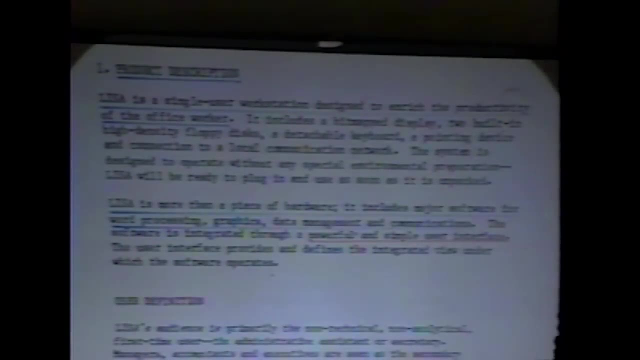 and we had specific applications in mind: Word processing, graphics management and communications. It wasn't intended to run thousands of applications, Not the Lisa. The concept that Trip Hawkins had was they had done studies and they found that most people on the Apple II 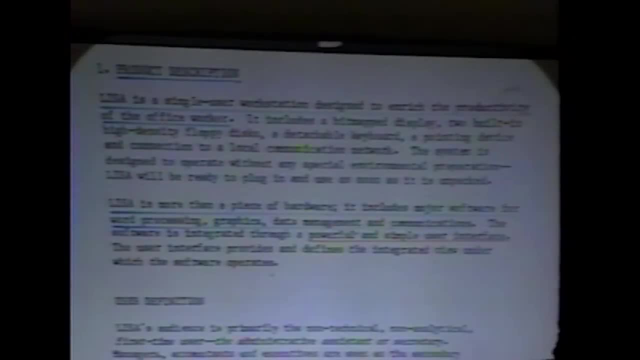 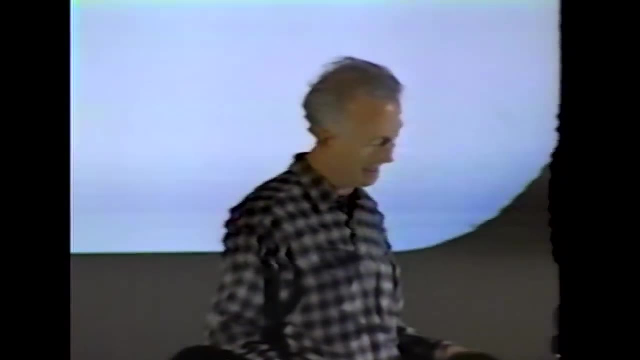 ended up using only two or three applications. Therefore, this was the great leap. all we need to do is provide two or three applications. That's all anybody will ever want. It was an interesting theory, And Apple funded a whole project based on that assumption. 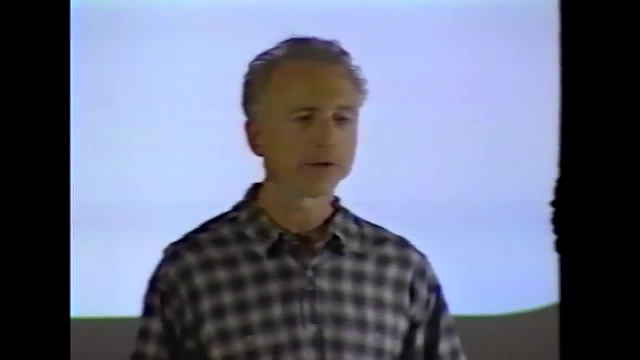 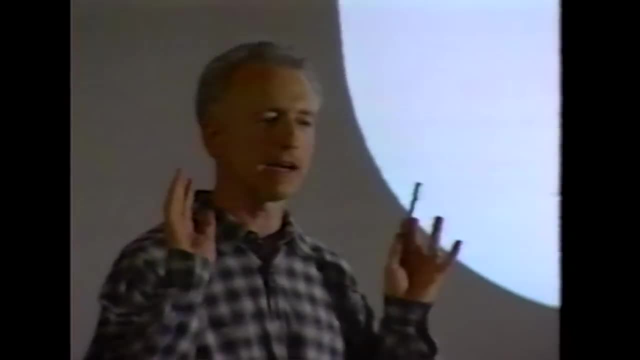 And then it said: the software is integrated through a powerful and simple user interface. And it doesn't say it here, but John Couch, who was in charge of the Lisa project, did a sort of Kennedy, we're going to send a man to the moon. 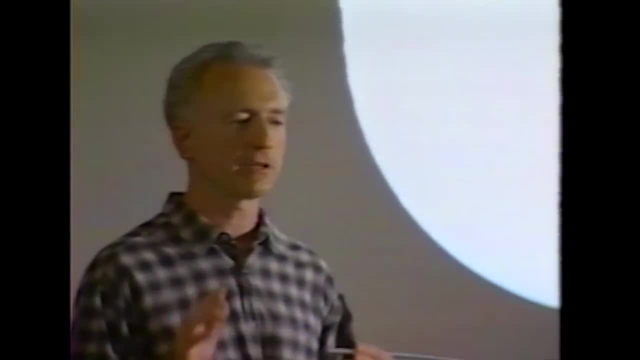 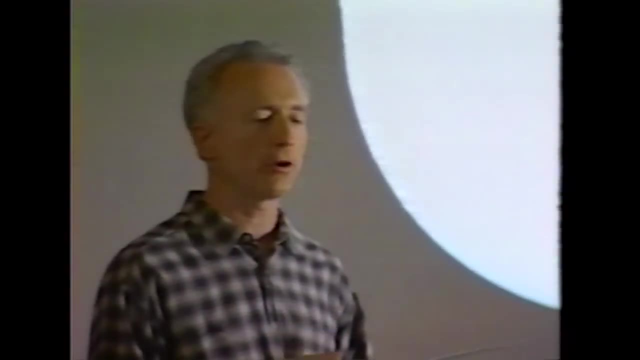 and bring him back thing He said. all I want is I want to be able to go into a spreadsheet, make some, put some numbers in, go and graph them, take the graph, paste it into my word processor document and include it in a report. 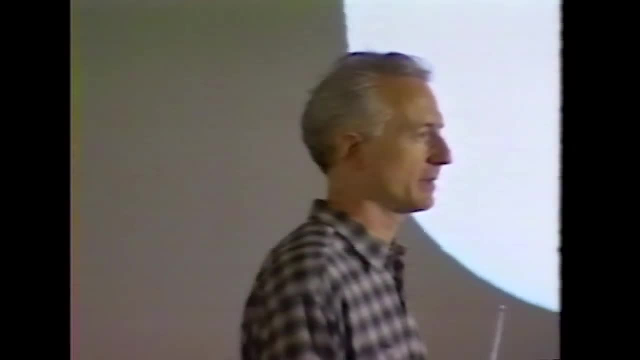 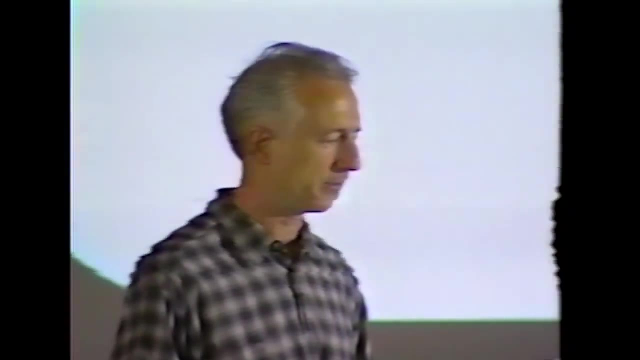 He didn't say paste, you know, put it in my word processor document. He said I can do all those things in an integrated way. then we'll be way ahead of anything available on the Apple II and all these separate programs that don't interact with each other. 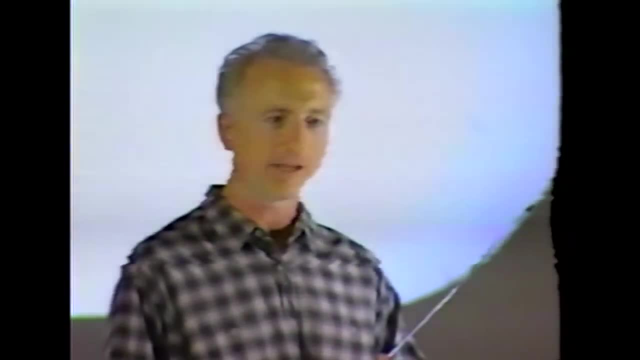 That's all he wanted. Whenever we brought him any issue, he said: remember what I want. and he went through the whole mantra And that was a very healthy thing. It kept us focused And then we also knew when we were done. 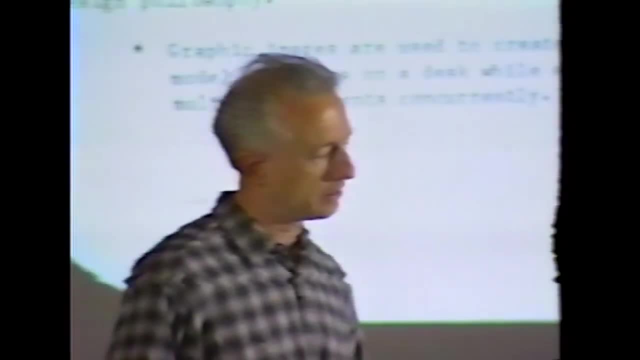 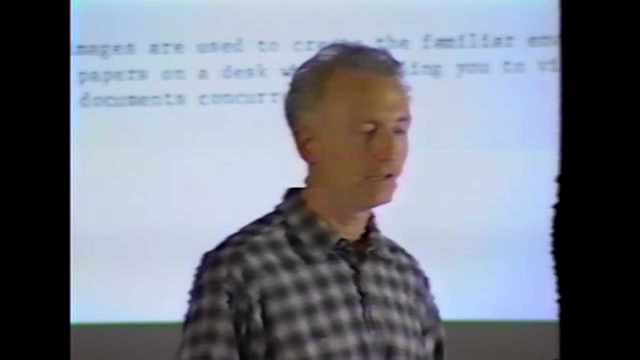 Well, who were the users? Non-technical, non-analytical people- Non-analytical- it's a very important point. First time users: Well, in 1980, there were a lot of first time users, almost everybody. 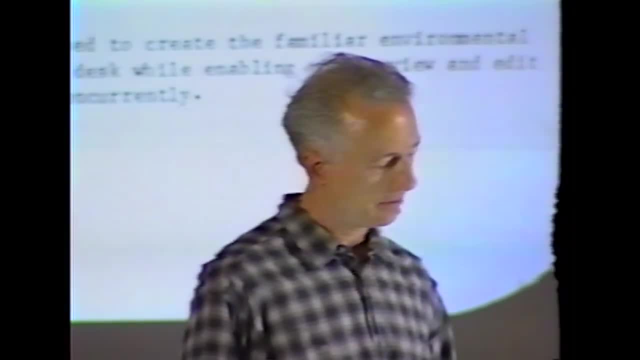 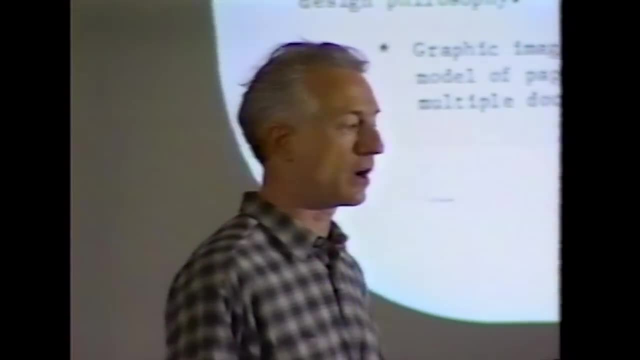 And here are examples: administrative assistants and secretaries. Also, secondarily, managers, accountants and executives. It wasn't for programmers, It wasn't for kids, It wasn't for people at home doing recipes. This was an office system. 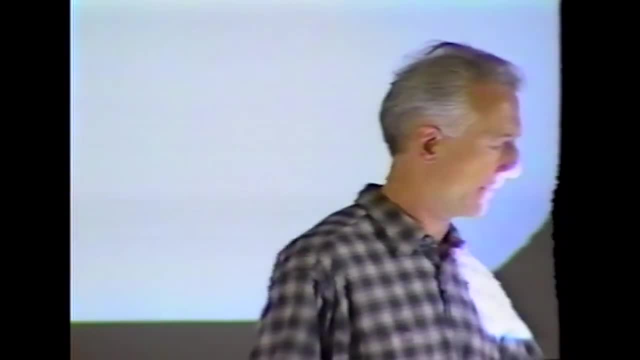 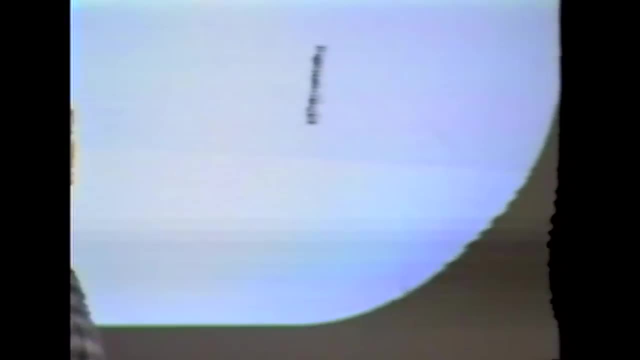 And so when you start looking at it and comparing it maybe with the Mac, you'll see some differences based on that, And you may see some similarities to Windows Design philosophy. So there was a whole section on the design philosophy and what were the most important. 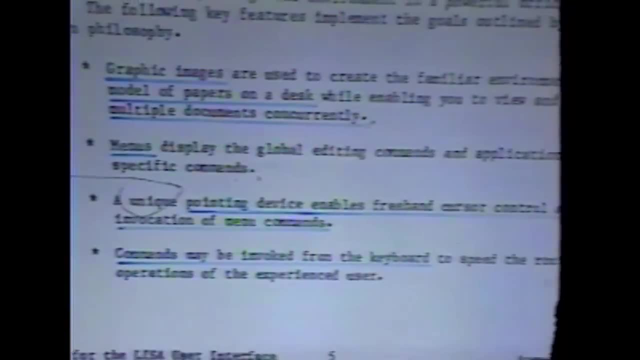 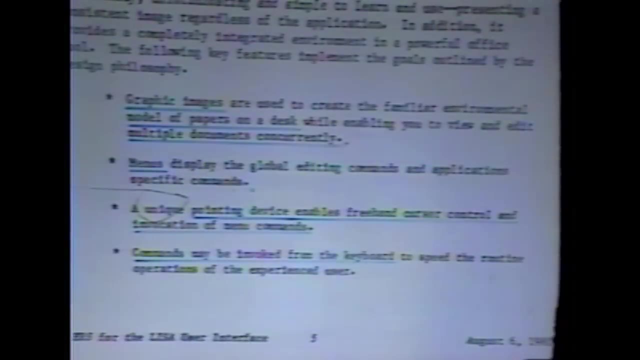 features to put in Graphic images. Well, it's a little bit very vague: Menus, A pointing device that you could move around freely, as opposed to the cursor keys we were using up to then And we were gonna let you invoke commands. 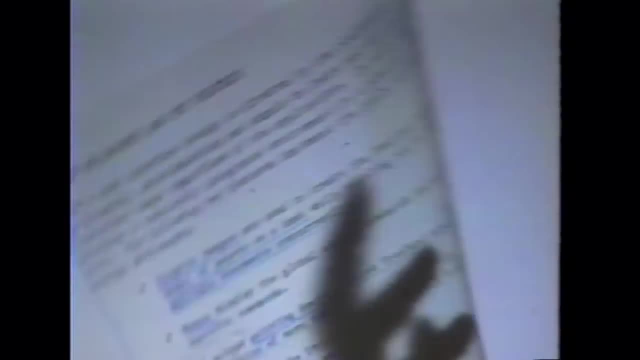 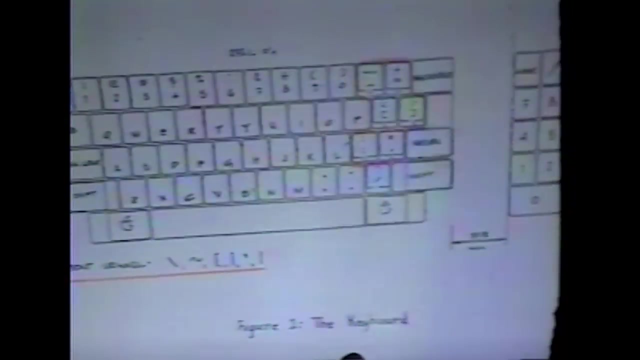 from the keyboard, also because there were times when you would do things over and over and people felt that sometimes the mouse slowed you down a bit. So let's look at this keyboard. This was the keyboard that existed on the hardware when I arrived. It had a code key. 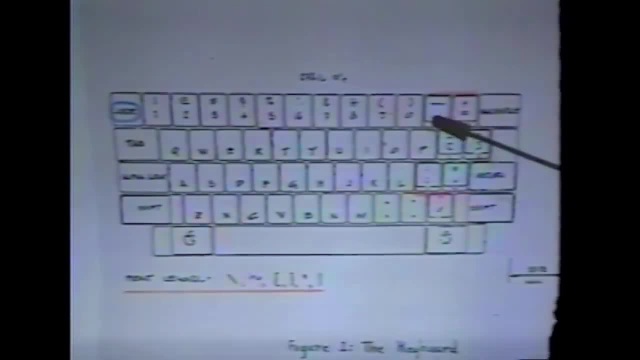 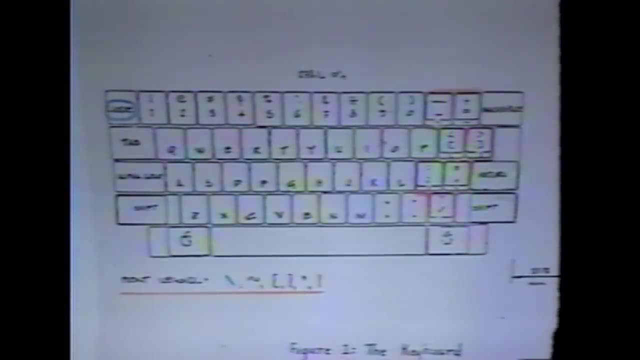 in the upper left corner And some of the keys on their fronts had some characters. In other words, in order to make the keyboard the width that they wanted, they couldn't fit all the characters on the keys, So they squeezed a few extra characters. 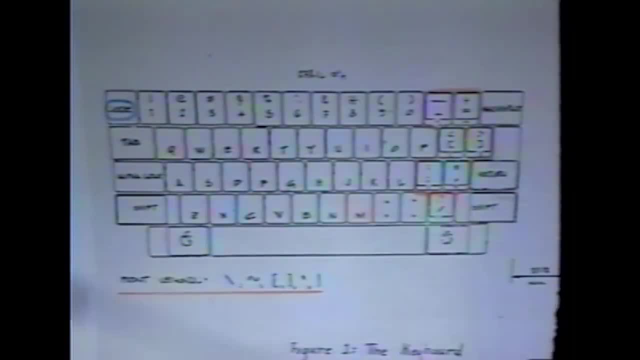 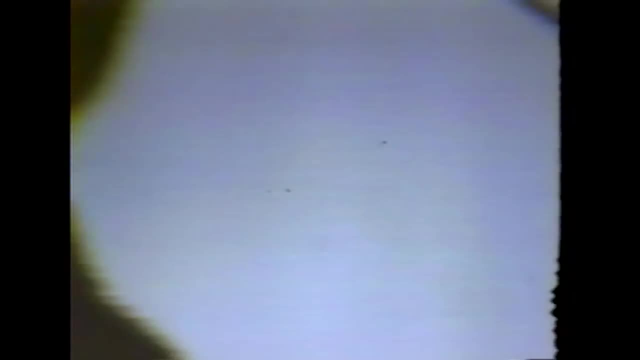 on the fronts of the keys and then had a special key to invoke those, And later we decided we could use that key together with other keys to do another function that you'll see later. Now I didn't like the hardware design too much and I wanted to change it. 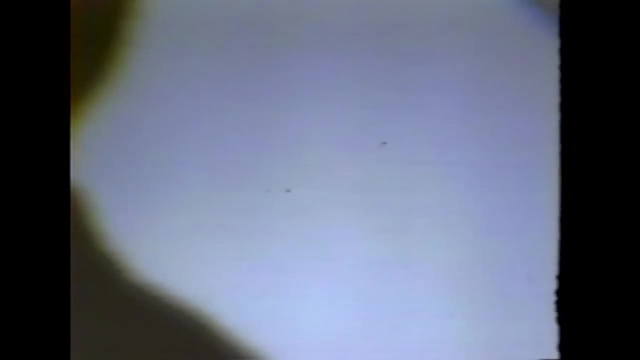 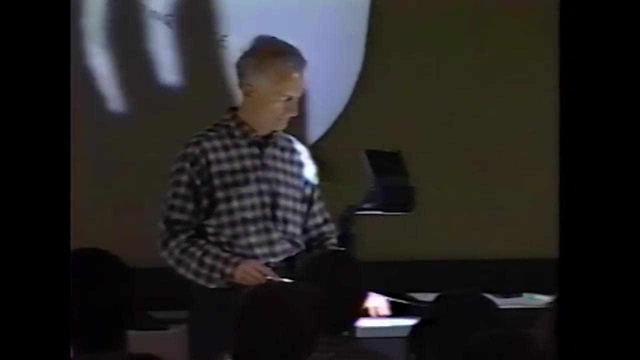 but they said: you can't change that, You know, you just have to ship the hardware that we already built, Otherwise we won't be able to ship this product when it's gonna go to market. I said: oh, when is that? 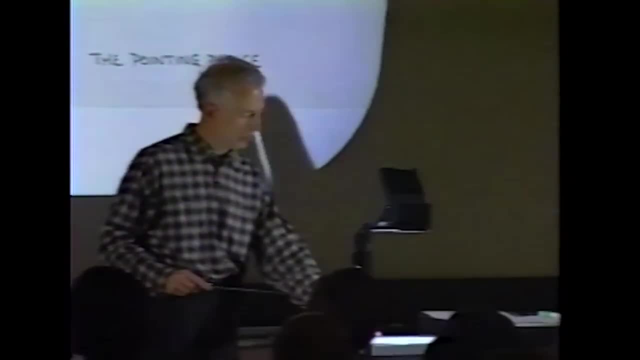 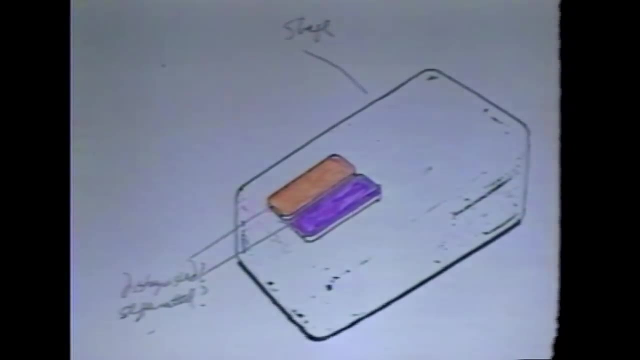 And they said six months. That was 1980.. To jump ahead and ship till middle of 83. Probably my fault, Okay. So here was the pointing device. It's kind of a brick, That's a mouse, And 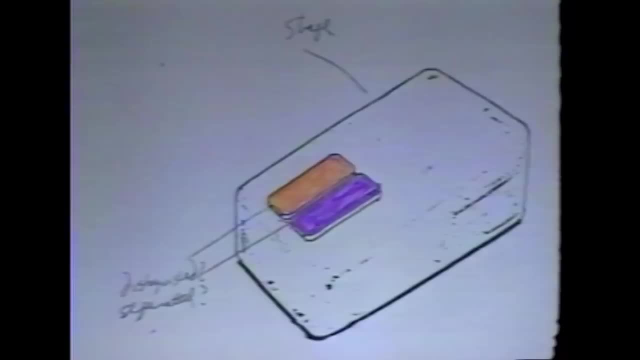 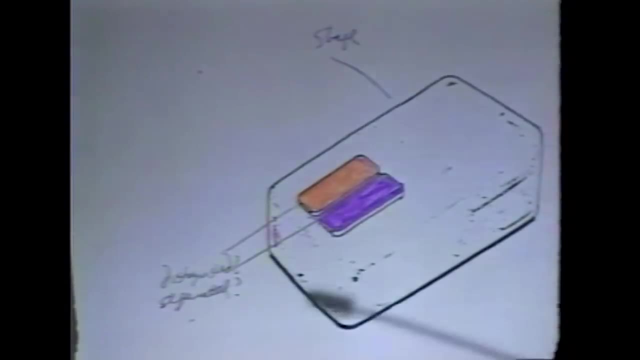 the color is me. I added color last night just to highlight things you should look at. But it had two buttons at that time and I hand wrote on here the shape And I wasn't sure what distinguished these two keys and whether there was. 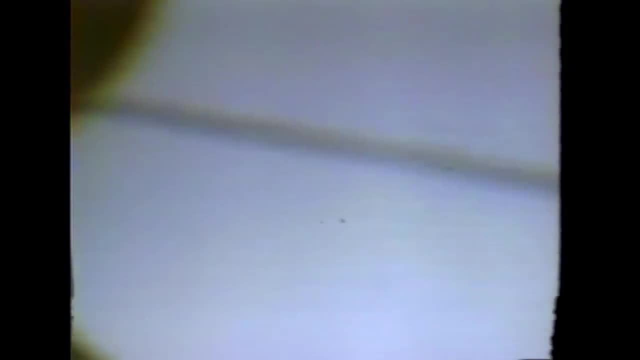 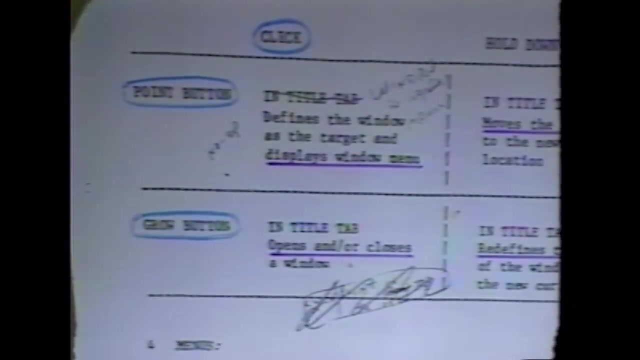 a little space between them where they were flush or what. So you'll see some of my handwritten scribbles on these memos, And here's how the mouse was used. Well, actually they didn't know a lot about how the mouse. 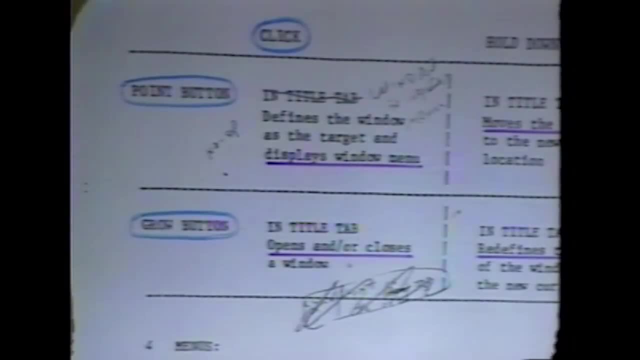 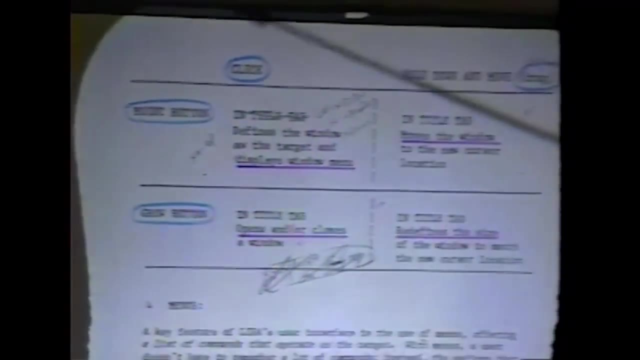 was used, yet They mostly were focused on the window manager, How the user would manage the windows on what we now call the desktop, And so at that time the idea was this: There would be a click and a drag And 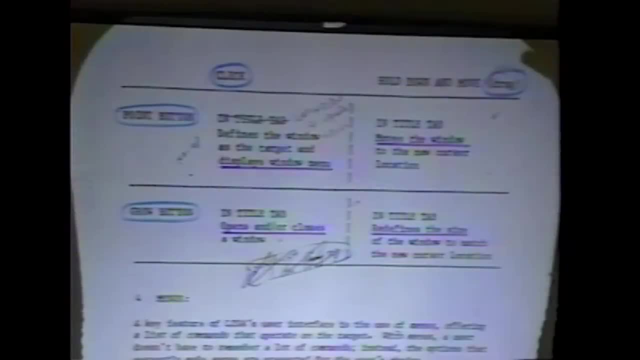 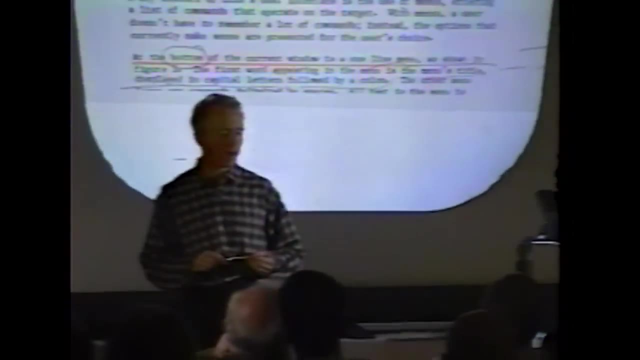 you could click, hold, drag the mouse and let go, And sometimes we called it drag, Sometimes we called it draw various names. And then there was the buttons, got names: The point button and the grow button, And depending on where you pointed, 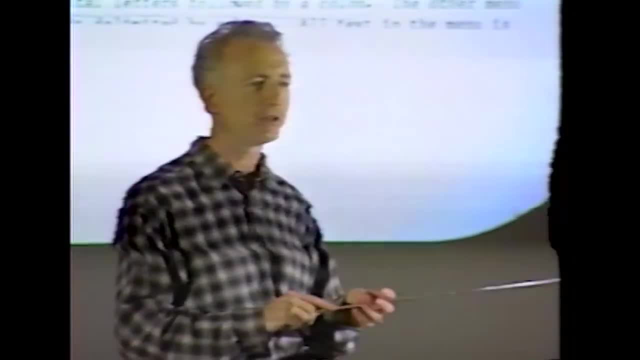 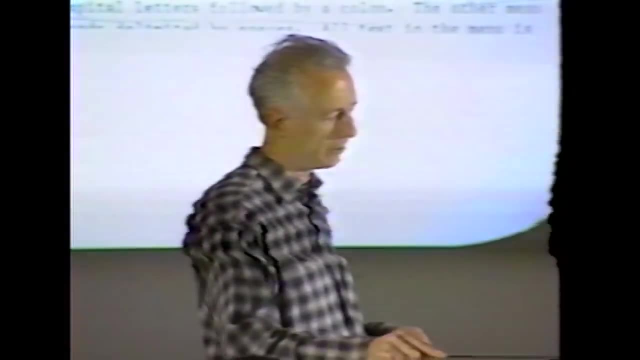 and whether you clicked or dragged, you know which button you used. this page here shows what happens. if you went into the title tab of a window- the little thing that had the name, And it either would display the window menu, move the window. 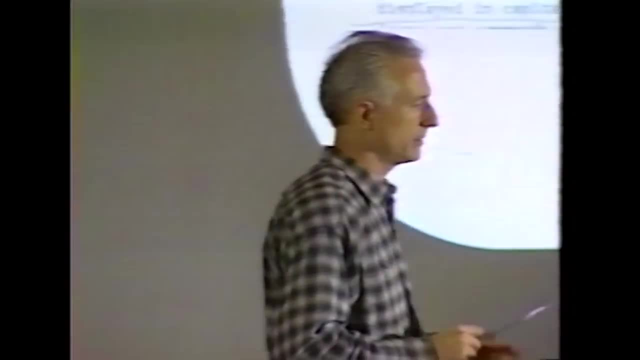 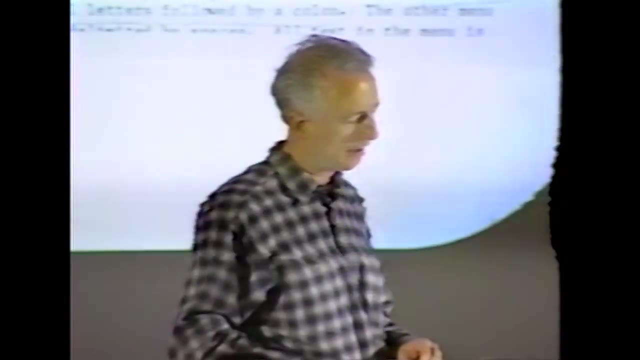 open or close the window. so there was no grow box in the lower right, There were no menus. It was all done with just one or two mouse buttons and a click or drag operation. Now there was a menu at the bottom of the window. 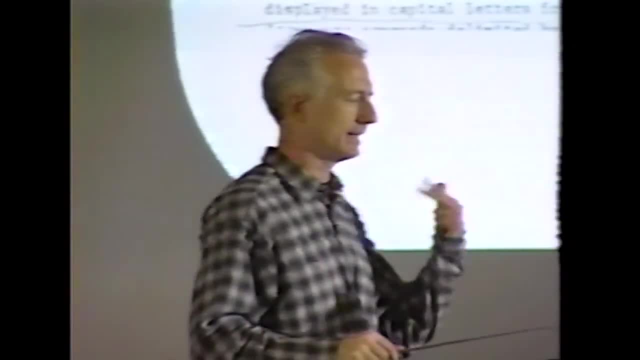 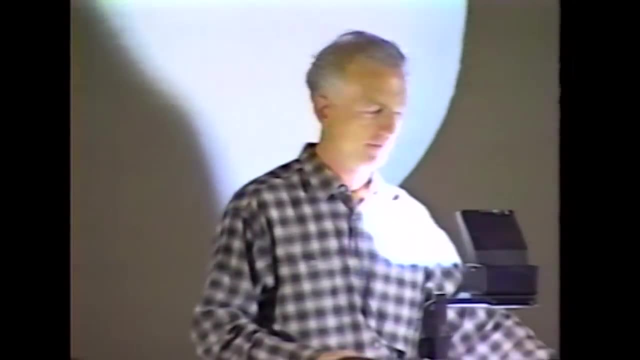 but it had nothing to do with window operations. It had to do with operating on the content inside the window. We'll get to that Now. I should stop saying when I got there, because by then I'd already been here for two weeks. 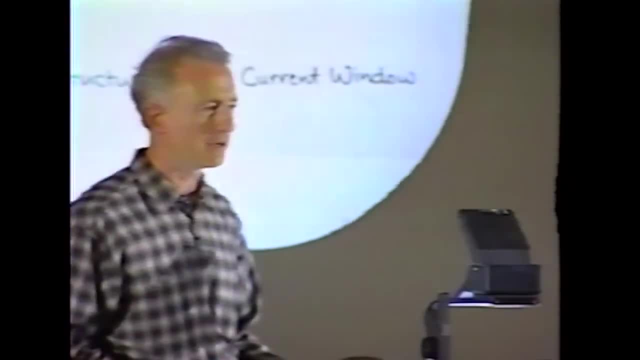 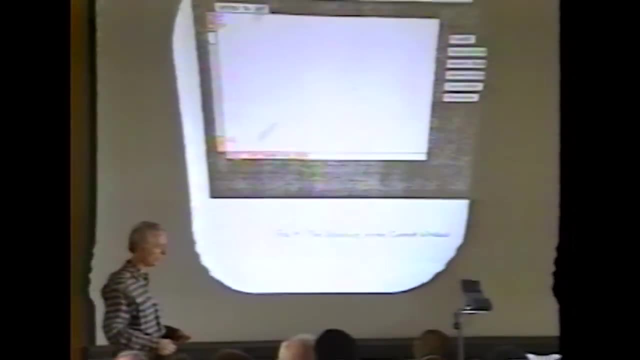 So I had some influence on this, I can't remember what, So this is Jeff Raskin, who does spell his name that way, And he was for some reason became the person who we were always sending letters to on the Lisa Project. 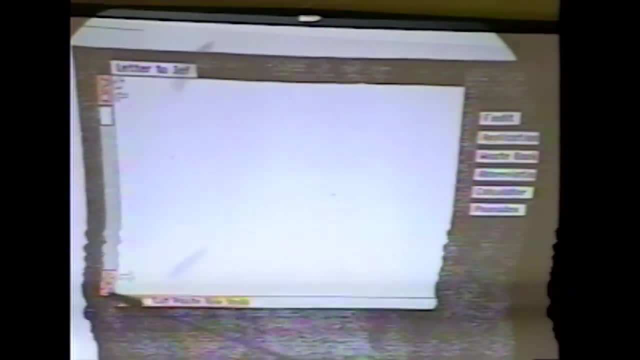 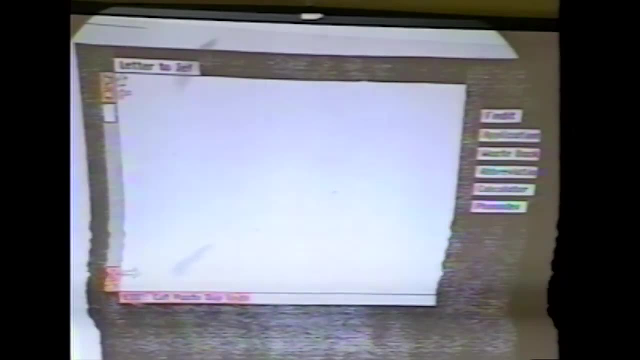 And, as you see, the scroll bar was on the left side. It had the horizontal scrolling arrows at the top, the vertical scrolling arrows at the bottom. Now, those of you who know the Next machine know that. that's the feature is that you have. 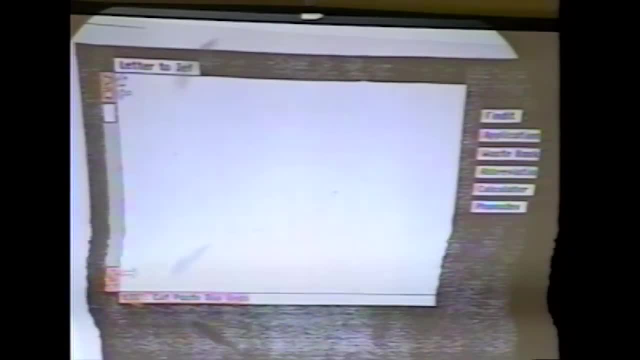 the two arrows close to each other so you don't have to move very far to go between the two arrows. That was actually designed by Jeff Paste Dupe to copy things and undo, And then on the side there were the equivalent. 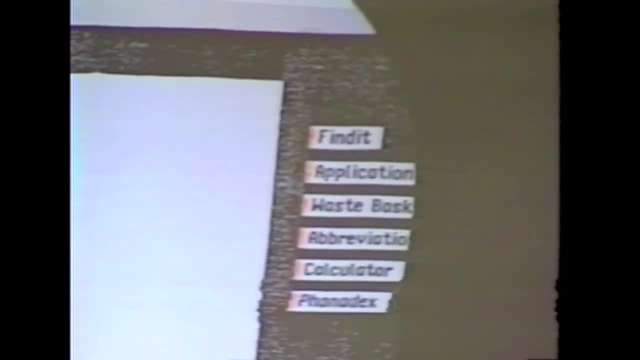 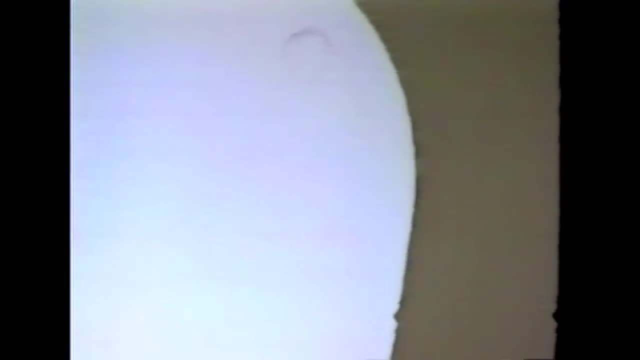 of today's icons. This was taken from Smalltalk, where you took the tab of a window, threw away the window and just kept the tab, called it collapsing the window, And these were windows that were available but closed right now and you could open them up. 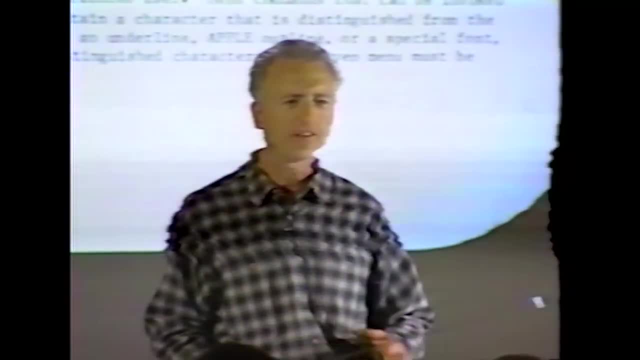 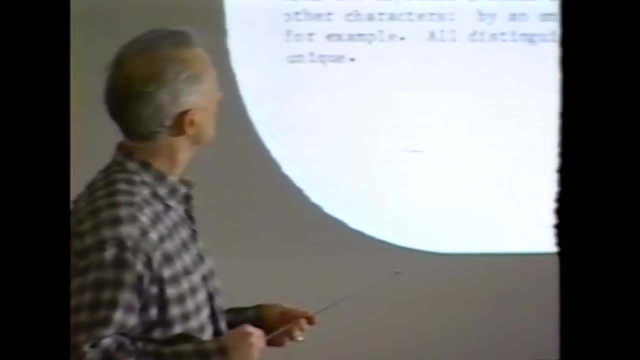 Okay, Then we had this idea of fill-in menus. They're what, just to jump ahead, they're what we call highlight boxes today, And there were two kinds. There were kinds where you somehow open a sub-menu and you get to type: 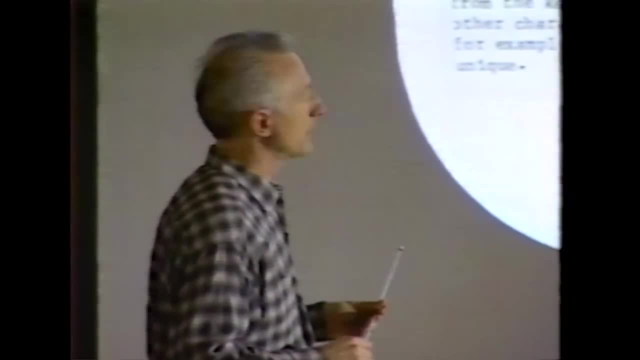 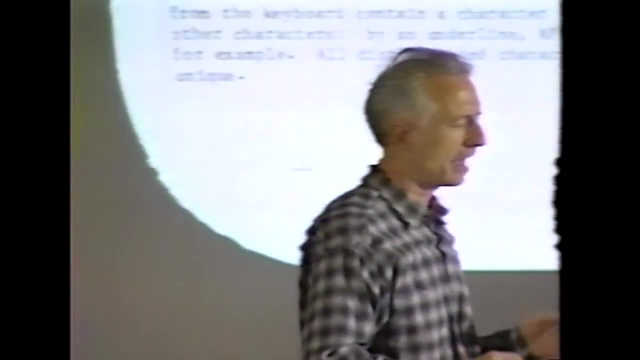 into that sub-menu- Don't ask me exactly how- And the other was where it actually opens up a big box. like we know today, That was this thing called Forms, And so it was a kind of a vague notion at that time. 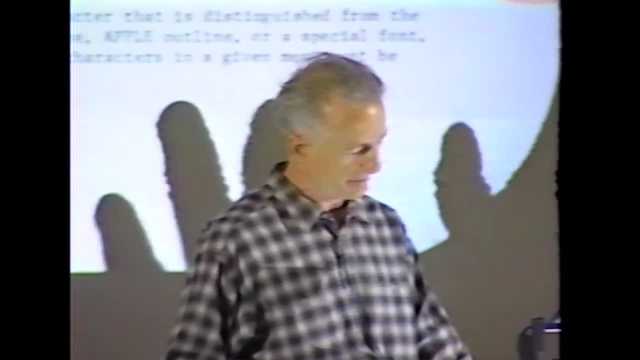 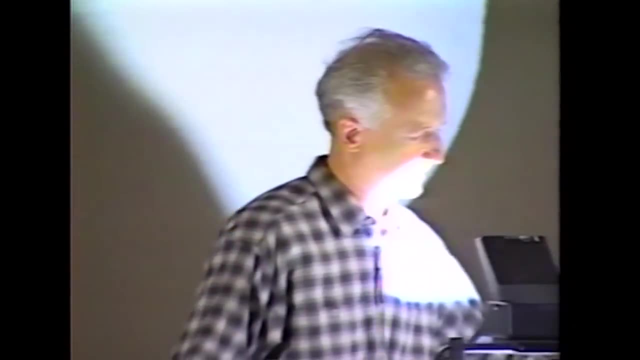 No one had actually drawn any pictures even of what those looked like, I think. And again, we said that menu commands can be invoked, and I wish I could remember what I disagreed with. I think I was afraid they would do too much keyboard stuff. 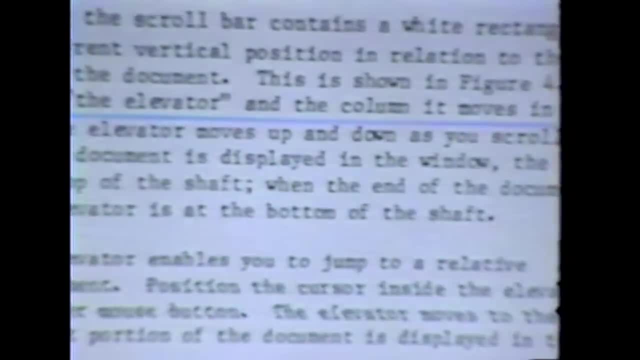 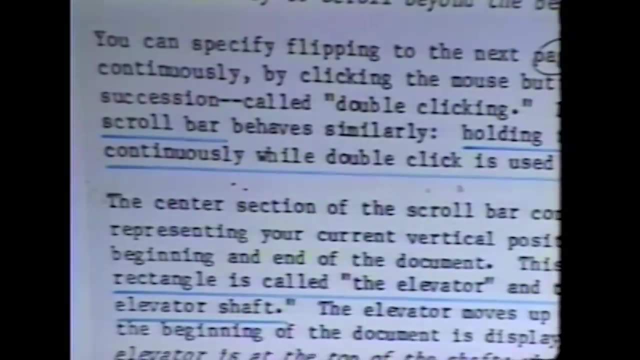 There were scroll bars and you would hold a button down to scroll continuously. Now there was an interesting idea here: that you could double-click to flip to the next page. Now anybody that knows about user interface design with single and double clicks. usually you make it so that 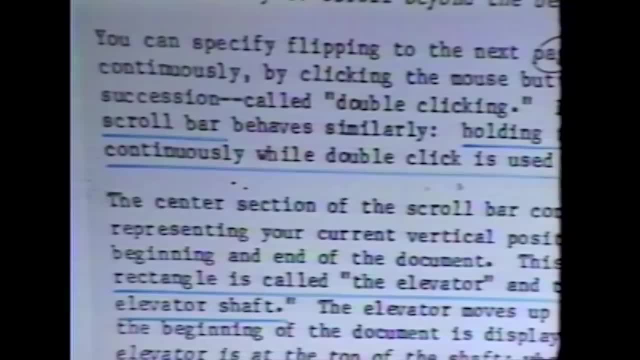 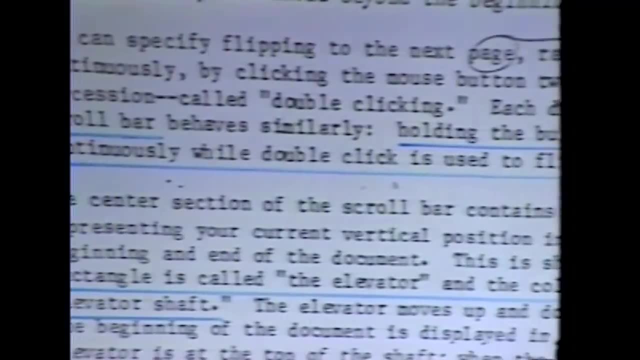 when you click once, you can start doing something, And then when the second click comes, it doesn't sort of negate what you already started to do. This is kind of interesting, because if you clicked once, it would sort of start to scroll a little. 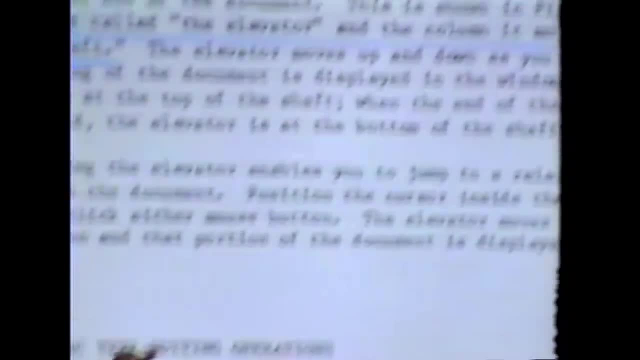 And then when you clicked the second time, it would realize you wanted to jump a lot, So you'd get a little motion and then a jump, which actually might have been kind of cute, But I don't think we ever implemented it. 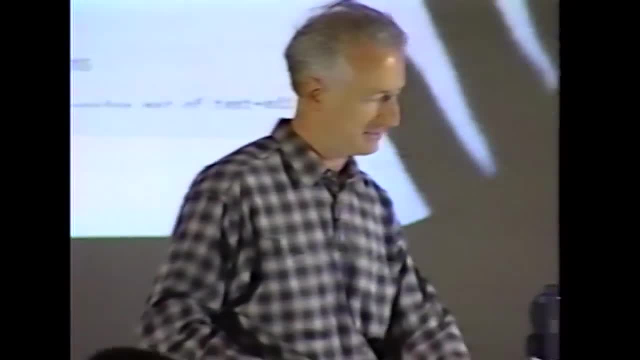 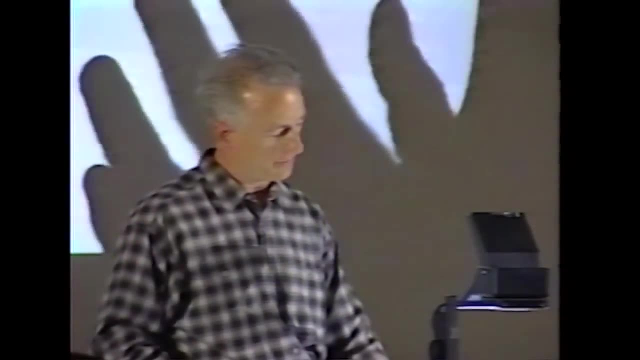 Then there was something in the called the Elevator Shaft with the elevator in it, And that was what is still today, that little box in the scroll bar that you see. There was the Abbreviations window. That was that code key. 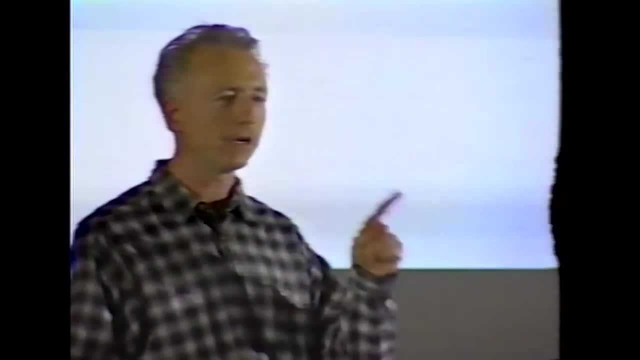 We had to find a use for it So you could type code and then hit a letter on the keyboard. It would look up in a table and it would expand your abbreviation. This was kind of take the kind of thing you'd find. 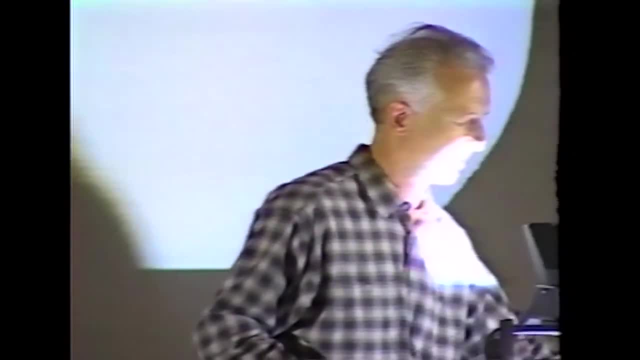 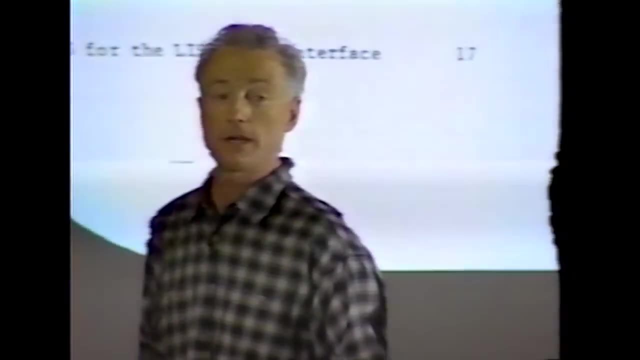 in a Wang word processor, So we put that in, because this was for secretaries. Then there was something called the System Error Window, And that's what you now know as alert boxes in Mac and Windows, And these were things. 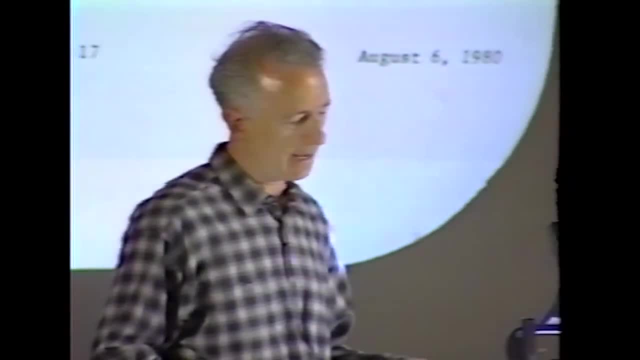 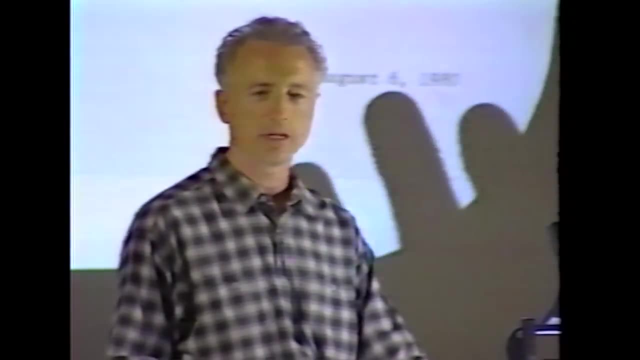 that would come up when there was a problem And it would make some kind of beep and it would tell you what the problem was. So I put a little question mark here: Is the system frozen when that comes up? Can you do other things? 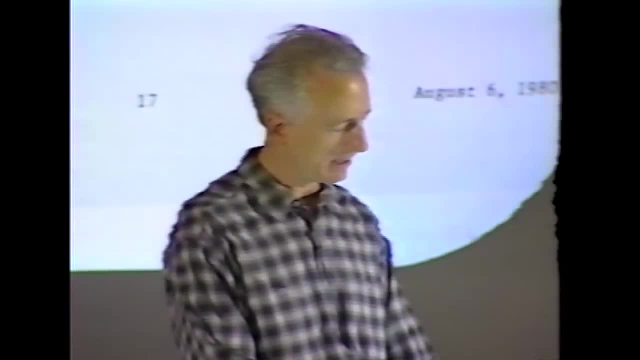 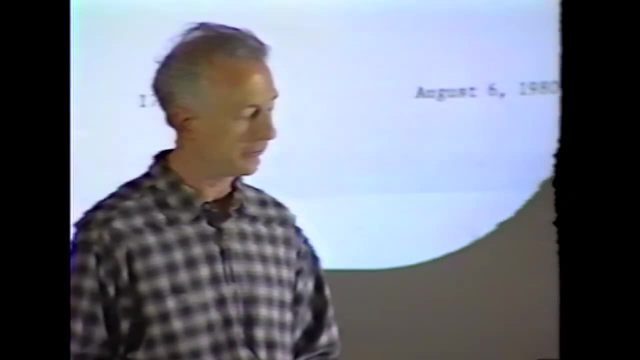 And we eventually decided it was modal, But actually that took quite a while to decide. Now we talked about testing. We said that the design is already based on studies of user reactions to various models And, as you saw, 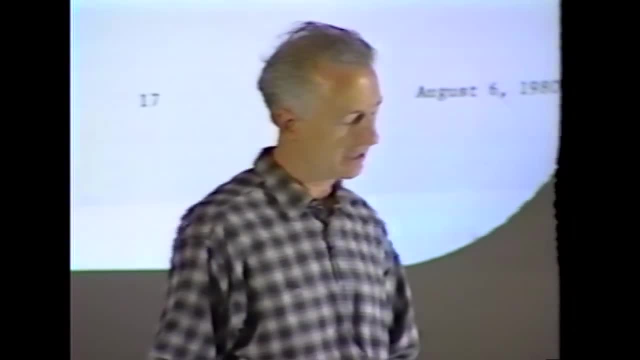 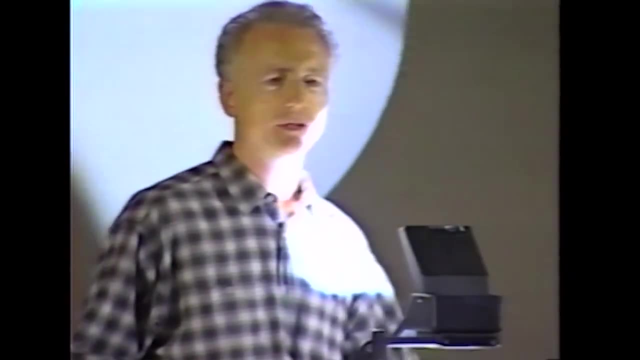 we did three or four hours of testing And we're going to do more testing and avoid any glaring design flaws. I was happy that that was put in because that meant we could go and fix the problem And I was sure it was there. 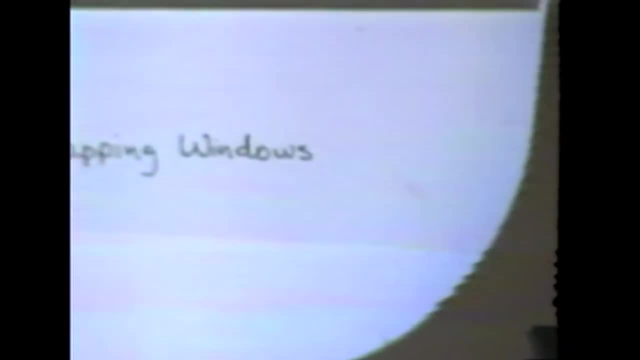 because we hadn't done enough testing yet. So what did it come down to? This is what it looked like. The basic model was overlapping windows, which is right. from Smalltalk, There was that box at the top, just like in Smalltalk. 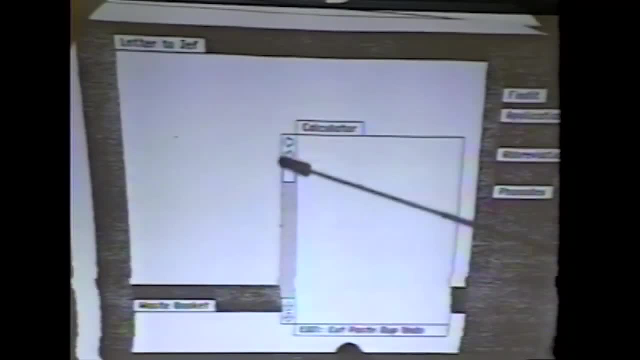 that little title bar. The scroll bar was on the left, just like in Smalltalk. only, instead of just that little box there were the scroll arrows there. We thought it would be nice to have something to point to In Smalltalk. 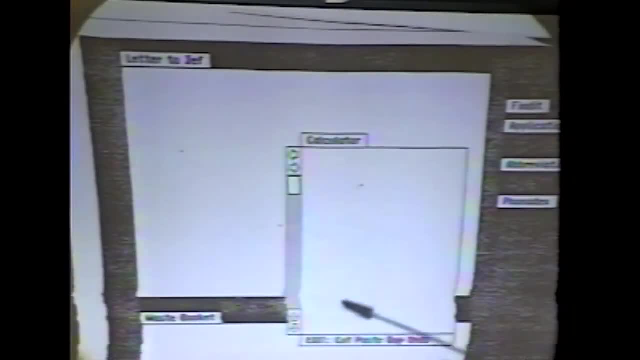 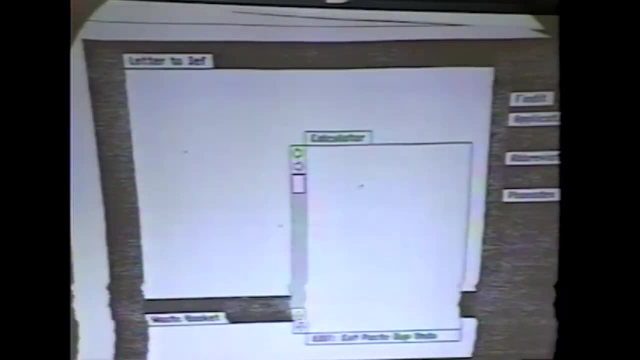 you push the button and then the arrows appeared And we thought that was a little weird And there was this menu at the bottom. Now, if any of you who's ever used something called UCSD Pascal, If you remember- 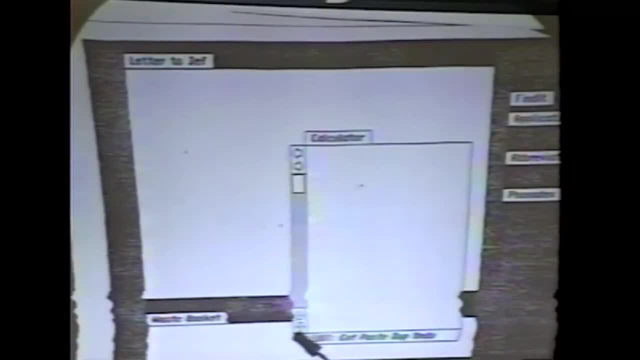 there were menus in UCSD Pascal And you would type the first letter of the menu name and it would bring up a sub-menu And you'd type the first letter of the menu name and you'd go through a hierarchy of menus. 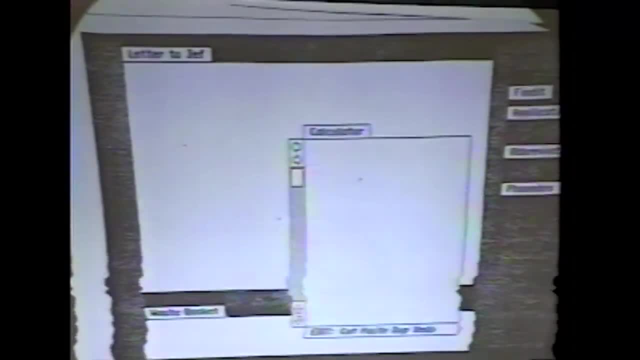 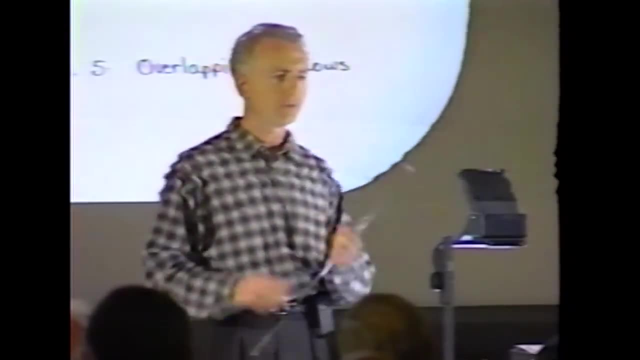 Now also, there was a machine- oh, I'm going to forget the number- a Hewlett-Packard computer 2000? No, it was a later model than that HP something thousand, that had a row of function keys. 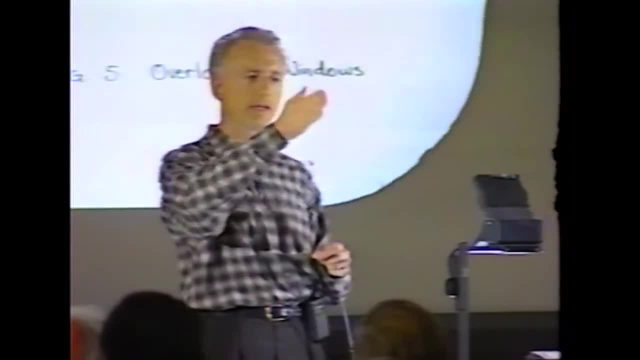 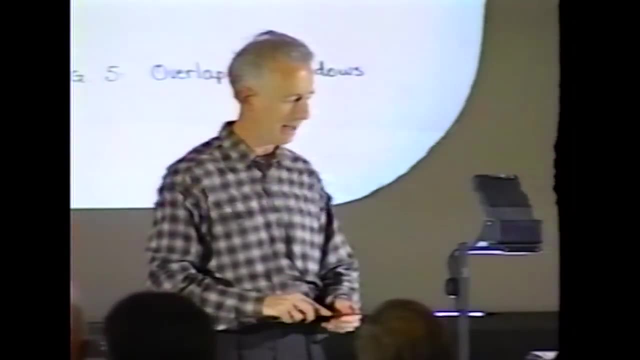 on the top of the keyboard and at the bottom of the screen under each key: Still have it, Still have it. And if you hit that key, that would activate that menu item. These were the two products that the authors of this interface. 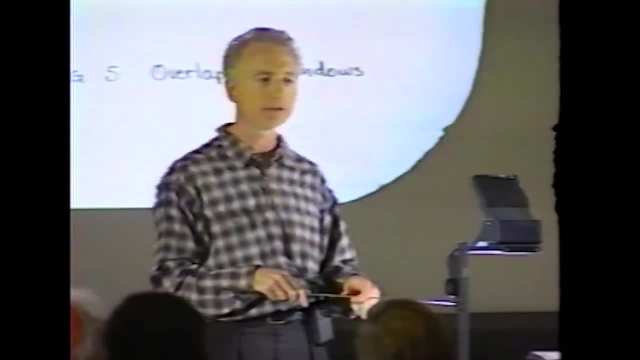 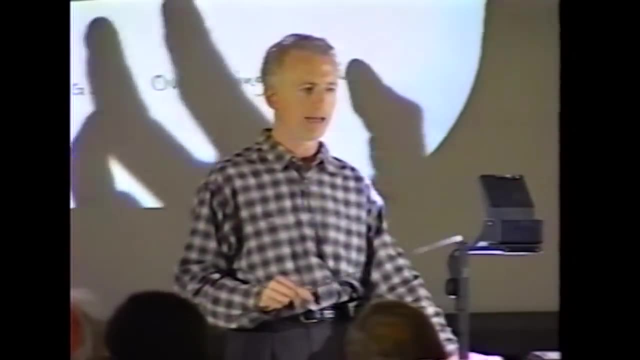 knew the best. They used UCSD Pascal to do their software development. Half of them came from Hewlett-Packard, And so this was kind of a blend, And so you could. they had function keys at the top of the keyboard. 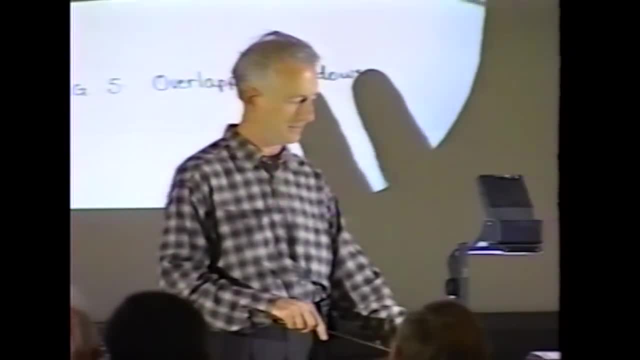 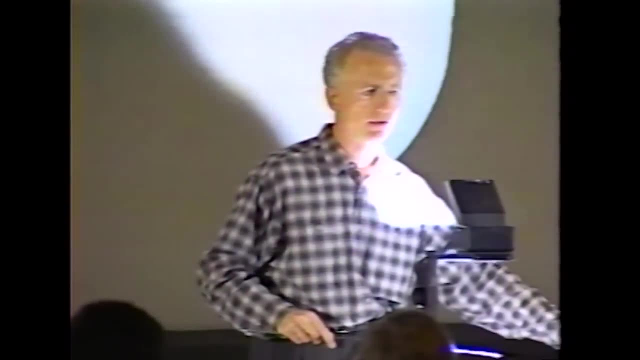 that you could hit that would invoke the corresponding things. And they also had these hierarchical menus that were straight out of UCSD Pascal- All right, Not the little pop-ups that were in Smalltalk. So that's where it was in August. 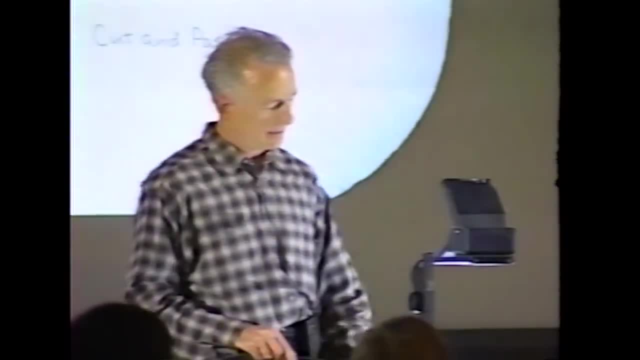 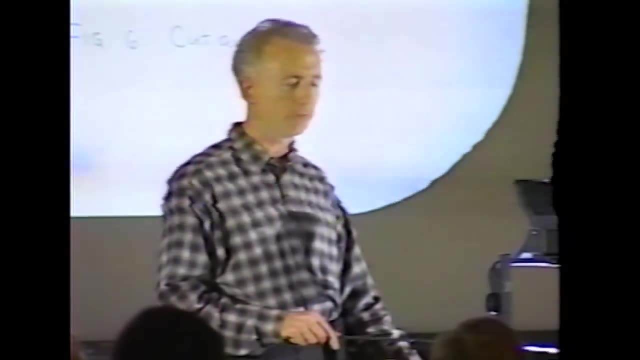 Cut and paste were two of the commands in the menu. That came from Smalltalk And, as you see, there was a waste basket. That's what you called the clipboard today. We used to call it the waste basket, Different from the trash can. 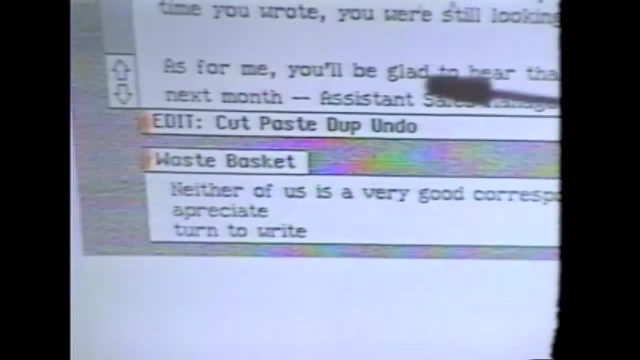 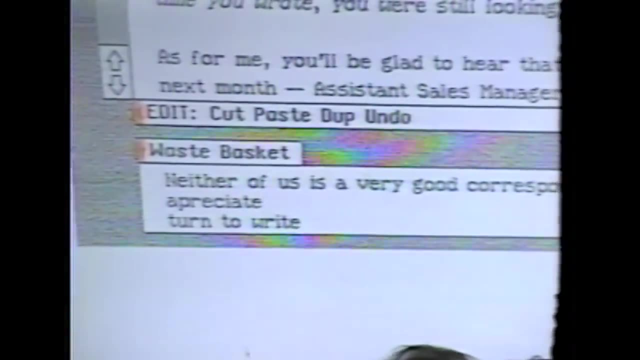 which was a confusion we had later And that's why we changed the name. But when you cut something and went in the waste basket, like in the office, you cut something and throw it in the waste basket, But then you could. 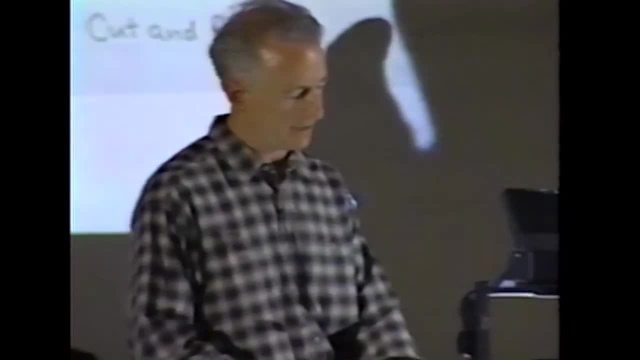 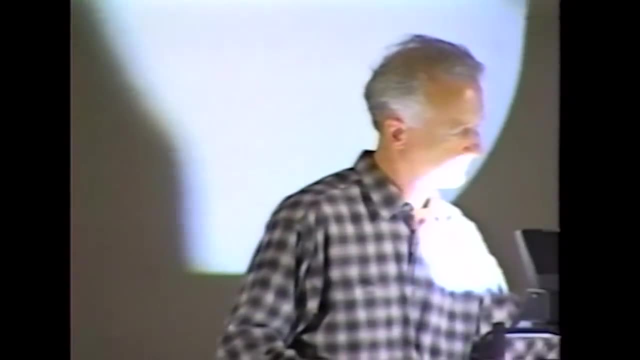 take it and paste it somewhere else, And it was sort of a waste basket, And so you'd select it with the mouse. Notice that when you select it, there's this little arrow here. That turns out to be a significant point later. 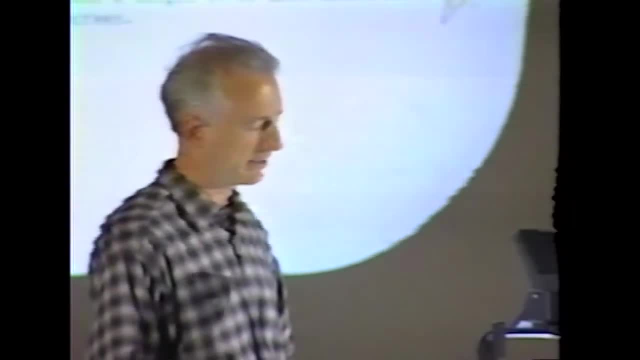 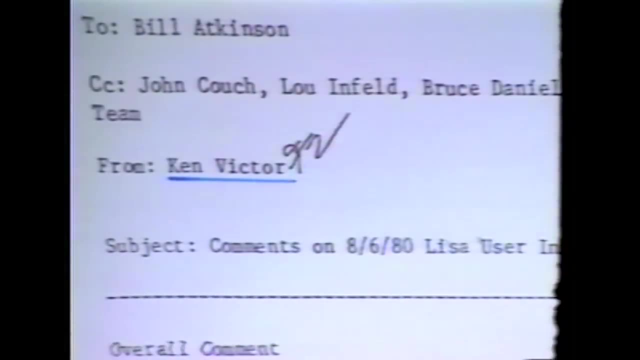 I'm moving fast because there are a lot of slides here. Now. Ken Victor remember. Is Ken here today? No, Ken was one of the reviewers of the document and he provided some input very quickly And he said: why can you only? 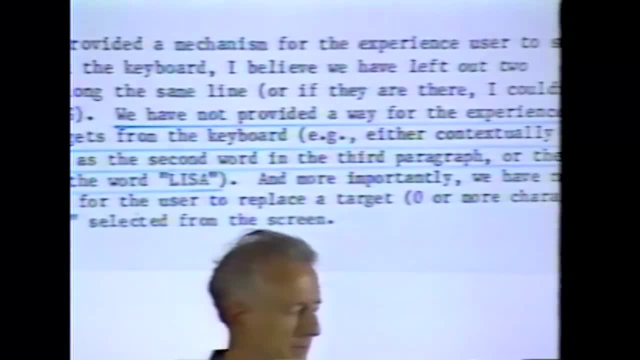 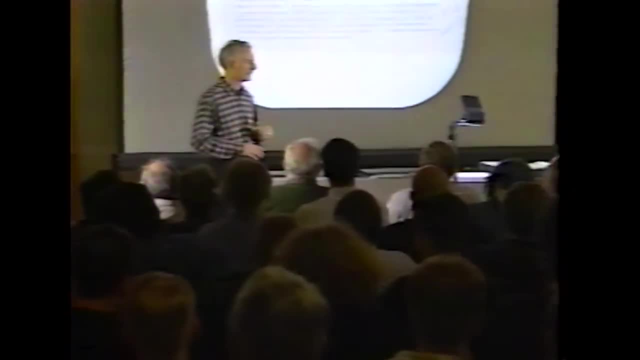 select it with the mouse. Now, this he must be someone who used Emax or something. He wanted you to be able to select it with the mouse, You know. fourth line, third word, seventh character, You know you should be able. 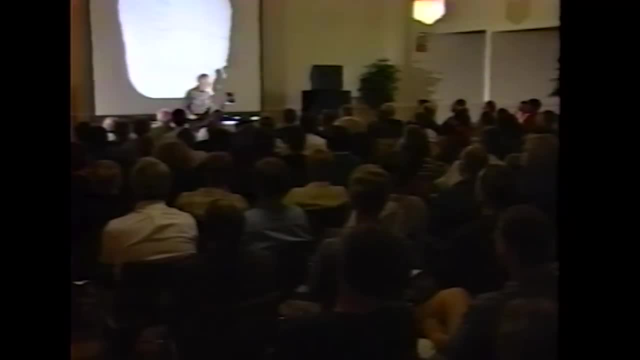 to specify what you want. And fourth occurrence of the word Lisa, you should be able to say things like that. And he was maybe years. either you know, he sort of didn't get it, or he was years ahead of his time. 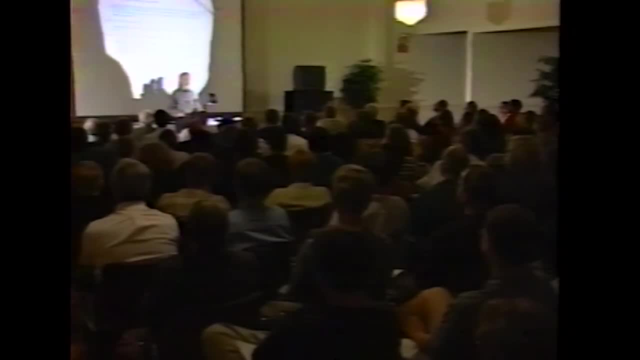 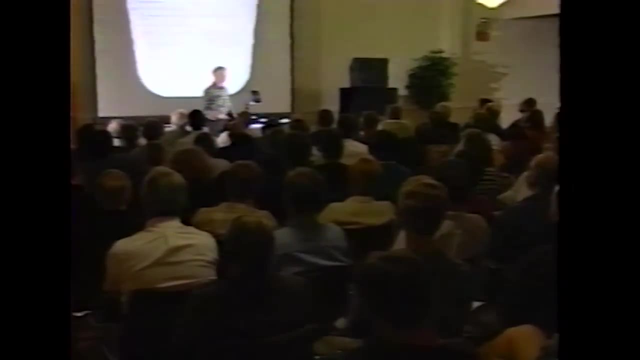 Whichever way you want to look at it, But it kind of this is what he would like to use, And we had to sort of explain to him that our target market didn't want to find the fourth occurrence of Lisa in the third paragraph. 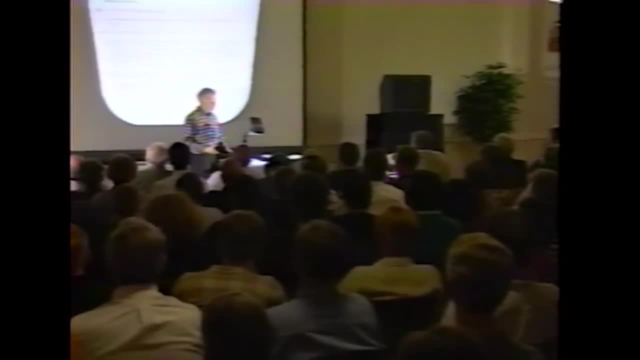 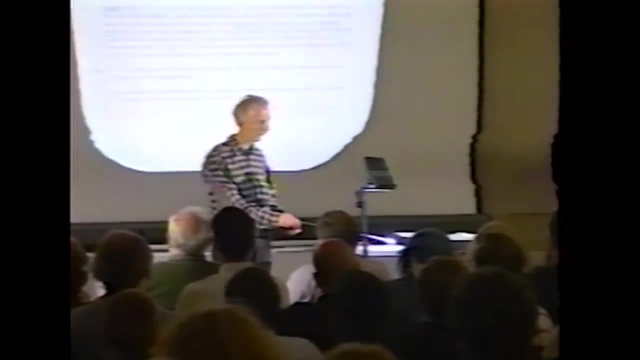 They could see it with the mouse, and that was just fine. Now here was something I wish we'd listened to At this point. it said that you were growing windows from the lower right. Now I showed you something before showing that you grew it. 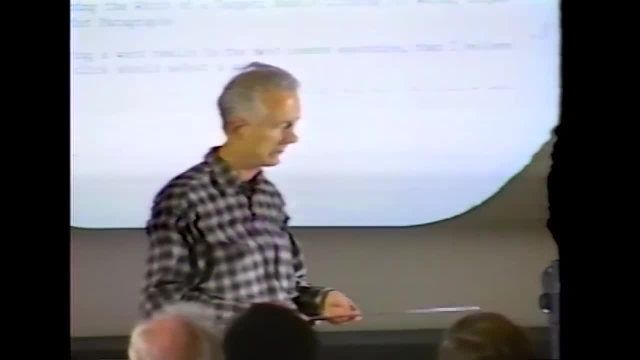 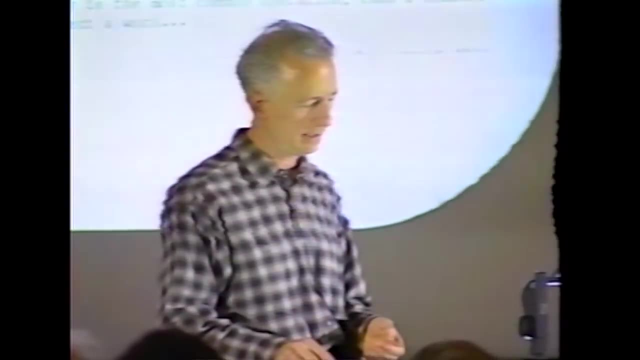 at the top. I think in this document it was sort of ambiguous whether you grew it from the top or the lower right, And he didn't like that idea. He wanted to be able to grow from any side, And I do think. 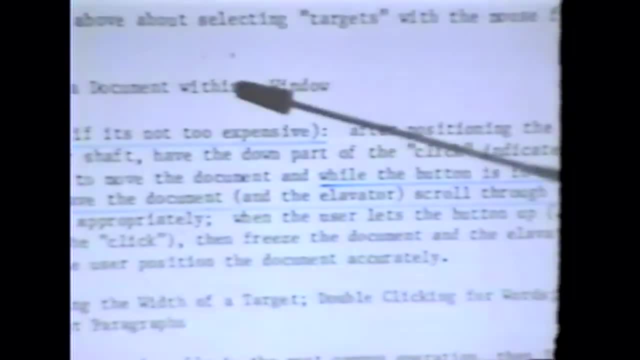 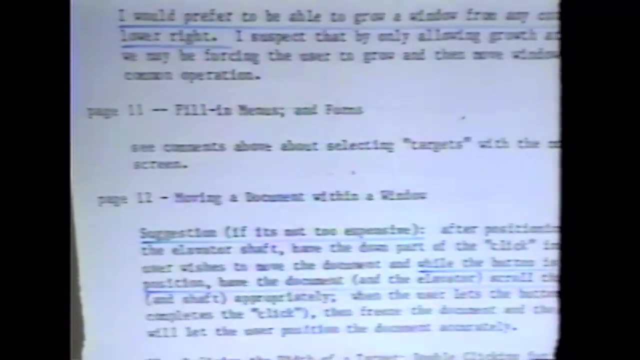 that's better, And we didn't pay any attention to him. I think we were worried about the screen space being too tight for him Moving a document within a window. he wanted to know whether we could do what we now call live scrolling. 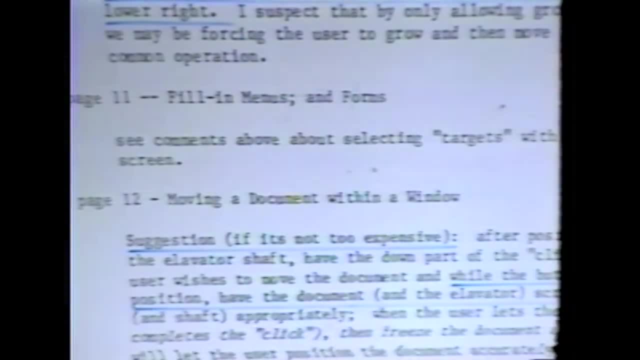 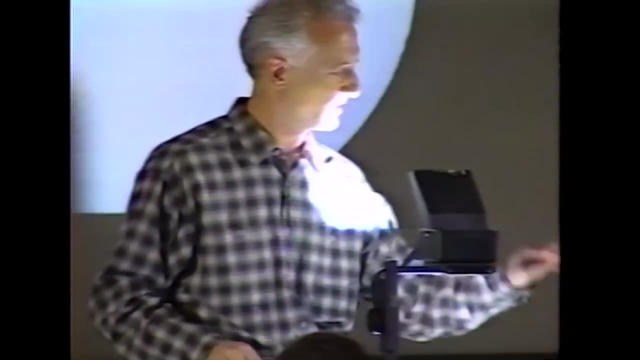 As you move that elevator up and down the shaft. he wanted the text to move continuously. The problem was that the Lisa processor ran at what a quarter Five megahertz, Five megahertz. It didn't even seem that fast to me. 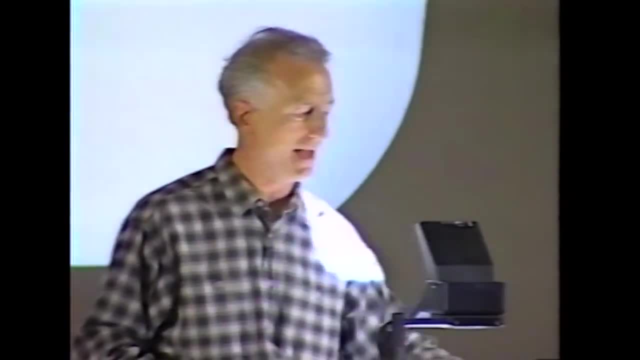 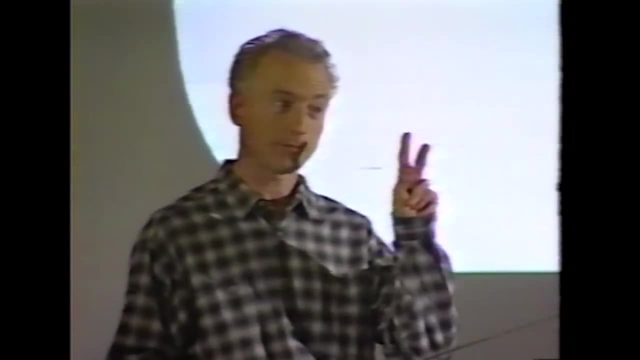 Couldn't do it, So some things were just pragmatic. He didn't like the idea of cut and paste. He wanted us to use, move, copy and delete and transpose. Excuse me, I'm just getting over a cold, In other words, 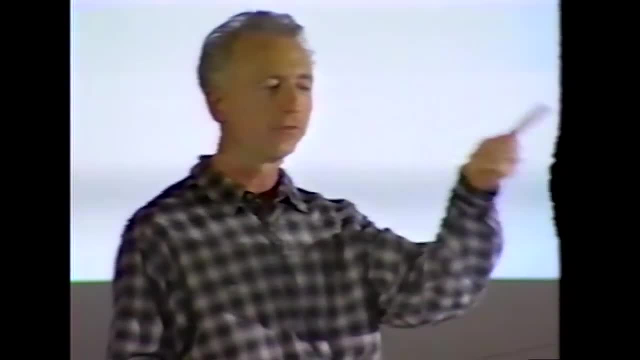 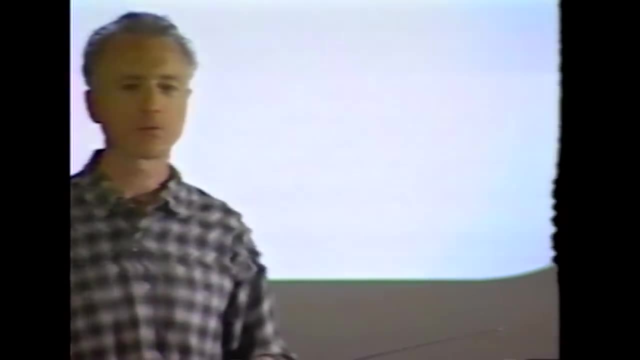 that you'd have two things. you would select, Move this to there, copy this to there, transpose these two things. Well, this wasn't the first time I'd heard that argument And in fact this is one of those religious arguments. 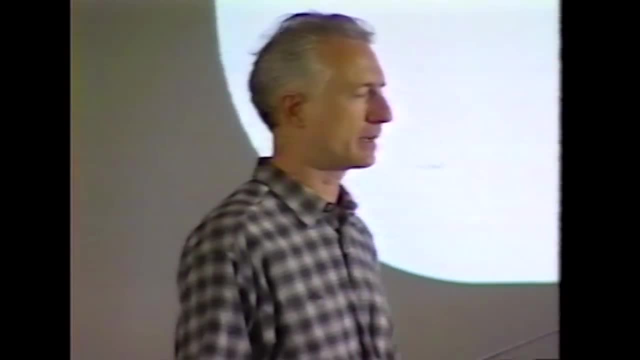 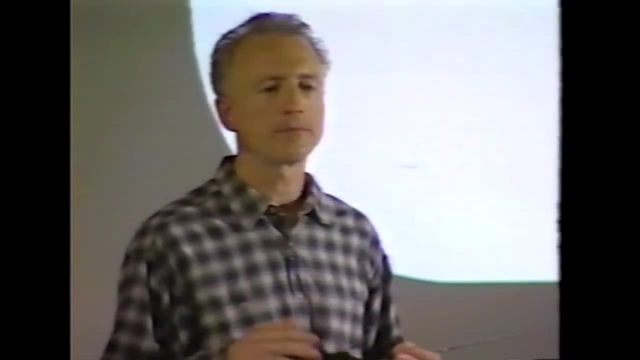 like one button or one versus two buttons. Do you want cut copy paste? Do you want move copy delete The reason we went for? well, you can argue either one. It is two steps to do cut and paste. 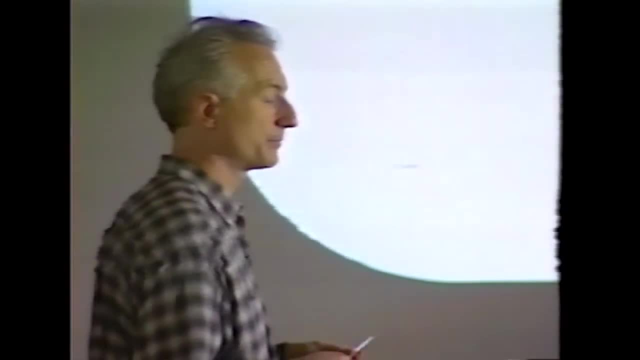 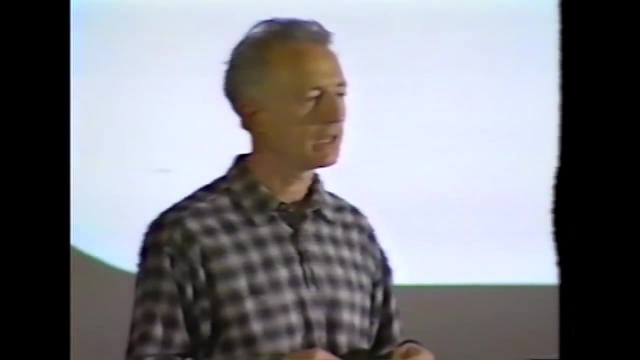 But the reason we went for. there are a lot of advantages to it. One is that move and delete sort of start with the same thing. Some people think that's good, some bad. Another reason is that you don't have to be able to see. 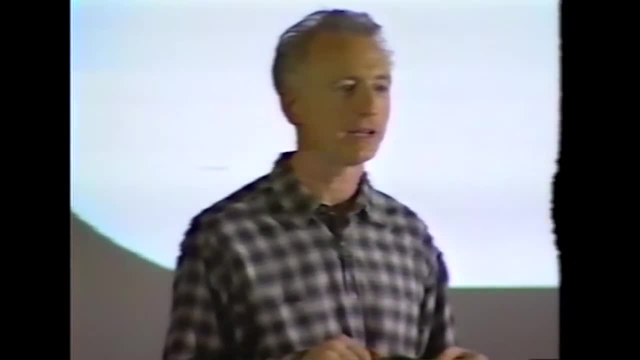 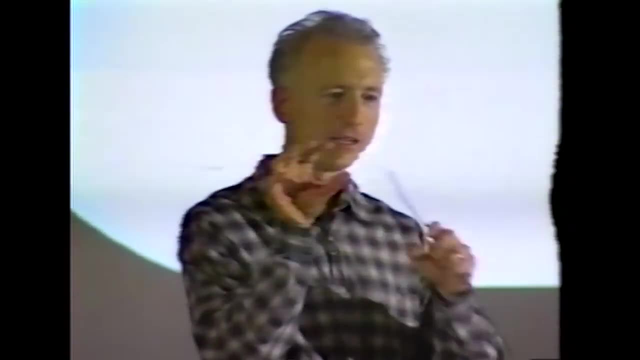 the destination when you are copying or cutting the source. That's the most important thing. And on a screen of limited size, when you have windows overlapping, it's sometimes very hard to get things all lined up. So you can specify two targets. 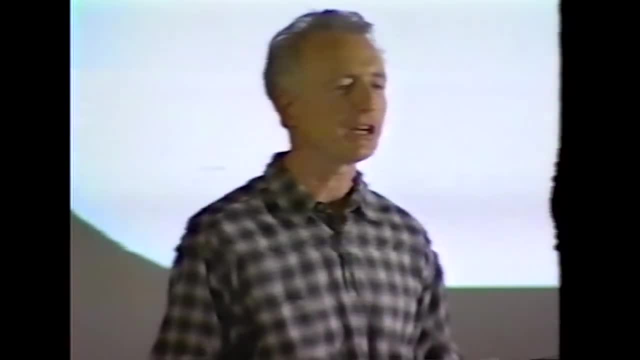 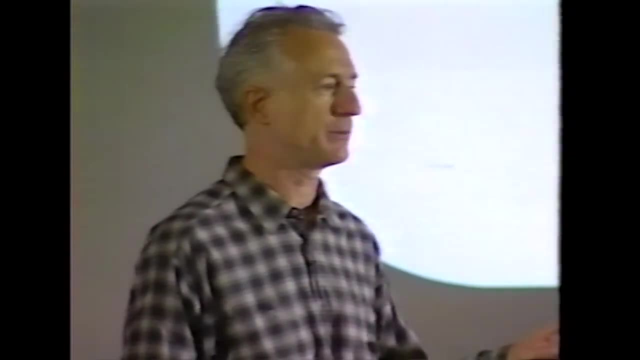 or you have windows popping up and down and you get very confused. The other thing is that I had a secret agenda, which is I thought it would be used not for what they talked about: office systems. I thought, well, that was good. 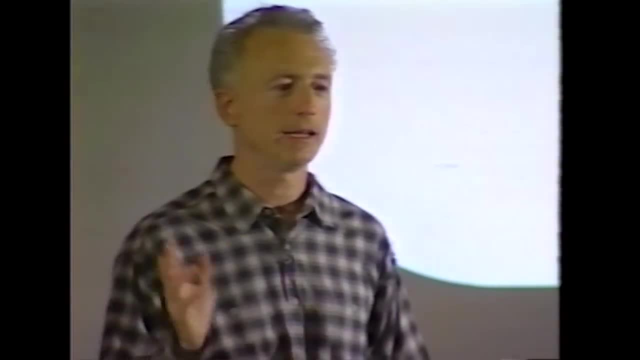 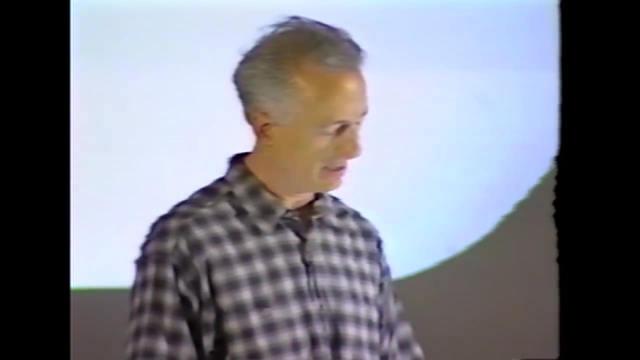 But I didn't want to be used just for that. I thought it would be a great machine for publishing and that we would be able to do cut and paste and do page layout, which was my own personal interest, And so I was advocating. 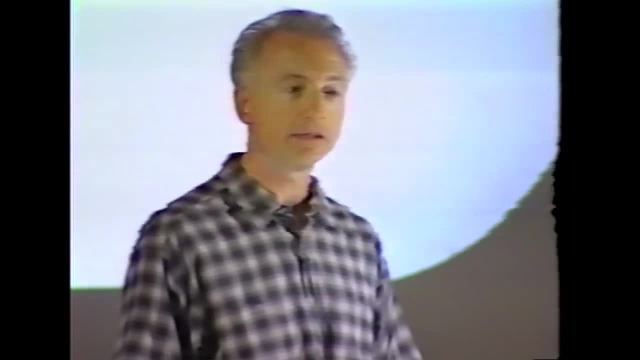 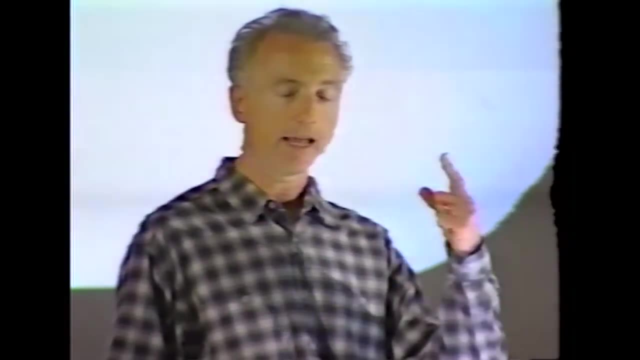 that because that was definitely the way you'd want to do page makeup. But we did user testing and the users slightly preferred the cut and paste model. The wastebasket window was able to not only have one thing you cut out, but multiple things. 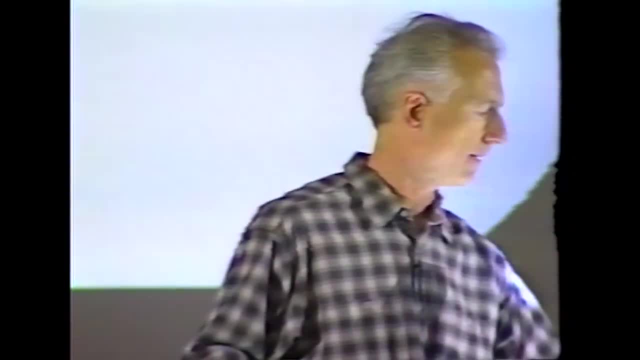 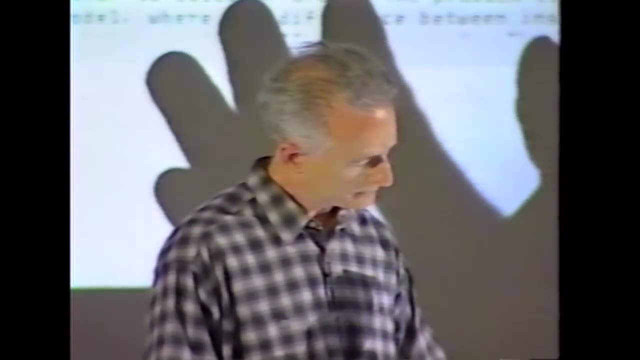 you cut out. We talked about how to deal with the multiple items. Some of us thought it should only hold one. He thought it was okay to have multiple ones and he lost in the end. Okay, here are some comments from me. I was complaining. 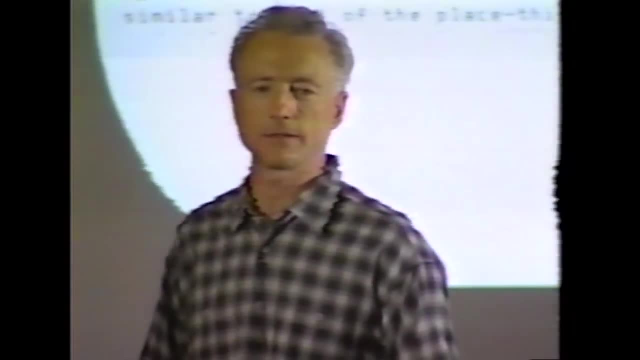 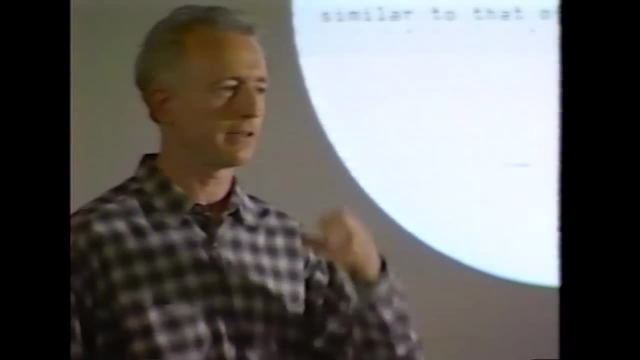 because nowhere in the spec did it say what the response time should be. It said all about the user, what they do with it, but it never said that this needs to respond within half a second. this needs to respond within two seconds. that needs to respond. 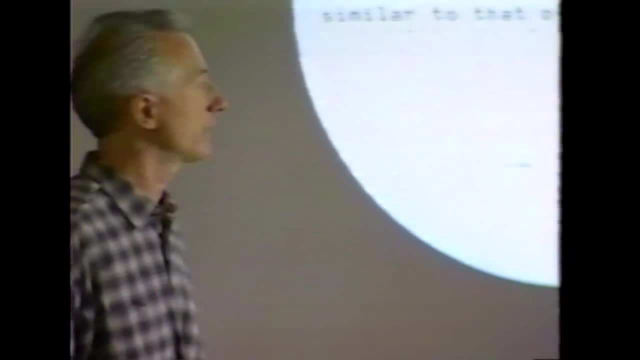 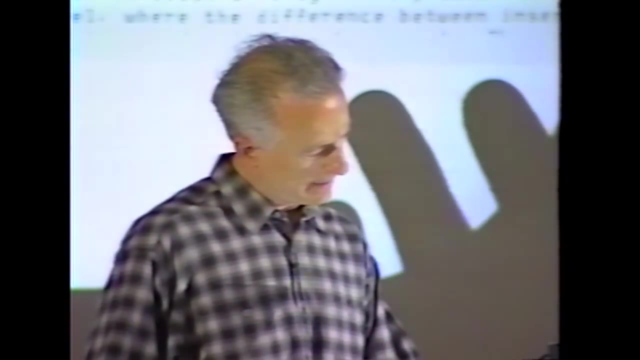 within ten seconds. Never said it anywhere and I was worried if it didn't say it the engineers wouldn't do it. If you ever used Elisa, well, it was really slow. I lost that argument. They said it'll be as fast as we can make it. 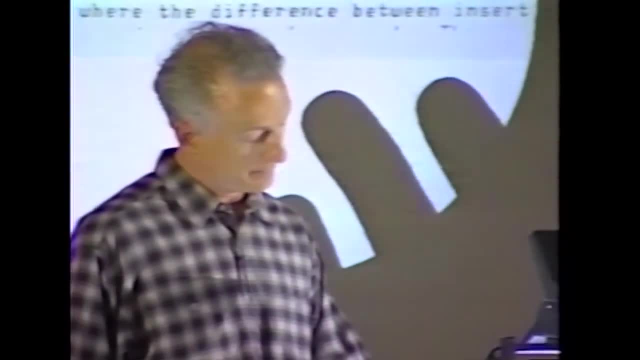 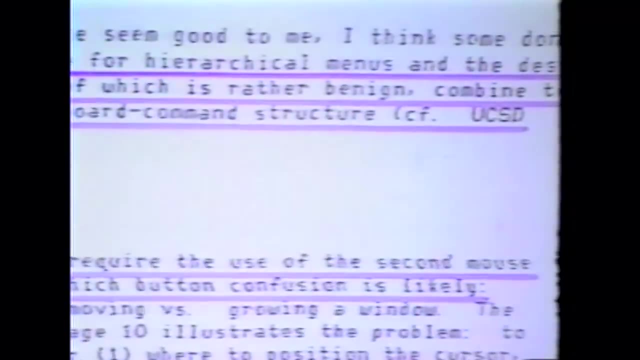 and that was too slow. And then it talked about a really interesting question, which was: well, we want hierarchical menus and we want keyboard accessible commands, so we seem to be fixated on the way they do it in UCSD Pascal. You type a key. 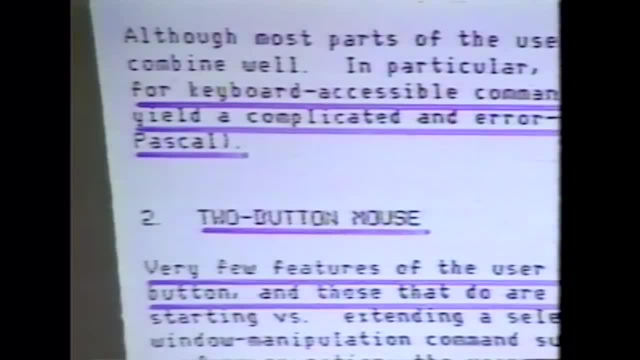 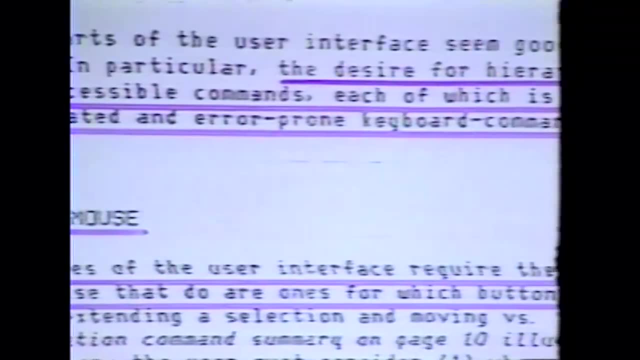 get another menu, type a key, get another menu. and that just bothered me and I thought there's a lot of mistakes going to be made and people are going to forget which level of the hierarchy they're in, how they get back out of it again. 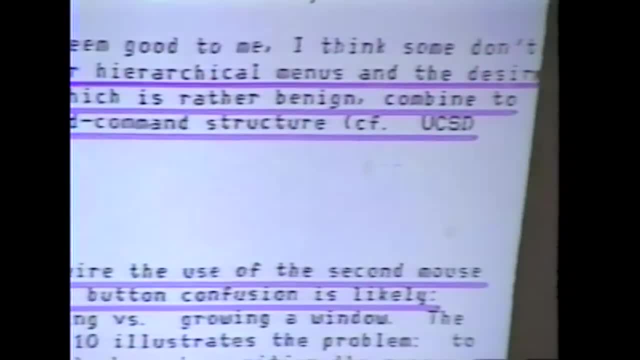 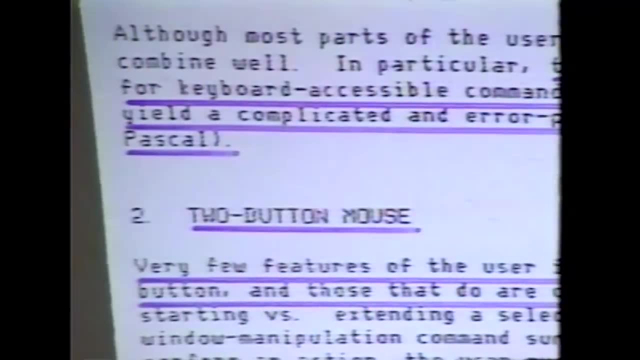 It's just going to be too complicated and I didn't like it, So we'll come to how that was solved later. The other thing I was complaining about was the two-button mouse. We didn't use the second button for much else, for a lot of different things. 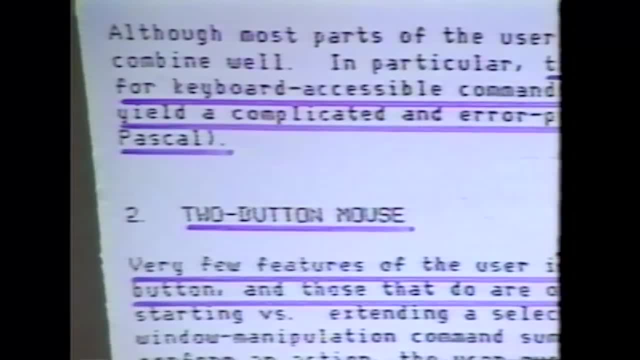 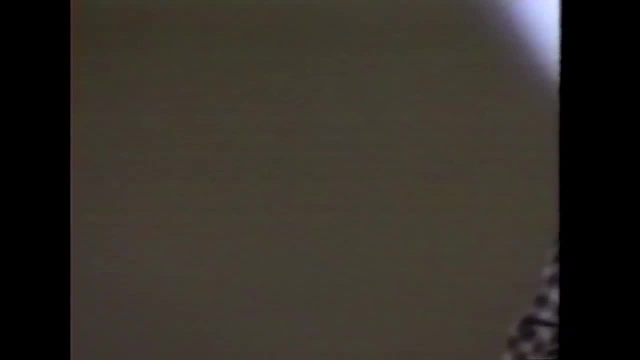 We didn't use it for much, and when we did, there was no way to remember which button did what, and so I just wanted to eject the second button and just have one, And that's August 13th. Operations on windows I proposed here. 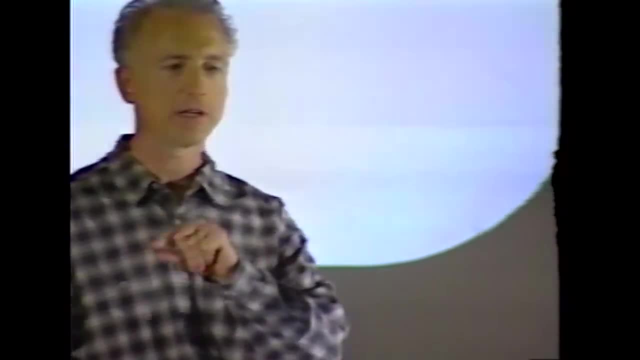 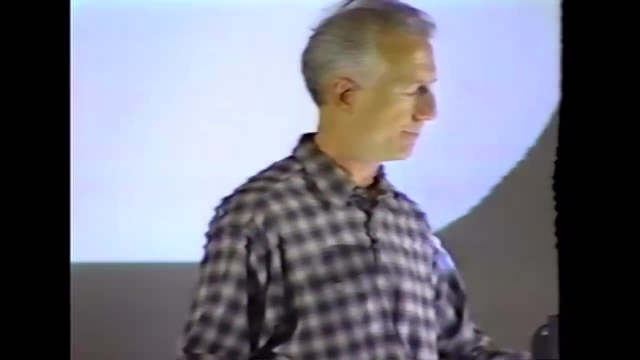 that we have this box in the lower right-hand corner that we use for growing the window instead of doing it from the top, And also I thought there ought to be a way to split a window into panes, And then I had a whole section. 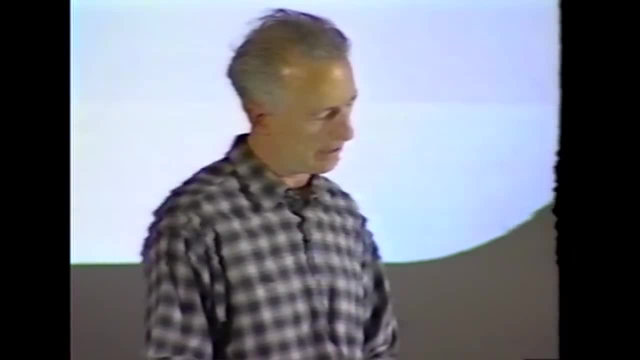 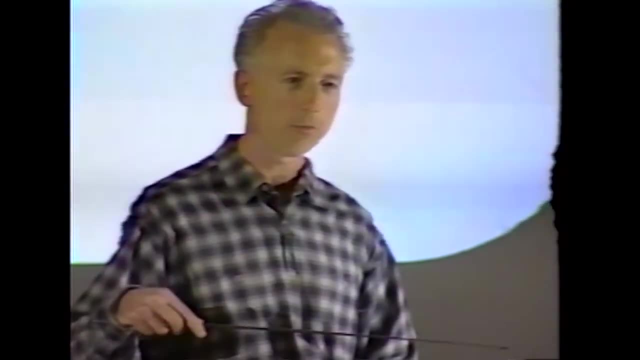 here about moving a document within a window. I go and talk about scrolling and why I don't like the way it is, And then I said: why don't we put you know, one arrow at the top of the scroll bar, one at the bottom? 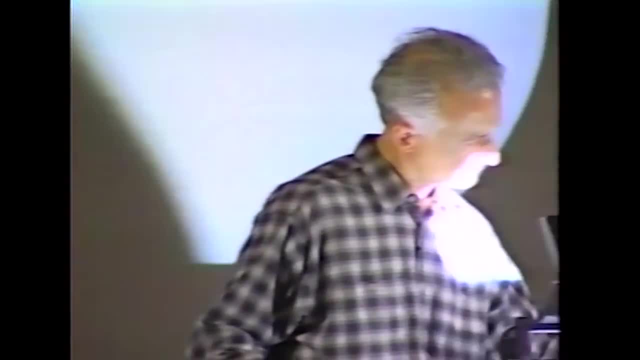 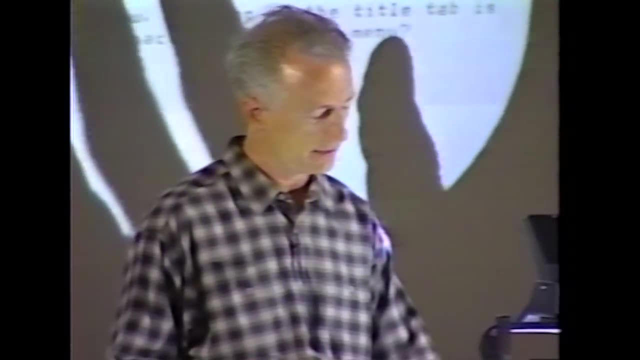 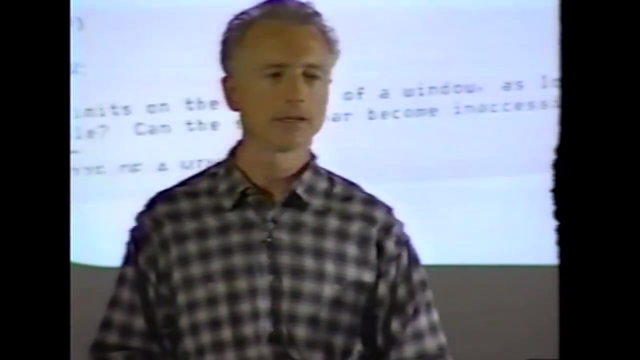 of the scroll bar And I actually prototyped it. Those of you who know the Xerox Star know that the Xerox Star had that feature. Those of us who were from Xerox were under a confidentiality agreement that we weren't allowed to tell the other Apple people. 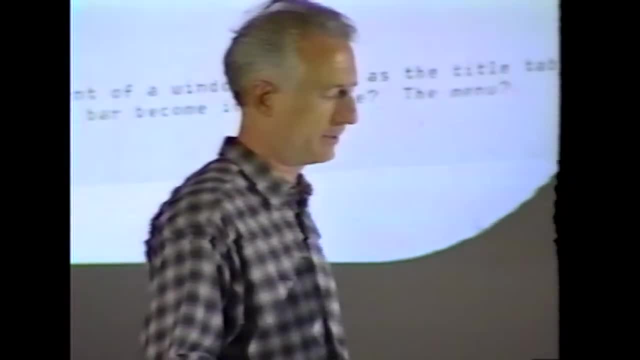 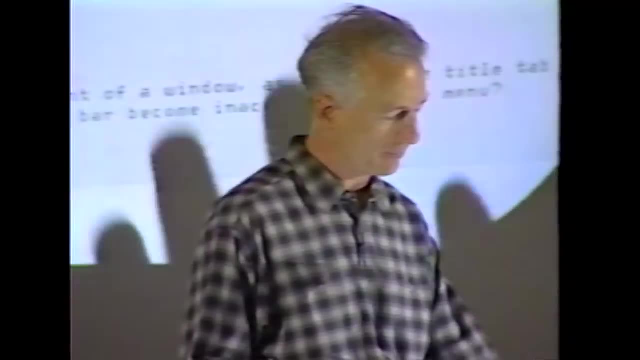 about the Star, And so, as you go through this, you'll sometimes find that things seem like- isn't it an obvious solution? You could have got it from the Star, but none of us were able to say how the Star was. 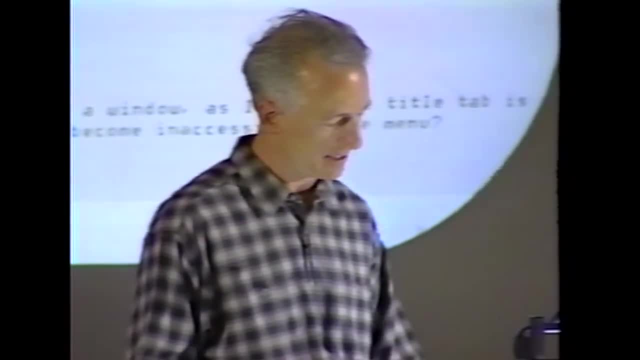 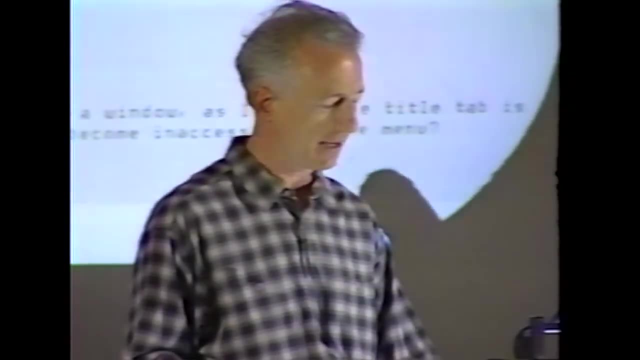 We were only allowed to comment on other people's proposals and make new ones, And it was an interesting kind of dynamic. But gradually over time a few Star-like things crept in, but not many until the Star actually shipped or was announced. 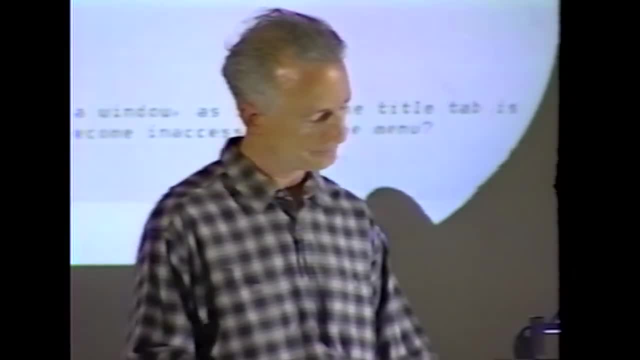 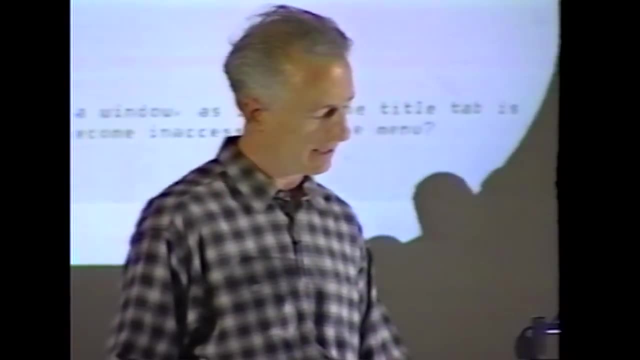 in June of 81.. But here we are in 1980.. Then I suggested we try an eye-shaped cursor for text selection instead of an arrow, And that actually is something I had done In my early years at Xerox in a particular word processor. 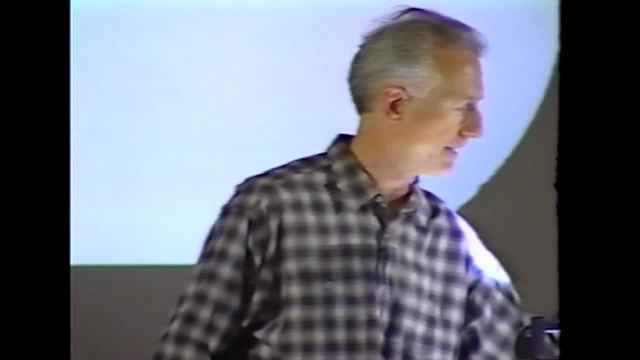 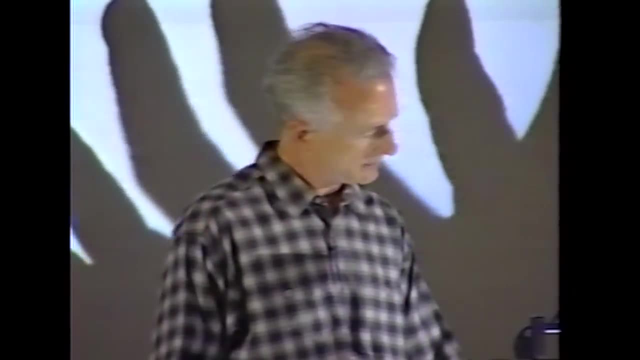 I'd done. I also said I wish the cursor would be bigger than 16 by 16, to go to 32 by 32, which we eventually did. Menus. this was what August 18th. I think we should experiment. 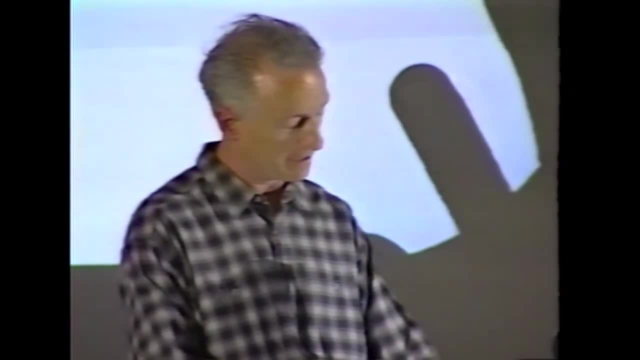 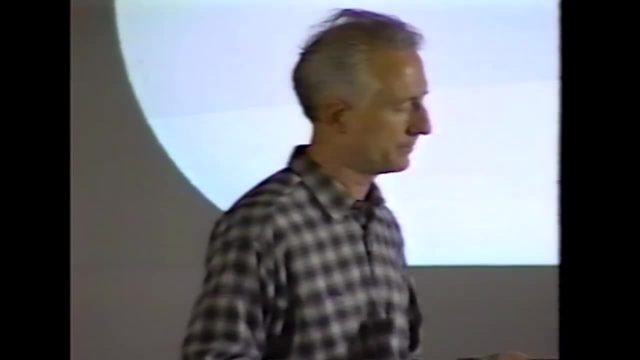 with menus at the top or right of the window or even totally detached at the top of the screen, full width. So up to this time we were doing sort of the way Windows does and every window had its own menu. And I was thinking: 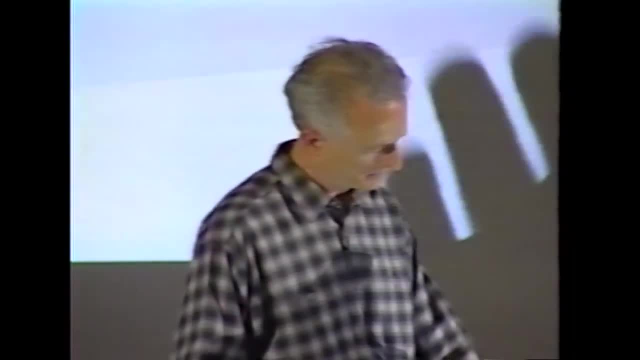 you know, maybe we ought to put it at the top, and you'll see why in a minute when you see the pictures. And then I said hierarchical menus. well, maybe we have to have them. we can't get rid of them. 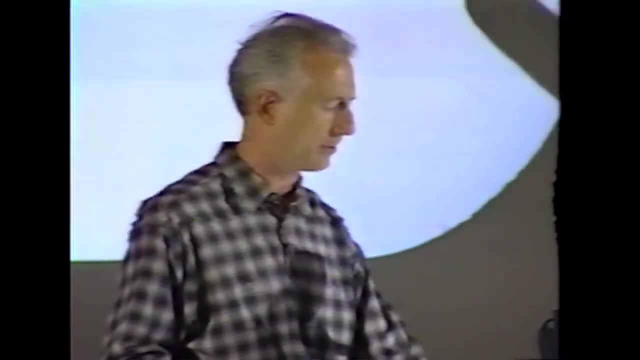 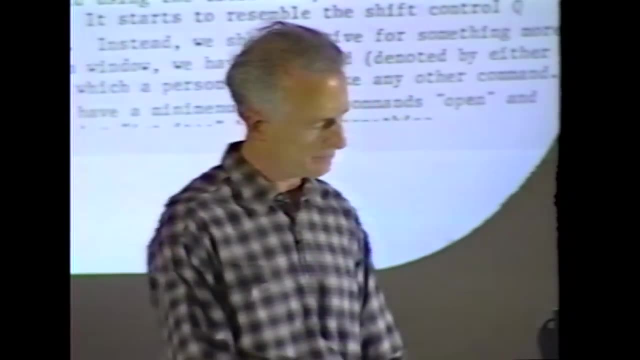 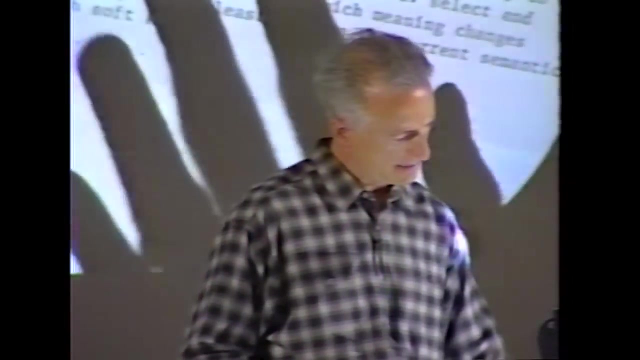 but could we make them mouse accessed instead of having to type all these keystrokes? So these were my two causes of the moment. Barry Smith, who was in product marketing, responded about the same time And he said at this point Bill had moved the menu bar. 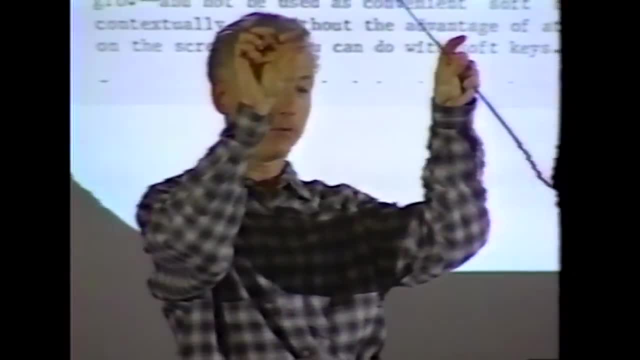 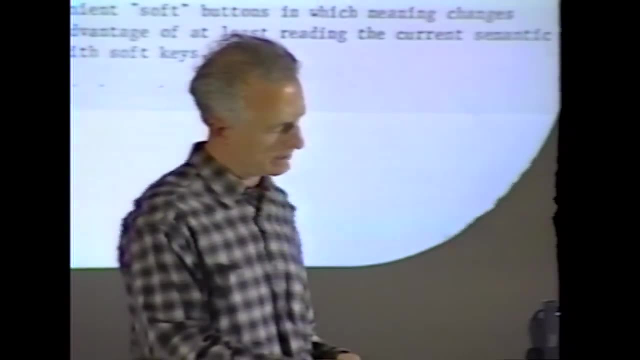 that edit cut copy paste thing from the bottom of the window to the top of the window. That was the change And Barry liked that. He likes them a lot better near the top. He called them near the top And then he wanted to know though. 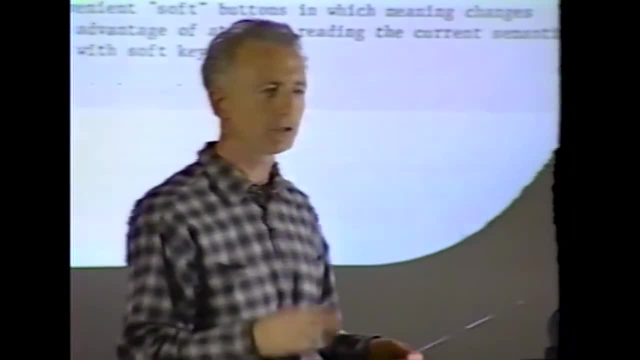 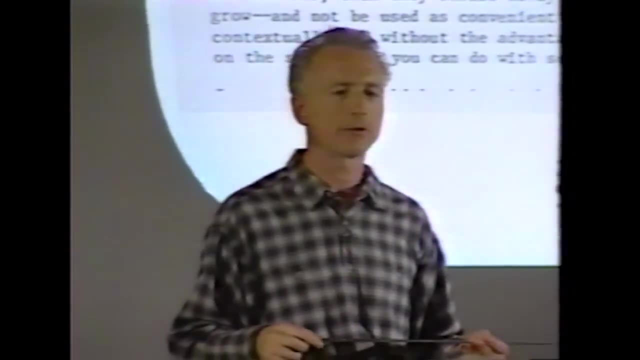 what would happen if there were a lot of menu items and could the menu scroll? And those of you who know the history of the Mac user interface know that at some point- I don't know, 1990 or so- we started adding scrolling. 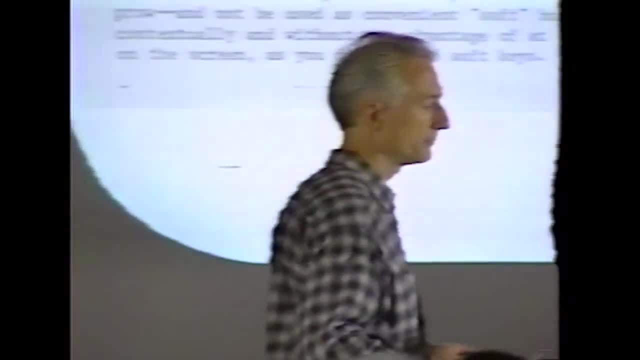 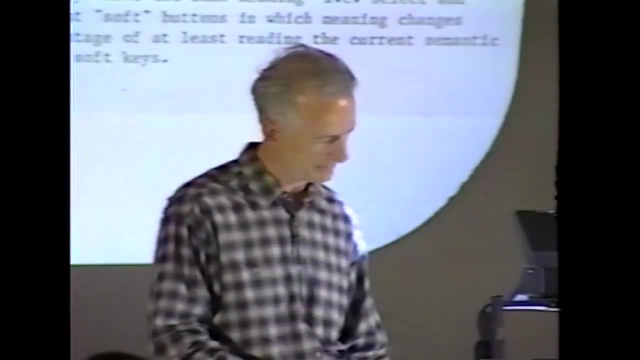 to Mac menus, But we didn't have them in the early Mac until Lisa And I was against it because that would have encouraged people to have a lot of menu items and I didn't think they should, So I kept that from happening. You can't constrain people, though. 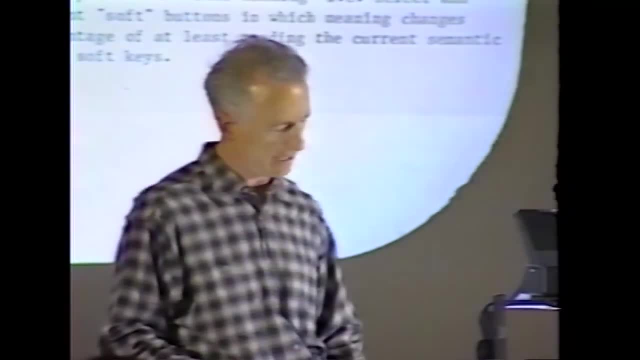 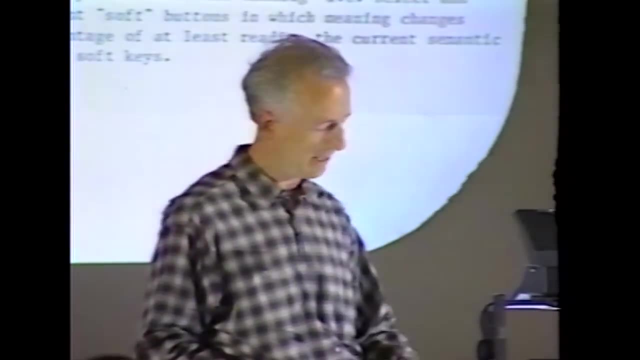 He also did not like the fact that you had to type multiple keystrokes to a hierarchical menu, And so he was thinking maybe we could get to something where it was a single keystroke to invoke a command, no matter where it was in the hierarchy. 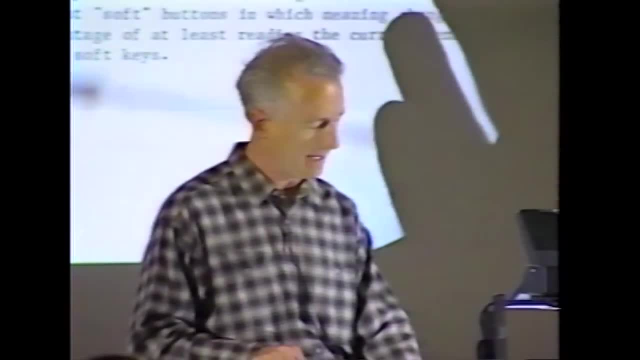 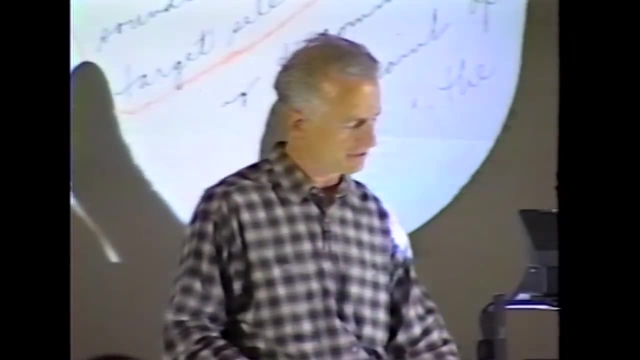 And I think Bill was experimenting with that at that time And he also didn't like the two-button mouse. He thought it was cool, He thought it was confusing. So August 18th- I guess that was August 13th before us. 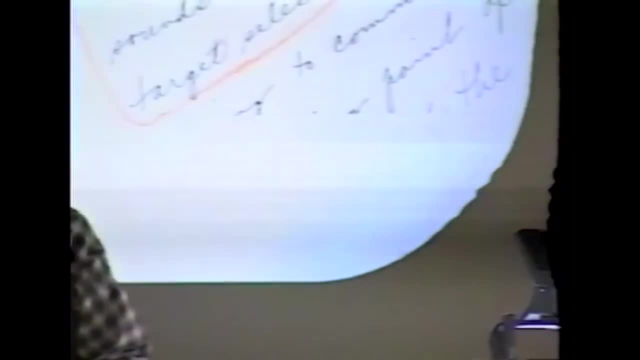 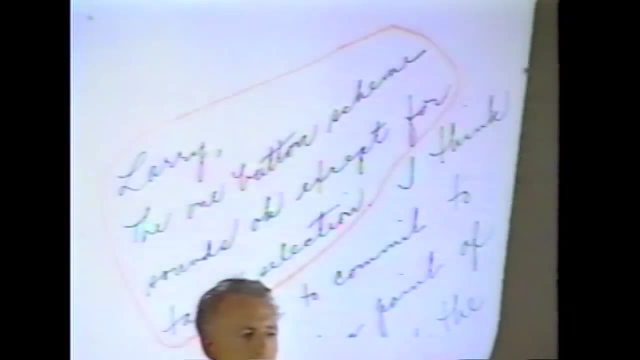 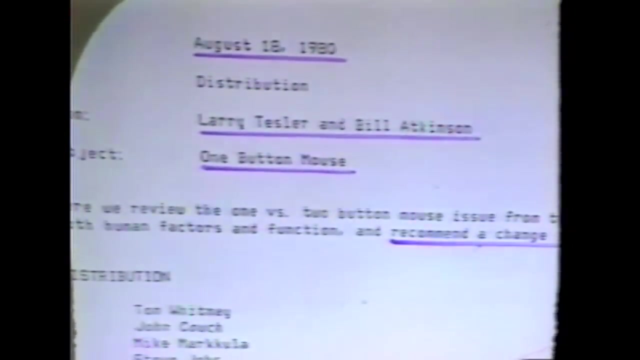 a few days later, after intense political polite discussions- heated sometimes- Bill and I decided: hey, let's get rid of the second button, Let's shake things up- One-button mouse. So we wrote this memo together so that people knew we were real serious. 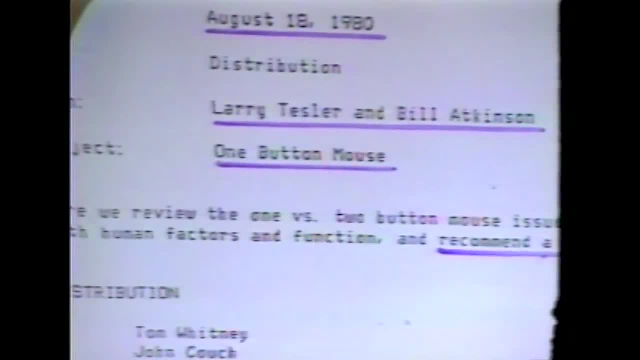 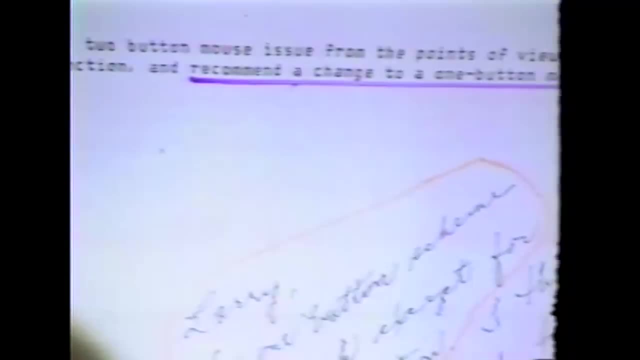 Sent it to the usual suspects And we say: we recommend a change to the one-button mouse And whoever wrote this comment, and I'm glad I don't know who. it was said: well, maybe not sure that's a good idea. 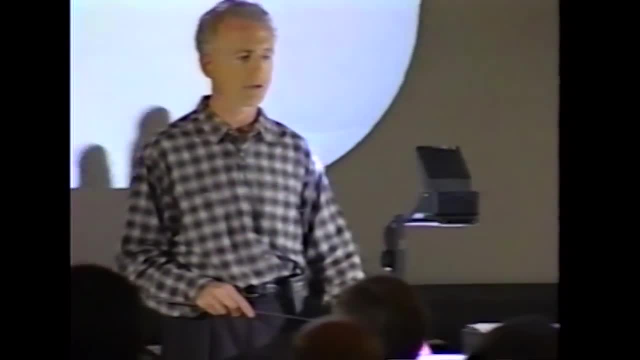 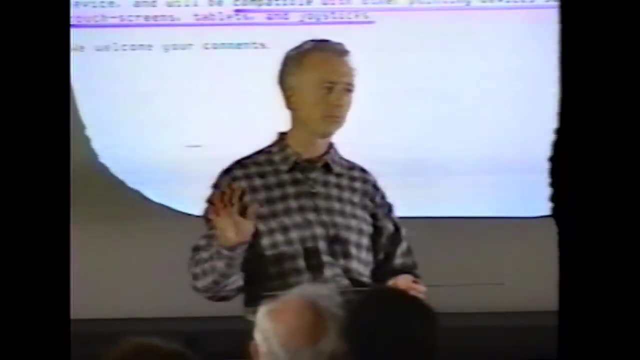 But it turned out Trip Hawkins, who later went on to found Electronic Arts and 3DO, was the product marketing manager. He loved it. He said that's what we got to do. We got to think more kind of consumer-oriented. 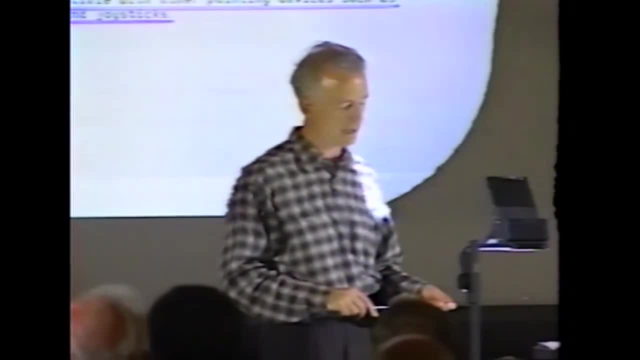 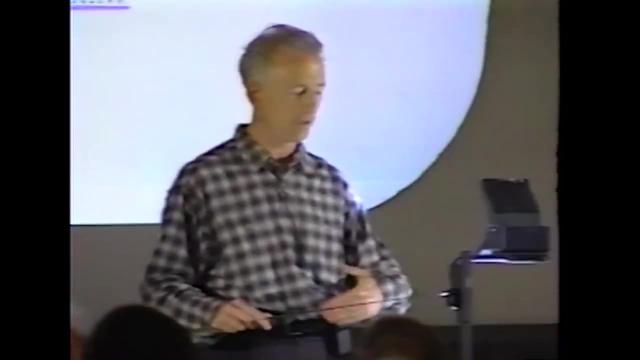 really simple, get rid of all this computer science concepts and give people something real simple. He liked the one-button, So after that we had a period, sort of goodwill, where we were able to do user interface design without a lot of complaining, which ended after a while. 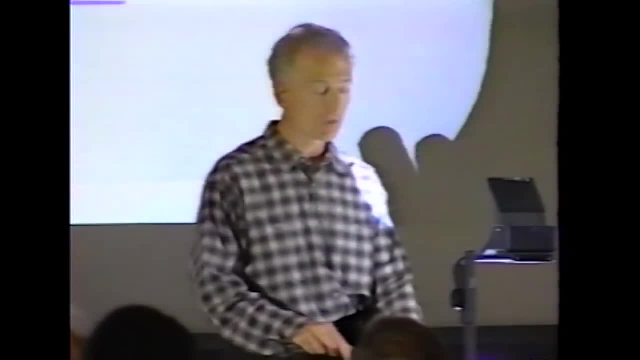 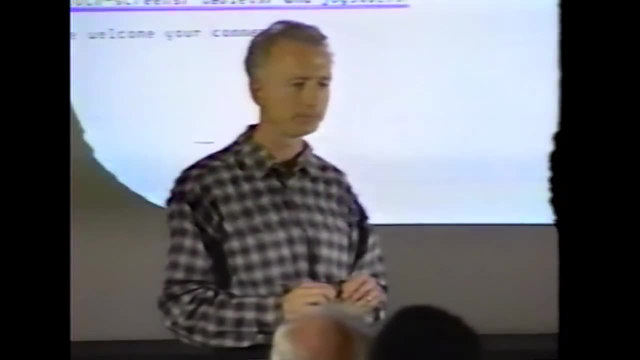 as you'll see. Well, if you only have one button, some things are hard to do. You can drag a short selection, but what if you want to select something three pages long? It's a long time to drag from one end to the other. 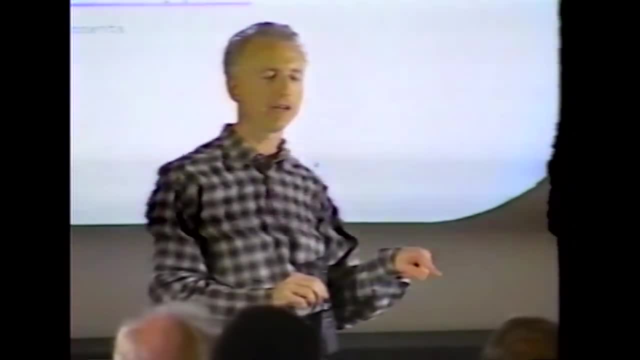 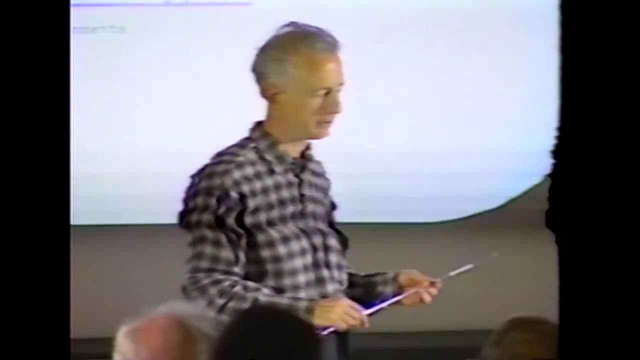 So we thought, okay, well, we'll use a shift key on the keyboard, Since this doesn't happen very often. you'll click the beginning of the selection, you'll scroll to where you want to go, hold down the shift key and click the end. 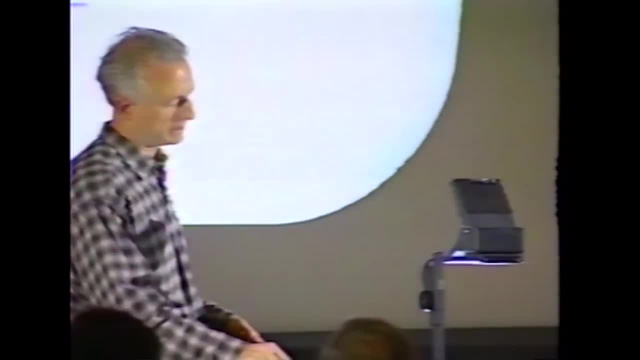 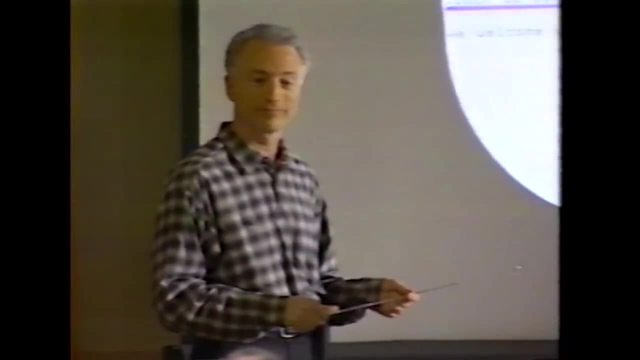 of the selection. So that's where we got the shift button thing adjusting selection. And then we said the one-button mouse is superior. Look at the reasons: Superior, human factors. You don't have to think of a name for each button. 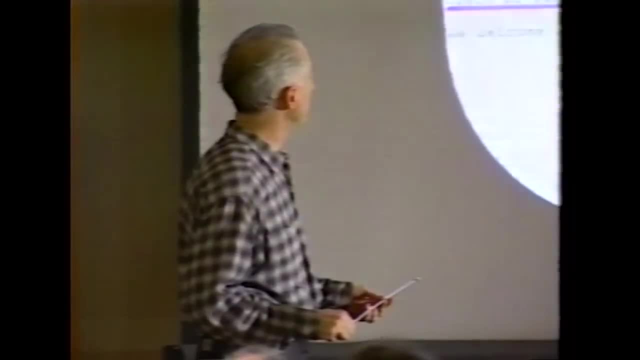 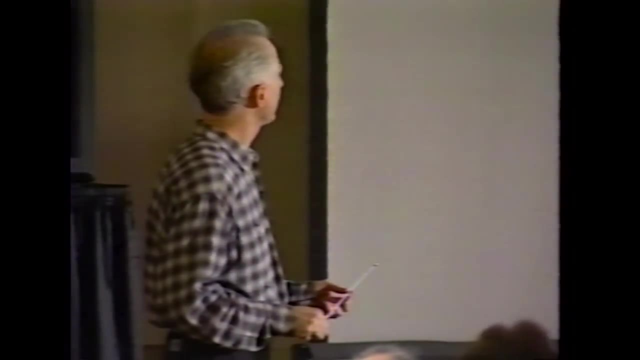 That's important when you're trying to ship product in six months. The mouse will be cheaper to make because one less button- I mean just think of what the cost of that little switch is. It'll be- and something more profound someday when we start. 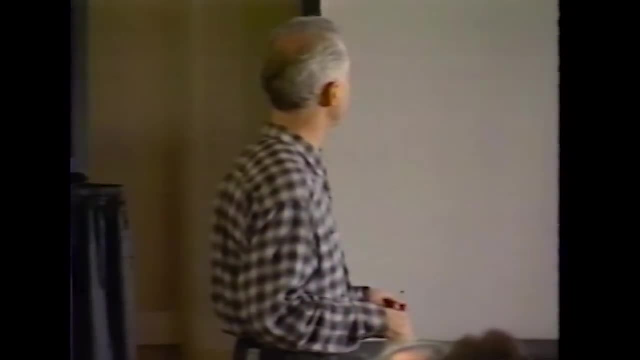 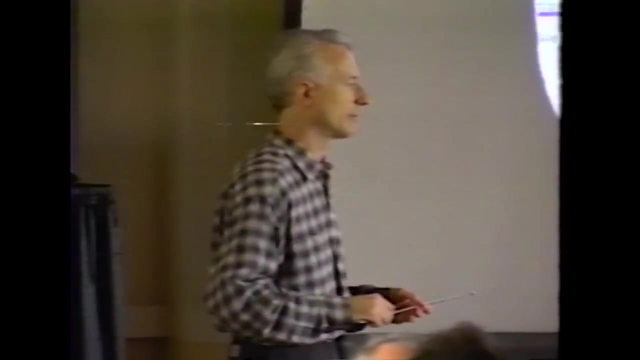 having other things in mice on our computers, like joysticks for games, tablets, touch screens. we'll be glad we only had one button, because that one finger or whatever, or pen that the user is using is the button, And that turned out to be sort of prophetic. 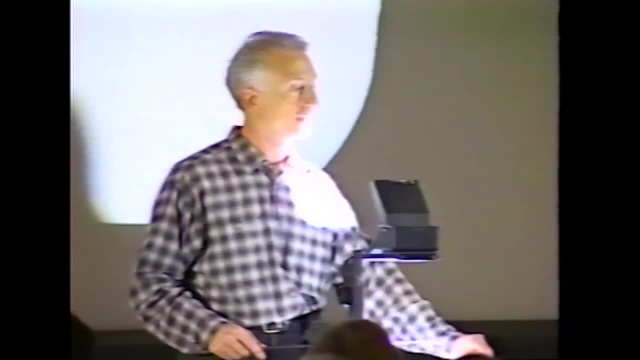 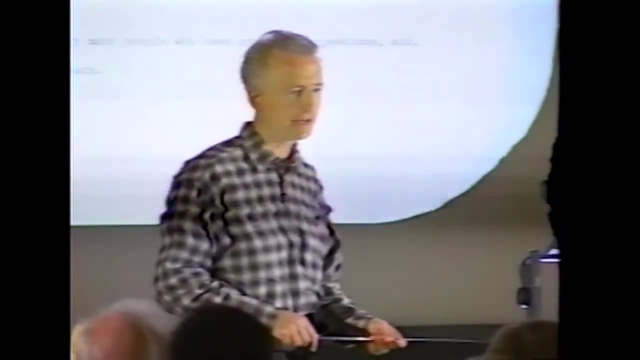 although very few such pointing devices take advantage of that. in fact, They usually have buttons anyway. Okay, so August 22nd is a revised version of the, the user interface, And it says this: is it now? We're done. 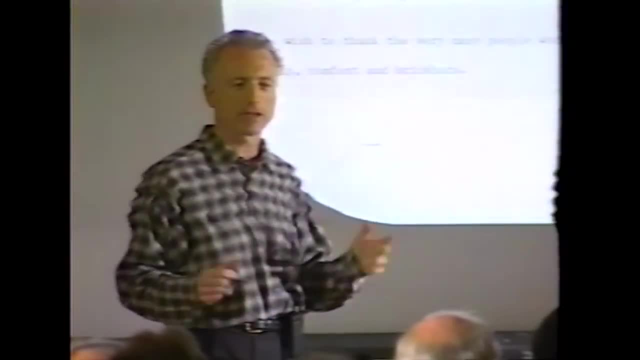 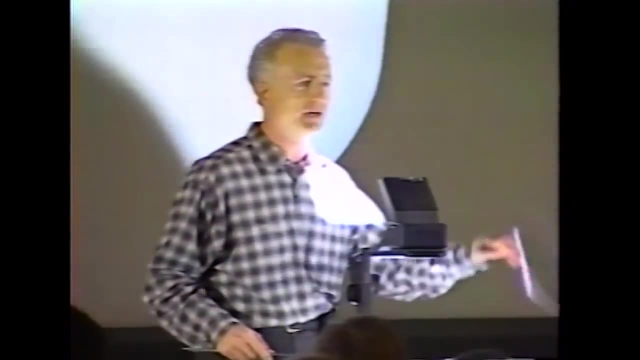 So now, instead of a week, you only have three days to return comments, because we must be done. There couldn't be more than one or two comments. They're probably just typos or something. By this point, we were working on this interface. 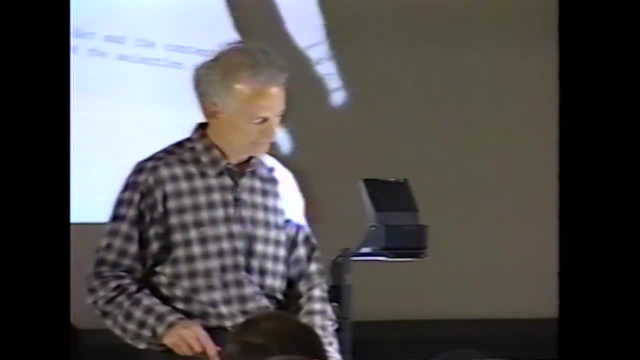 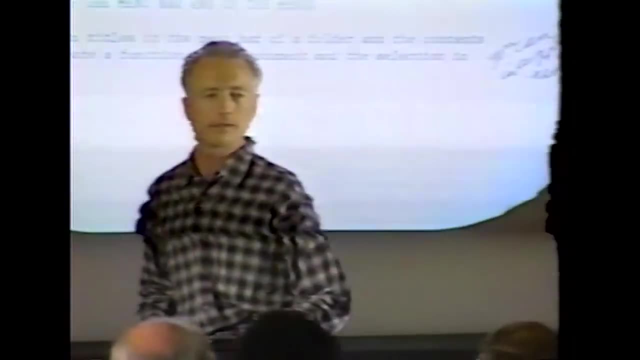 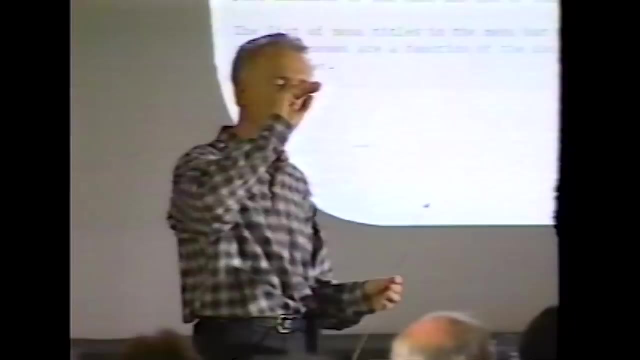 for a month already. Okay, so what did it have in this version? It had a concept called dim highlighting. This was introduced for the first time that I know of here, that if you have some of the menu items, instead of eliminating menu items. 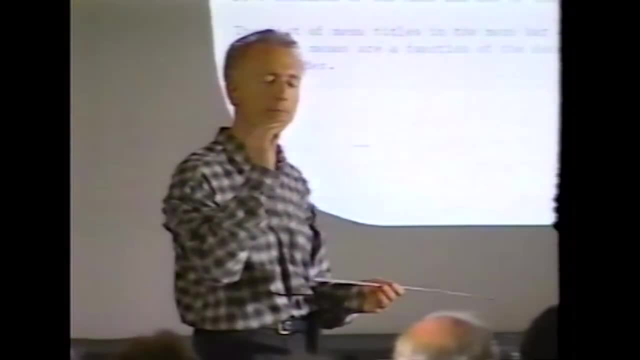 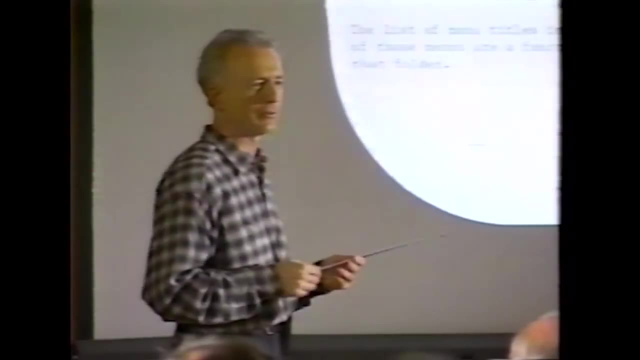 that weren't relevant, which we would dim them, we would gray them out. Instead of being black type, they'd be kind of in gray type, And then we said they can be evoked anyway if the user wishes, although they wouldn't. 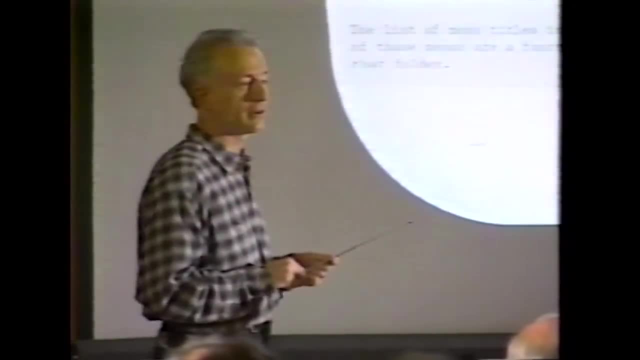 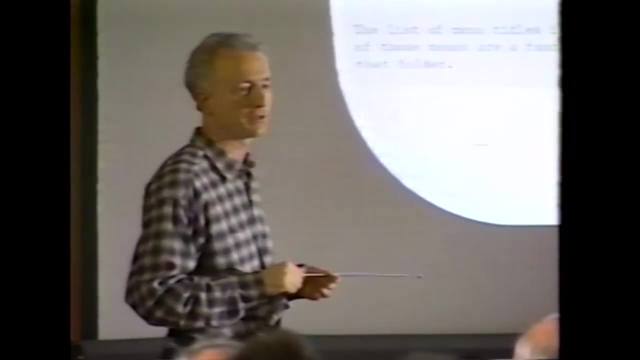 do anything. And and we also were going to use dim highlighting for another purpose, which was to show toggles, And, as you know, that was later changed to have check marks instead of just using this for two purposes, because that was very confusing. 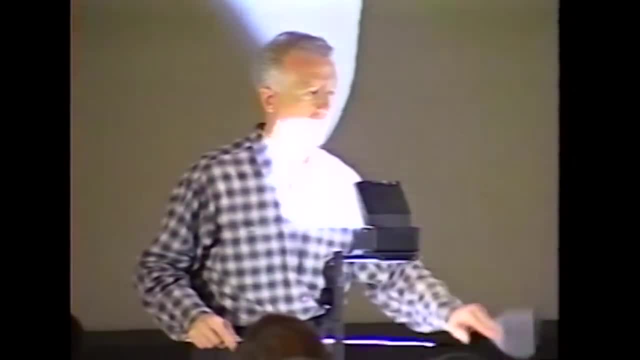 But at that point we had to get away with one mechanism for both things, And it was Occam's Razor. If one mechanism will do, they don't have two. Well, it turned out that one didn't do, so we had to apologize. 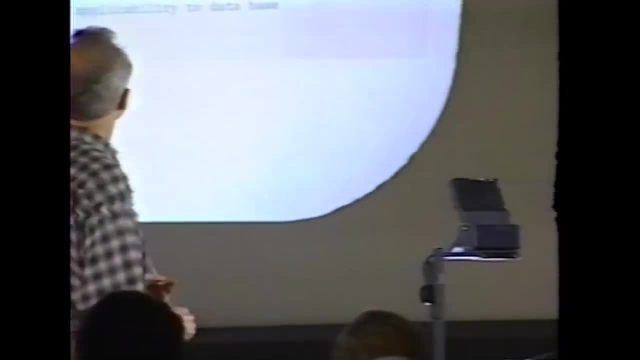 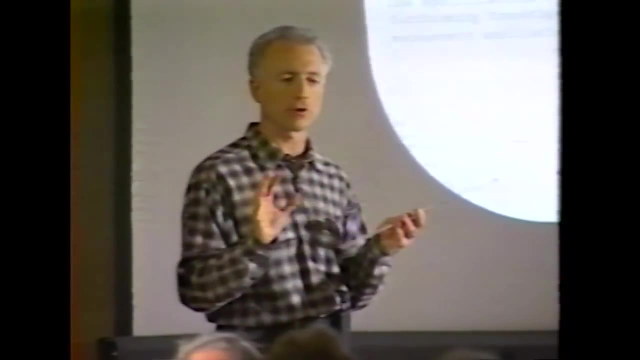 to Occam. Now, as you know, you can do command keys on the Mac, or at least a keyboard, and you can invoke commands from the keyboard, And we knew it was important to reserve some for the most common commands because it might be okay. 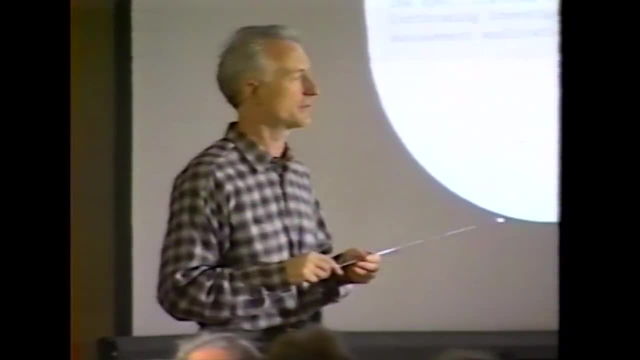 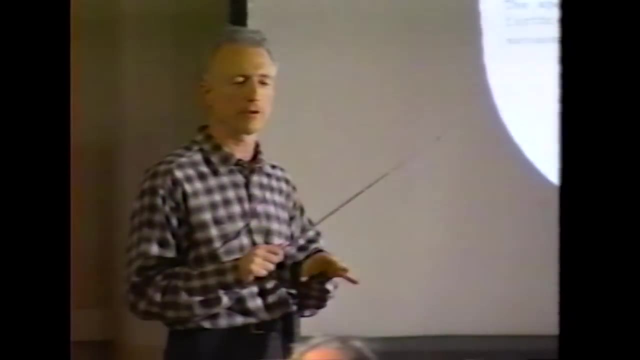 for an application to use, you know, Command Shift J for something. But we wanted to be sure cut, copy, paste, undo were the same for everybody: bold, italic, underline and normal. We thought these would be used the most. 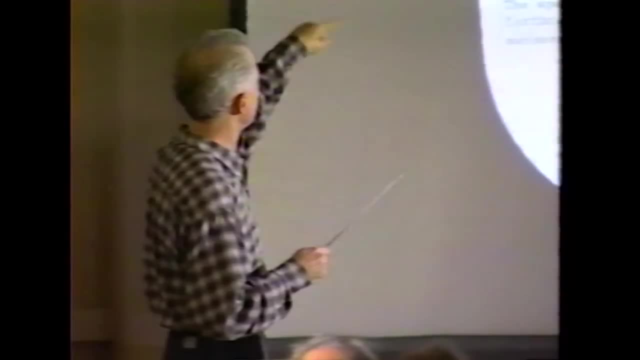 And so the whole sequence. I'm not going to go through them all today, but we had various theories And, as you see here, it's rather different from what we ended up with. ZXCV was sort of the order on the keyboard. 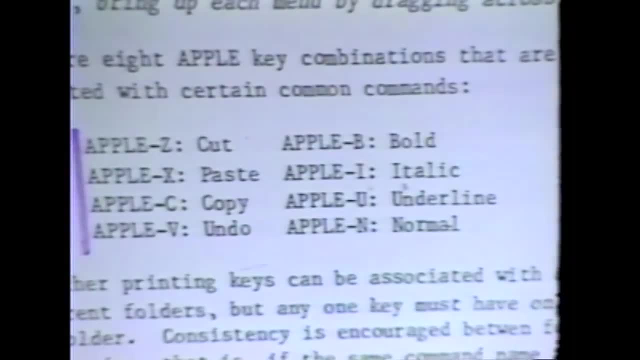 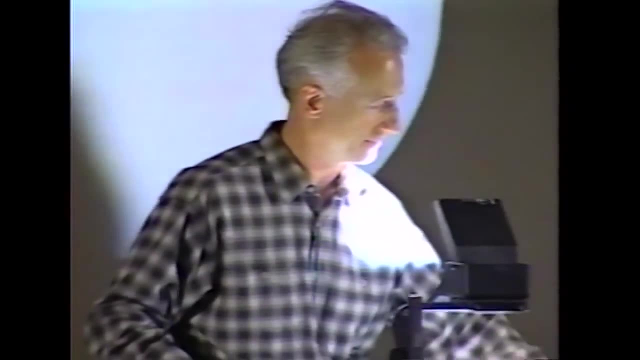 Cut paste, copy undo was the order in the menu, so that was it. Over time we refined this. This led to many very heated arguments. People would rather argue about trivial things like this than important things, But we did have fun arguing. 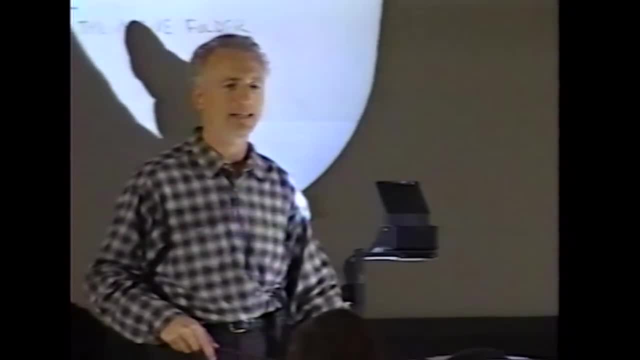 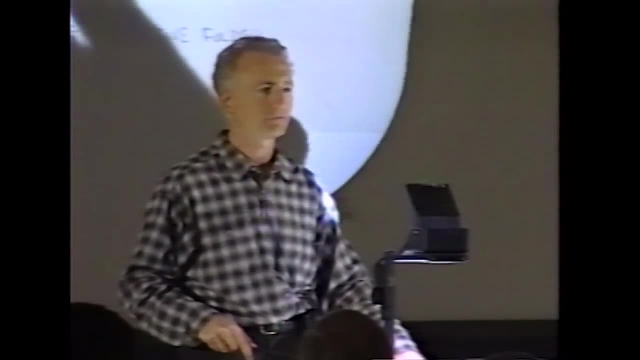 Does anybody remember what they really are Today? Control-I, Control-B, That's right, Control-I, Control-B. And then for cut, Control-X, Control-X. The same as WordStar. WordStar Copy, WordStar. Oh, I didn't know that. 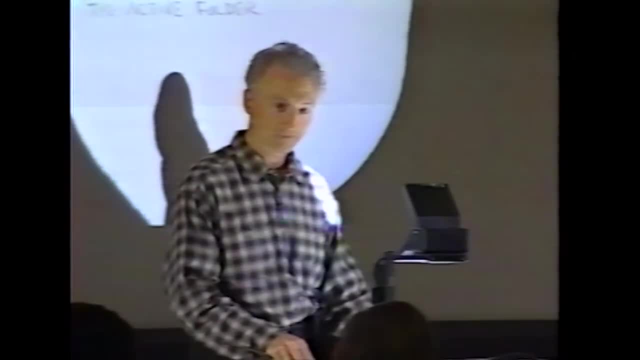 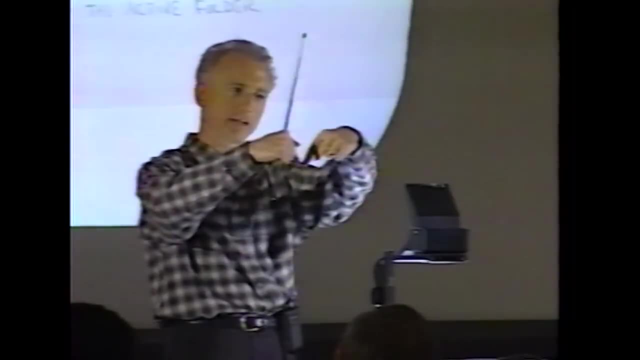 Yeah, Didn't know that. That's part of the problem of most computing is people don't realize. Well, we did X because it was a cross-out And we did V because it pointed down like this and you were inserting like an upside-down carrot. 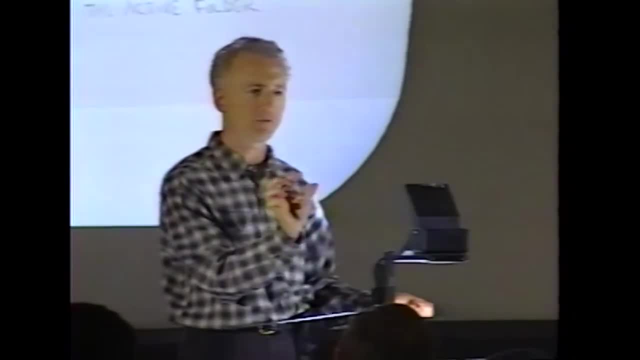 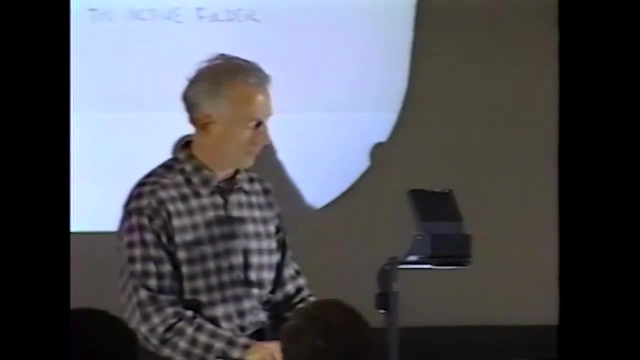 That was paste, And Z was the closest one because we figured you'd undo a lot, And C for copy. That was easy, So that's how we did that. Okay, So this was the anatomy of a window. We had title tab. 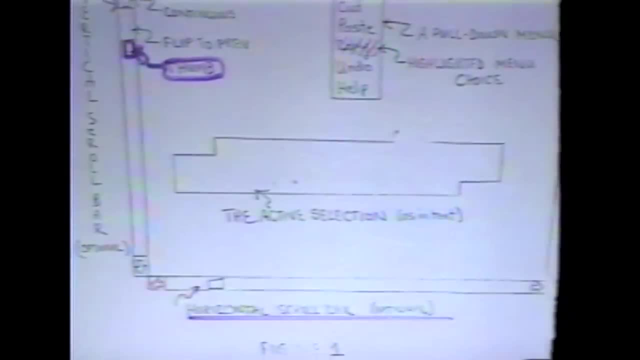 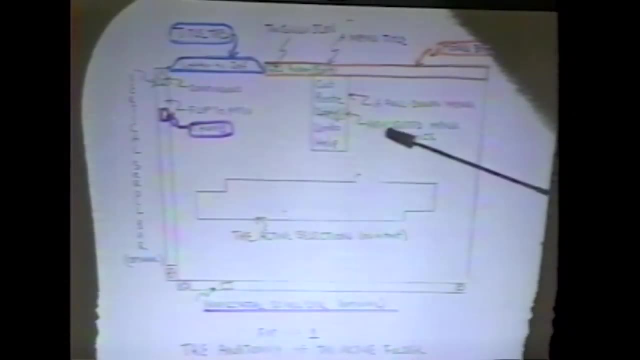 Now notice: next to the title tab we now move the menu to the top, as was commented upon. Someone obviously had got a sneak preview draft in that earlier memo And look, There are menus that are popping down from the menu bar First time. 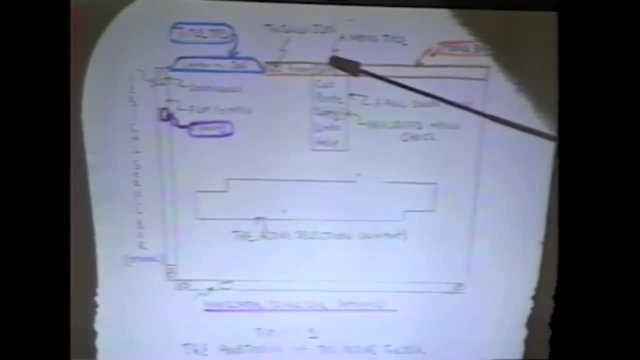 When it was the bottom that didn't make a whole lot of sense. But now that it was the top, Bill Kidd came in here and replaced the previous menu. like it did in UCSD Pascal, He could use the second dimension and have a menu. 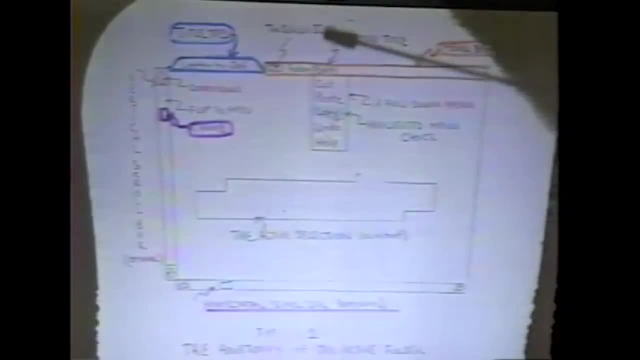 pop out to the bottom. Don't ask us how we were going to do third-level menus, But at this point this was good enough. We had two levels of menus and we were happy. Over here there was the elevator shaft. Now we called it. 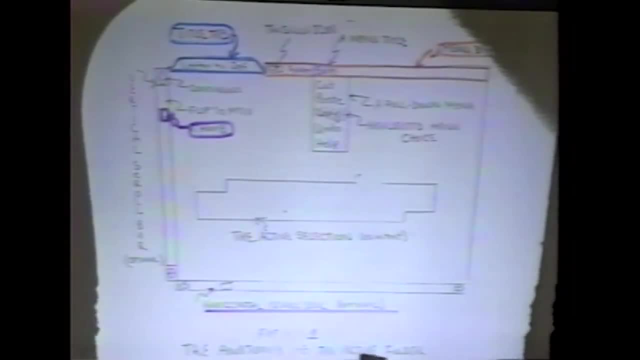 the thumb instead of the elevator, because we wanted to have horizontal scrolling too, And elevators in those days didn't go horizontally, although Scientific American says they're about two. And then we had continuous scrolling arrows And notice that the text was going to move. 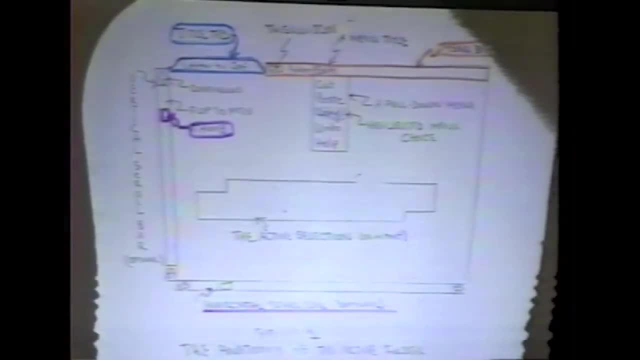 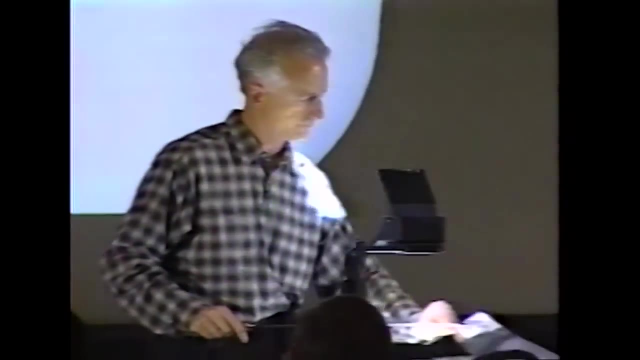 that way, as opposed to the other way, which is what it does now, And that was an interesting argument that I think I have covered here too. Okay, We had active folders, so we had to have passive folders, The folder that wasn't active. 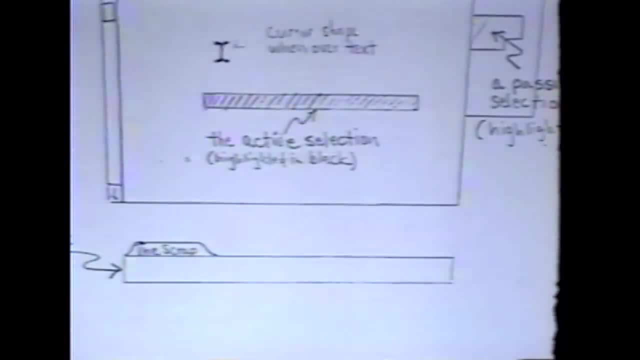 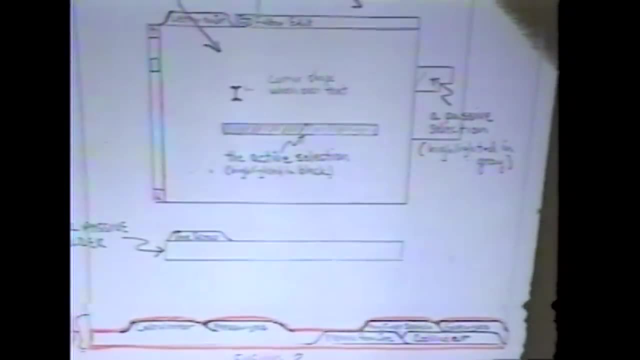 was passive. Now look at the bottom. Who has ever seen Mac OS 8?? And when you drag a window to the bottom of the screen, it just kind of pops and becomes just a tab, and then you can click it and it'll end. 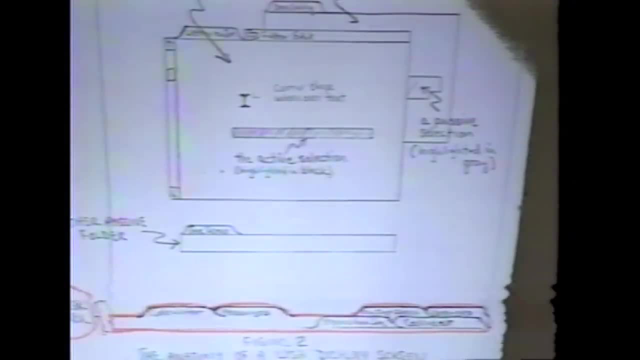 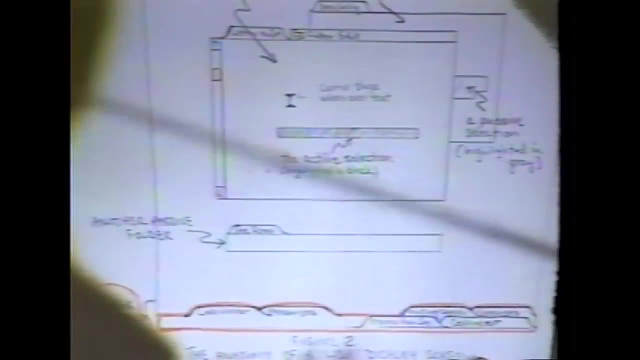 the screen, It'll slide open. Guess what? That wasn't the original design in August 1980, that what we were going to do on the Lisa, And it only took 17 years to implement. Microsoft did something sort of similar, but not really. 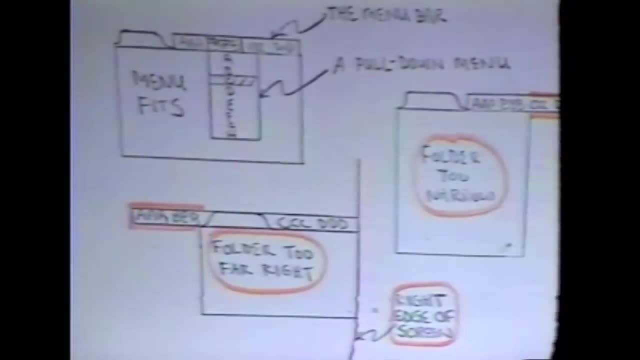 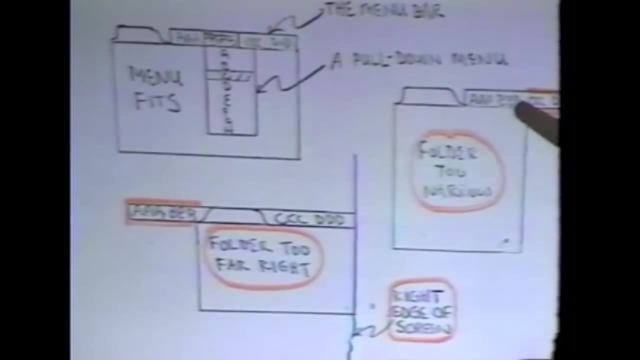 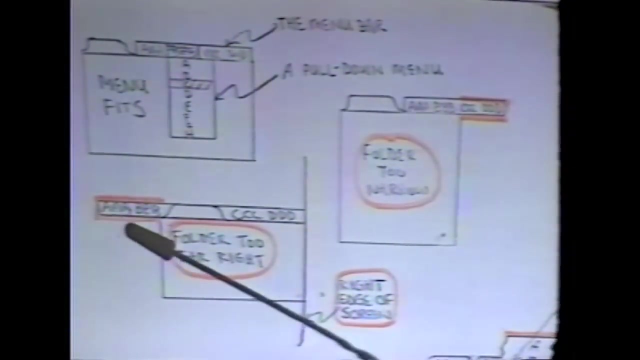 the same. in between There are some differences, but I won't comment right now. Now, so what happened if the window was narrow? Well, if the window was narrow, this shows that the menu was over on the right and it couldn't stick out to the right. 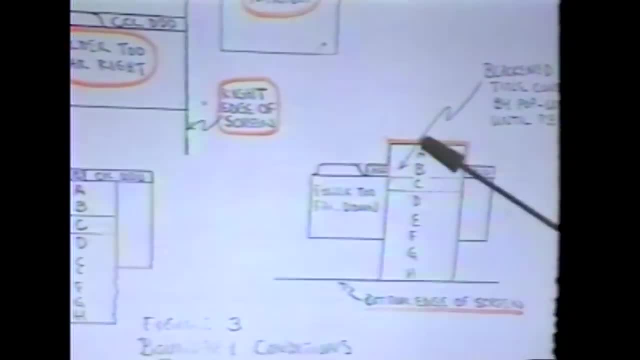 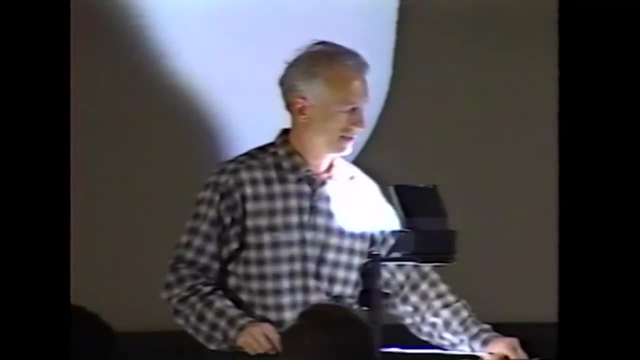 it would stick out to the left And it was too close to the bottom of the screen. then it would do this, And so Bill showed all the cases and I- you know a lot of us- weren't too happy with this, So I went back. 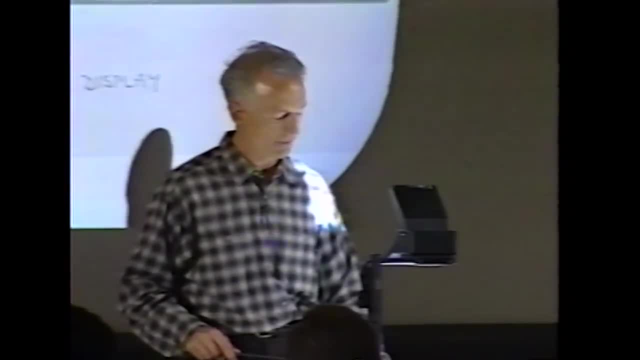 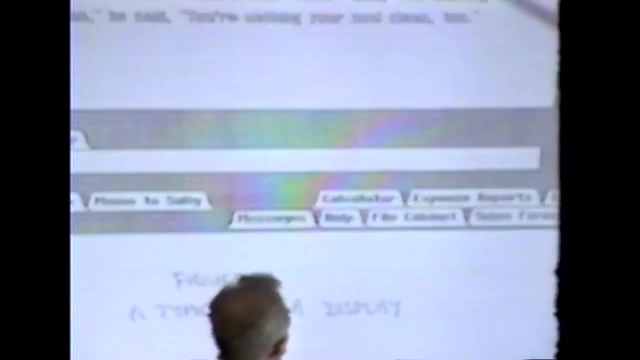 to Bill again and I said Bill, the top of the screen, the top of the screen. None of us like the idea of a two-line menu, which is the way Microsoft solved it in some version of Windows, And he's got highlighting of the menu item. 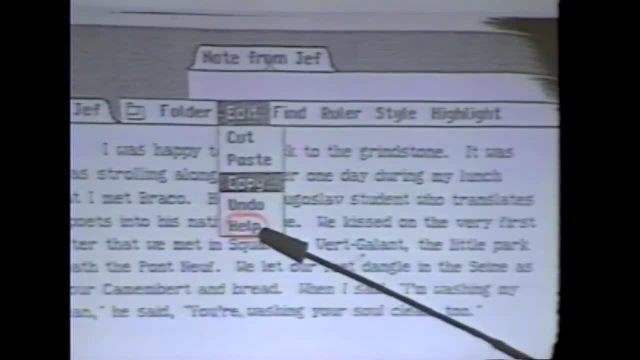 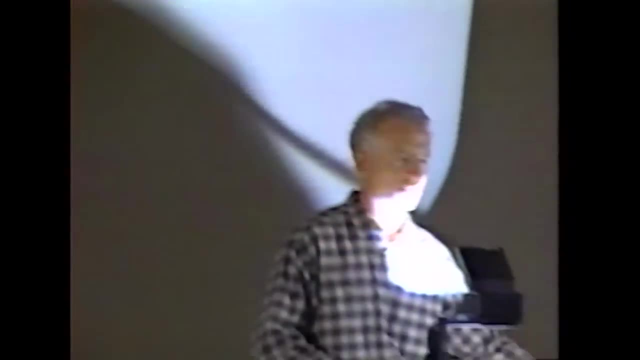 Bill had a long night one night and came back with that And we had the help menu in here. The way we operated was that Bill spent every night programming and the next day we would do testing and arguing. I don't know when he slept actually. 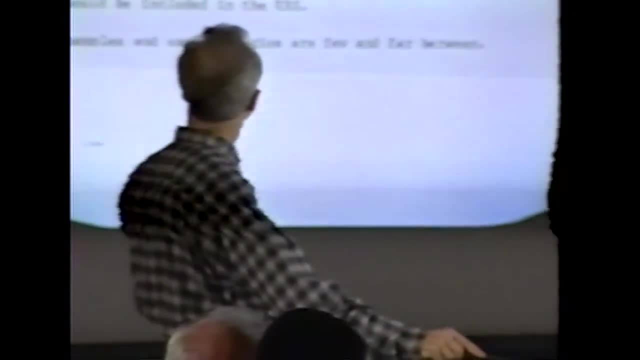 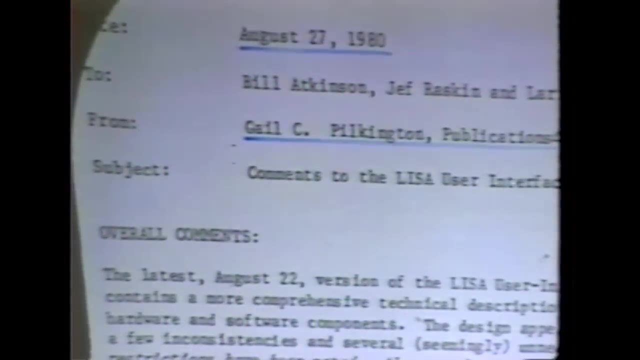 Did he sleep And then he would do it again every night. Here's a memo from Gail Pelkington. in Publications, The people writing manuals for the LISA were key in commenting on the user interface design and a lot of good criticisms. 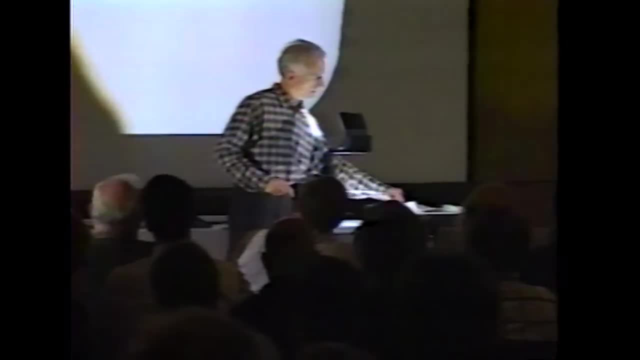 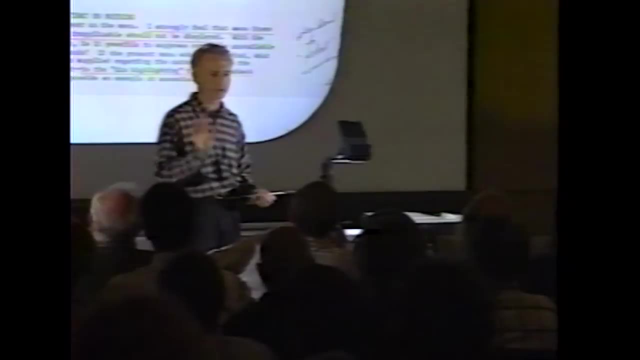 And Gail actually had been at Xerox before. So she said: I don't like pull-down menus, I think they're ugly and they cover things up. So you know I'm trying to cut something and the first thing that happens is: 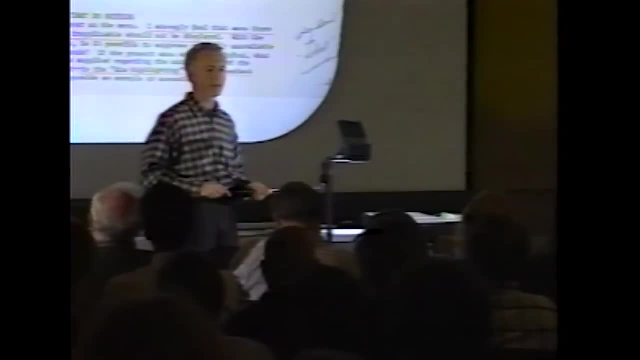 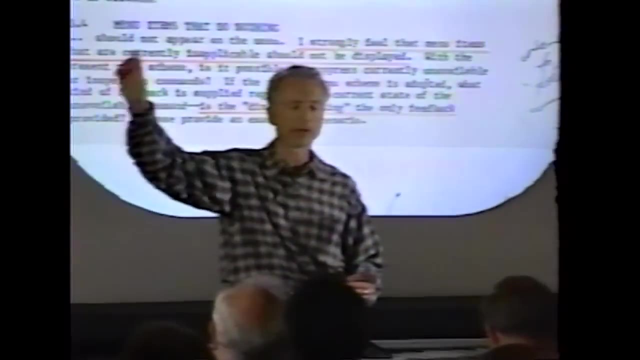 the menu comes down and covers up the thing I'm trying to cut, No good. And then Bill had this feature that you could, which he still has: you could drag the mouse along the menu bar and the menus would pop up one at a time. 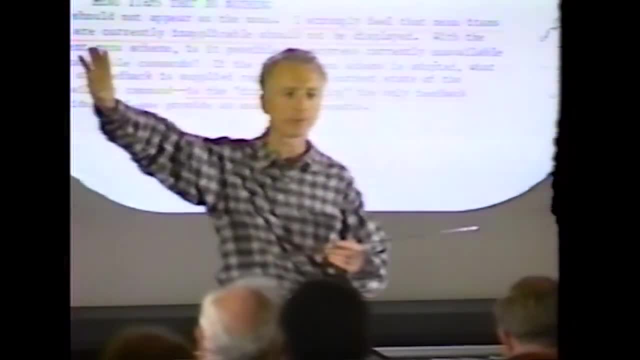 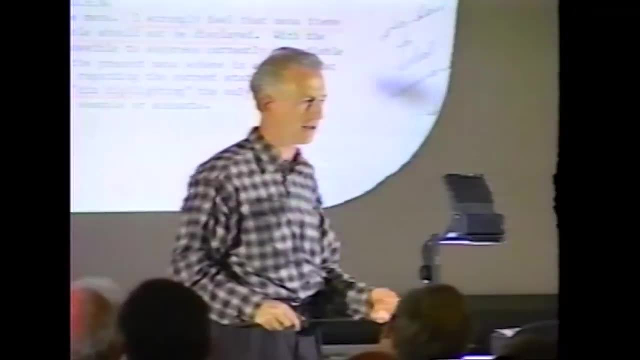 And we thought you can see all the available commands in one swoop. Well, she thought it was terrible that you had to do that to see all the commands. I don't understand, because in UCSD Pascal you had to, you know. 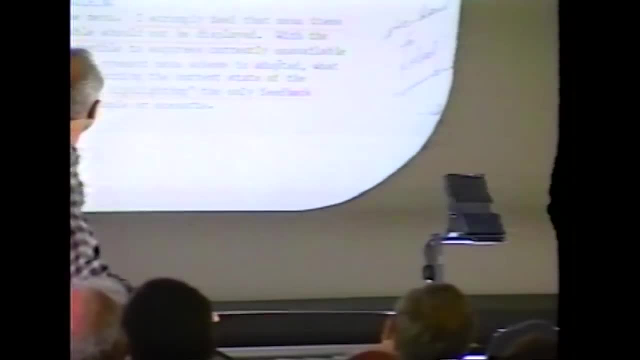 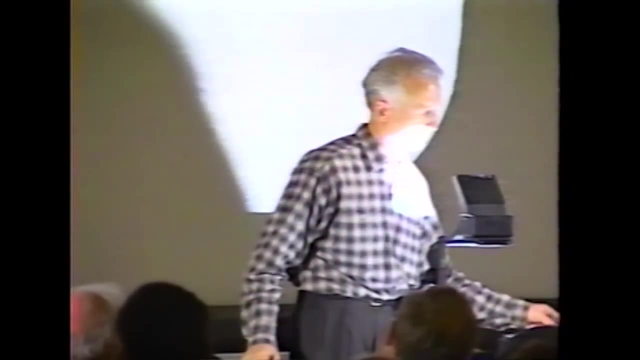 hit keys for 10 minutes to see all the commands, So I didn't quite get that. She also didn't like the idea of dim highlighting. She thought we should just suppress the items altogether. So we had dissent in the group And we always had. 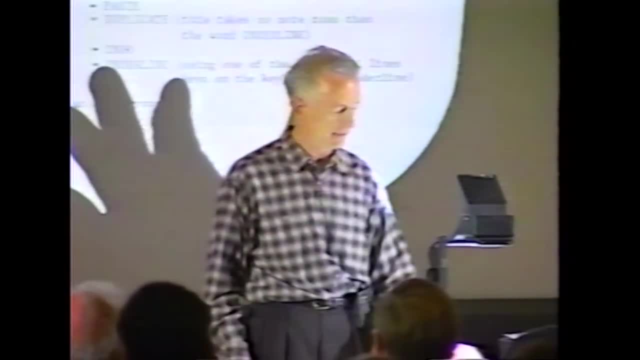 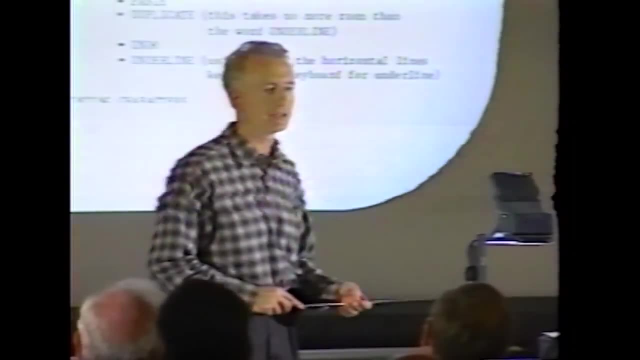 dissent in the group. I just chose that because it was a memo that I had, illustrative of dozens of people who had dissent over every issue, Nothing specific about Gale In particular. she said: you know, last version of this Beck. 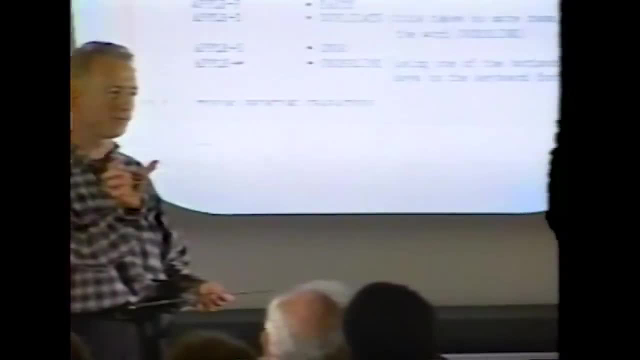 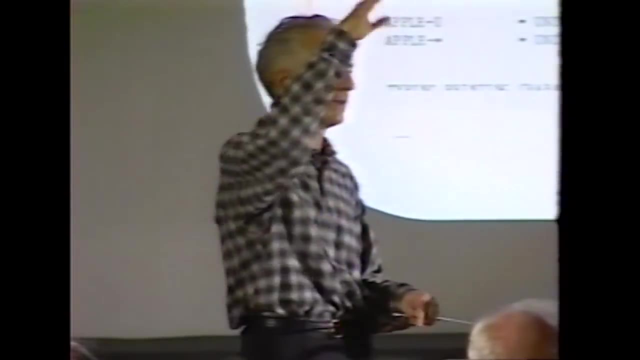 I thought we only had one issue, which was when the menu, when that little menu bar at the bottom, was full. we didn't know what to do about it, And you should have just solved that instead of moving into another place adding drop downs. 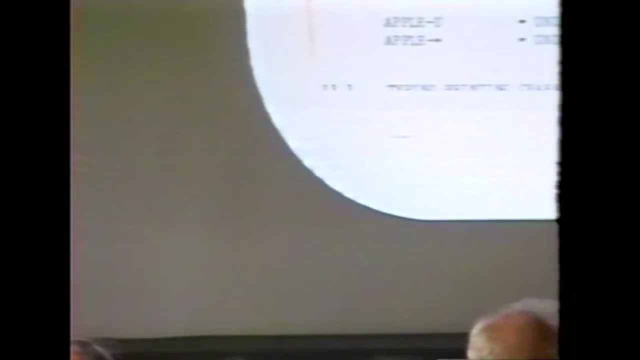 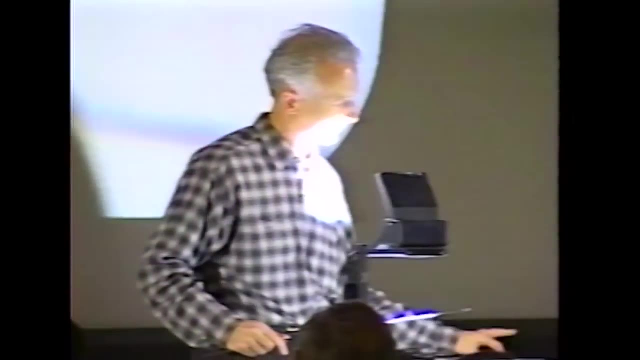 and all these other things You over designed to solve the problem. And besides, I don't like X. you know Z for cut and X for paste. She had her own proposal. that was mnemonic, So September 22nd is now a month. 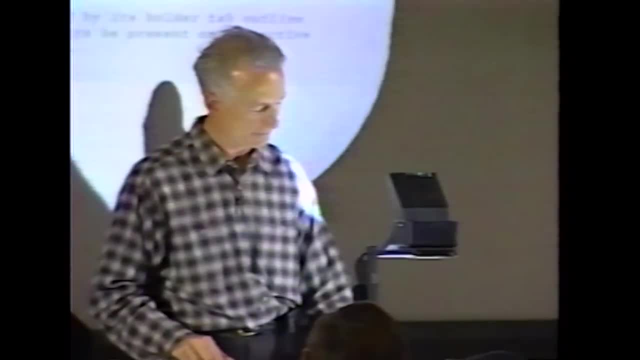 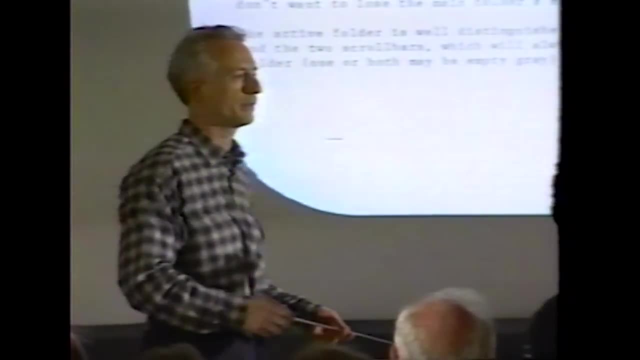 after I first said: Bill, why don't you try the top of the screen? Bill had a very long night and came back with the menu at the top of the screen with command keys, check marks, everything. I mean he had everything. 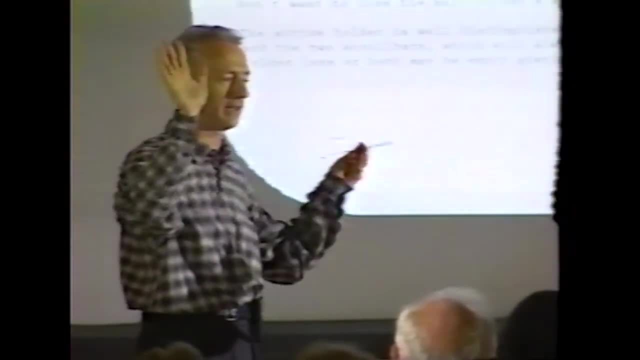 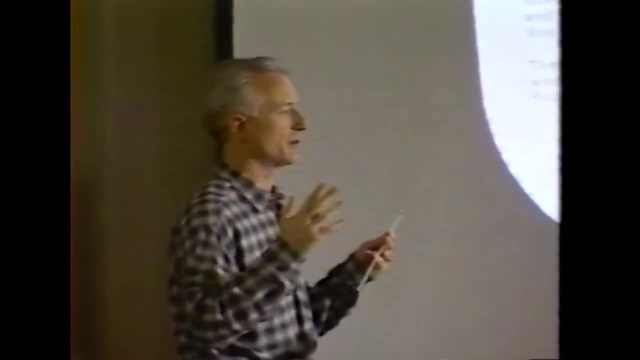 In one night he invented the entire mechanism of the menu bar at the top of the screen. To me it was just a place to put what he already had, But he, once he realized it was there, he could do a lot of other things. 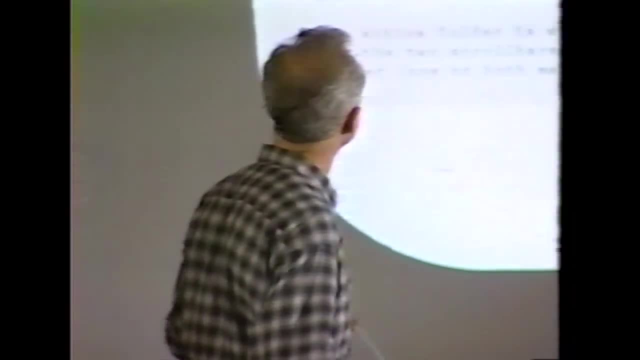 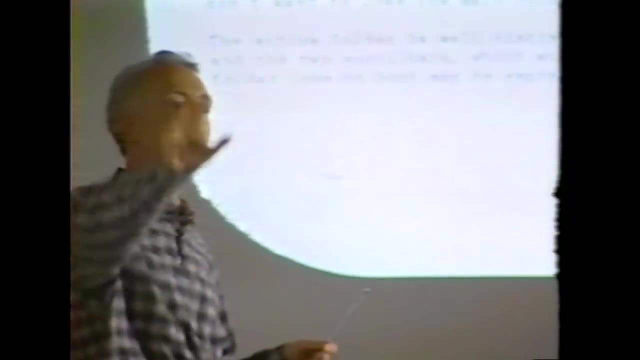 And he implemented an amazing amount in one night. So he wrote a memo to justify it and said there are some problems with it. You have to go way further to reach the menu. That's a problem, But we decided, since there were. 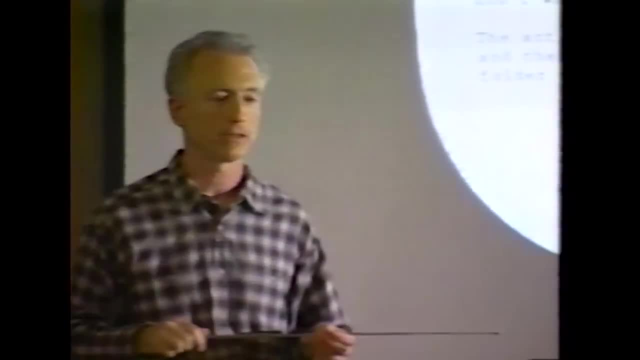 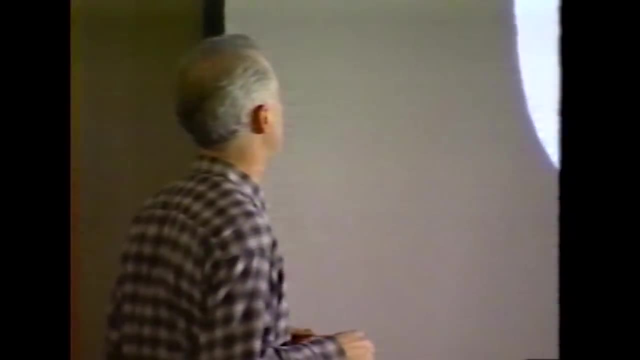 command keys and he made it very easy to have a single stroke command key in this version, this all night version, that okay, if you really wanted to go to that menu item a lot, you could hit the command key on the keyboard instead. 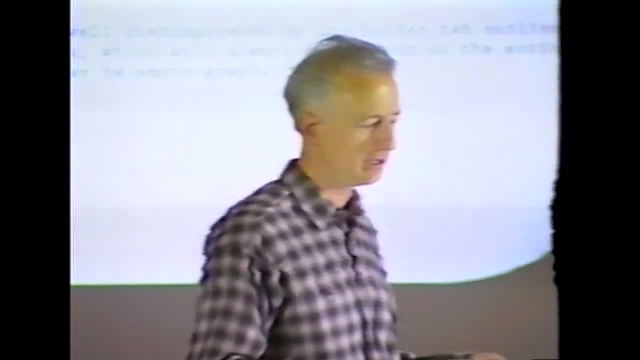 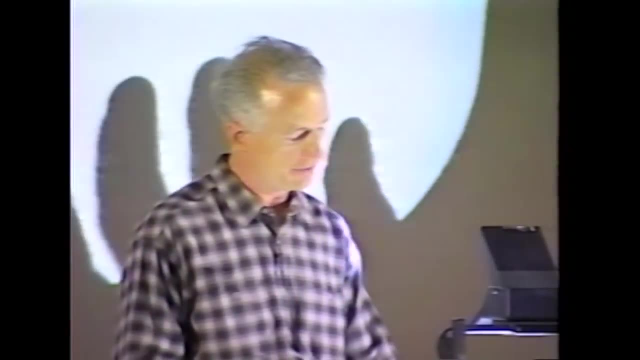 because you couldn't really be sure which menu applies to which window. and sure enough, that's still true today. But trade-offs, you know why was it good? It was good because you got rid of all those ugly cases of sticking out menus. 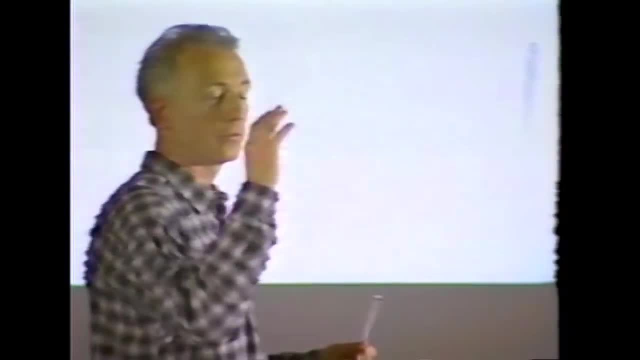 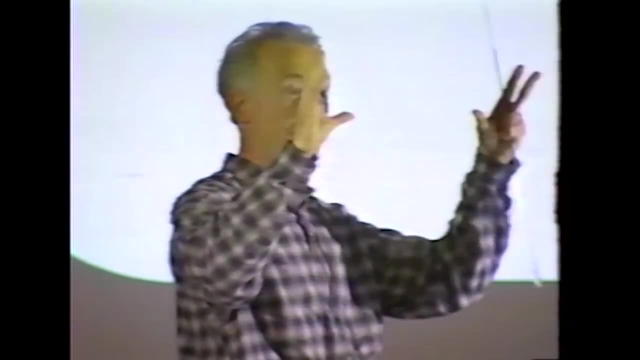 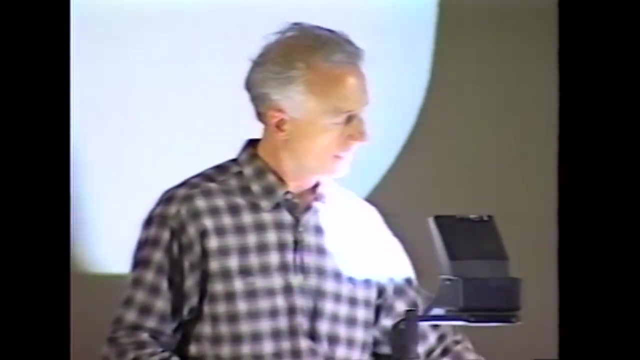 And and also the dialog box that came up when you had a command with parameters could always go in the same place, And we had a problem before with the dialog box coming up, and so we could put it in a standard place under the menu bar. 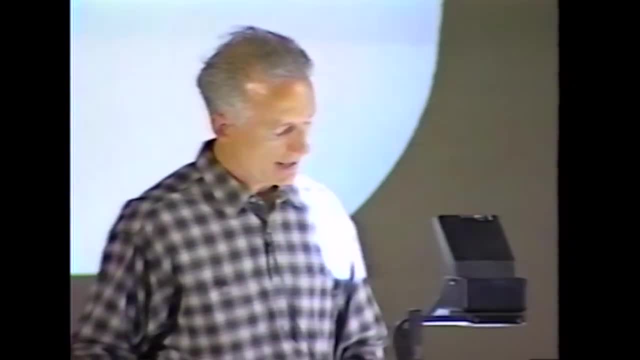 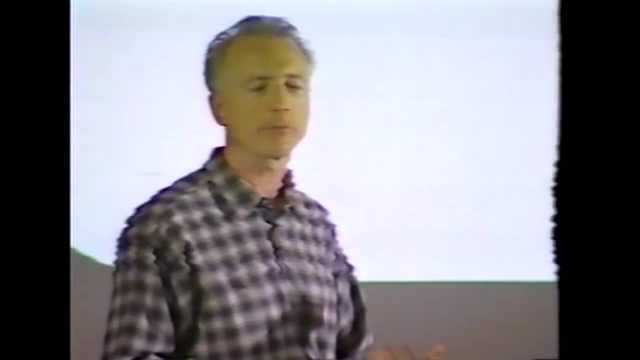 So this was all the result of his long night of invention. And then a couple more examples. we could put some global commands in the menu. Before we didn't, we hadn't figured out yet where to put the global commands. They didn't really. 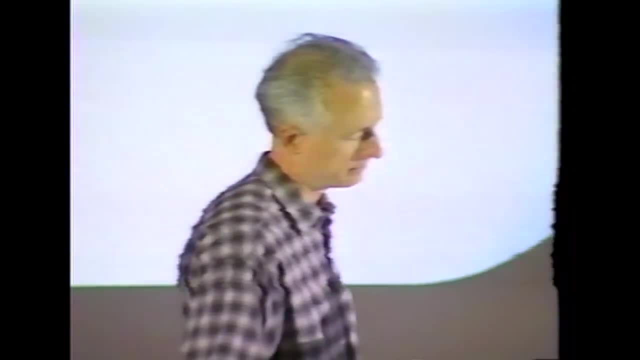 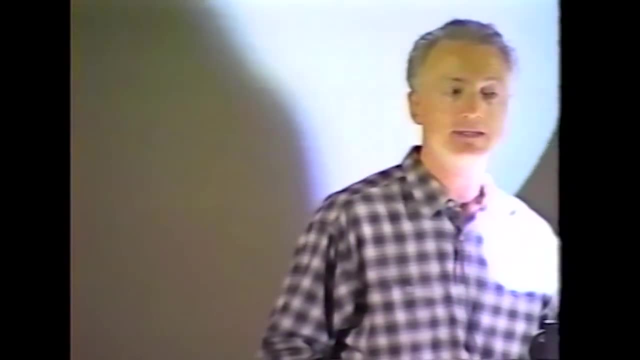 go anywhere because every menu was in a window. but now, having a menu at the top, we could have global commands, like you know, shutting down or whatever. It didn't take up room at the top of the window. Okay, now we're in February 81.. 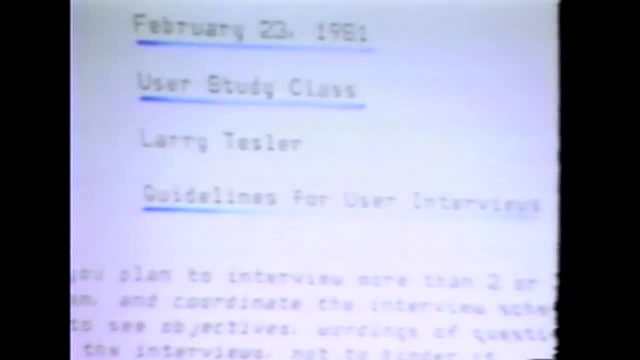 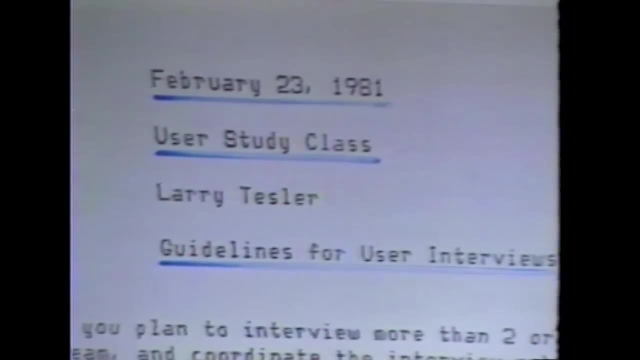 So we've leaped ahead now several months. We're all. programmers are busy implementing stuff. They're designing an operating system. telling us that we're holding up the project when they're still designing the operating system? I was in charge of the applications group. 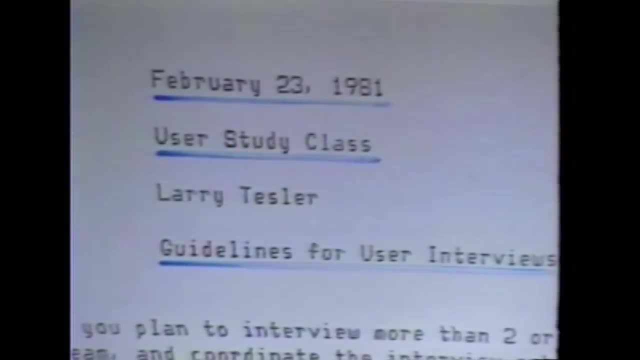 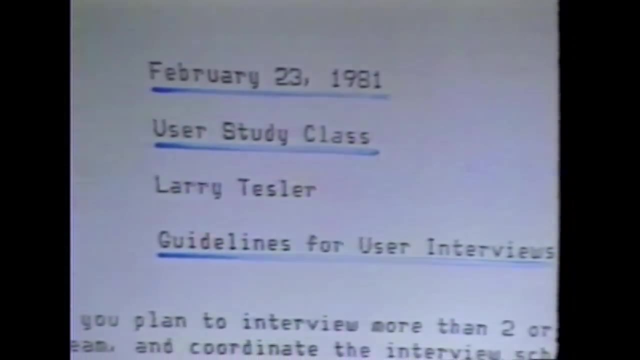 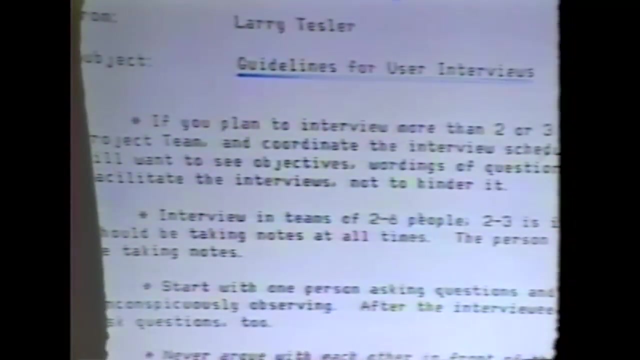 and we were the reason the schedule was behind schedule. the project was behind schedule even though they still were designing the operating system. So I wrote a memo for other people who were going to help out with user testing and I read: made guidelines for user interviews. 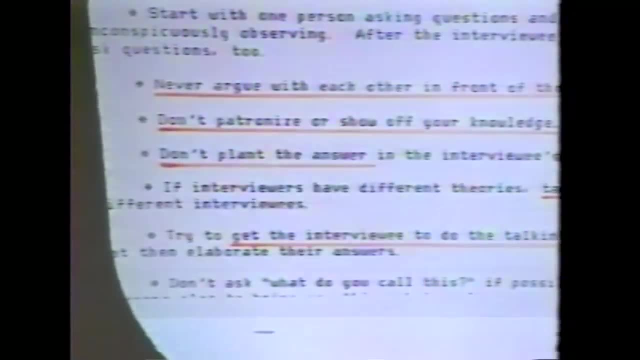 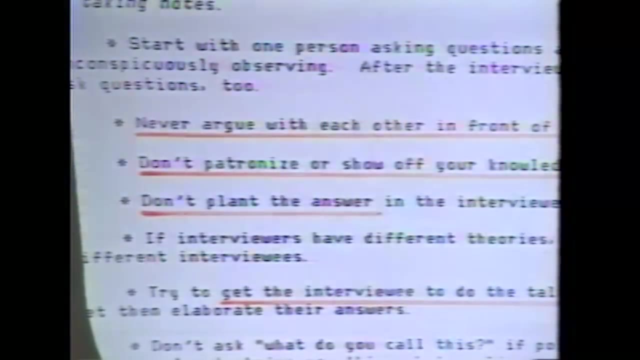 So never argue with each other in front of the interviewee After they leave. you can shoot each other, it doesn't matter, but not while the not while the subject's there. Don't patronize the subject, Don't show off your knowledge. 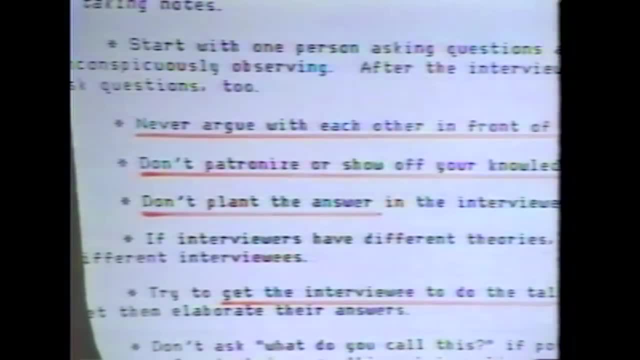 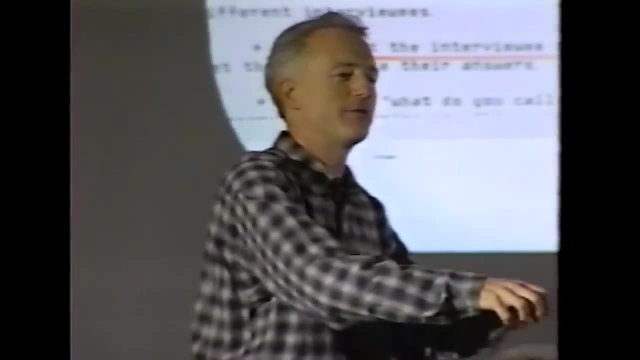 I wrote this because I would be bringing engineers into the room and I'd sit them in the back and the user would struggle to do something because they would be trying to figure out whether they want to do something or they don't. So I wrote a memo. 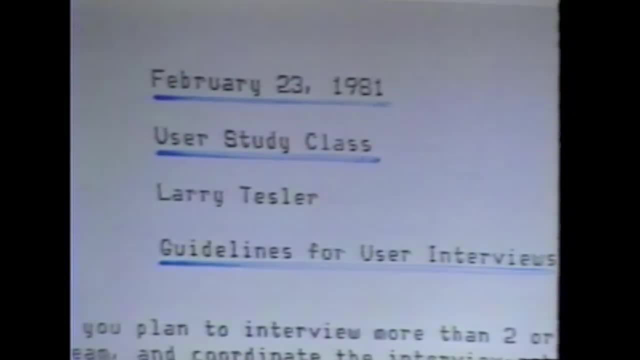 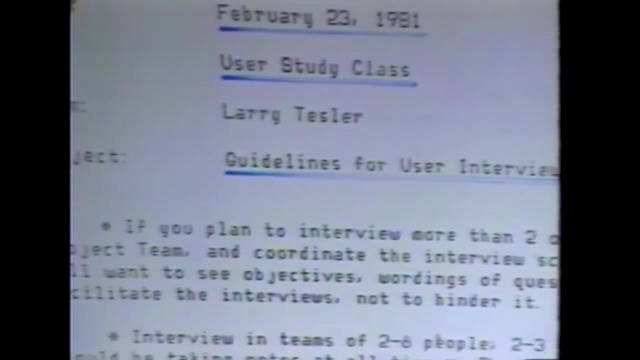 for other people who were going to help out with user testing and I read, made guidelines for user interviews. So never argue with each other in front of the interviewee. After they leave, you can shoot each other, it doesn't matter, but not while the 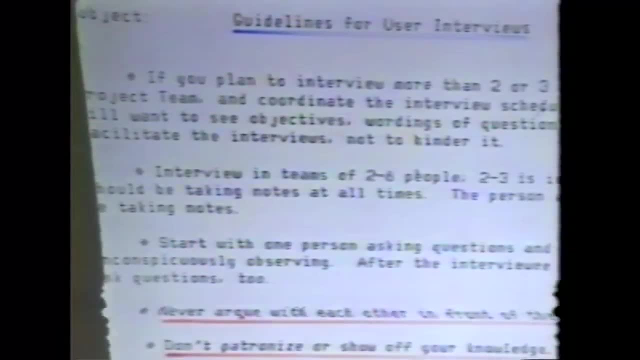 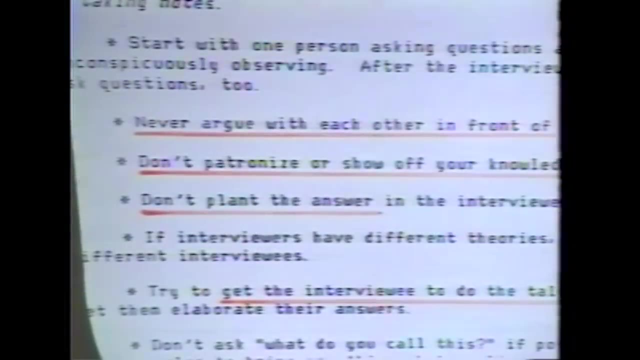 not while the subject's there. And so I wrote a memo for other people who were going to help out with user testing and I read: made guidelines for user interviews, Not while the subject's there. Don't patronize the subject. Don't show off your knowledge. 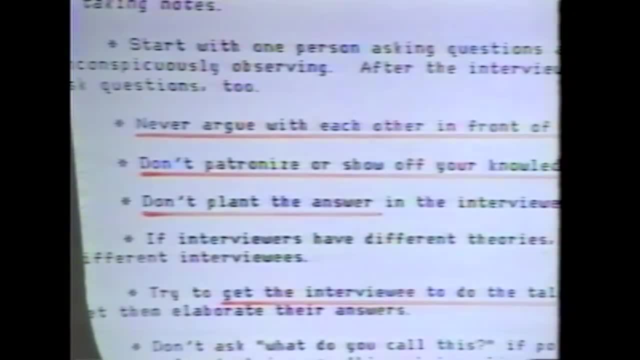 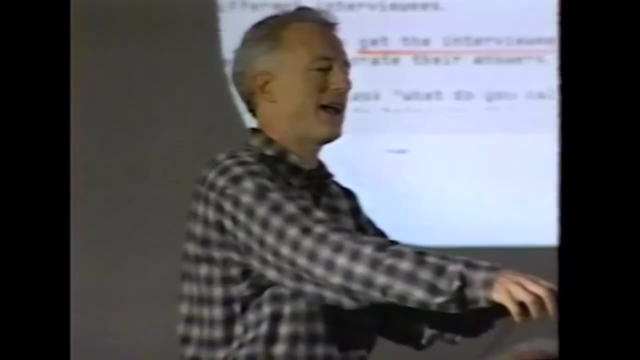 I wrote this because I would be bringing engineers into the room And I'd sit them in the back And the user would struggle to do something And the engineer would run forward, jump out of the chair, run forward, grab the hand of the person and say: 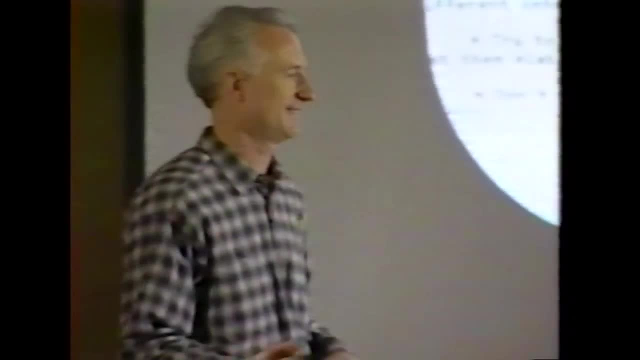 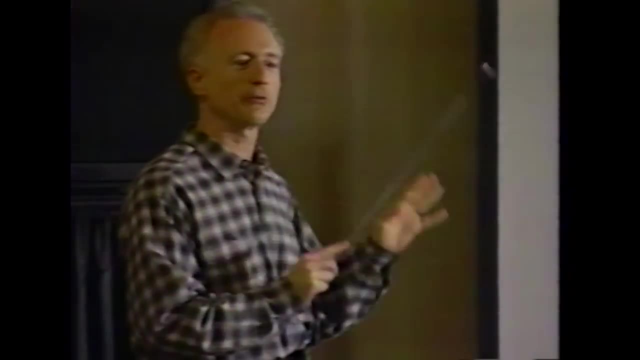 It's easy. You just do this And I go, No, no, no, You don't get it. So we tried gags, We tried all kinds of things, But finally I said: Look, I'll let you in the room if you observe these rules. 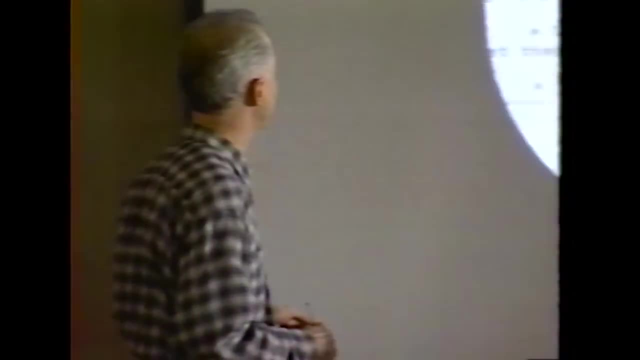 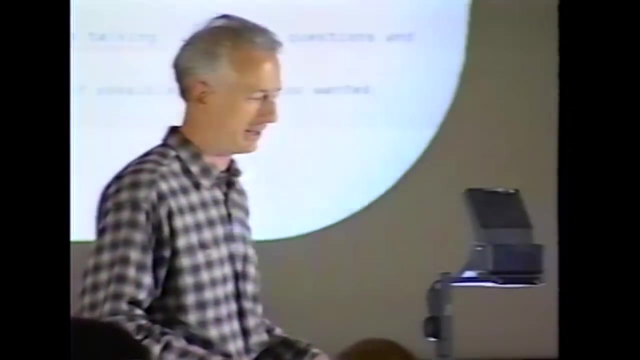 Don't plant the answer. Take turns asking questions if there's several of us there. So we get different. we may each see different things And mainly try to get them to do the talking. This is not a lecture by you. This is a test of them. 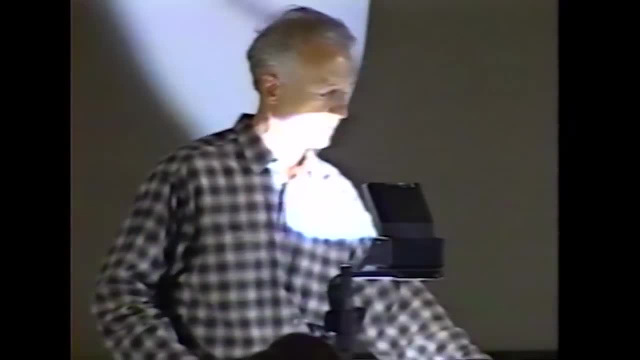 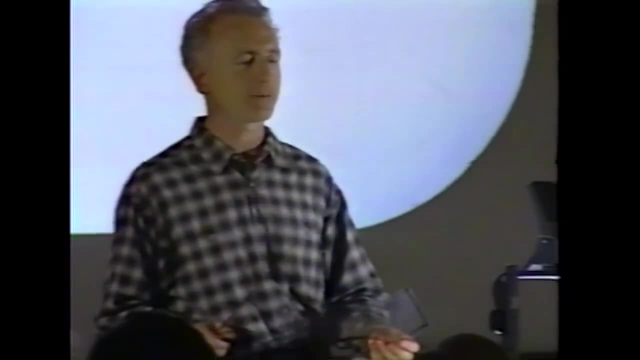 And you want them to verbalize all they possibly can. So a typical thing that would happen is we bring somebody in to prove that the user interface thing they put in was absolutely right And we were totally wrong, And then the end user would usually prove we were both wrong. 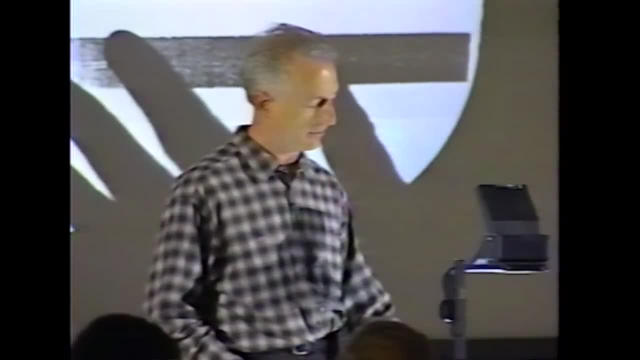 Both things were hard to use, And then we'd have to go back and redesign it, Or half the time the user would say: Well, why doesn't it just work this way? And we'd look at each other sheepishly and fix it. 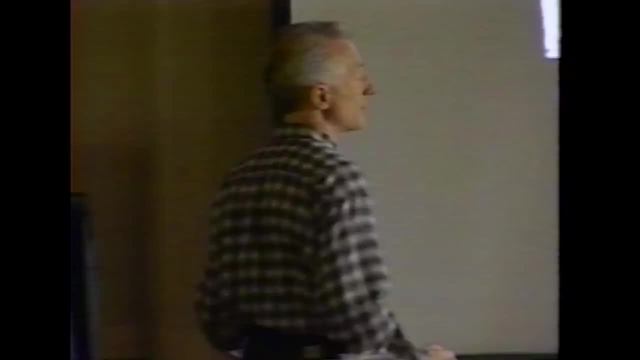 Now here was an interesting one for those of you who do user testing. If you're going to name things, you don't just say: What would you call this? People paralyze, Like, Oh, you're asking me to invent a name. 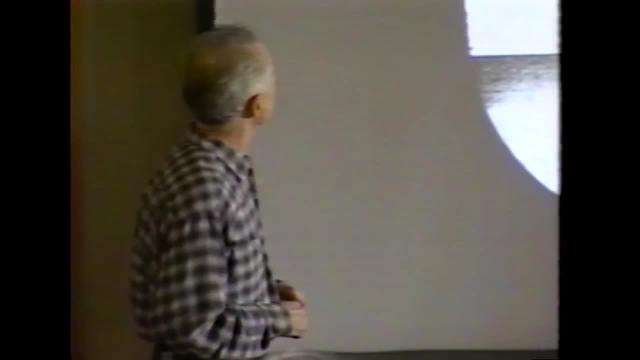 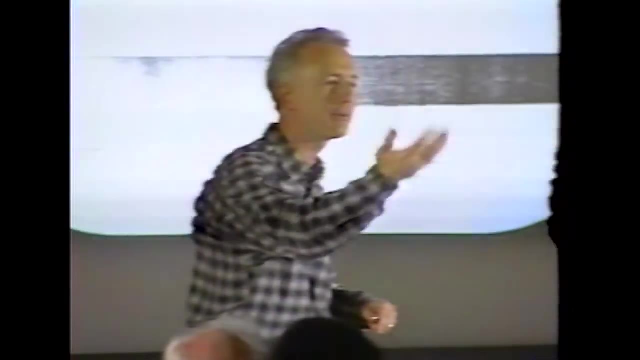 They just get totally paralyzed. They can't think of a name. But you say something like If someone were to bring you this, if you wanted someone to bring you this, what would you say? Bring me the. And then people would come up with something. 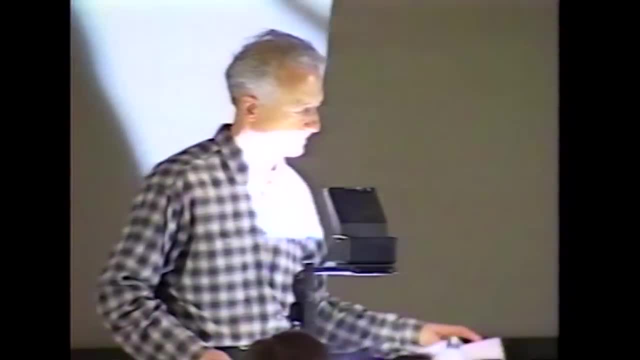 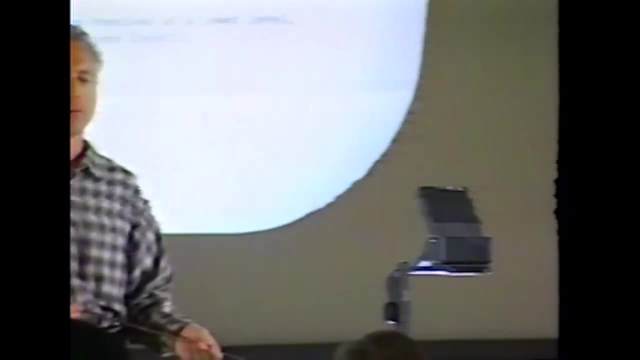 It actually worked pretty well. People have similar techniques. I've heard for other things April 3rd, 81. Well, at this point they were starting to get very nervous about the schedule. The operating system design was done, I think. 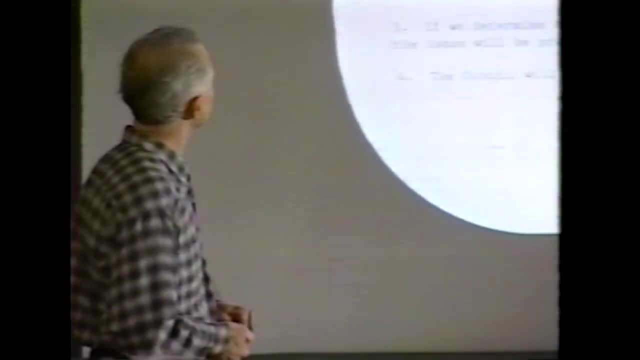 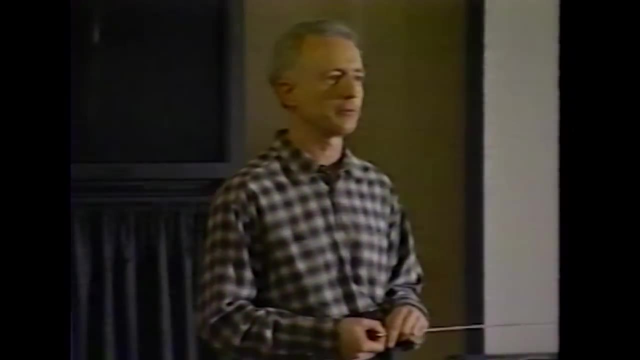 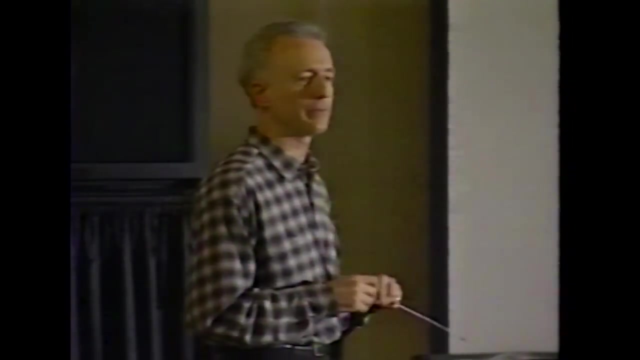 And so we were holding things up And they decided the problem was that these engineers, instead of just writing code, like like good sheep, were going in and you know, worrying about whether it was usable or not. So they decided to take all power away from us and put all the decision making into a council. 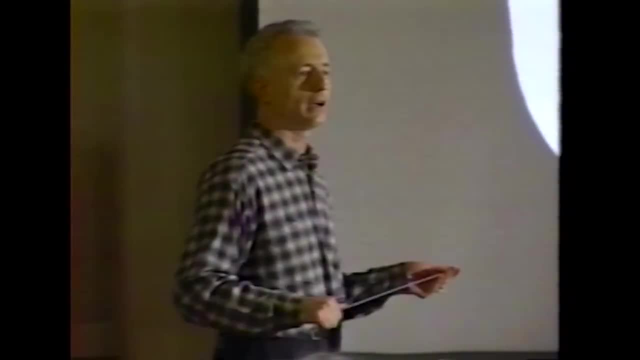 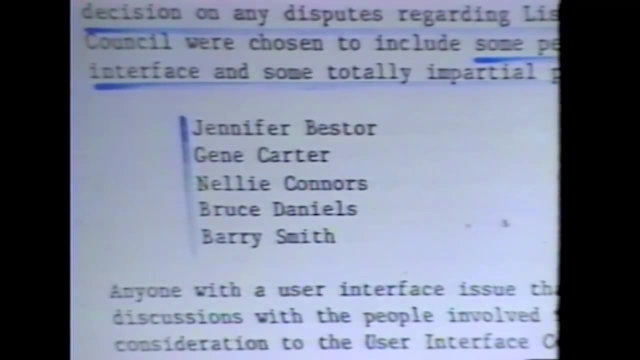 So who was on the council? First person was the division controller in finance. Second one was the VP of sales, who was always on airplanes. Third one was the head of publications for Lisa, which was a good idea. Fourth one was kind of the architect of the group. 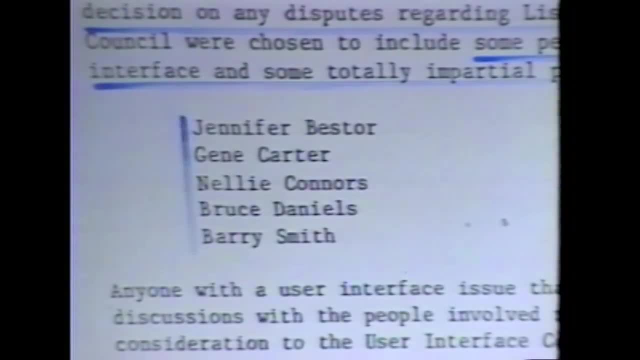 That was good. And the fifth one was somebody in product marketing who you saw had made comments before. that were pretty good ones. So I was looking at this going: OK, maybe we can live with this, But the main thing they did that was very good is we instituted a process for what to do if you had a user interface issue. 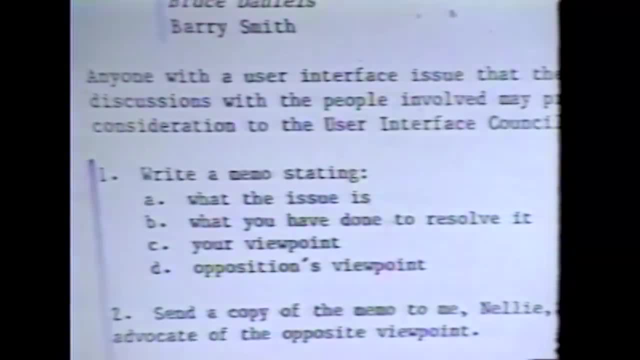 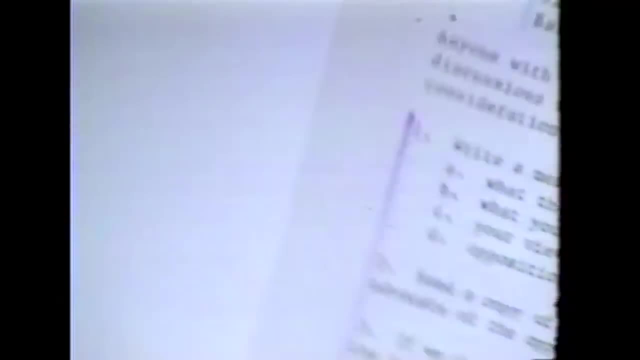 Don't spend eight hours arguing with each other. Write it up, make your points, get back to work And then we have a process for dealing with it, But the council will rule by majority vote. So I think what a way to design a user interface by majority vote of the controller. 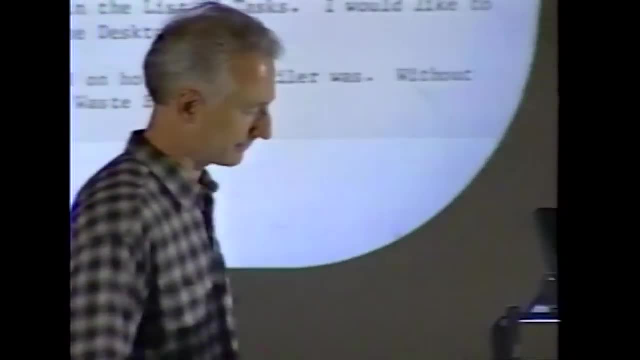 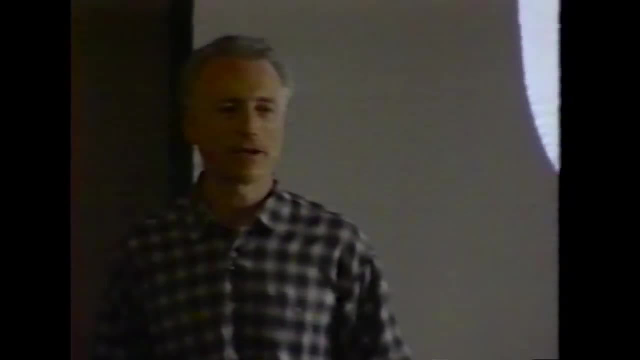 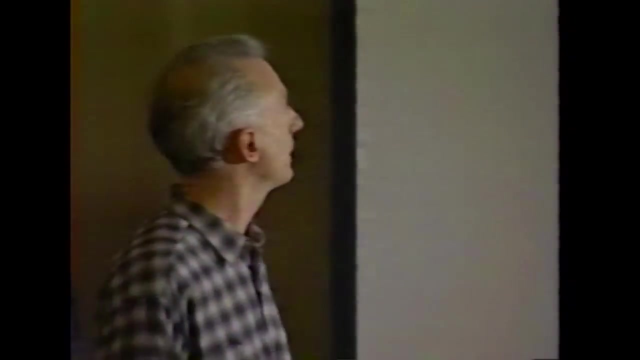 The sales VP. OK, But we started. this motivated those of us who decided we had to do this, the right way to actually run more user tests, Because we thought, well, maybe we can overwhelm them with facts and that'll overcome this reliance on votes of committees. 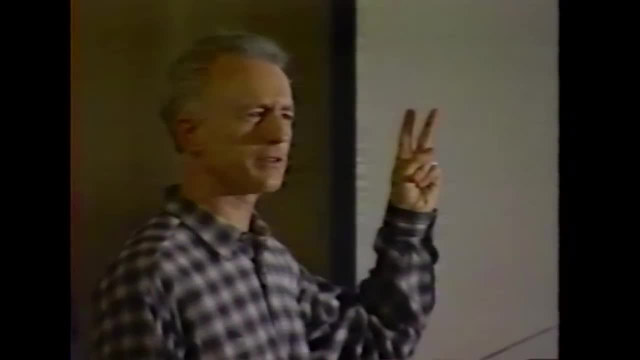 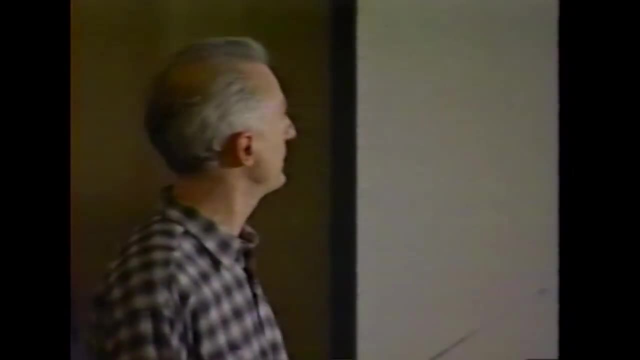 So Chris Dewar, I can't remember. Wallace Judd, I think Wallace maybe worked at Xerox before this. I can't remember. These are two people that got involved with user testing. The filer is what you think of them as the finder today. 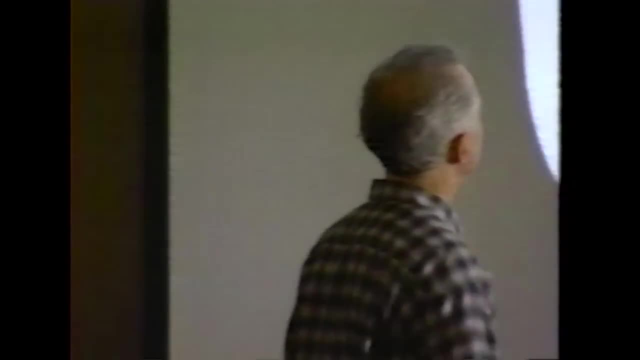 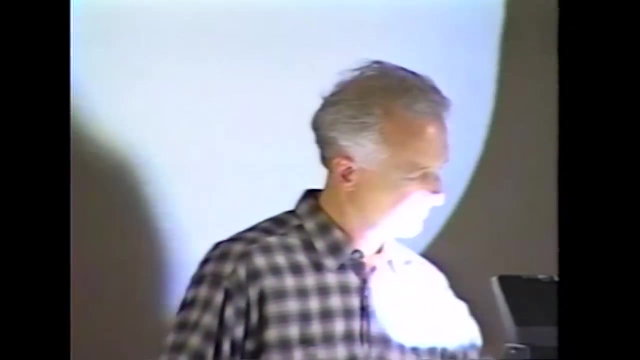 And they ran some tests and came up with all sorts of comments. I've underlined a couple here, Like there needs to be a way to select multiple icons at once- Well, they weren't icons yet, even- But ways to manipulate multiple things at once. 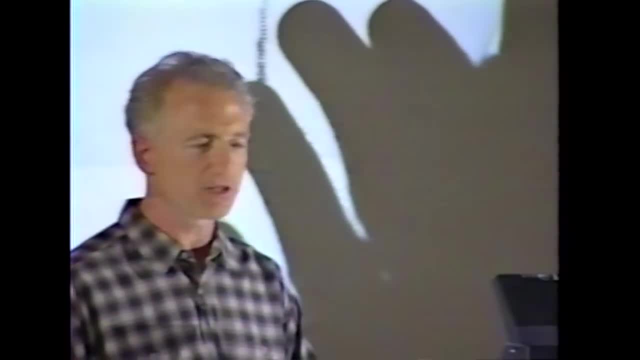 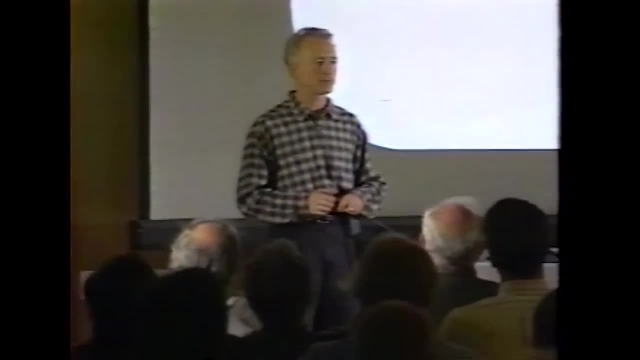 But basically, after making some comments, they said: you know, this is a good idea. Their own personal experience with testing was that you hired a testing firm, you spent a lot of money. three months later you came back with test results. 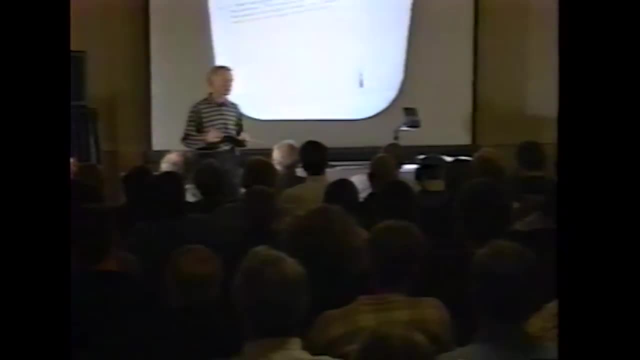 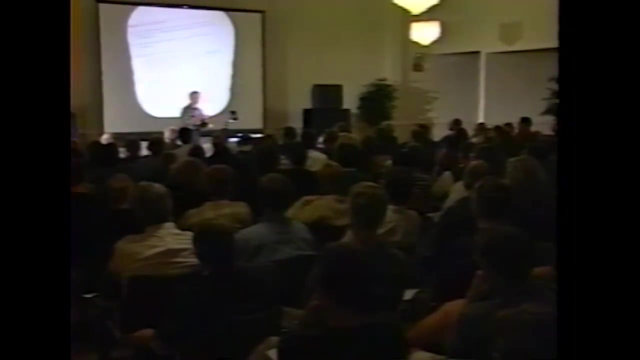 And then you did some things and then you did it again. you know it took forever. And they said: you know, or they would take a book and give it to a subject, have the user read the manual, try out the manual, videotape the whole thing. 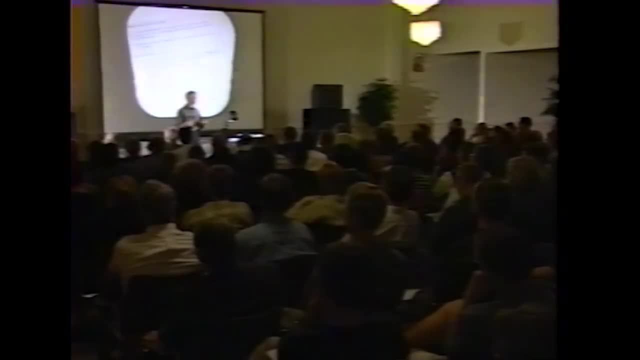 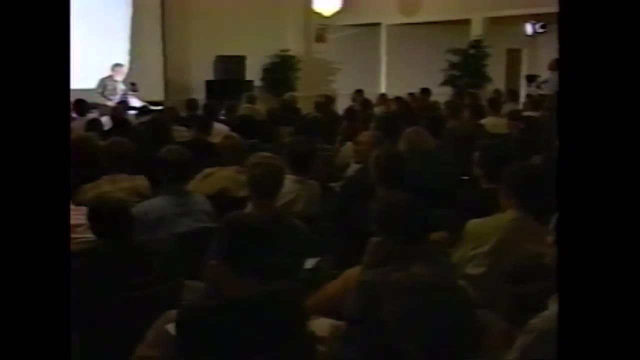 And she said: you know, this wasn't bad. just sitting down next to the user and having a dialogue with the user, trying to get the user to talk and express what they're doing, is not a bad way to do it. So that was good that we got the people doing the user testing to adopt this much knowledge. 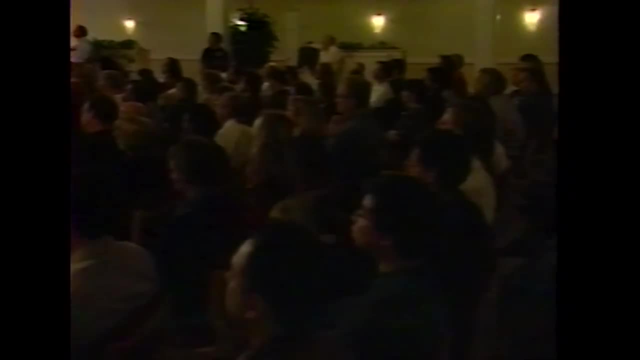 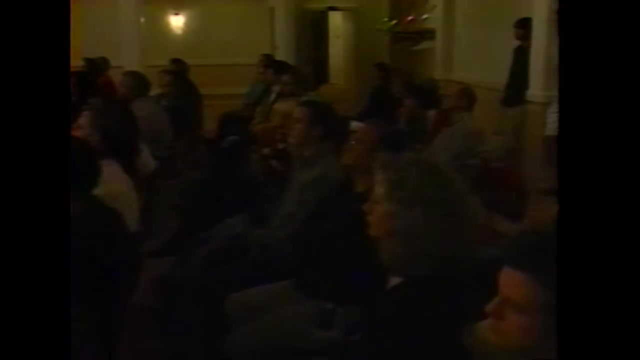 So that was good, Thank you. Adopt this much simpler and cheaper paradigm. We tape recorded the sessions and they found that useful. They went back and listened to the tapes And, however, the tapes were hard to hear because the people in the room were making noise. 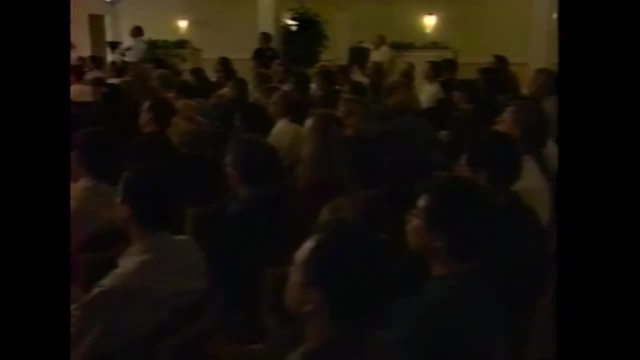 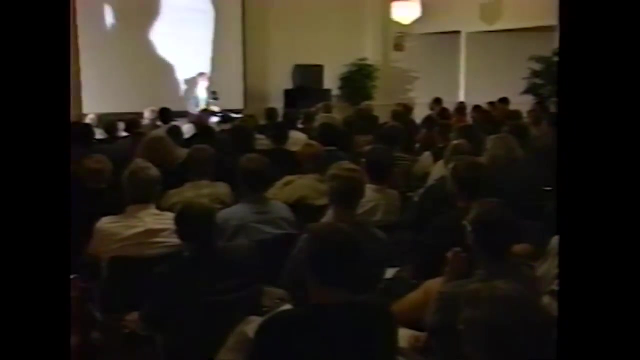 So they asked the observers to be quieter. I'm going to have to remove these from the box now. It starts going a little quicker now. But one problem, she said, was that we're only testing Apple employees. We would get Apple employees. 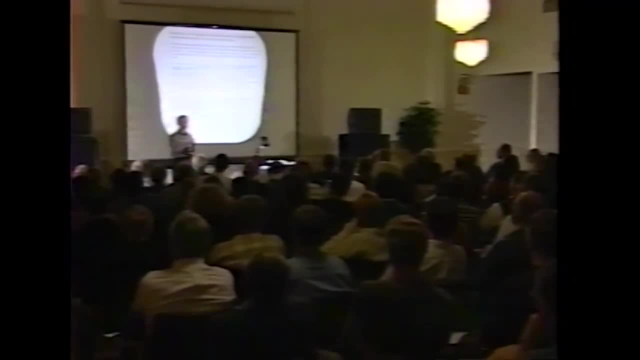 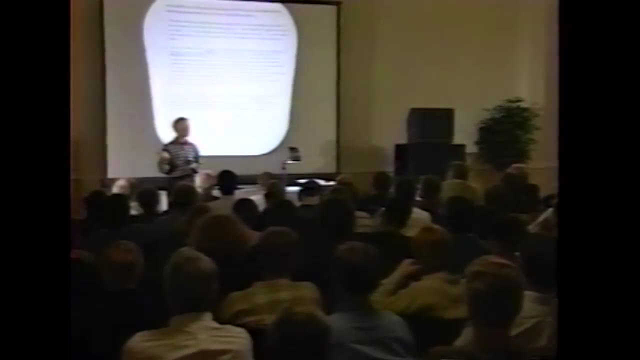 The day they took the job, the day they started work, we'd get them in orientation. The person running orientation would say: well, after orientation, you go straight to work or you go, you know, be a user test subject. 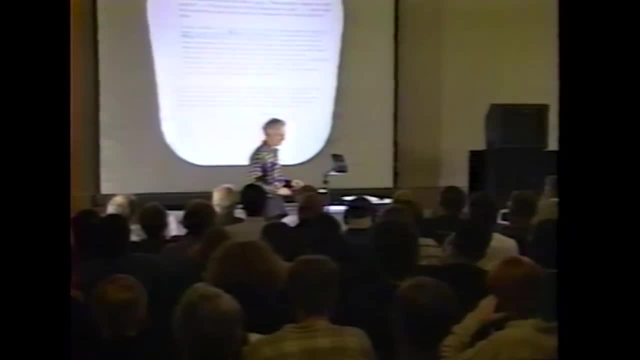 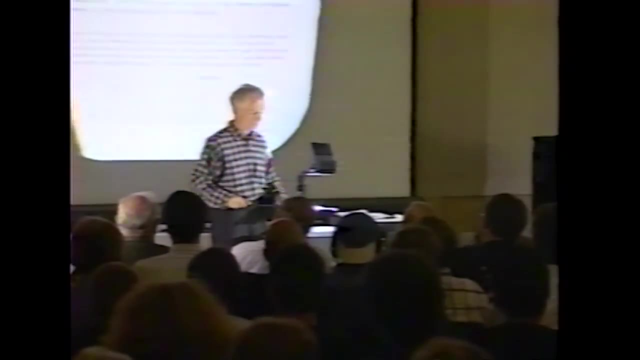 And, hey, you get out of work for a few more hours. So we got a lot of people to come over and be user test subjects, And almost all of them had very little computer experience because, although Apple would have liked to hire people with a computer experience in those days, there weren't very many. 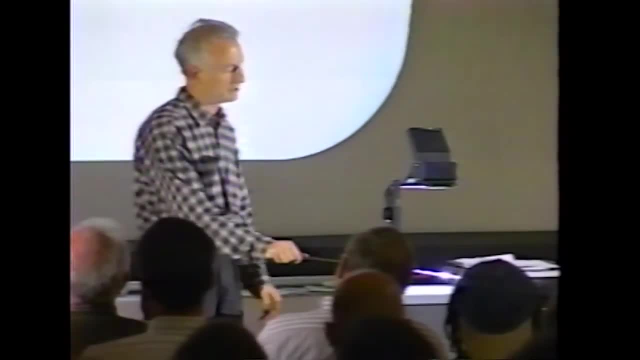 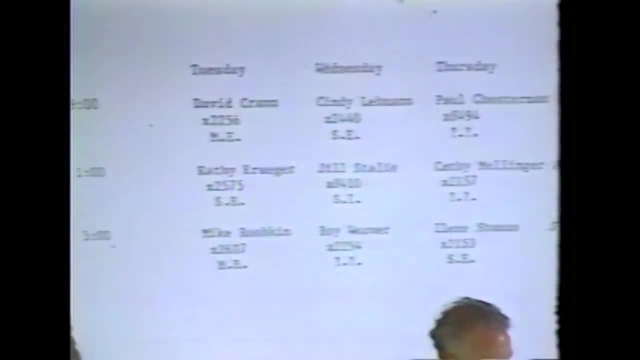 So, and here's a typical schedule, One it was. we weren't trying to do two an hour anymore. One person at a time, one each day, nine o'clock, one o'clock, three o'clock, much more civilized. 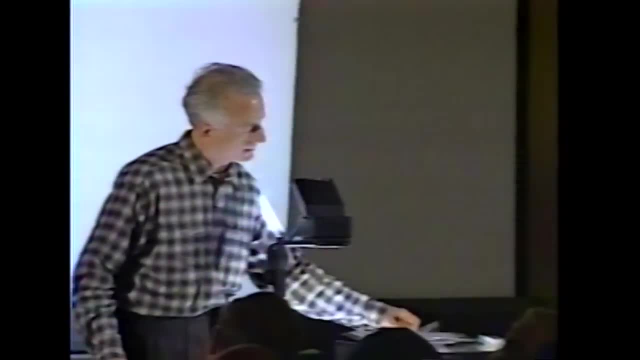 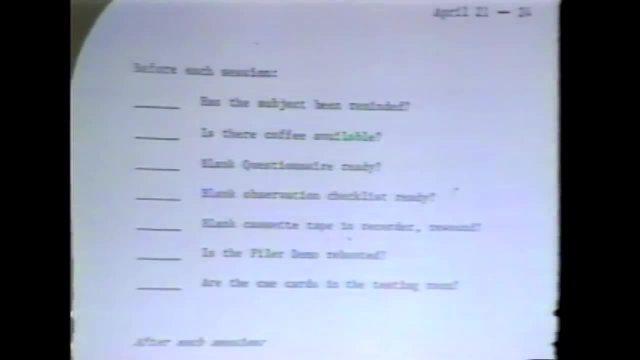 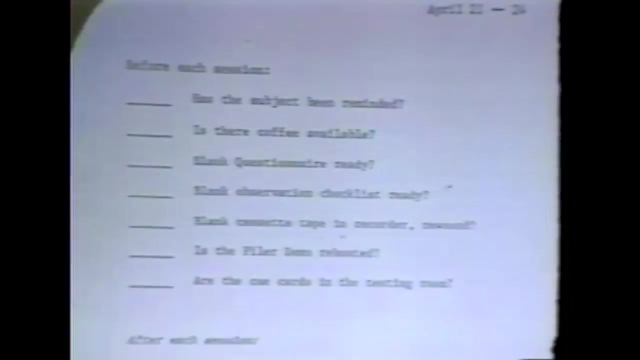 And we had a checklist that the tester went through Before each session. have you reminded the subject of whatever? I have no idea, whatever they're supposed to remember. there's some list. Is there coffee available? Do you have a blank questionnaire ready for the person, because we had them fill out a questionnaire at the end. 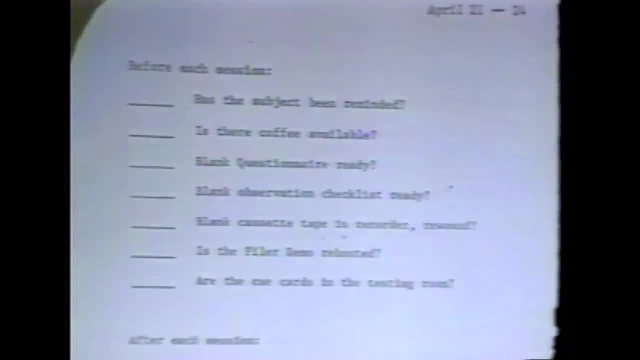 Do you have the checklist ready? Have you rewound the tape? Have we rewound the tape for this talk today? Have you rebooted because it crashed? if you didn't, Are the cue cards in the testing room, et cetera? 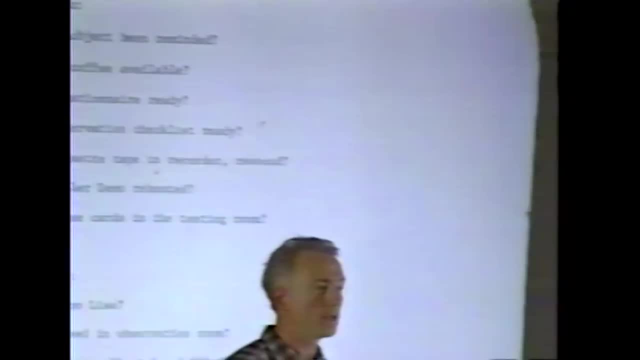 After each session did you cover up the Lisa again, because the room had a window and at night you could see in the window and see the secret Lisa machine. Did you close the blinds for double measure, et cetera, et cetera. 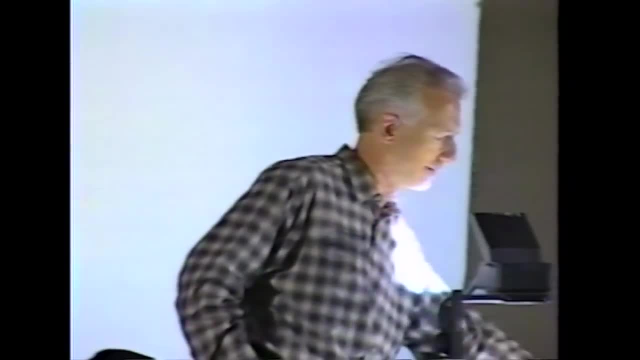 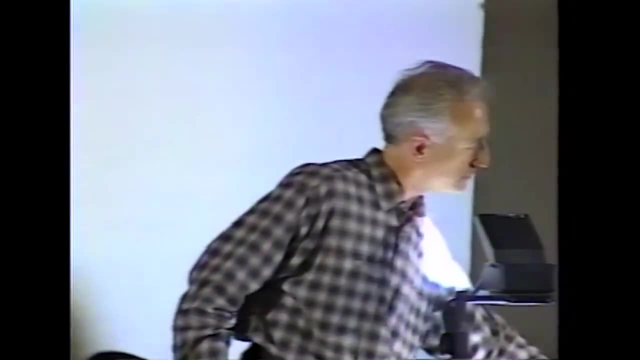 So we had a lot of questions. We had a lot of things to remind the tester about. That's a good idea. if you ever run user tests, have a checklist. Now Wallace, the guy who received the last memo, wrote this memo about some testing results. 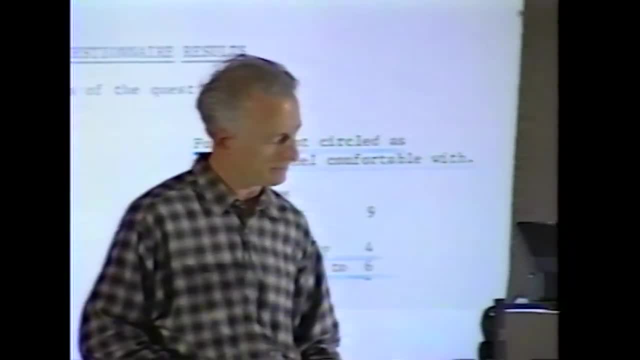 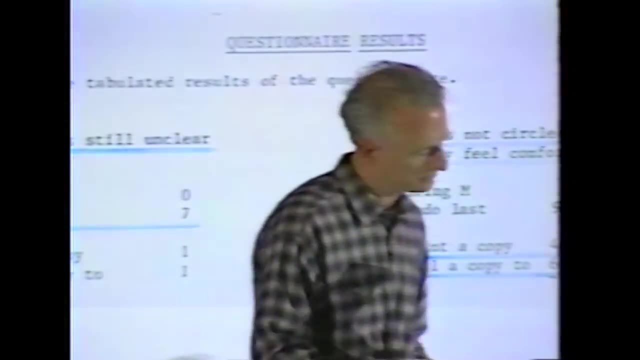 And he said he spent about an hour, a subject which was pretty typical. That's the way I like to do testing myself. And he said: well, some functions were still unclear, in particular seven subjects out of how many, It doesn't say, but not a lot. 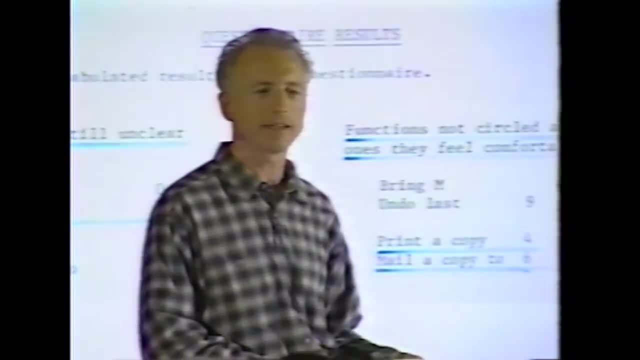 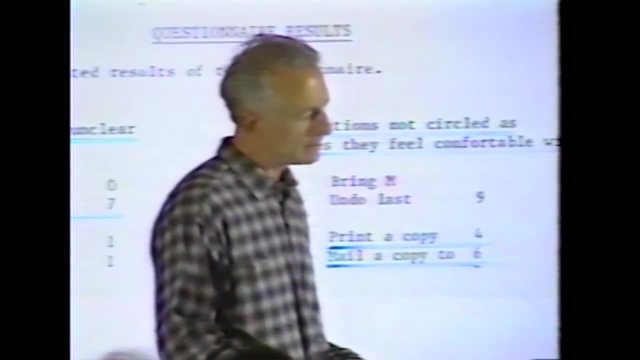 Well, not very many. Most of the subjects had trouble with undo last command. They'd never seen such a thing in a program before and they just didn't quite understand what it meant. Then there were other ones they understood but they didn't feel comfortable with somehow 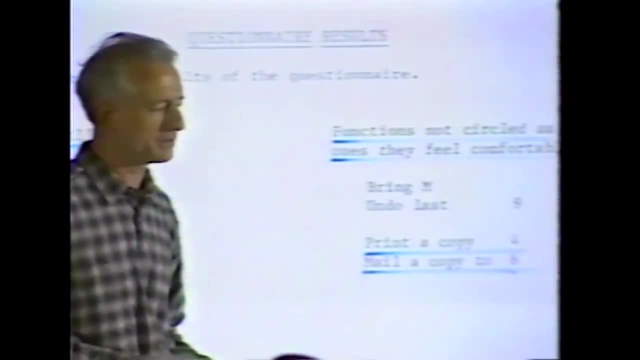 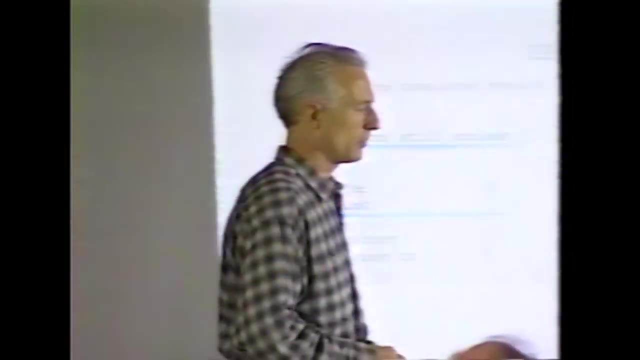 One was print a copy, one was mail a copy. Well, I believe the reason was that we didn't have printers yet on the machine and we didn't have email. In fact, we never had email, so we're probably just shown these and not really couldn't use them. 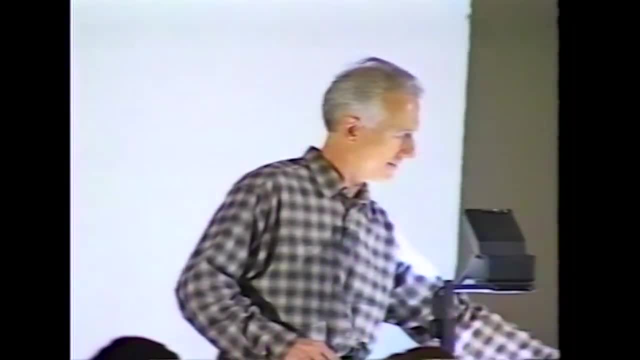 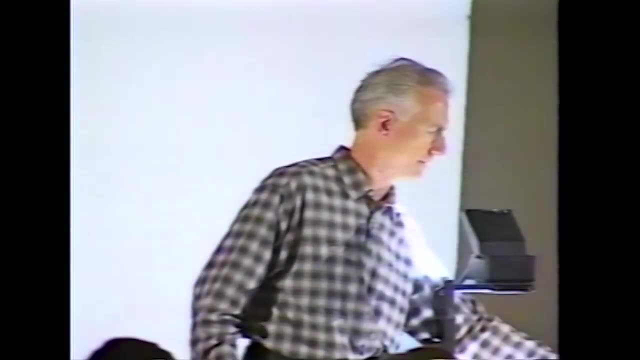 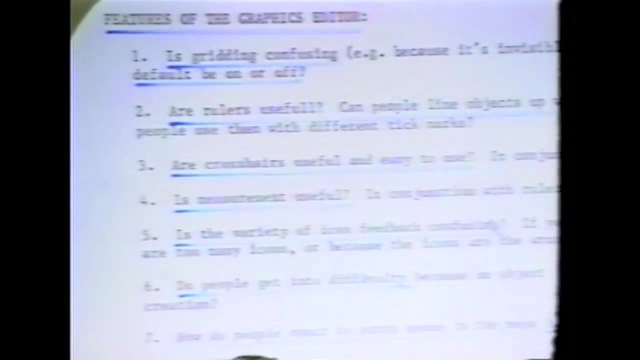 And so, of course, they didn't understand them. Graphics editor- user testing. this was LisaDraw, which became MacDraw, later implemented by the same guy, actually Mark Cutter, And we wanted to test various things. was this confusing? is that confusing can you use? what happens if you try to use rulers at the same time as crosshairs? 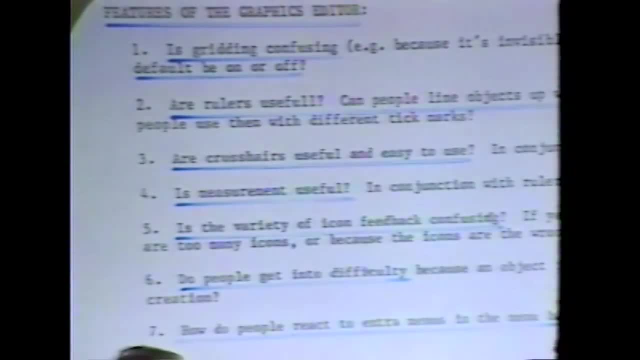 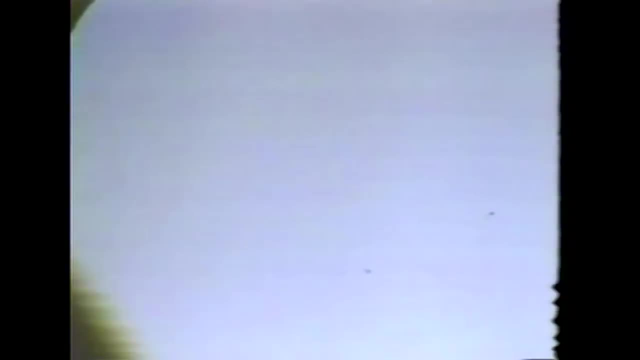 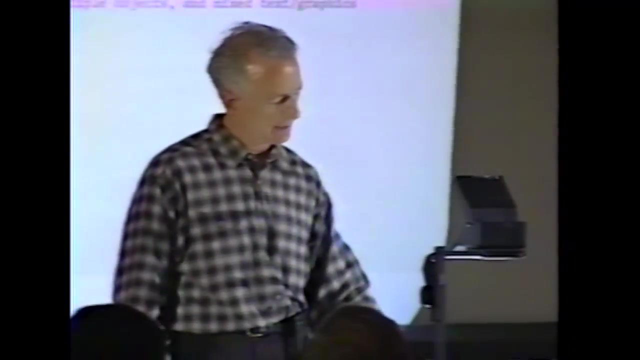 Is that too many things on the screen? And considering all the widgets that are there today in a Photoshop or something, why were we worried? But there was even worry about whether people could use a graphics editor. So we did that. We didn't use a graphics program because, well, you know people, most people can't draw, so they wouldn't use a graphics program. 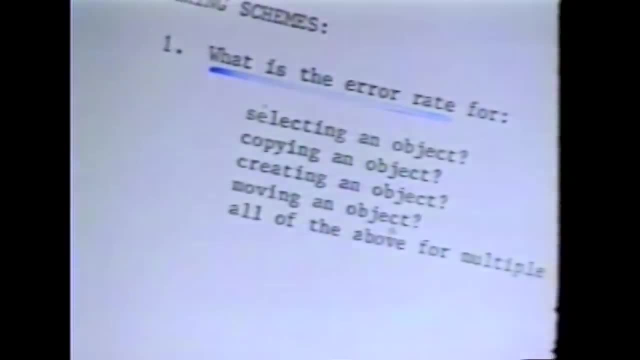 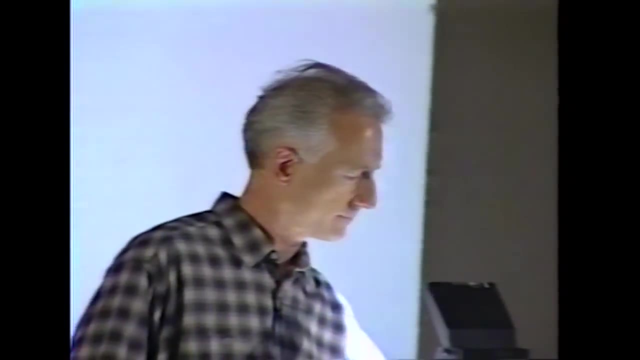 And we also wanted to know the error rates, And so a lot of counting was being done and looking at tapes to see how many times people made errors and try to reduce the error rate. So we're trying to be sort of scientific, even though we were on this headlong schedule. 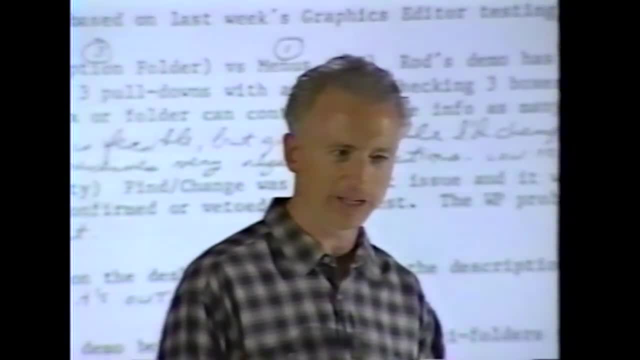 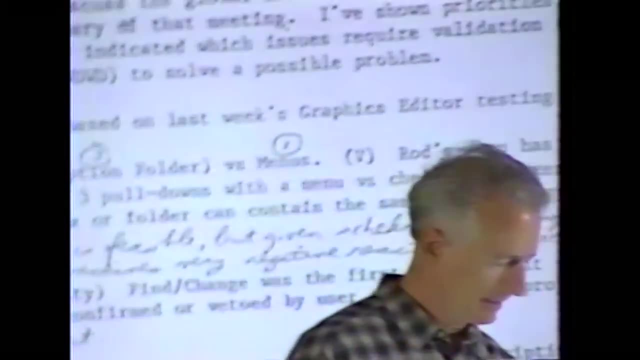 You may have noticed that six months have already gone by and we haven't shipped. In fact, it's about a year at this point. Okay, So June 81. Pat Marriott: He writes this memo about validating the prototypes, And Trip Hawkins, at this point, is at his wit's end. 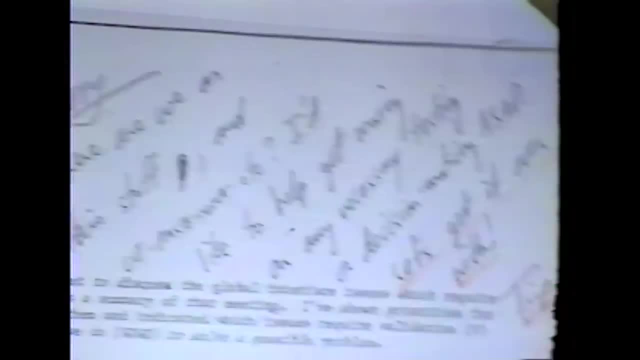 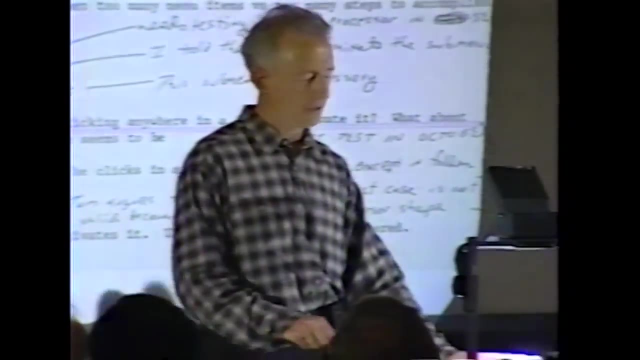 He says: aren't we done with all these decisions yet? Let's get on with it. Why are we still talking? Okay, But here are some of the issues. Should the arrows point apart, away from each other or towards each other? 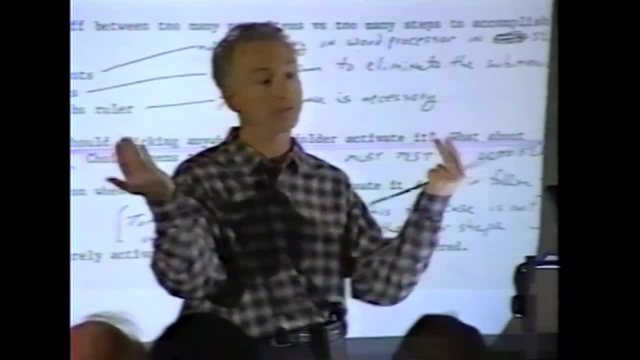 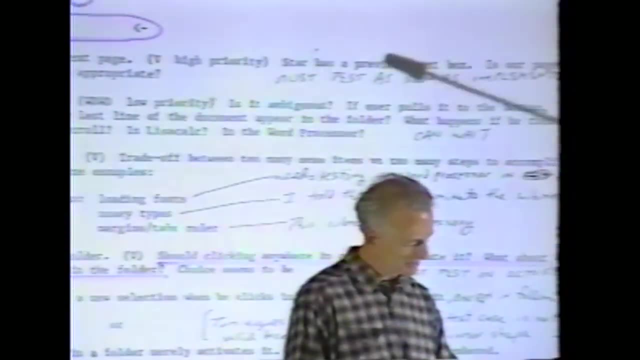 Because, after all, the text moves in the direction that's opposite to the arrow direction. We could flip the arrows and make them point to each other, And I wrote a comment here. We can wait until September to test this. No hurry. I wasn't in sync with product marketing, who wanted all the decisions to be made. 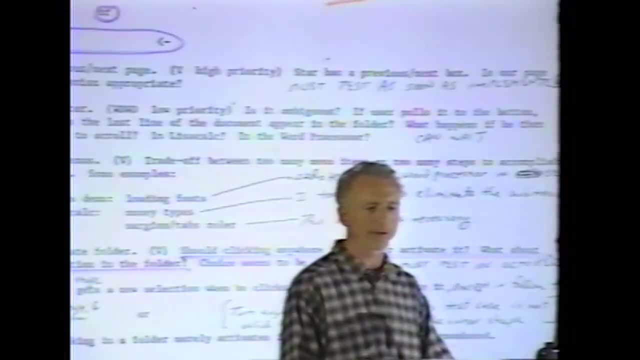 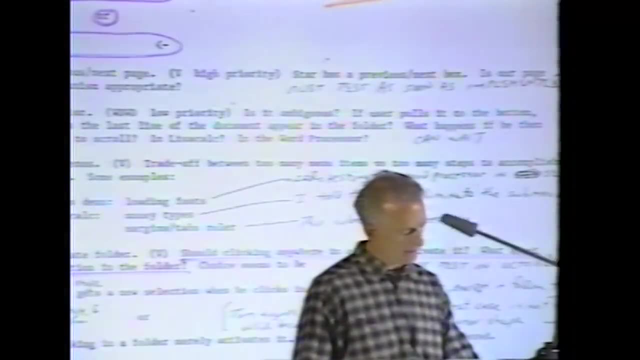 Because I knew that changing this was a matter of, you know, about three minutes of programming, So what was the hurry? I'd rather work on harder issues, like you know: getting the software to fit in memory or something, And there were some questions about clicking in folder. 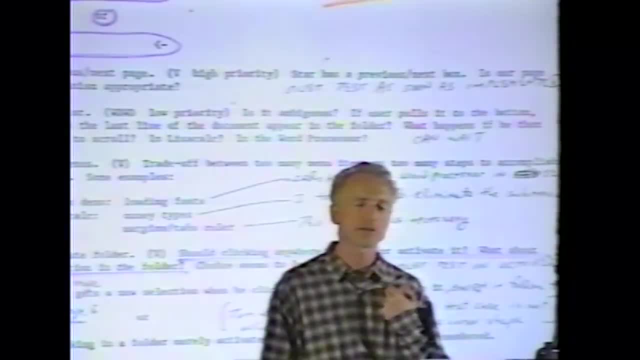 Oh, by the way, the word folder when you see folder here we used to call Windows folders. I forgot to mention that earlier. It might have been confusing. here Every window was a folder, Even a document window was a folder. 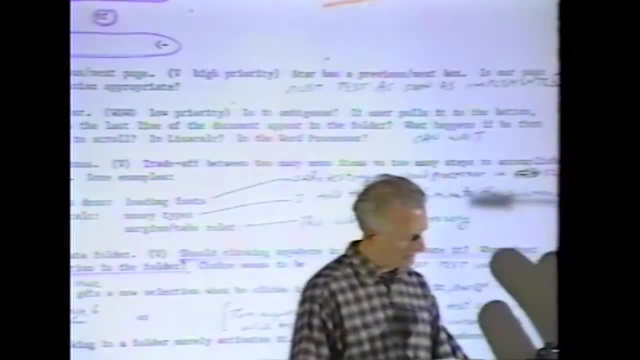 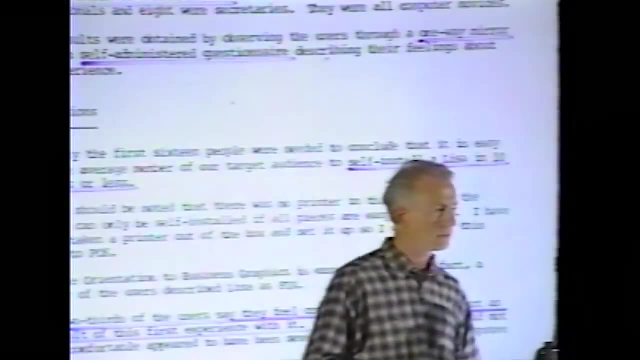 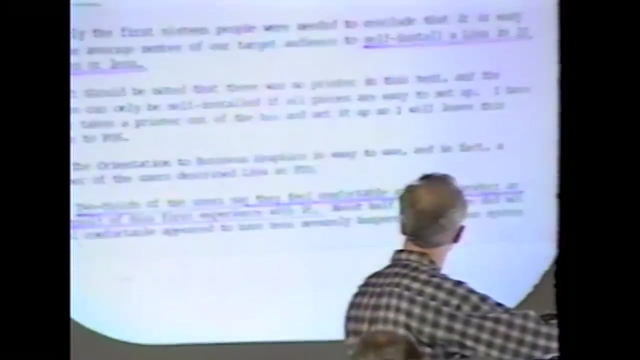 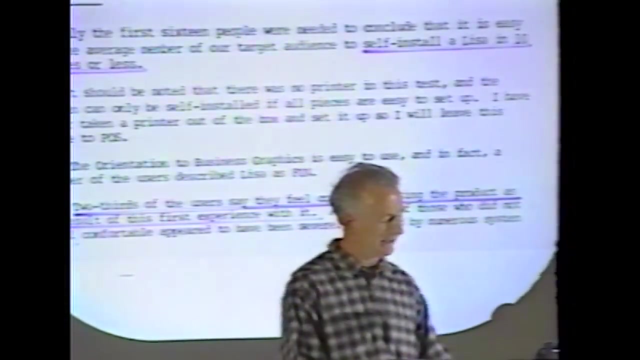 Not just the ones on the desktop, And we wanted to test, we wanted to do some tests on that, The whole thing. The mirror, Thanks, Okay, What was that? Okay? October 81., October 81,. we took the Chris's advice to heart, Chris Durer's advice. 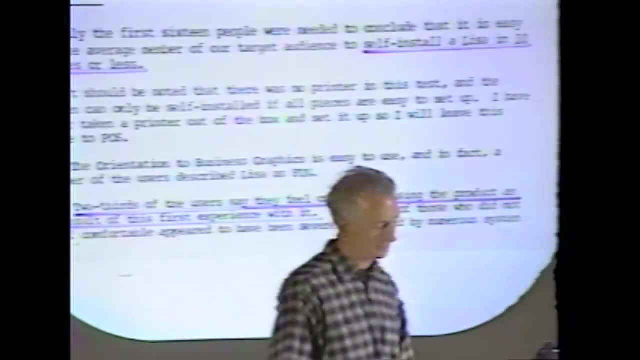 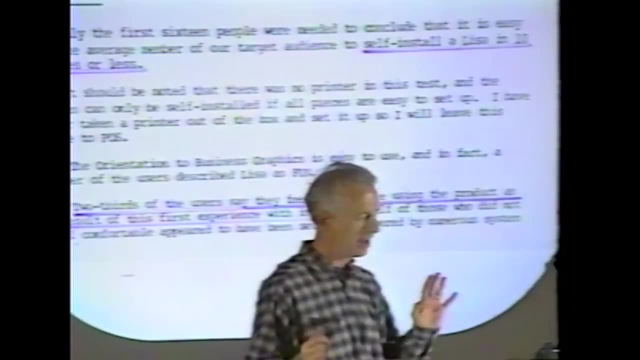 And we did outside testing. Twenty-four people who did not work for Apple were done in a one-way mirror room in Daly City. They didn't know what company it was that was showing it. You know, blind test. The psychologists had their day. 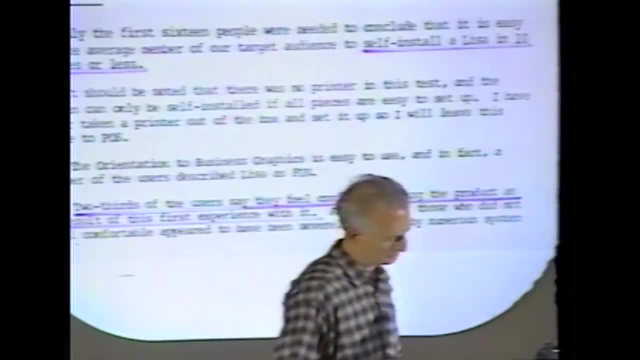 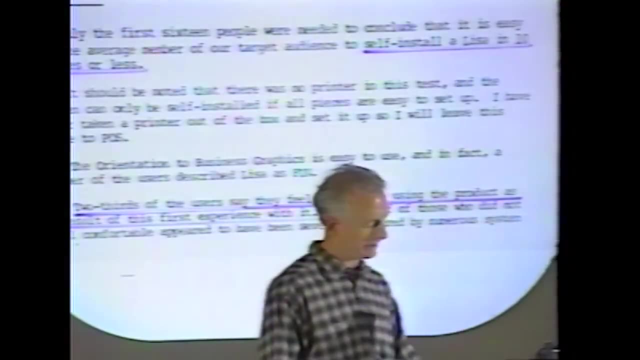 We got to do this, you know right, And this was the thing that there was no way we were ever going to do this. Too expensive Takes too much time, But at this point product marketing was going well. maybe we better test this on real people. 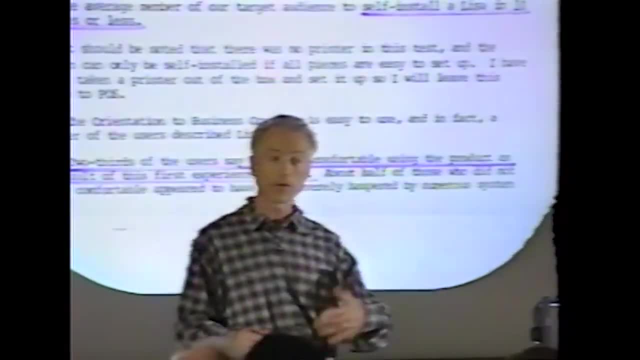 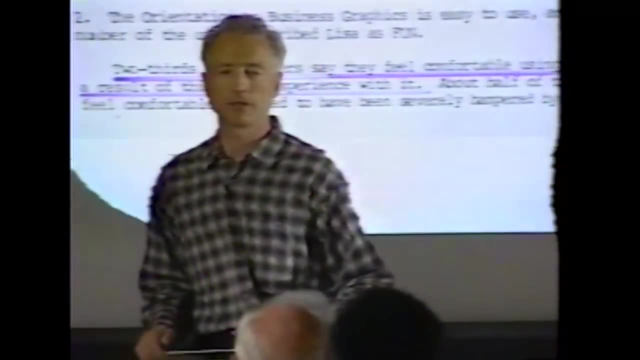 And we wanted to know whether they could read the manual and install the hardware and get the thing running. And they did it by themselves And it turned out that it was ten minutes on average that a person could, from the time they opened the box to the time they could get set up and running something. 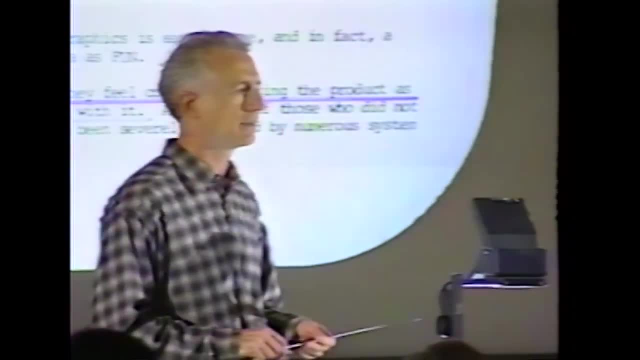 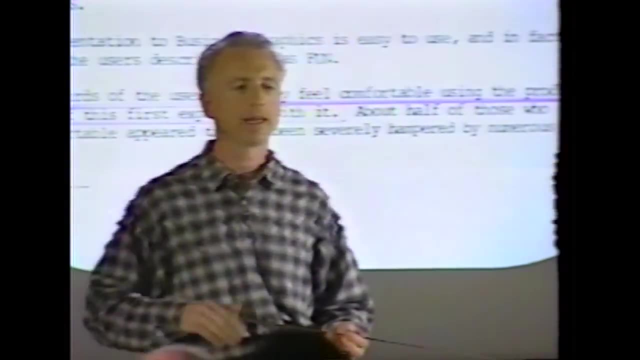 And we thought that was pretty good. Those of you who were at Apple later know that on the Mac it was even easier at the beginning. But as the Mac got more and more developed, that number went up, And when that number started getting about an hour, Jean-Louis Gasset got extremely upset. 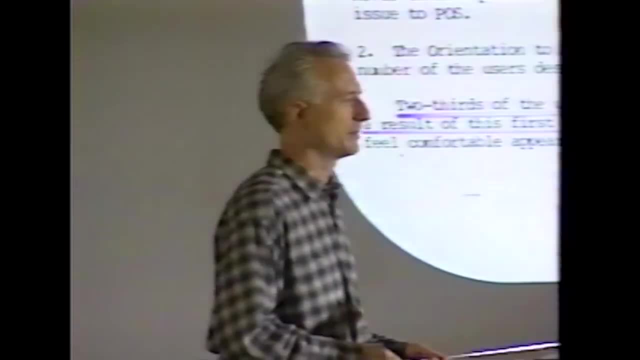 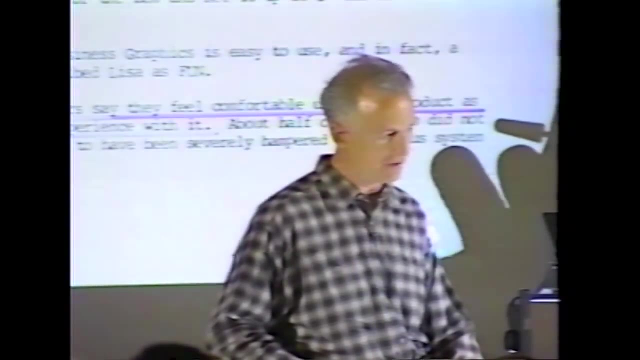 And he ordered new user tests And they ran user tests about that and got the time back down to ten minutes again. But there were some bad years in there. It was very hard to open a Mac box and figure out how to set it up. 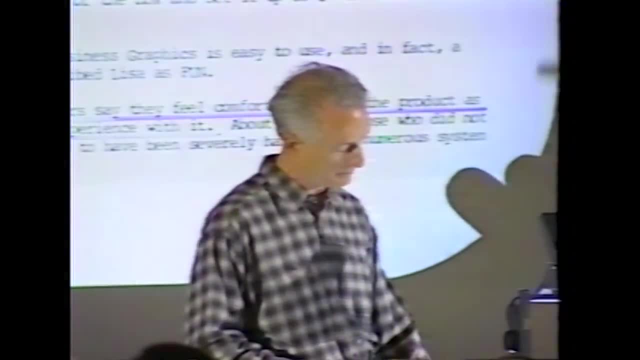 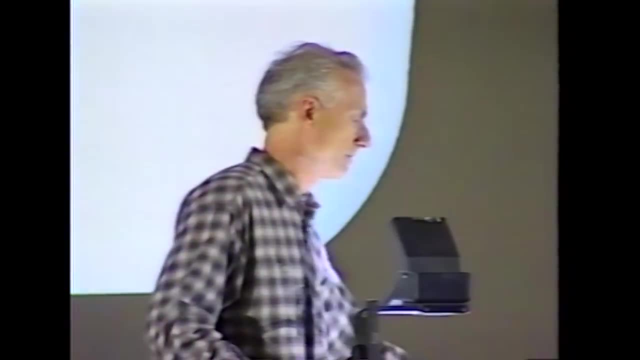 Two-thirds of the users say they felt comfortable using the product as a result of the first experience, And about half of the people who were half of the third that were uncomfortable were people who happened to run into crashes and so on, Which probably affected their trying to beat the clock on setting up the system. 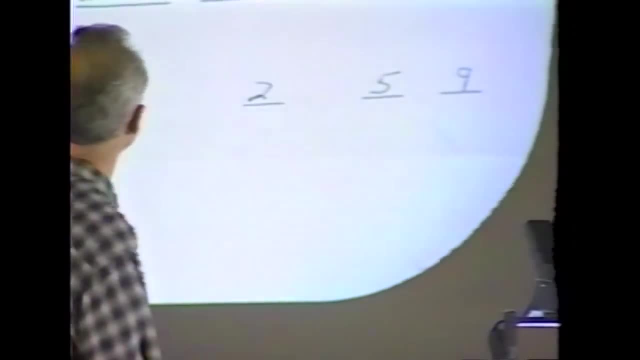 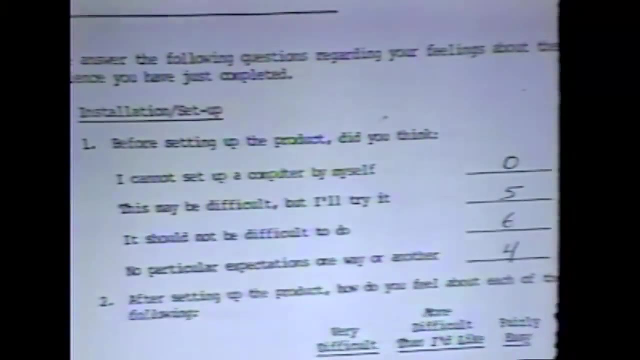 It's kind of frustrating And we had a questionnaire they had to fill out. This is the result of the questionnaire, So those numbers are how many people have that answer? And they didn't think it would be that difficult to set up Before they started. 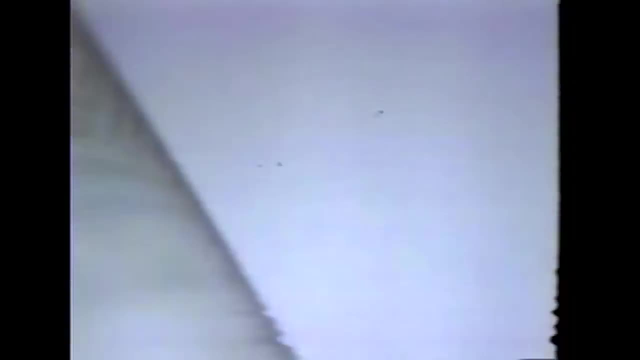 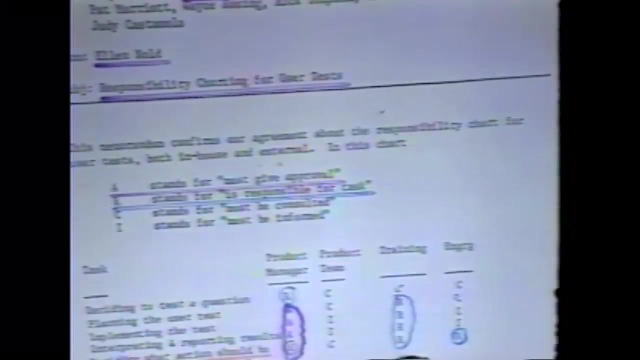 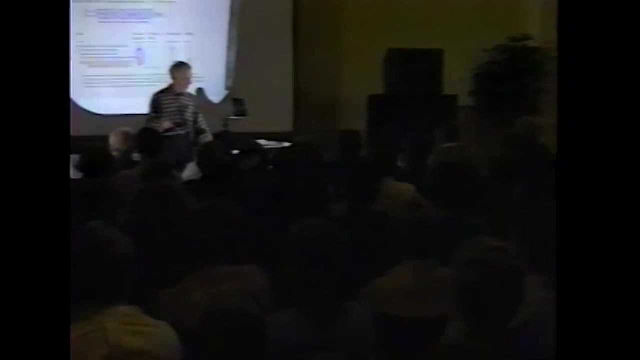 But then after they did it they found that it was very easy. Alright, now it's still 1981.. Now I should mention that the Xerox Star was announced at NCC or something- National Computer Conference, I think- in June of 81.. 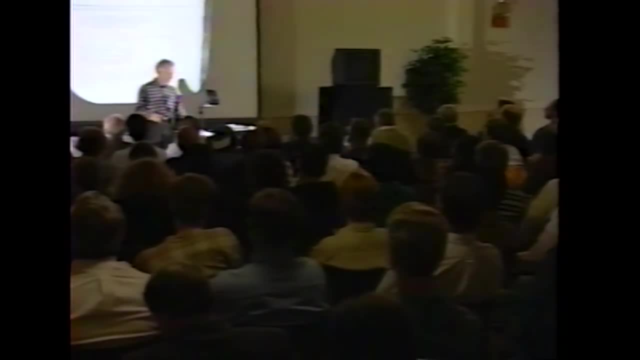 And some Lisa people flew out there, Got a look at it. Bill Atkinson went, I believe, And Steve Jobs went, Or maybe he sent Bill and didn't go himself, I can't remember. At this point we had a guy named Greg Steichleder who had joined the group. 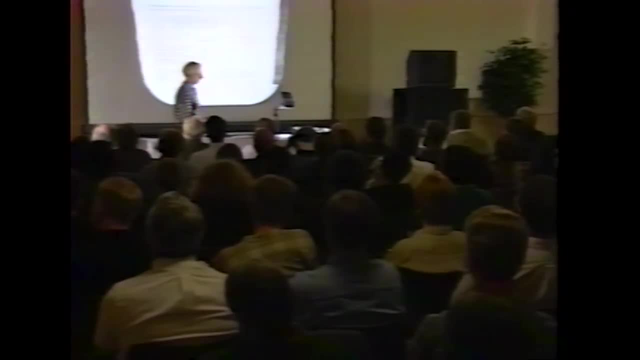 Working for Ellen Nold in the training. Lisa Training- Some of you may know Greg because he's more recently been an entrepreneur- Sold a couple of companies And Ellen is sending a memo to various people copying Greg On responsibility charting for user tests. 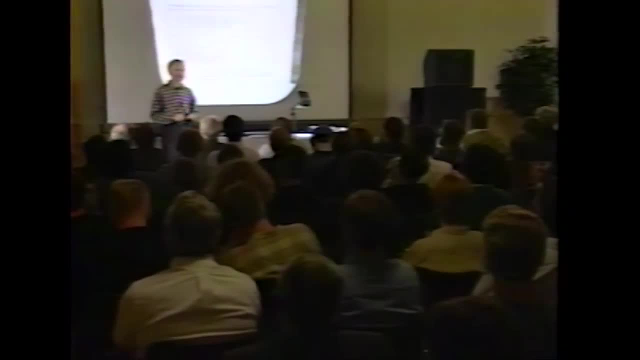 Now that user interface council we talked about before, with the majority vote. I don't know if they ever even had one meeting. We kind of overwhelmed them somehow, And by this time, a few months later, we had to have a new process. So the new process was that, based on some lecture we all went to by some management consultant, 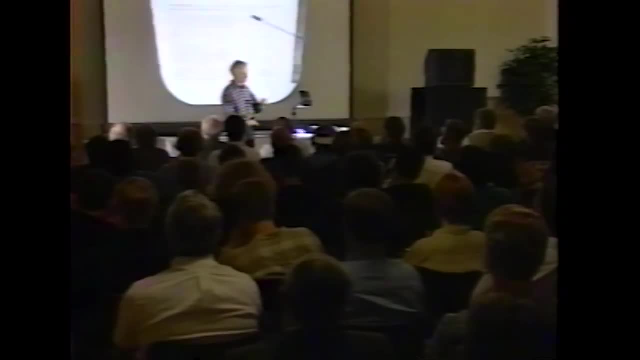 We were going to have people with authority, People with responsibility, People who were consulted, People who were informed And basically, product management had all the authority, since Ellen worked for them, And engineering and training, which is Ellen's group, had all the responsibility. 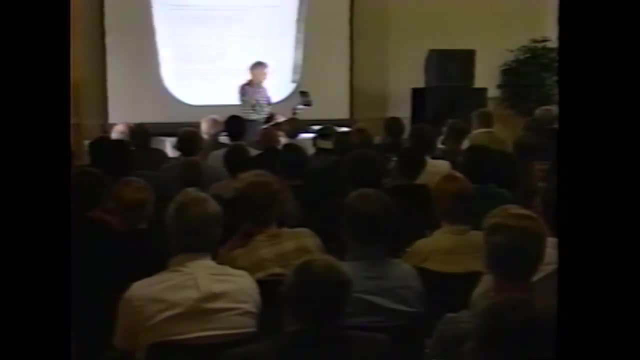 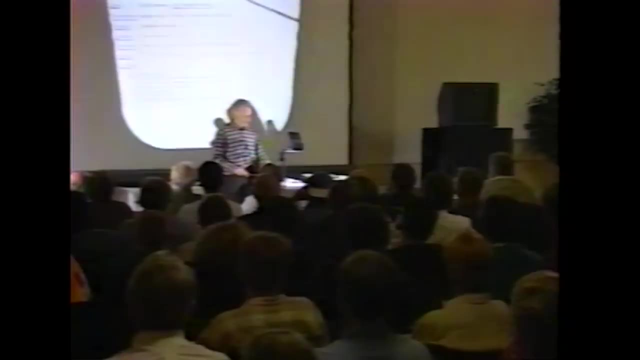 So we did all the work, And then product management would bless it and say that February 1982.. A year and a half has gone by. Engineering user test. This is a sample test. This is a write up of a test. 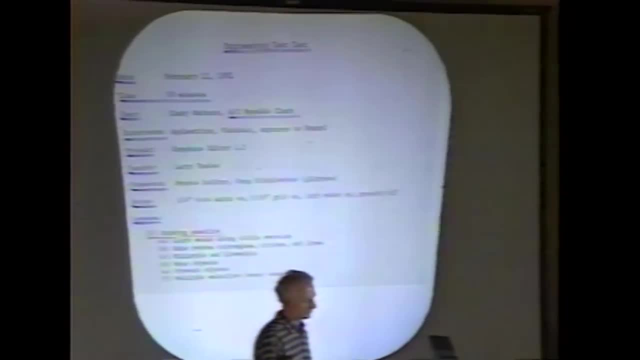 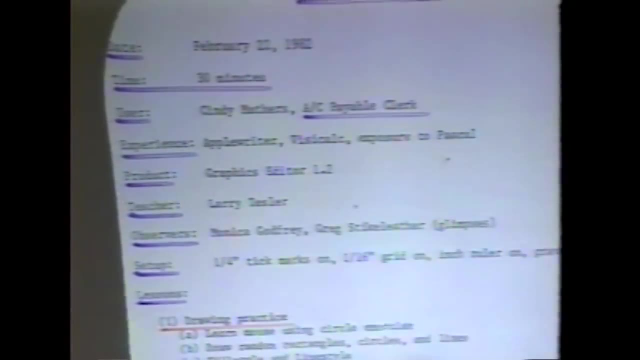 We had a standard form to write them up in. Now we're getting real formal here, Not just run it to Steve Jobs after the test and tell him what happened. We were writing, You know, formal reports, What the person did, How they did. 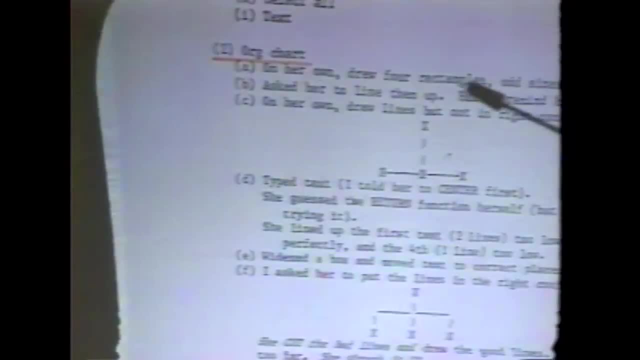 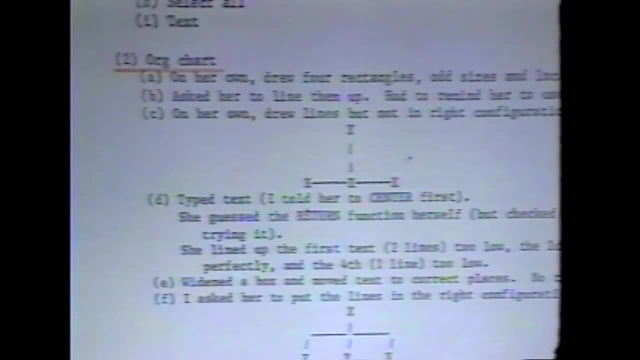 I'll skip over a little bit of this. Oh well, The person had to draw an org chart And here, not having a graphics program myself that had printing working, yet, I was doing it in the word processor and drawing little org charts here. 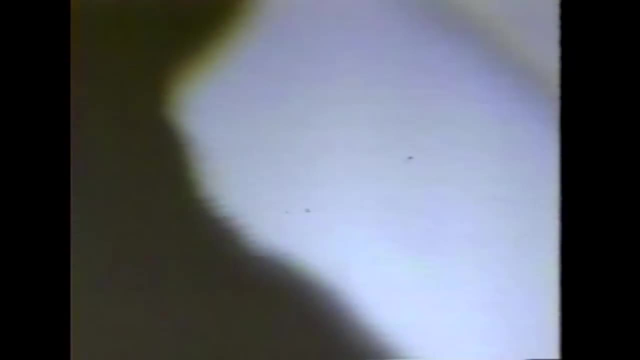 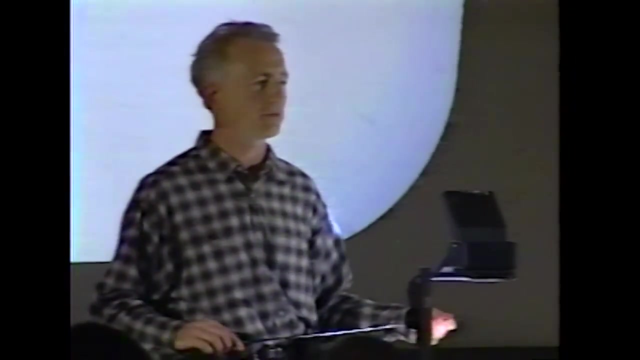 But they were really doing it with a drawing program And, by the way, the thing that won over the product marketing people was when we gave them the drawing program. It was the first one to get working. I had Mark Cutter just try to get it really reliable. 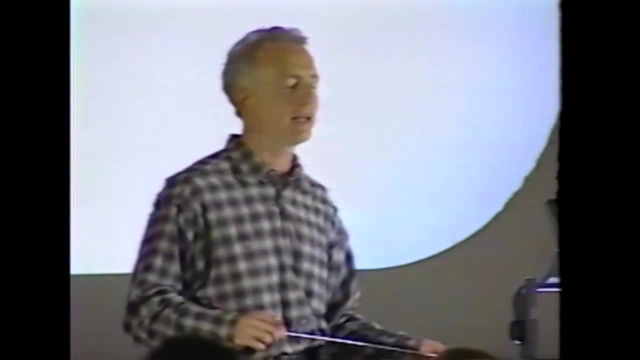 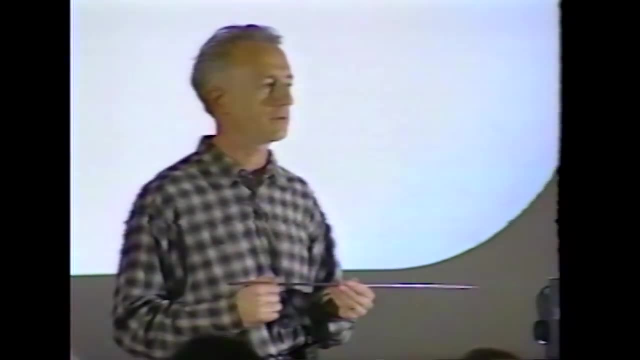 And don't worry about too many features. And then we gave all the product marketing people a Lisa, Some temporary operating system and the drawing program. That's it. It was a single tasking operating system at that time And they all started using it to make foils. 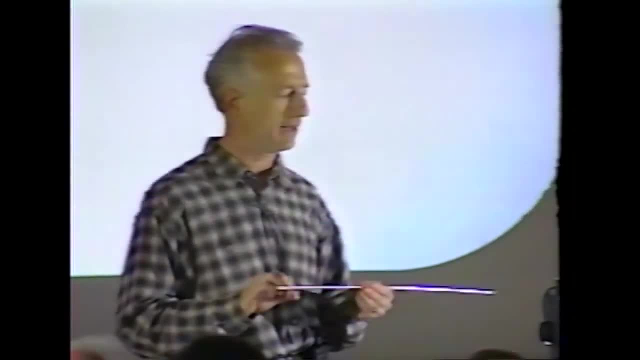 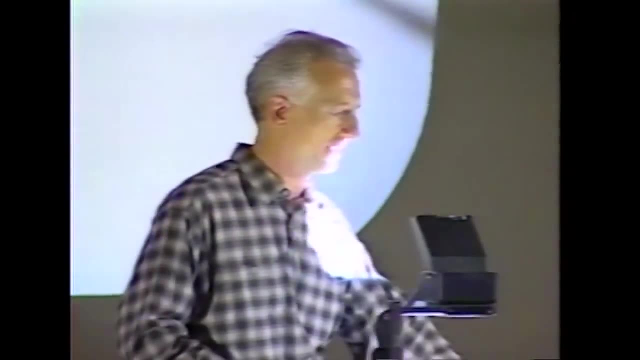 You could do text, You could do boxes, you know, And they all did foils And they fell in love with the Lisa And they even started to understand the Lisa And gradually the complaints started dying down And they started trusting, like maybe we knew what we were talking about. 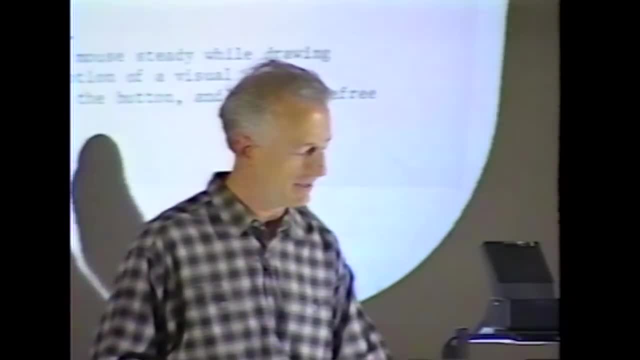 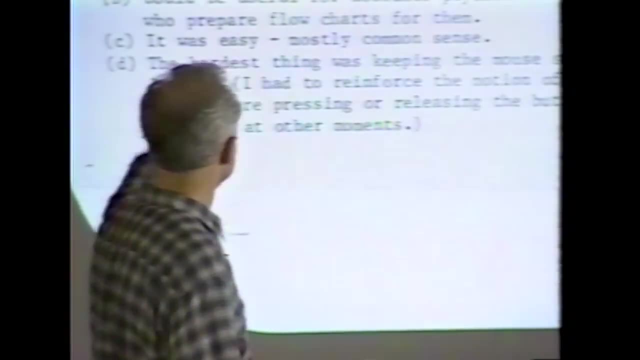 So that was a very good political move And I always make sure Mark gets it And I always make sure Mark gave him, you know, good, stable versions of the draw program. They draw a floor plan And then at the end they had comments to make. 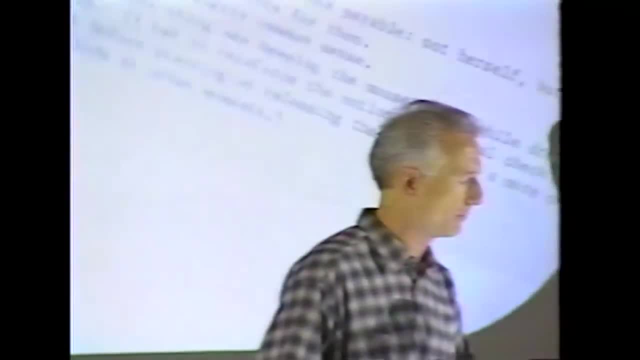 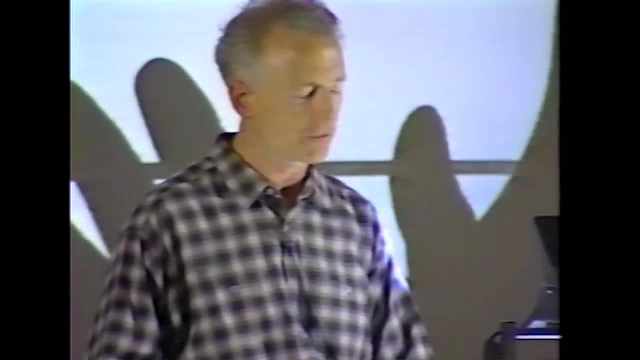 And you could see that the comments were summarized And people were basically really positive about this program. Sometimes there were complaints and we addressed them. Now, this particular test was, I guess, run by Greg Stike-Leather and me. He probably ran the test and I was in the room. 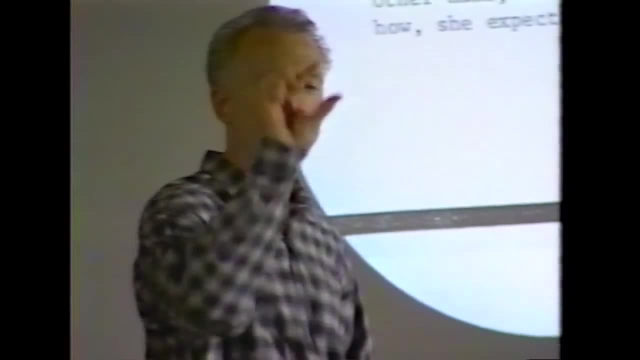 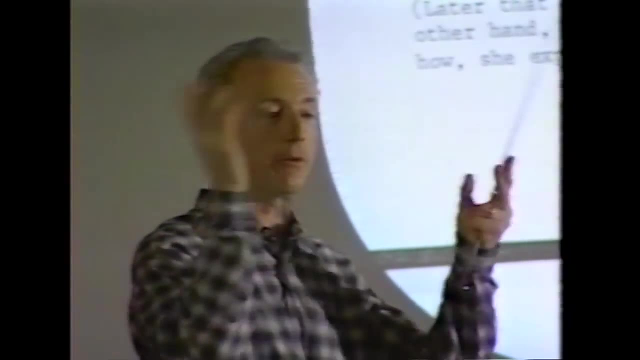 Or sometimes we switched off And he made a comment, which was that I-beam, which was the cursor that you use to select text, When the person would start typing. that little cursor was covering what they were typing, So he suggested that we get rid of it. 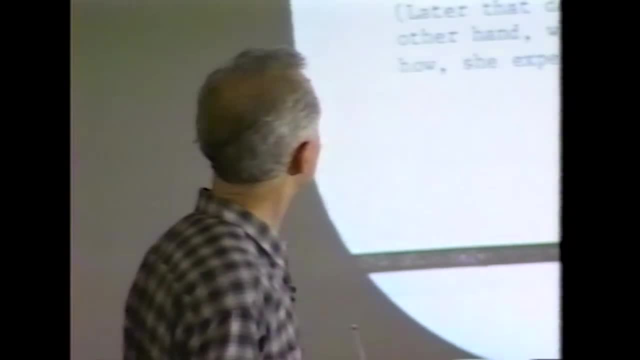 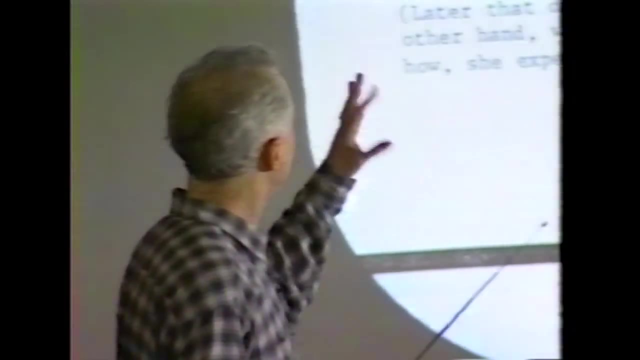 Well, there was no mechanism to get rid of it in the software, But he didn't know that, And so it was good that he was there and he suggested it, And we then implemented that, And I pointed out that the stretch handles were a problem. 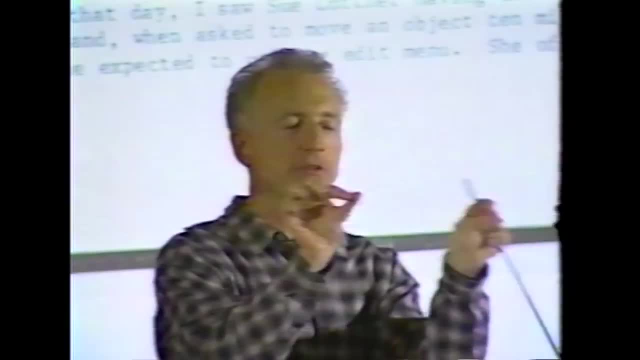 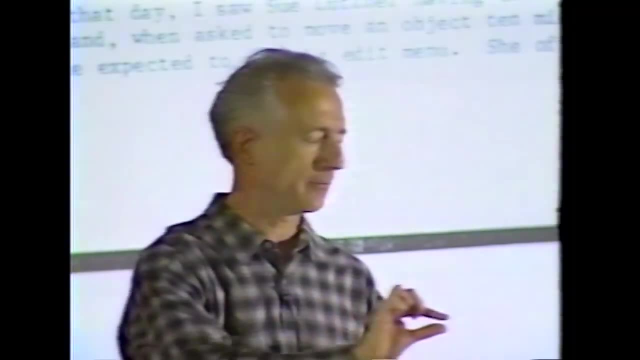 Initially, what Mark had done was he studded the outside of your object like every fourth pixel with a little handle. So big objects had, you know, beads all the way around the outside. It was like a necklace And this really confused the people. 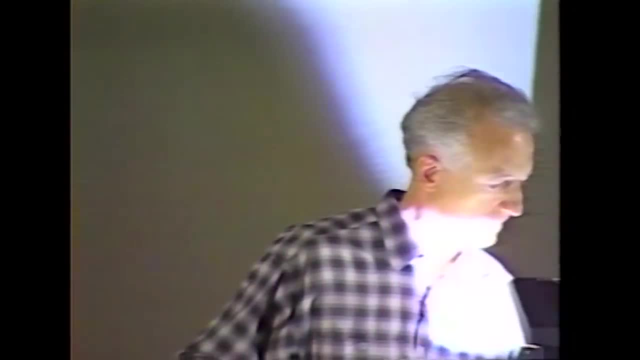 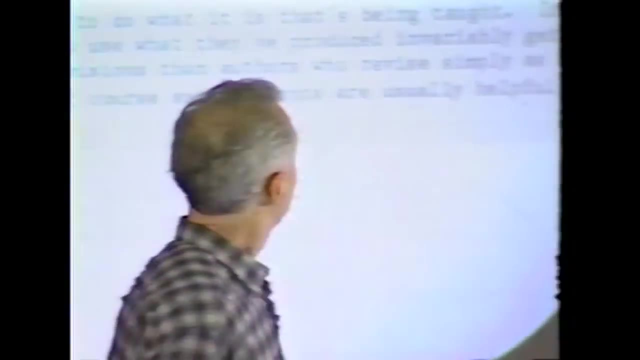 And I suggested we just have the four corners and the four sides and that's all. And that is the way it ended up. First I'm going to show you all the good comments. We had a lot of stupid suggestions too. And now, remember, we had user test guidelines before. 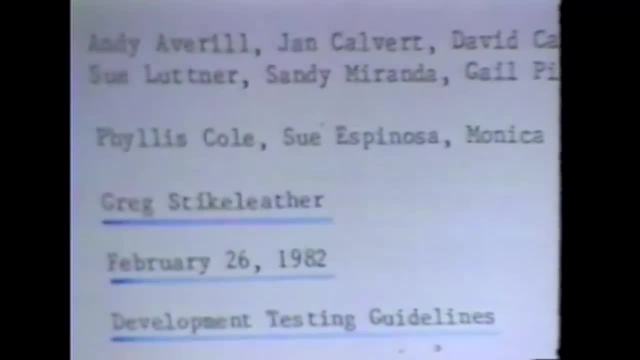 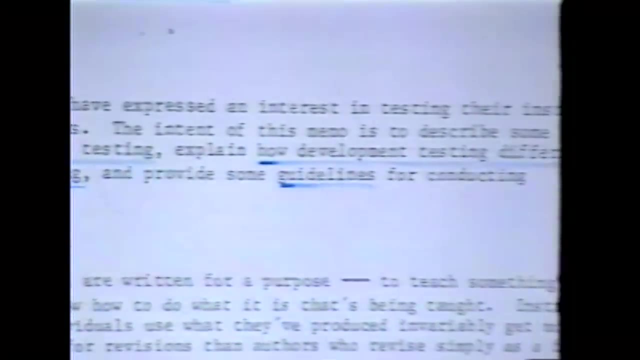 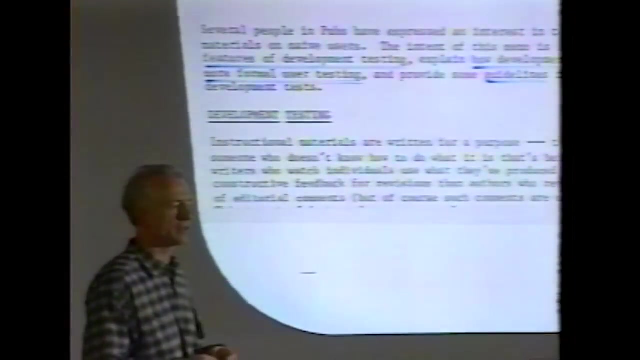 Greg wrote some new ones And here he was trying to address this to people who might have been used to formal user testing And had never experienced what he was calling development testing. And you know, things you test after the fact and things you test while you're still in development 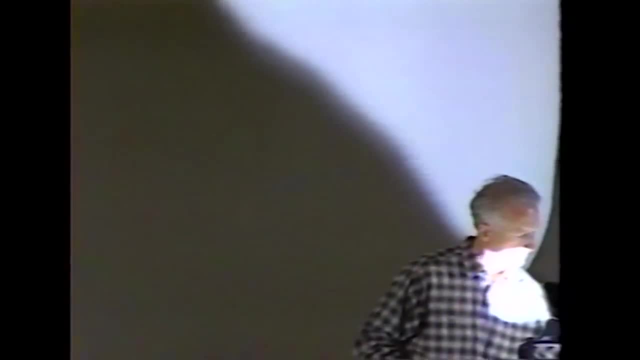 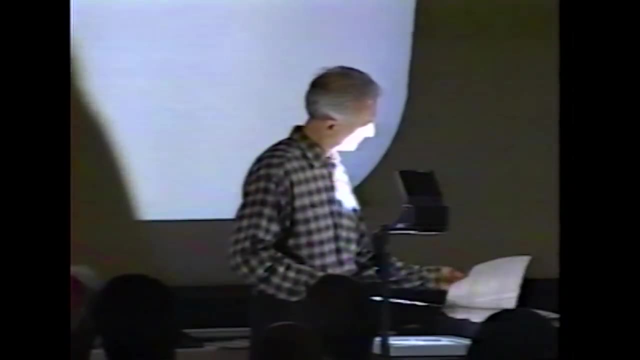 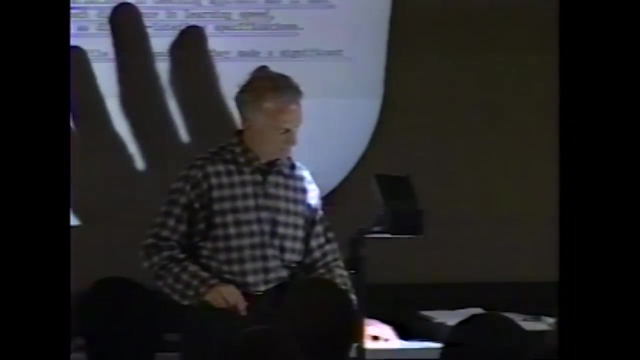 So he made some guidelines And they were interestingly a little different from mine, A different level, And I think I didn't bring them, Just the fact that he did. Okay, All right, getting near the end here, Excuse me, 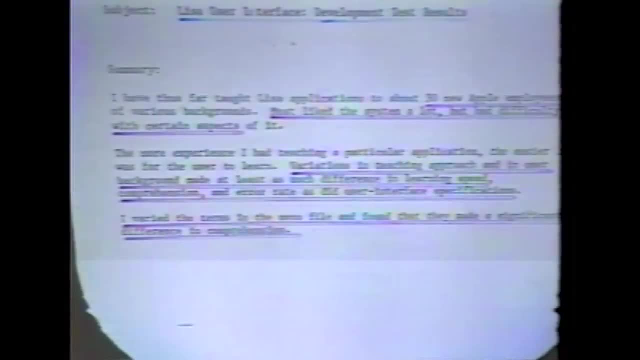 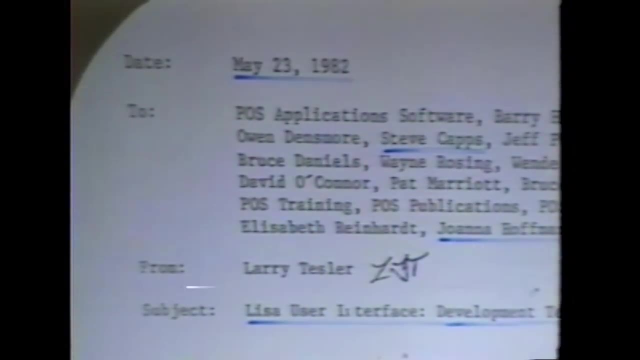 May 82. A little less than two years since I arrived, I had just finished some tests. So Greg said we should run development tests. So we did. We ran development tests And I taught 30 Apple employees over a period of several weeks. 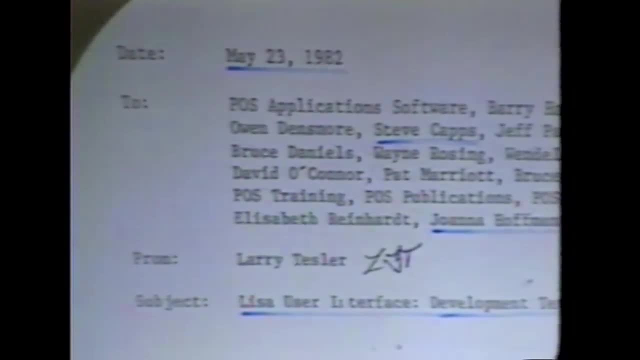 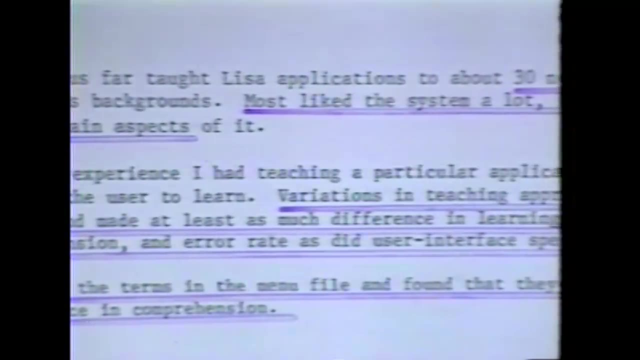 Several different applications To see whether you know we were on the right track, And by this time people were accepting this as a good approach, Because it was a lot better to be informed by a user test than to just see who talked the loudest in an argument. 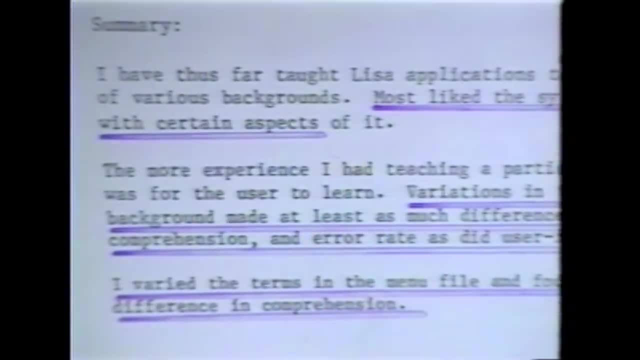 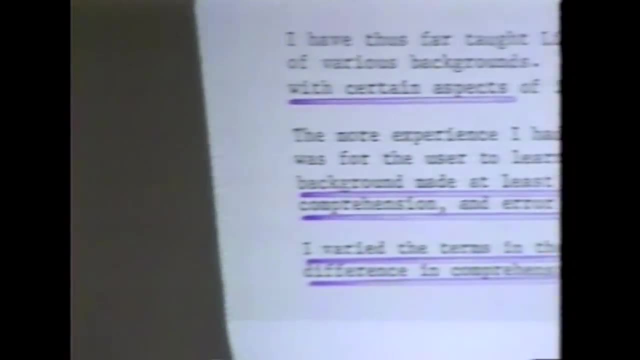 Or who had the most political clout, And what I found was that the way we taught it made a lot of difference. You could take the same user interface and teach it a different way And people would get real confused or understand it And or make more mistakes or fewer mistakes. 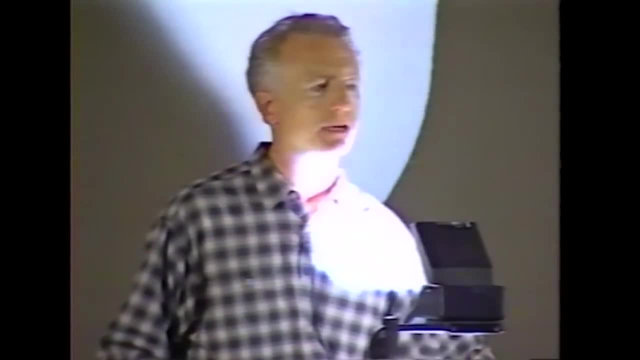 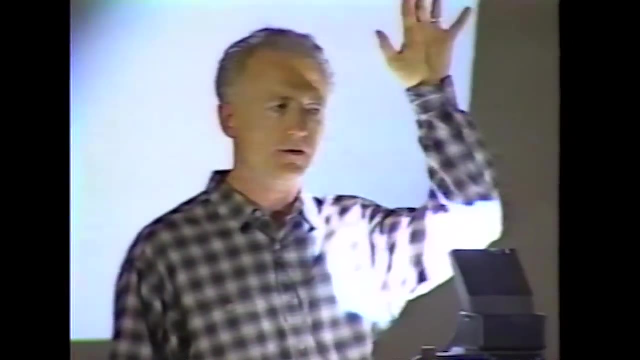 And terminology made a difference also. So we then started a terminology project that Ellen Nold ran, Which ended up- and I have many slides I didn't bring on that- And that ended up with the file menu, the edit menu, etc. 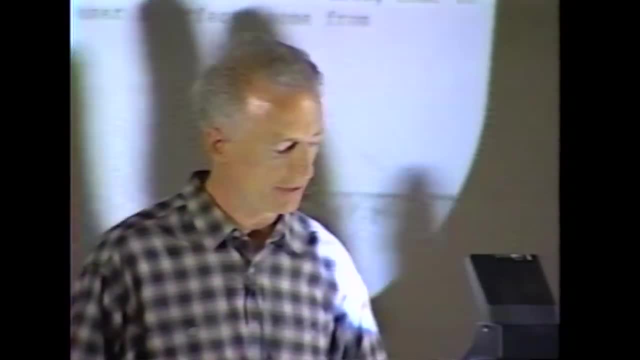 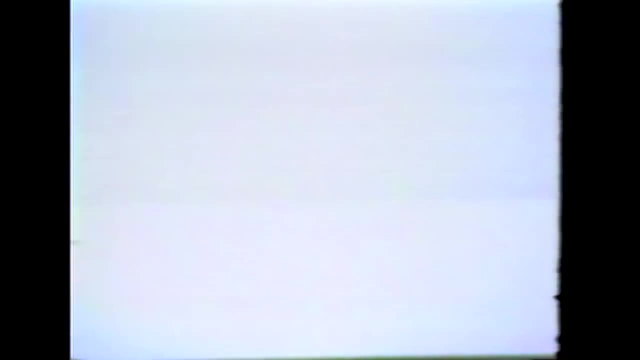 As you know today And the various commands that were in them- You know choosing all the words for everything- That have pretty much survived into the Mac. Let's say 95% of them survived into the Mac And most of them went into Windows also. 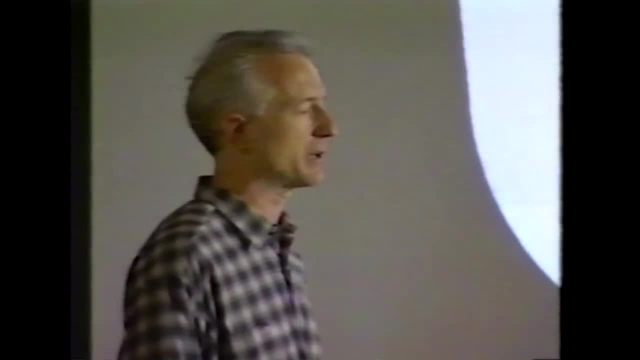 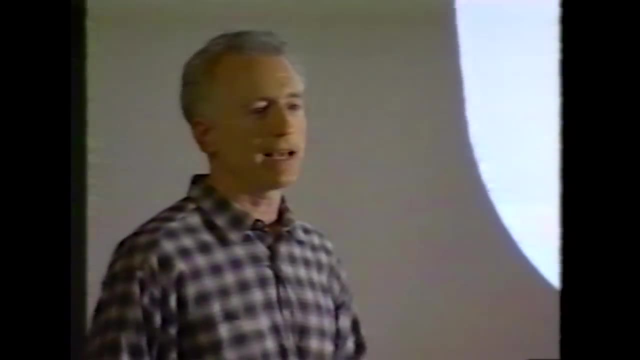 So that was a very healthy terminology exercise. We did a lot of testing and a lot of debating, A lot of linguistic analysis, And one thing I say here is that after all these tests I discovered a lot of things that could be better. 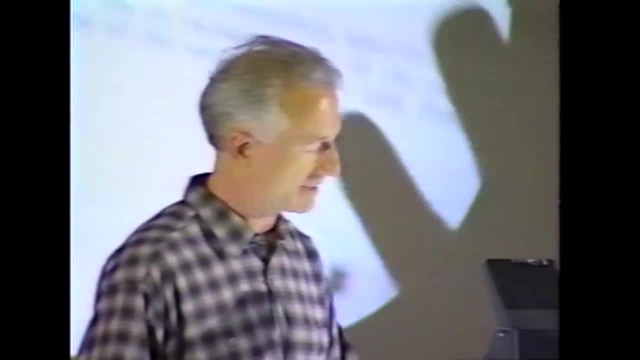 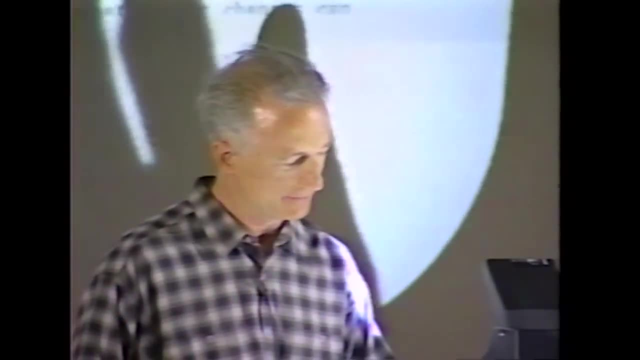 But we do have to ship a product, And it's been a long time since I've been at Park. We'll ship a product, But couldn't we fix these in the next release? Well, little did I know. There would only be one more release. 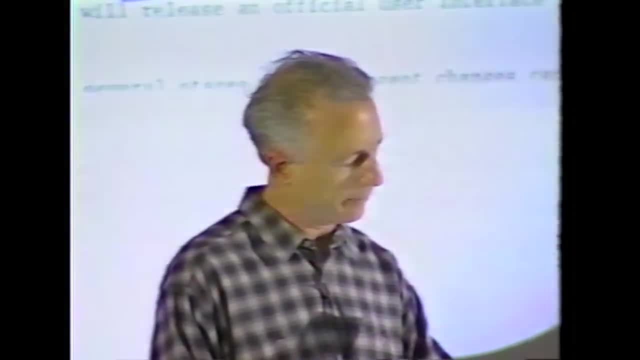 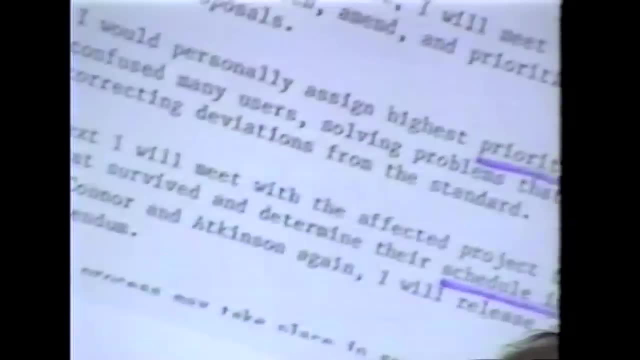 And then we had a process again Where we were going to be very careful about prioritizing all the user interface changes And measuring their schedule impact And being sure they were worth. it Didn't have to be zero necessarily, But it had to be worth the schedule impact. 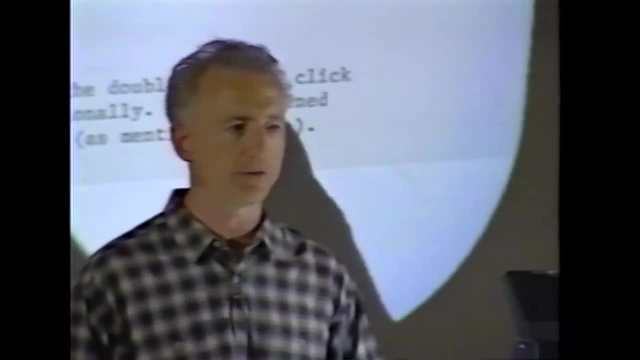 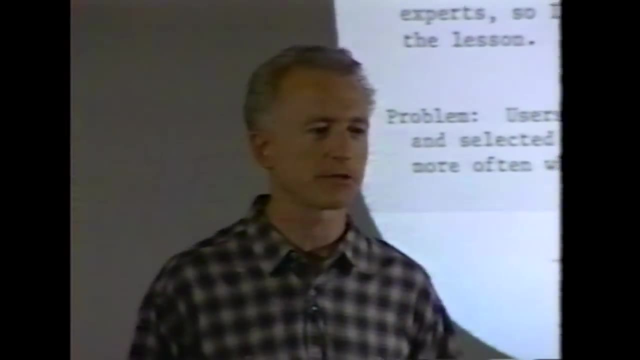 I think by this time people were really realizing That our only differentiation was ease of use, And it better be really easy. And then I went through some problems. This thing went on, by the way, for about 30 pages, So I'm just going to show you one page. 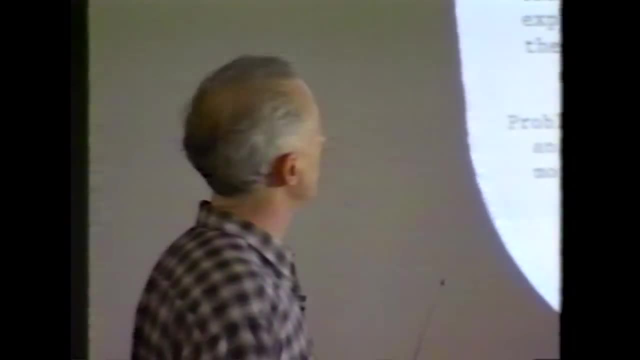 Cursor changes were not consistent And there were cursors changing shape everywhere. The I-beam wasn't the only one. Like no matter where you went in the window, You got a different cursor shape And I thought you know that's too many. 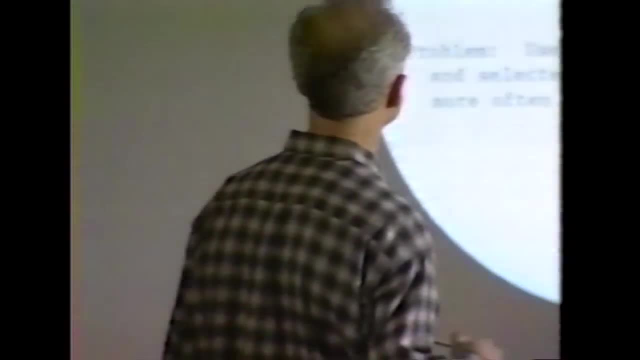 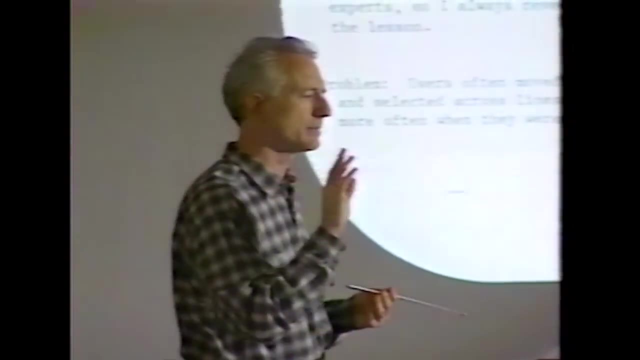 Let's simplify that. We had double and triple clicks at that time And some people it was the amount of time between the clicks mattered And you couldn't control it. So I suggested we add a preference item That people could control that time. 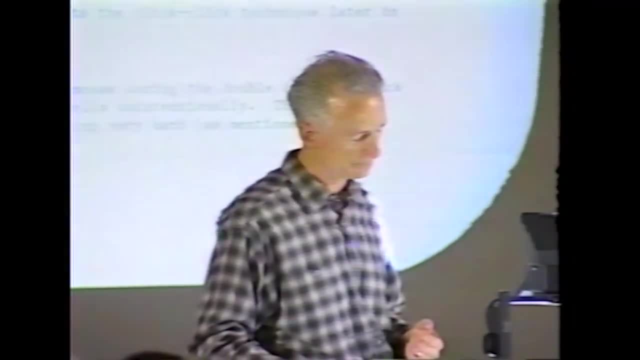 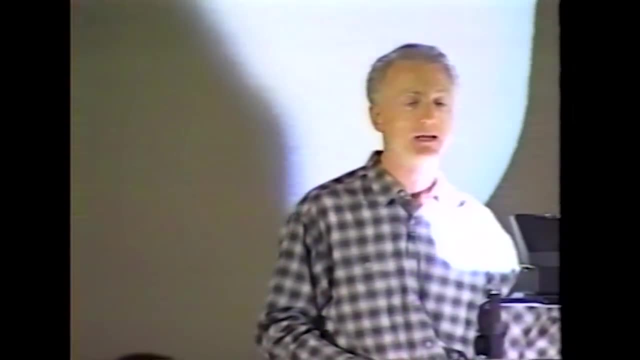 Which, of course, is what you do today In Apple's mouse control panel, And I also had some comments about how you teach it And in fact, when I looked at that whole memo, I'd say there were at least as many comments I made about how to teach it. 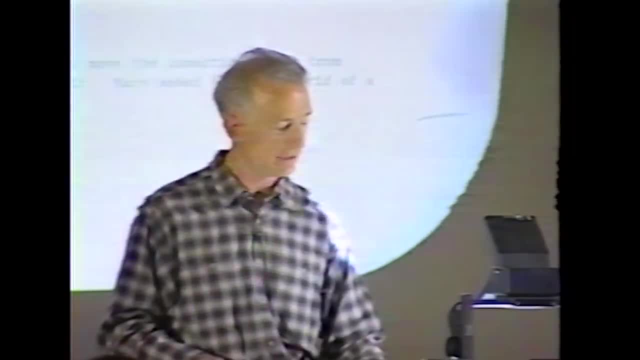 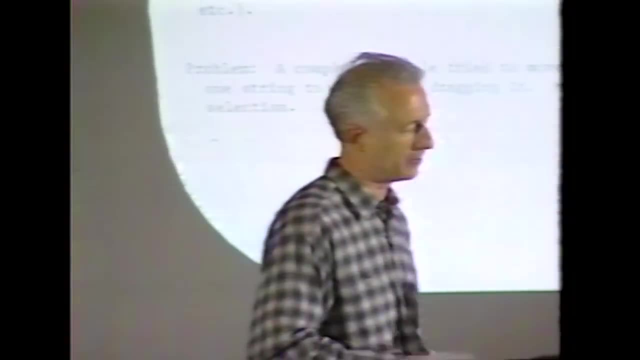 As to what it is, And then months earlier- I think it was One month earlier- Greg Stikeleather had pointed out That the I-beam should disappear when you type. I don't know if I forgot or whatever. 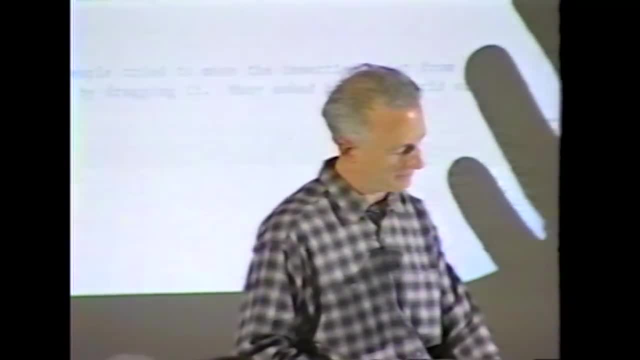 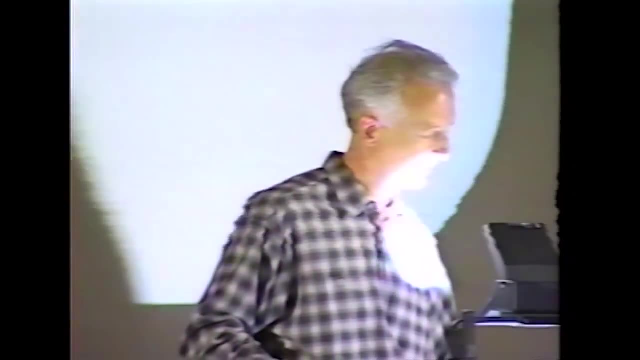 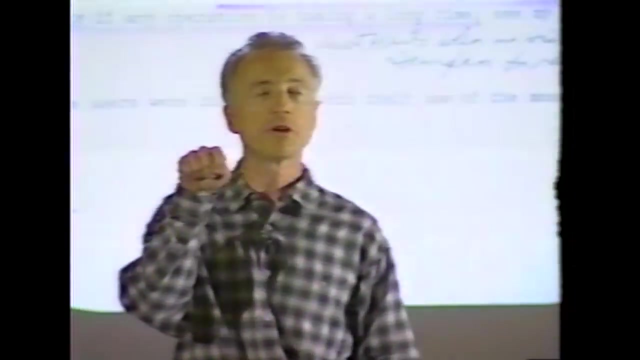 But I suggested the same thing again, Or observed it, And I proposed we hide the cursor, And here in the margin is something I wrote later Saying it has been implemented. If you're wondering about the cursor changing to a clock Or an hourglass, 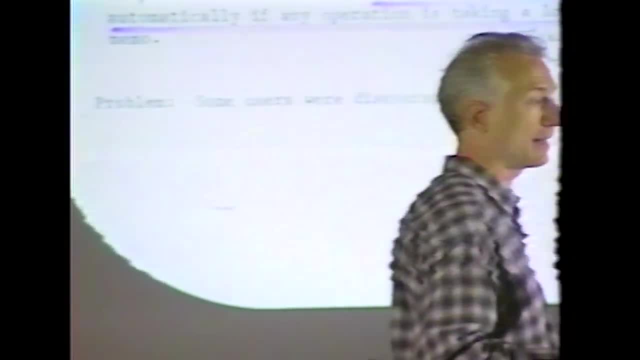 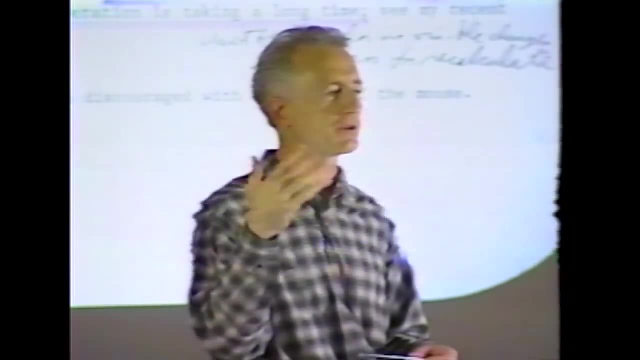 Various other things. That was something that was actually at Xerox. Xerox had that at Park And the thing was The way we did. it was We would wait a certain number of seconds And if the operation wasn't done, We would put up the hourglass. 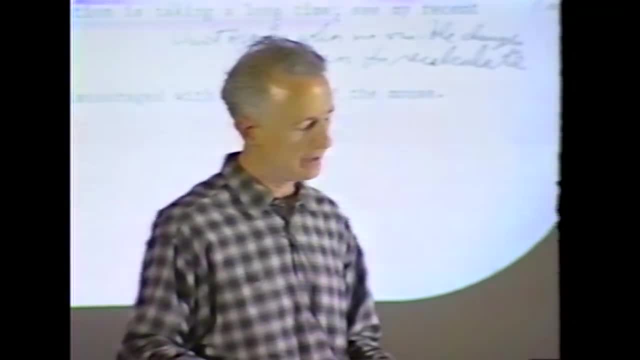 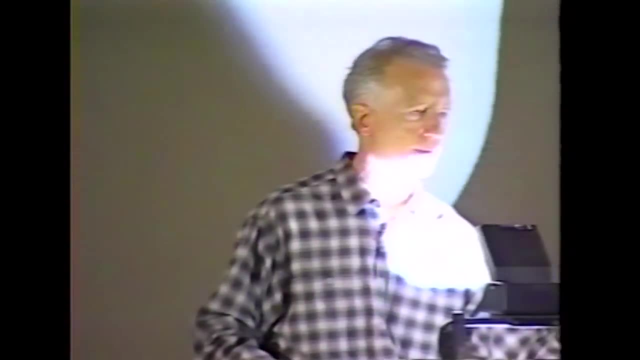 Trouble was, By that time The operation was probably done, So We, Or some of the applications, forgot to put it up at all. So we came up with some clever algorithm For having it come up automatically And disappear at the right time. 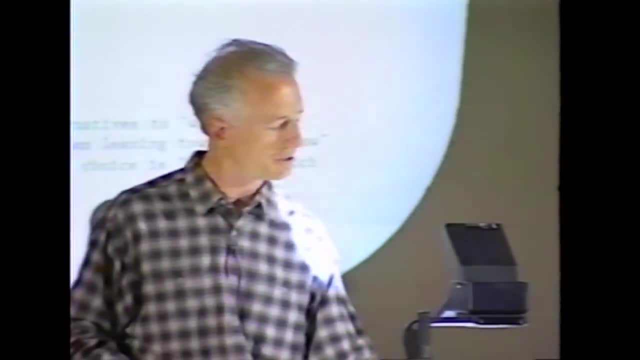 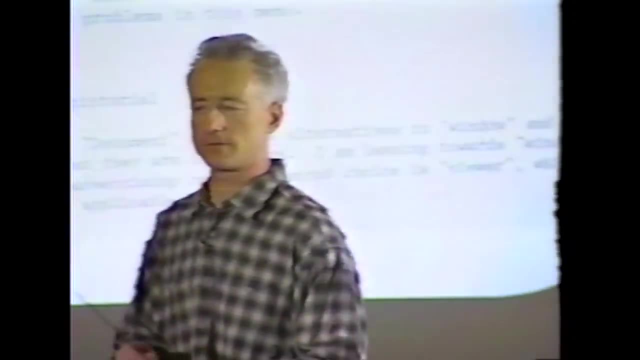 And all that sort of stuff. Now here's the big change. The star had come out a year earlier than this And we were all told by management And ourselves. Don't pay any attention to that. We were all told by the ship. 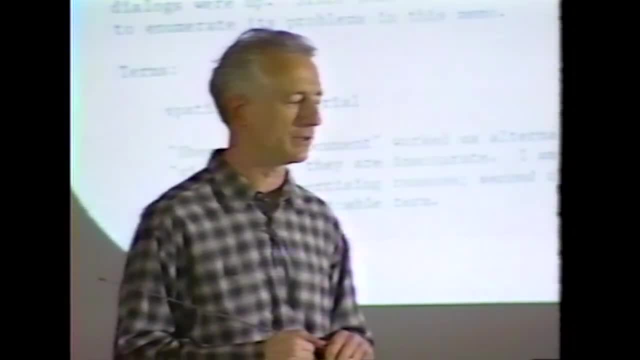 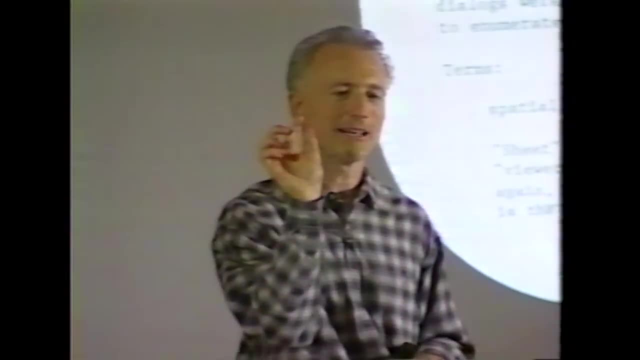 But in everybody's heart They kind of felt like: You know, Most of the lease is easier to use than the star, But there's one thing about the star That is really, really nice, Which is those Those little icons on the desktop. 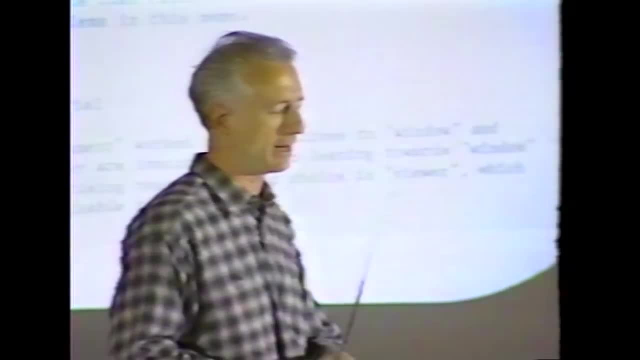 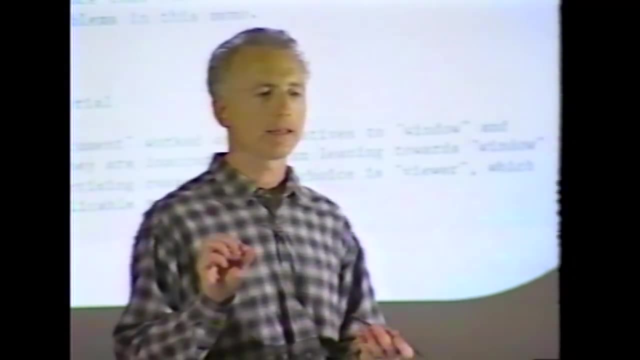 There was icon envy. That was very serious And we weren't allowed to work on it. But around March of that year Some of the guys got so troubled by it That they started working at home On weekends On an iconic filer. 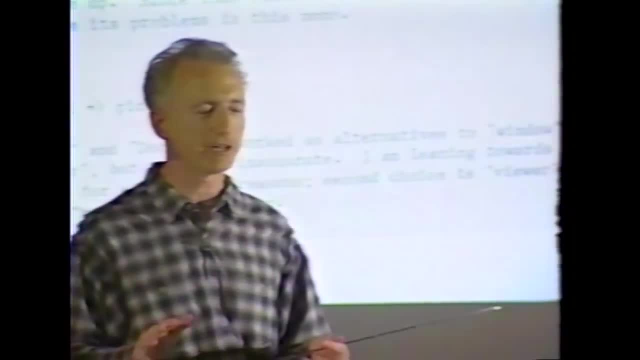 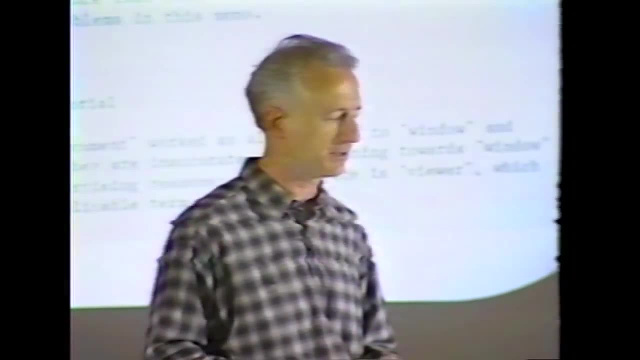 We called it And at first it was a big secret And they started letting people in on it A little bit at a time And finally Everybody found out about it And there was a major uproar That people would dare to make changes at this late stage. 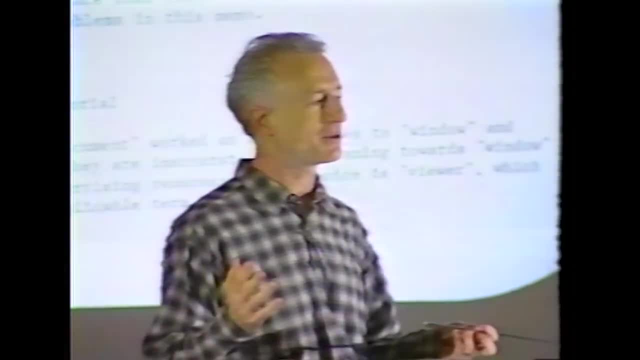 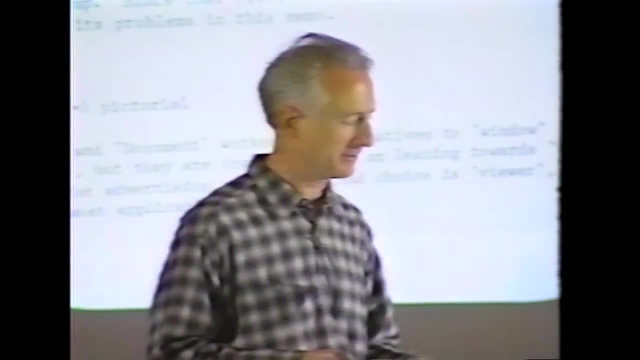 But they'd already implemented it And so you couldn't complain about the schedule impact And the person writing the manual Thought it was kind of a good idea. So she kept saying it wouldn't affect her schedule And So nobody knew what to do. 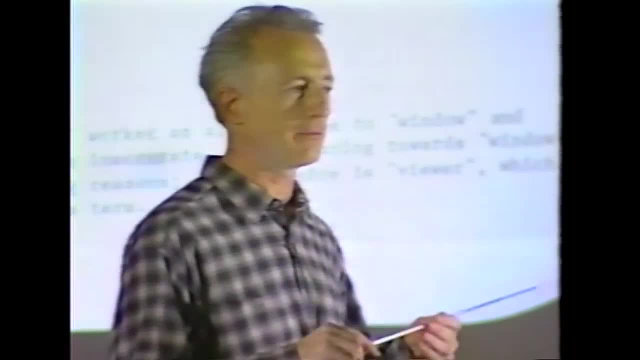 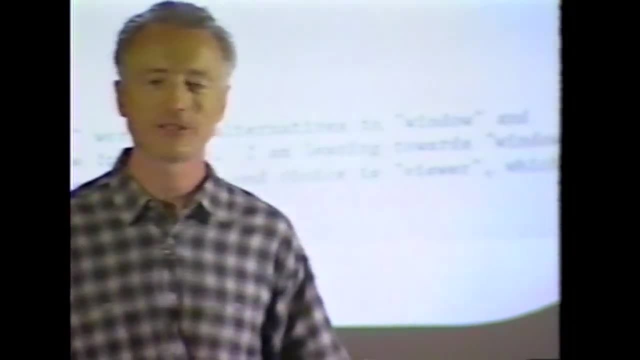 So I said So. I made a deal with Trip Hawkins And Wayne Rosing, Who was the engineering manager at that time. We'll run user tests And let the users decide. So I ran tests And you know what It turned out. 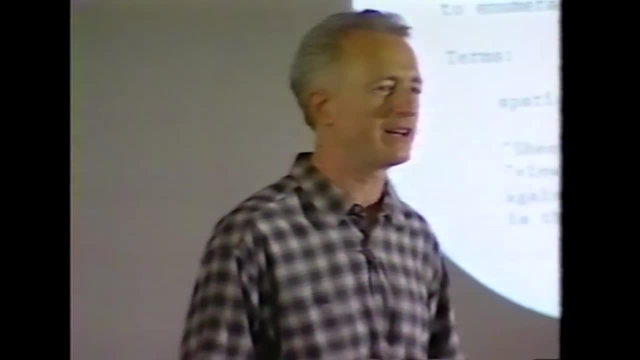 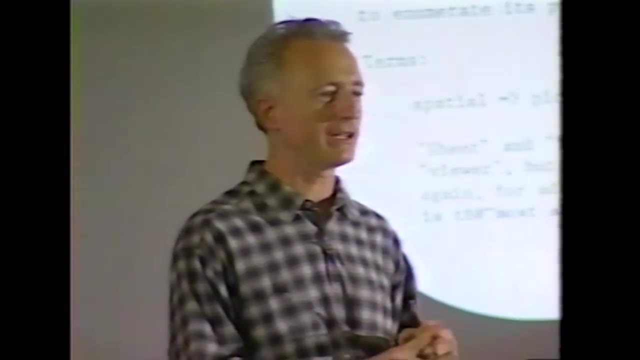 That the interface we have, Which I won't bother to show you, But it was kind of a More like find file- It's the closest thing I can think of- Was actually equally good In terms of ease of learning, Equally easy to use. 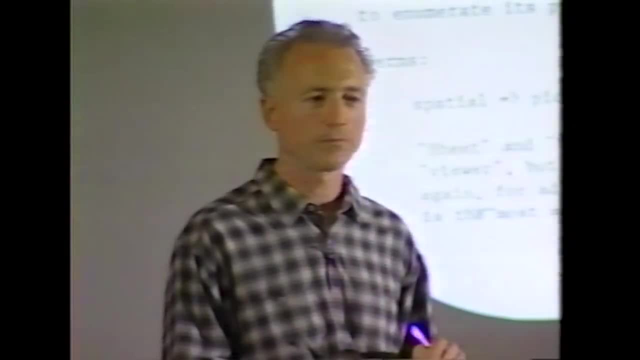 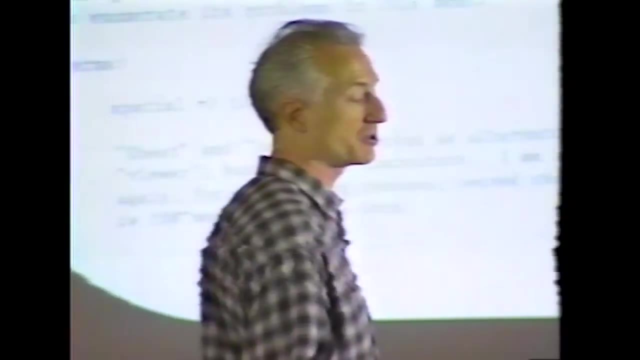 Same error rate, Very low. People understood both. There was no difference And we already had one. So why did we change? And the last question I asked her Everybody is: Which did you like better? And they all Like the picture one better. 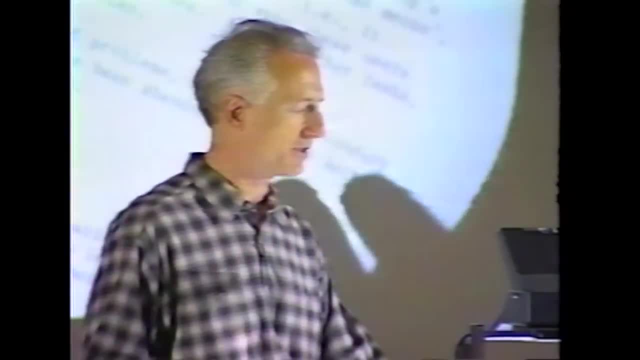 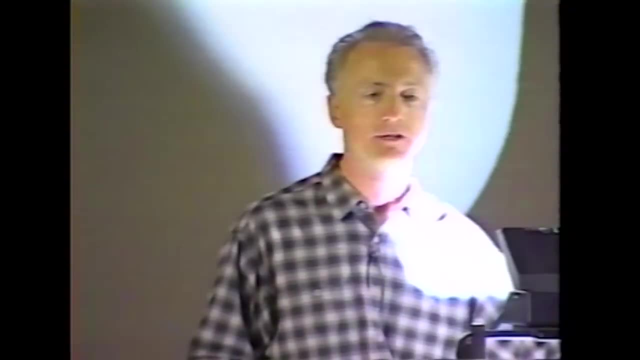 And so we made A decision That had nothing to be: Nothing to do With ease of use, Nothing to do With ease of learning, Nothing to do With error rate. It wasn't a human factors decision At all. 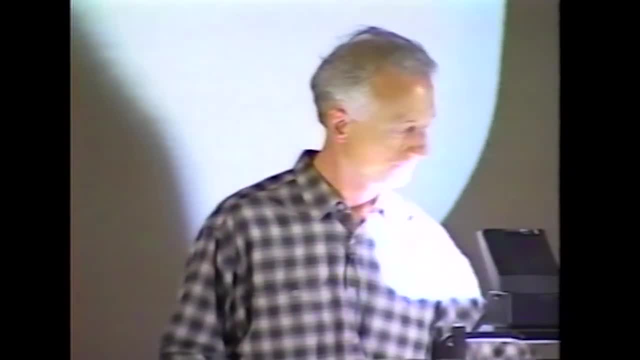 In the traditional sense It was a decision Based on what Customers liked, And there's a whole history I won't go into here About the icons. They didn't actually Come from the start. They came from some IBM did. 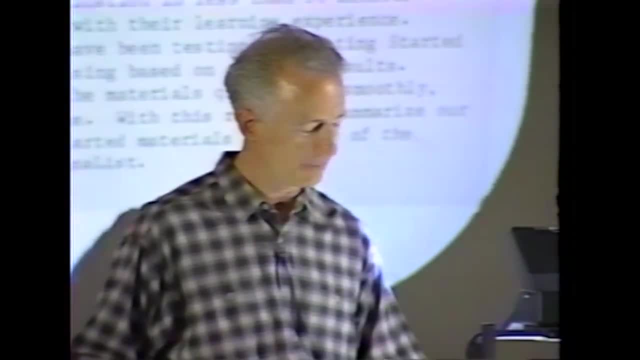 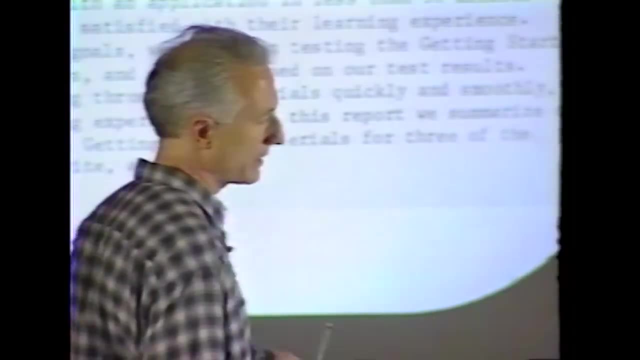 I'm not going to get into that Long story. You can read The proceedings Of Microsoft Versus Microsoft Lawsuit Or something To find that out. Okay, So This is my last Slide here, So 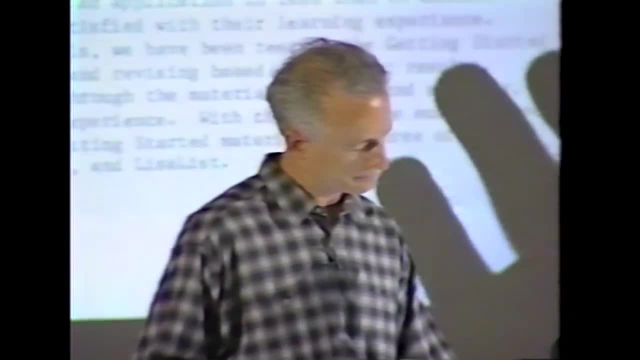 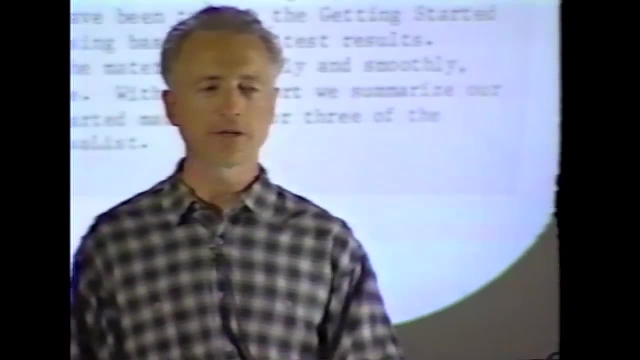 And This was a memo That included On it Chris Espinoza, Who was In the Macintosh Group At that time, And the Macintosh People Who had been doing A totally different User interface. 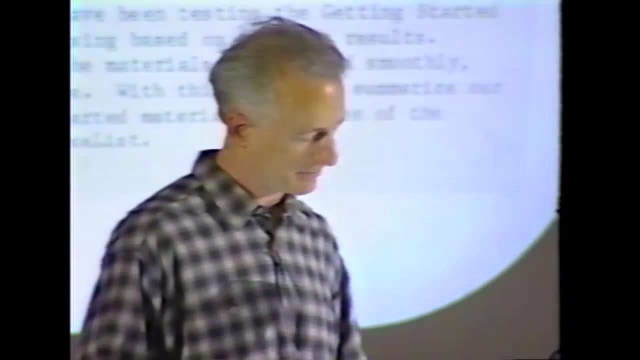 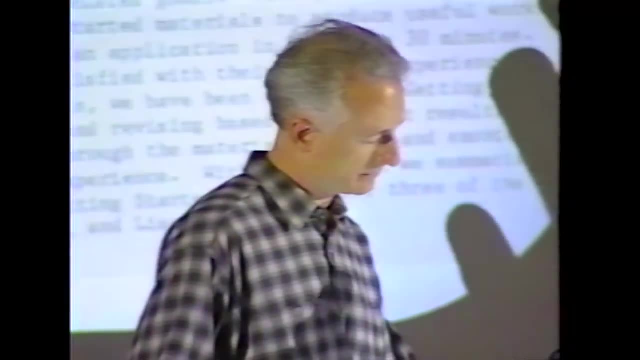 At some point Decided They really Ought to do Some subset To find their User interface. We started Copying The Mac People On it And With that September Eighty Two. 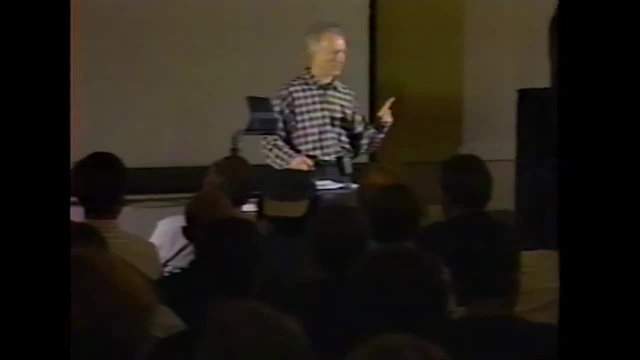 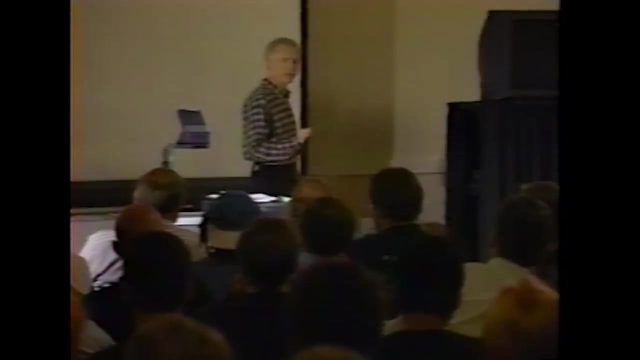 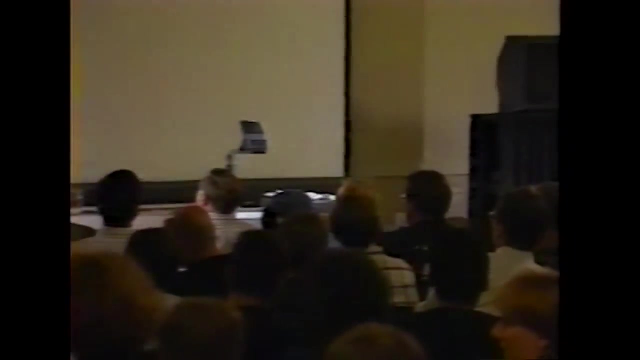 I'll Turn it Over To Chris. Yes, I Got Show The tape To Now. You Use One For Both. What I've Got Here Is Thirty Seconds. 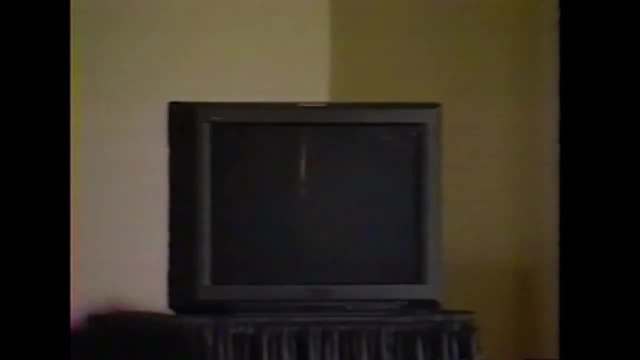 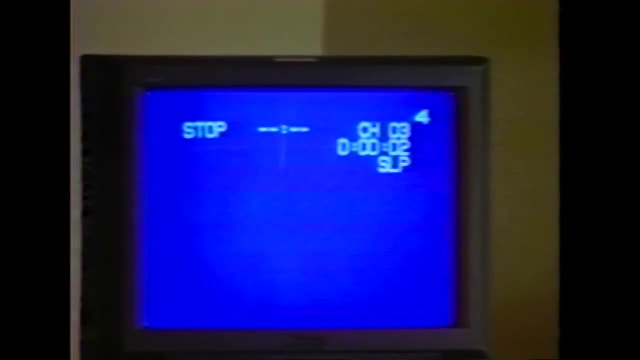 Because The Tape Is Really Bad- Of One Of The Very First User Test In July Of Nineteen Eighty And The One And We 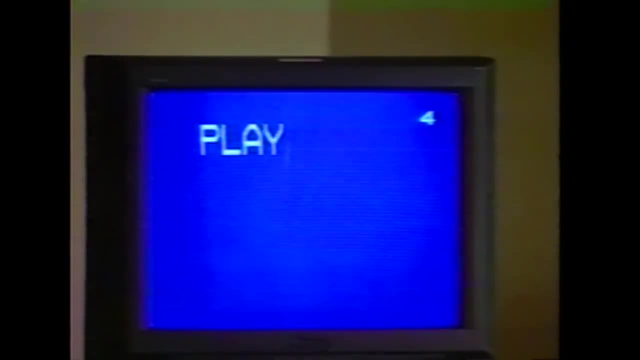 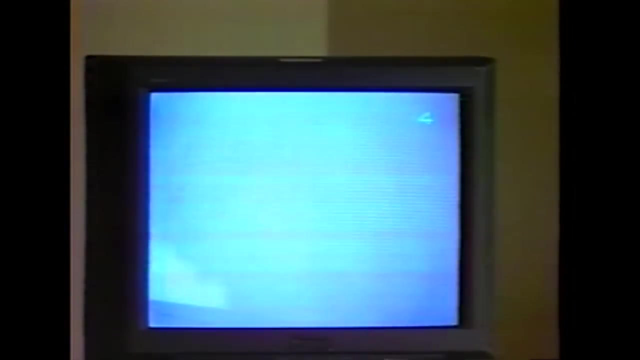 Think It's Set Up. Let's Try. And Is There Audio On? Yeah, I Taught You To Place Whatever You Type. Places That Another Option. 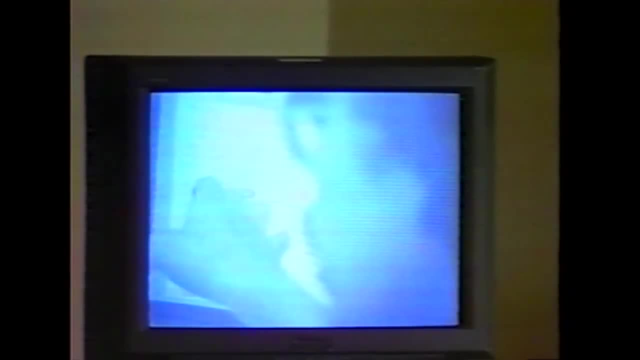 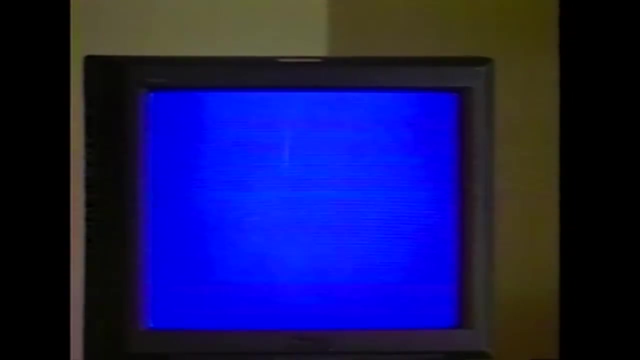 That We Have To Use A Person Made With The Mouse, And He Just Explained Something Very Simple And She Didn't Understand It, So He's. 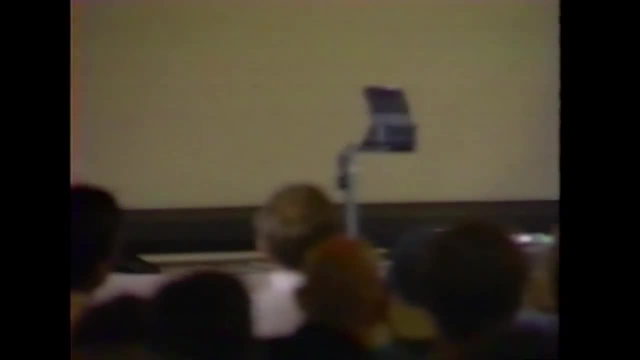 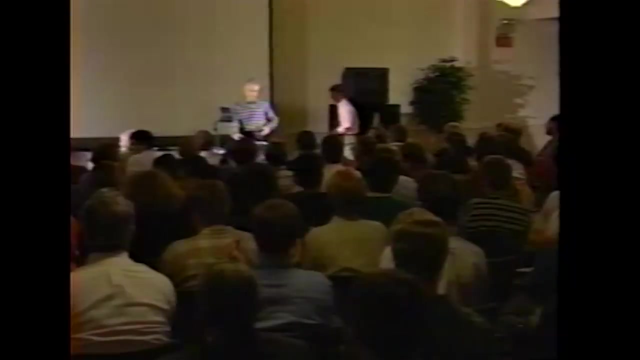 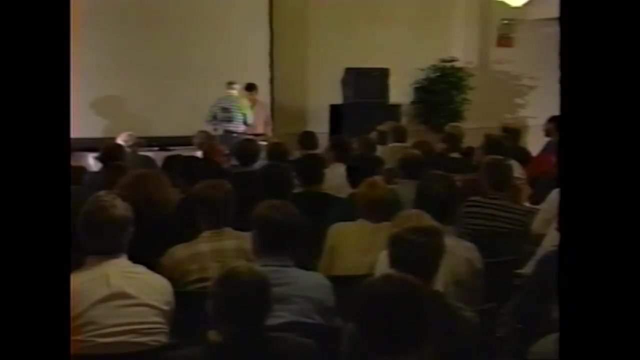 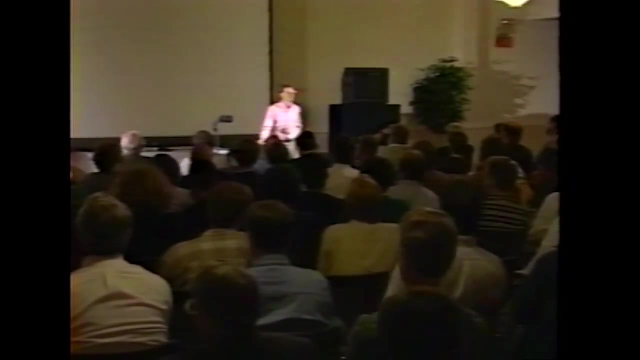 Starting All Over And Now We Got To Great Thanks, Very Much, As Larry Said, The Work, That End Of The Very Fruitful Period Of 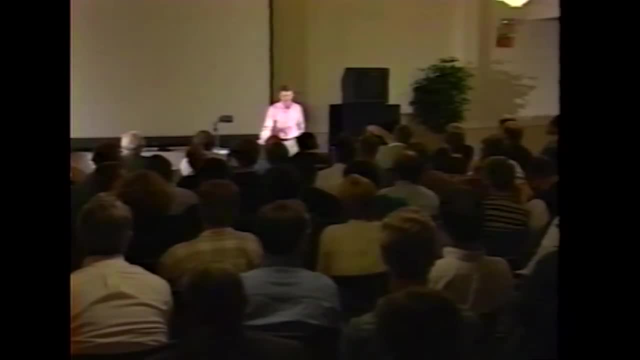 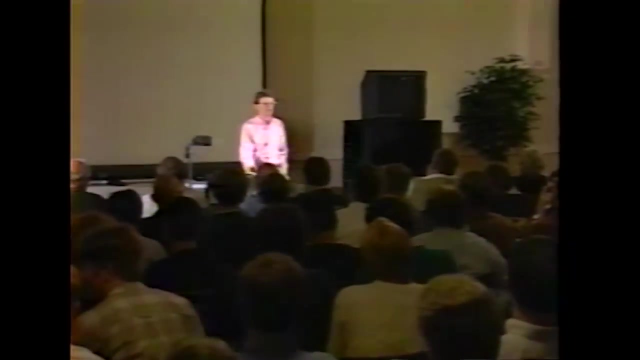 Lisa Human Interface Design. I Can't, I Cannot Believe How Much Work They Went Through In A Short Period, Months In The Year. From Some 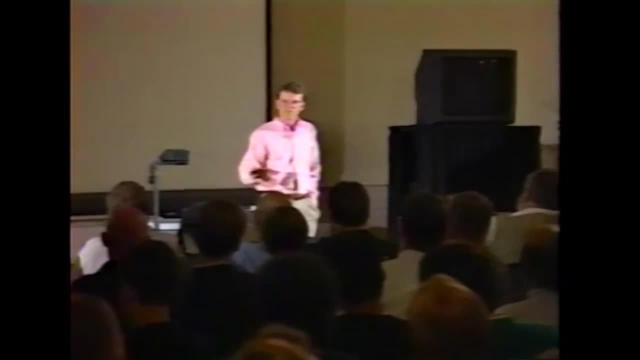 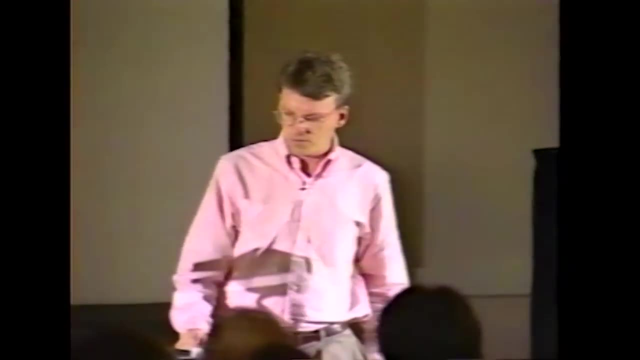 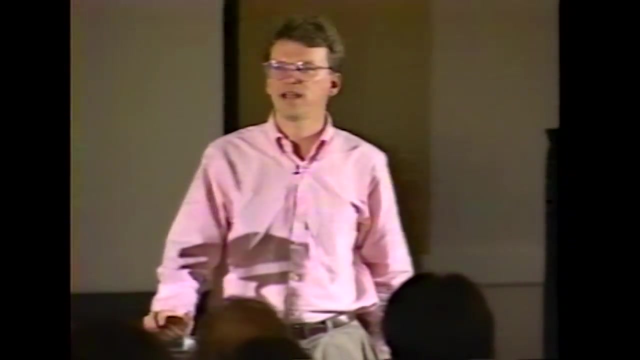 Companies We'd Acquired On How The User Interface Came To Be, That, That A Lot Of The People He Was Referring To, A Lot. 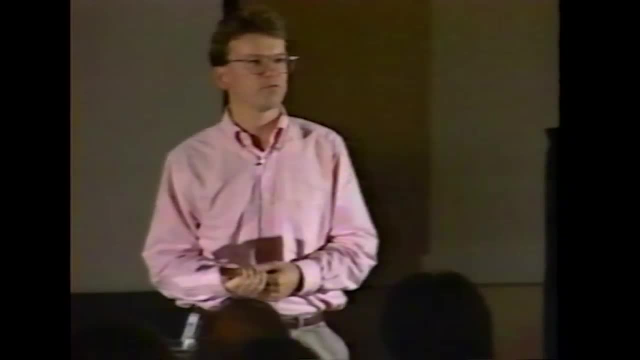 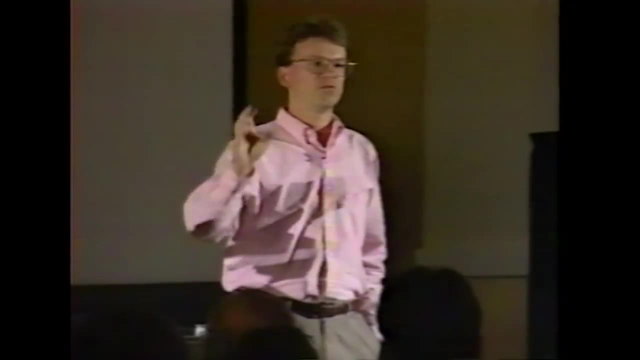 Of The, the Apple II and the Apple III human interface effort that was going on in the personal computer systems division, which was by that time physically remote, down in the big black triangle-shaped building at the intersection of 280 and Lawrence Expressway called the Triangle Building. 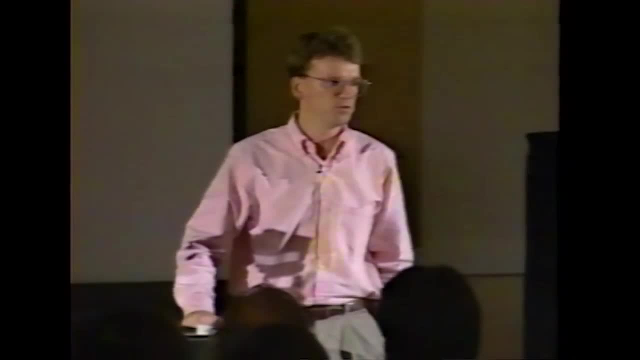 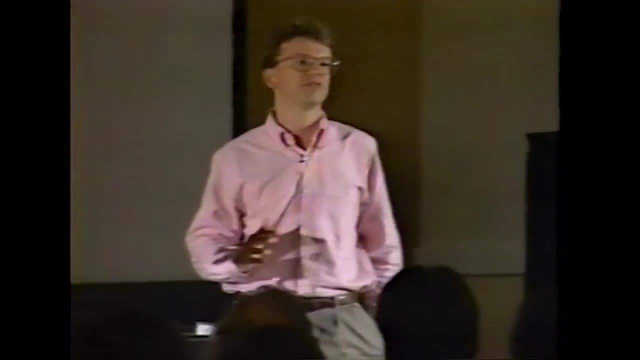 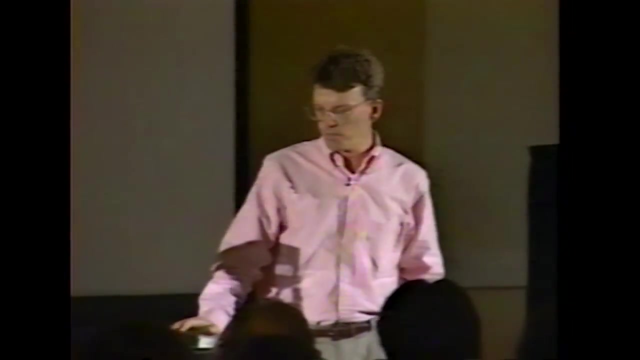 or, by then, the Bermuda Triangle, because it's where the Apple II group had been moved to die. The thing that you really have to understand about the crucial difference between the Lisa Macintosh human interface effort and what was going on in the Apple II group was not. 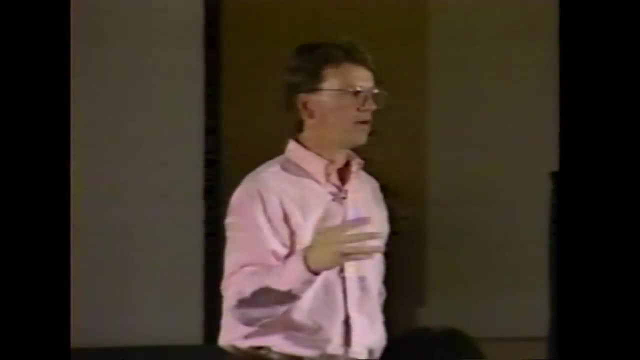 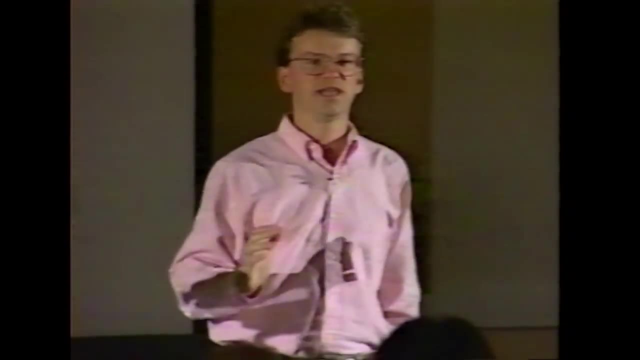 the difference between the graphic human interface and the text-based human interface, though that was an important part of it. The crucial difference was that in the Lisa and the Macintosh, the engineering groups were completely integrated in and the driving forces behind making the computer easier to. 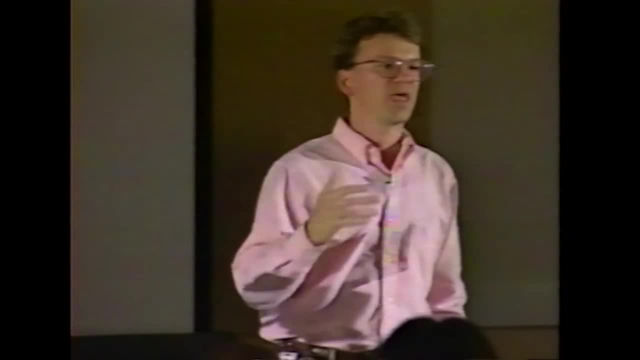 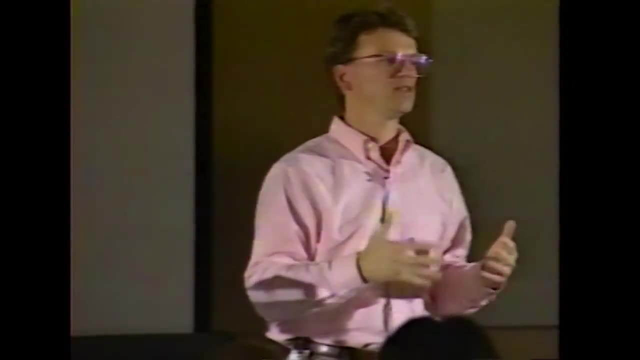 use, Whereas in the Apple II the evolution of that had been that the impetus for making the computer easier to use had been that the impetus for making the computer easier to use and which programs were selected to make that, had come from the publications department. 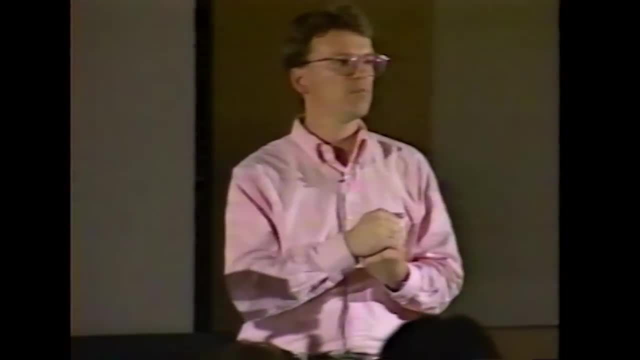 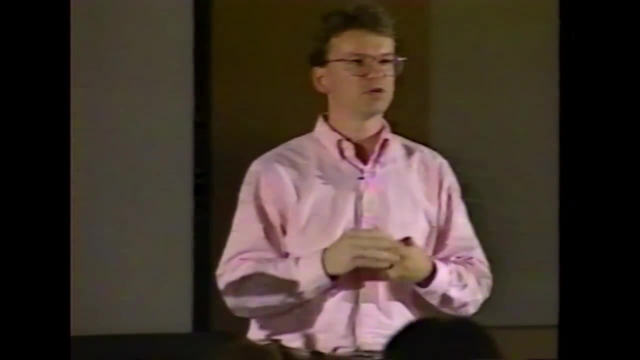 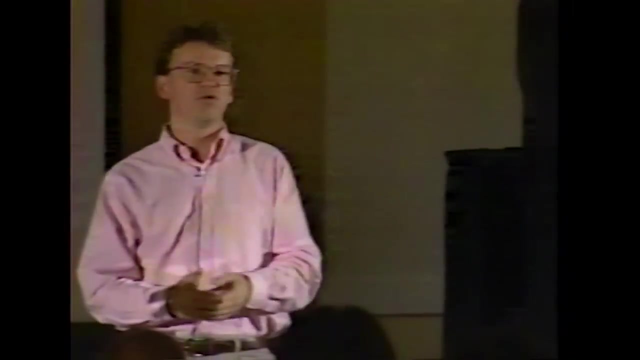 the training department and the department doing demonstrations for in-store retail sales. Our effort- and I was a member of that group and our effort was primarily to mask the complexity of the real underlying software that we were already shipping by putting sugared user interfaces on top of the real interfaces and by putting training. 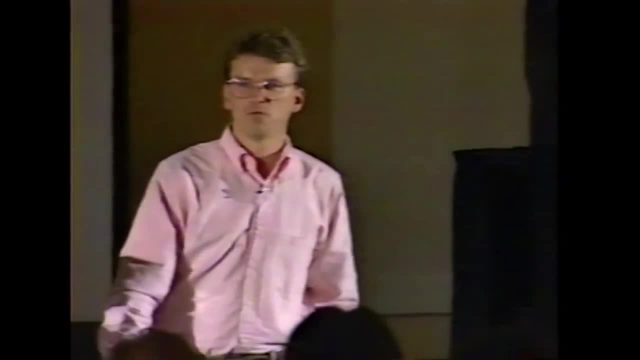 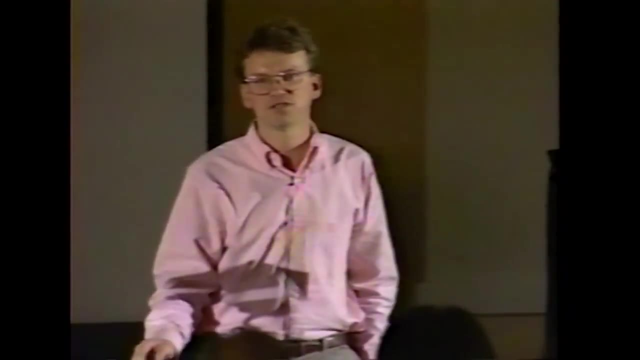 programs on top of the strong user interfaces, on top of the real computer programs. And this was, remember, the Apple computer by 1980. Boy, we'd been around for three years. We had a long history behind us in the personal computer industry. 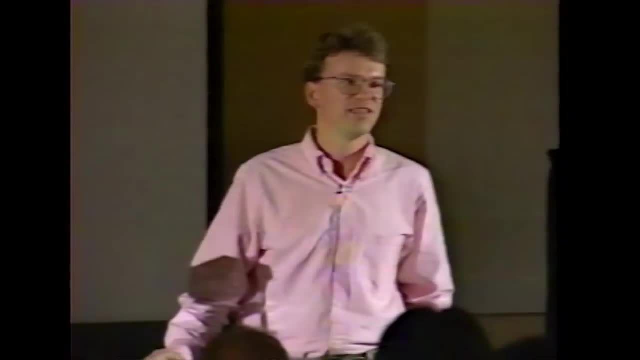 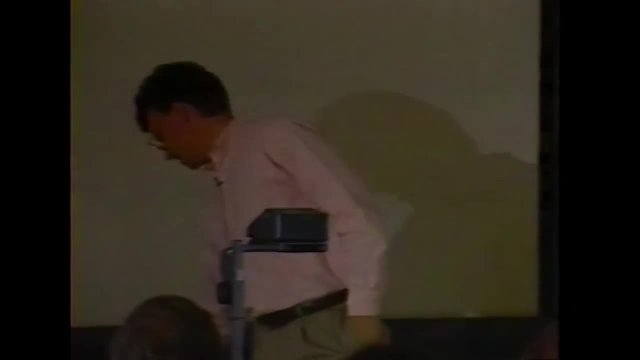 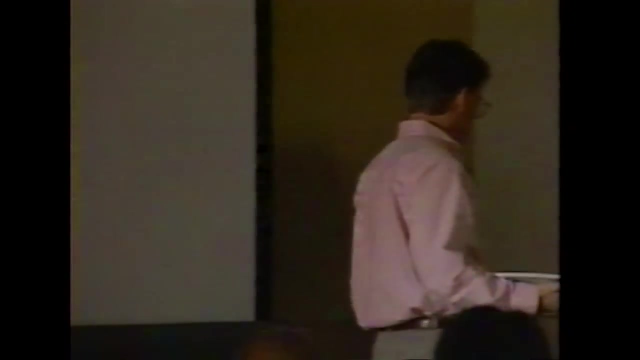 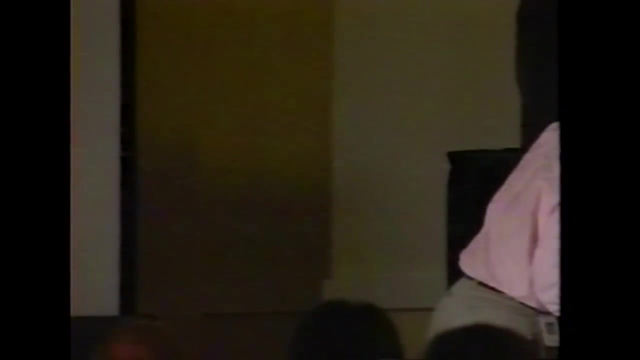 And we had a lot of accumulated legacy software that we couldn't just haphazardly change. We really had to work on it. So one of the documents that I have here is a document. I've got it on video here, although I don't think it'll be that easy to read. 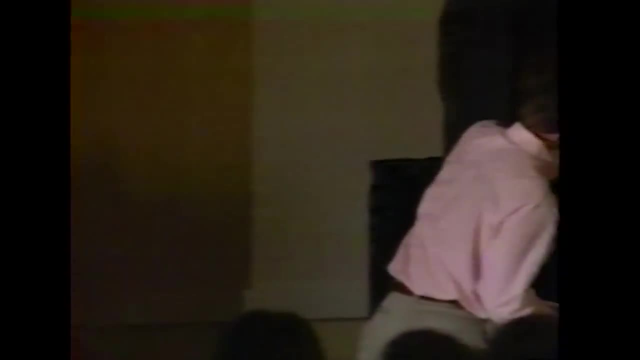 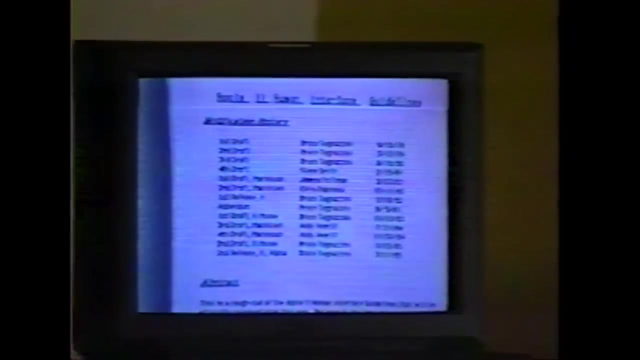 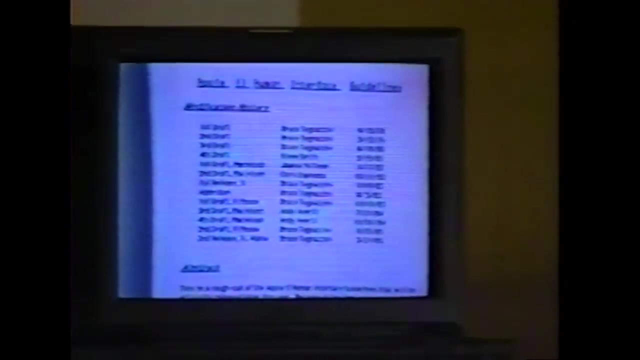 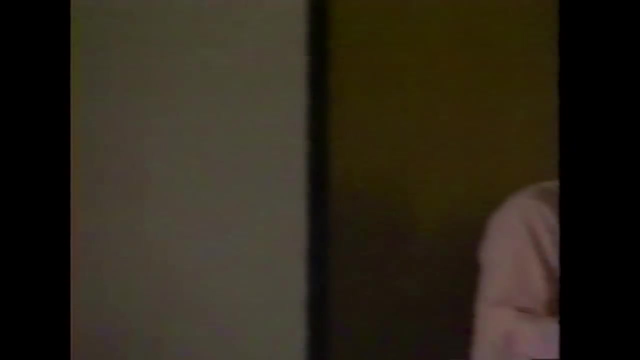 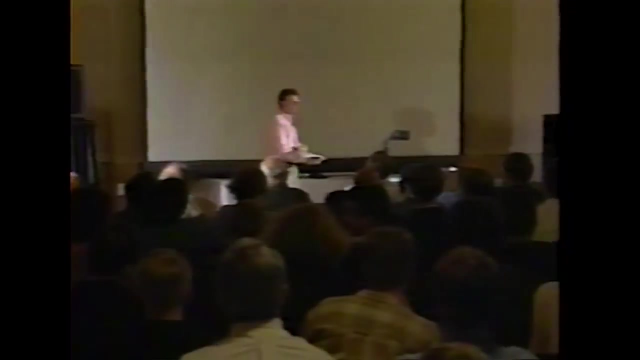 Manuals consistent and provide a consistent and familiar and productive experience to readers of manuals. Bruce Togbazini took the concept of a style guide for growing men. This is the. this is that document And this is the change. This is the change history of the Apple II: human interface guidelines that show the first draft Bruce Togbazini claims to have written in September of 1978. 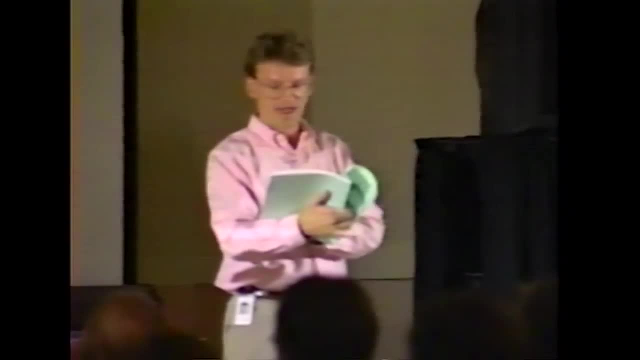 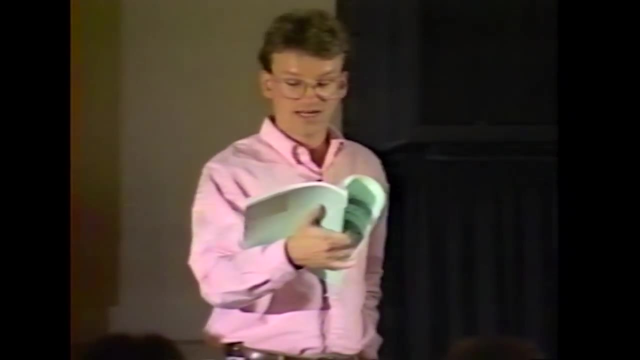 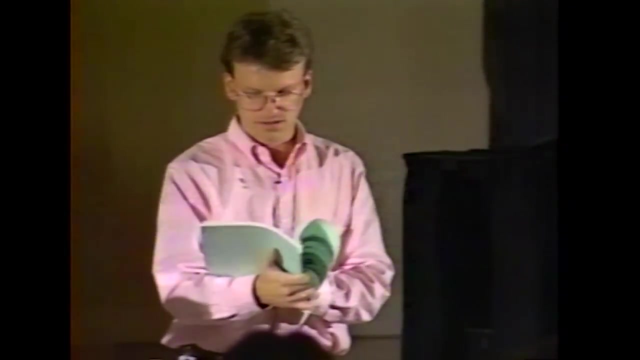 Second draft in March of 79.. Third draft in mid-1980.. Fourth draft with Steve Smith in early 1981. And then it got into the Macintosh group in 1982. And that's when I incorporated many of the things from the Lisa efforts. 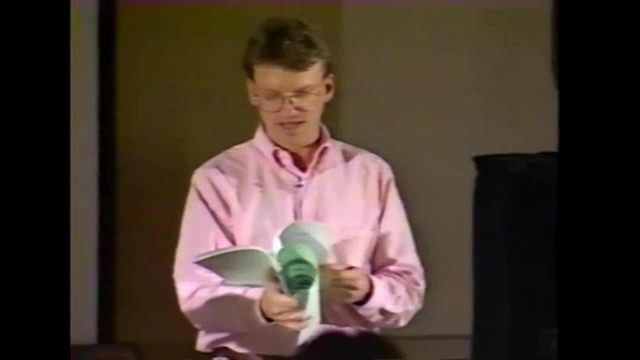 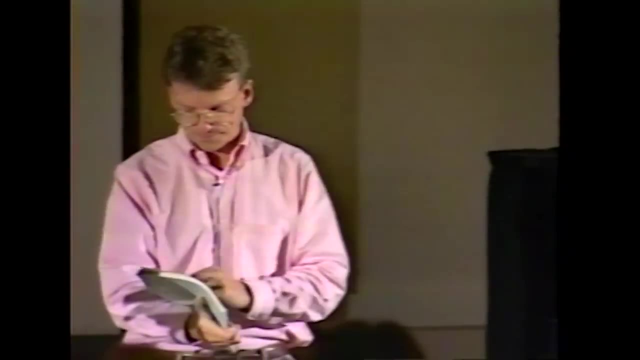 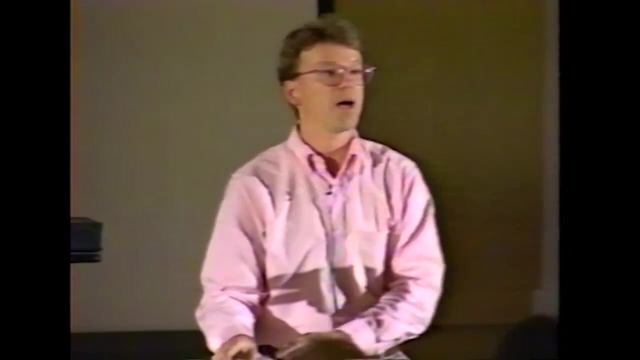 And then it moved back over into the Apple II group to cover the Apple II graphic user interface. But it originally started as an Apple II text human interface document And it came originally from Bruce's efforts with JD Eisenberg writing an application called Apple Presents Apple. 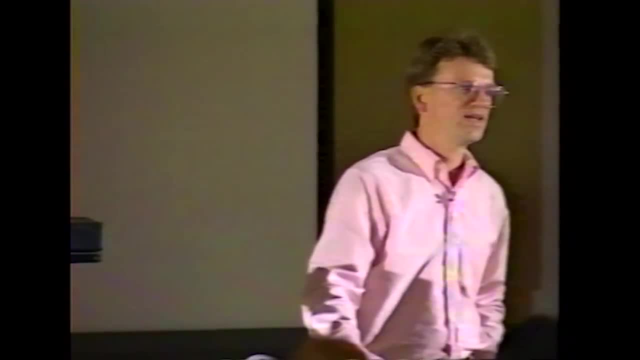 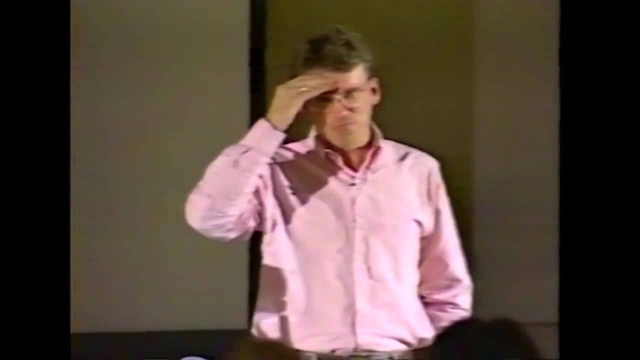 which was the main in-store or first user demonstration program for the Apple II, Bruce started out. well, I don't know where Bruce started out, But when we've when we encountered Bruce Togbazini in his long and checkered career. 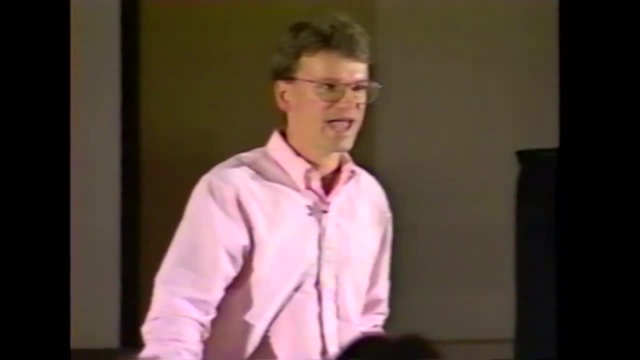 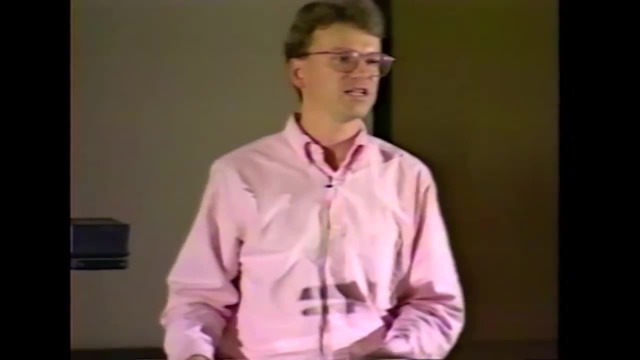 he was the proprietor of a computer store in San Francisco, which is where the Apple Corps of San Francisco used to meet, And that's how he got into the Apple community- by selling Apple computers. So he had frontline experience of what happened when a person encountered a personal computer for the first time. 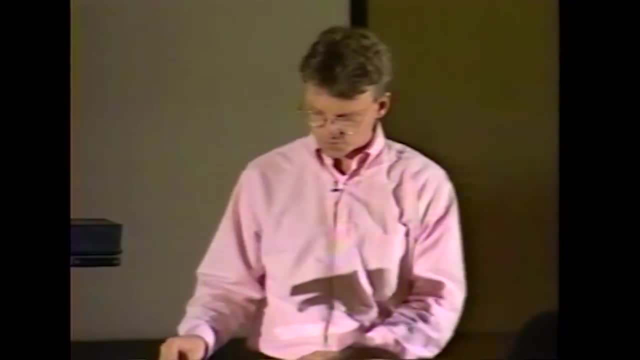 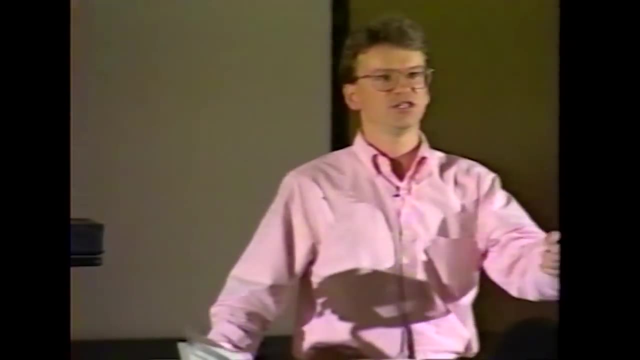 When he came to Apple, he started writing demo programs with JD Eisenberg And one of the things that they did was they tested on real users in real situations where you bring somebody who's never seen a computer before. much like the Lisa group was testing. 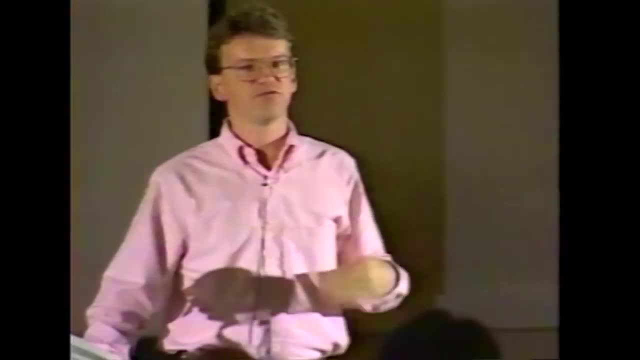 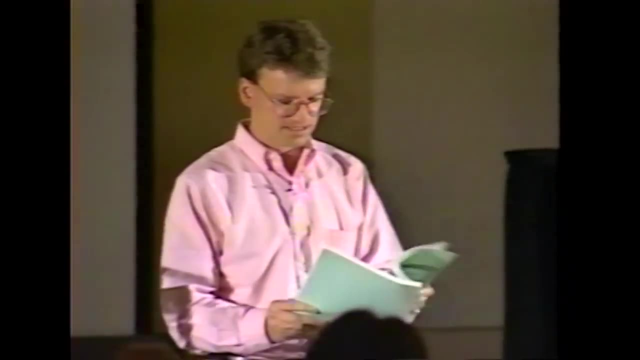 people off the street or new employees, put them in front of this program and gave them no advice whatsoever. I'm going to read: Bruce tends to philosophize a lot in this, so it's not going to be as useful to put up slides. 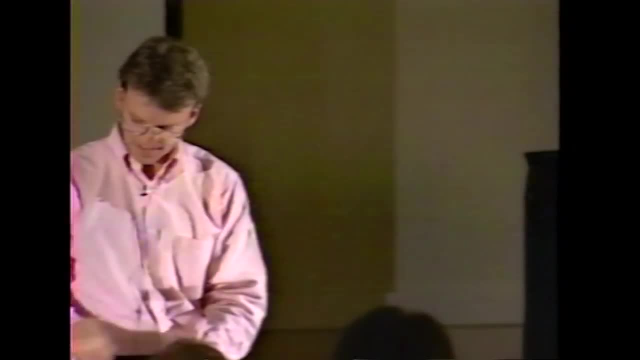 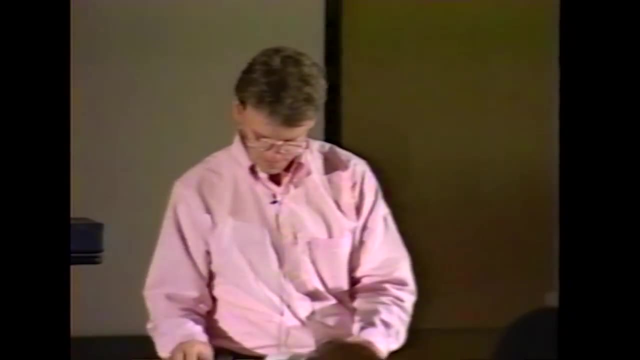 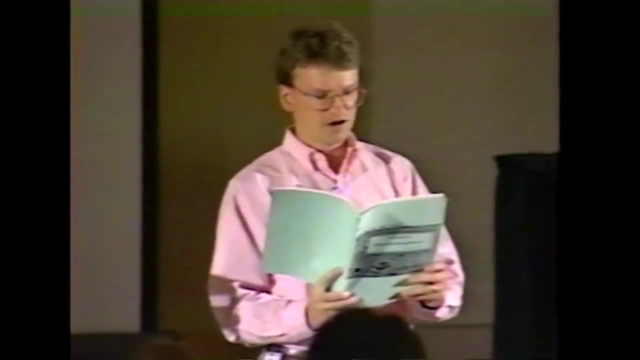 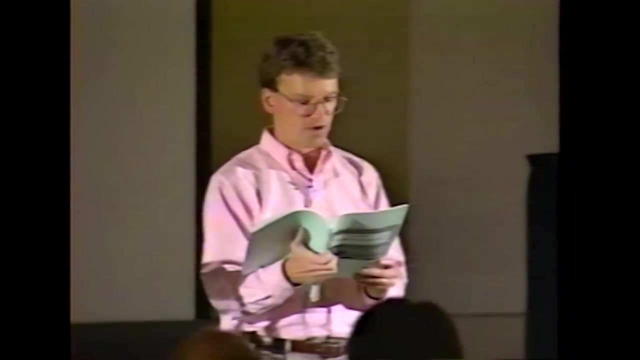 But I'm going to read to you some of his experiences Here. we go From user testing. Our testing method is as follows: We set up a room with five to six computer systems. We invite groups of five to six users at a time to try out the systems. 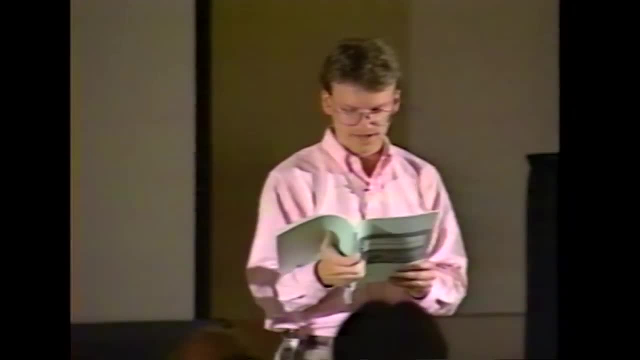 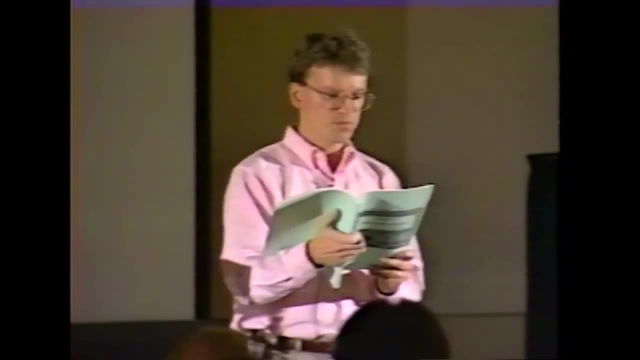 often without knowing that it is the software rather than the system we are testing. We have two of the designers in the room, Any less, and they miss a lot of what's going on Any more. the users feel as though there's always someone breathing down their neck. 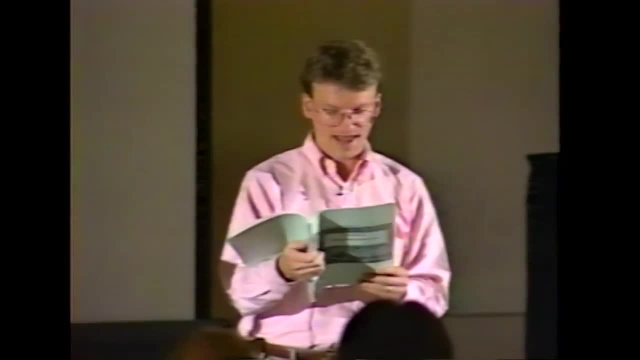 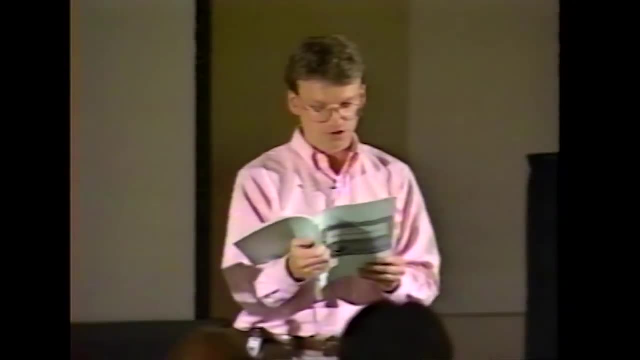 The initial ground rules are that no questions will be answered, as by the time the formal testing begins, we can supply a draft of the manual, Usually by the second group. some glaring defects in the interface have shown up and we have to give them help getting past the stumbling blocks. 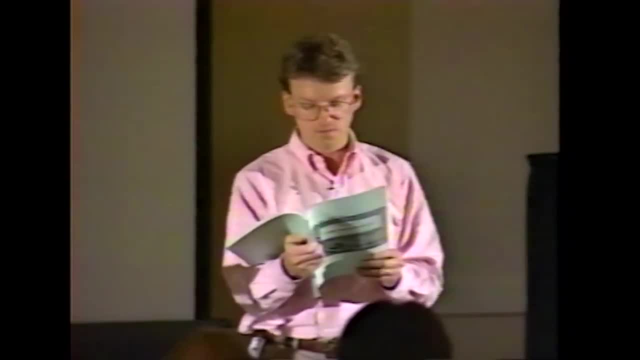 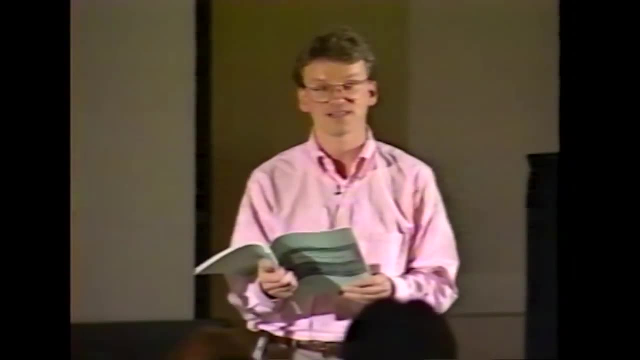 Ninety-five percent of the stumbling blocks found are found by watching the body language of the users. Watch for squinting eyes, hunched shoulders, shaking heads and deep, heartfelt sighs. When a user hits a snag, he will assume it is his fault. 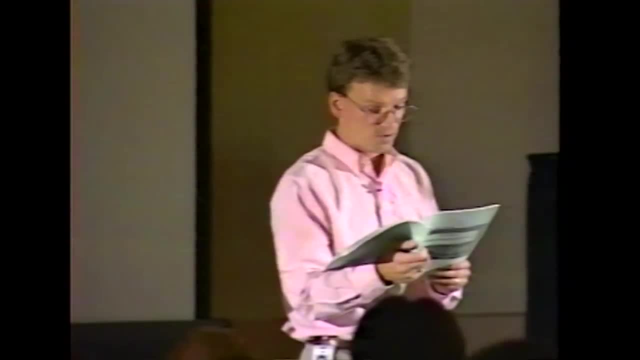 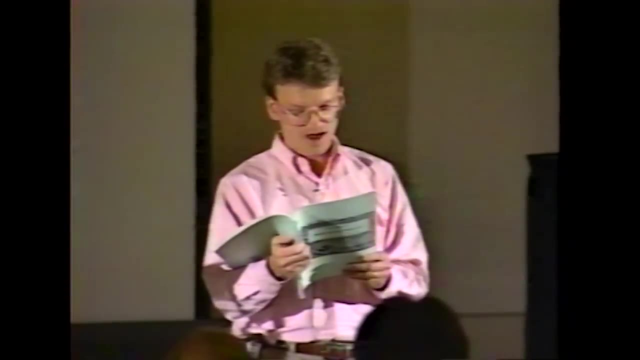 He will not report it. He will hide it. Make notes of each problem and, where it occurred, Question the users at the end of the session to explore why the problem occurred. You will often be surprised at what the user thought the program was doing. 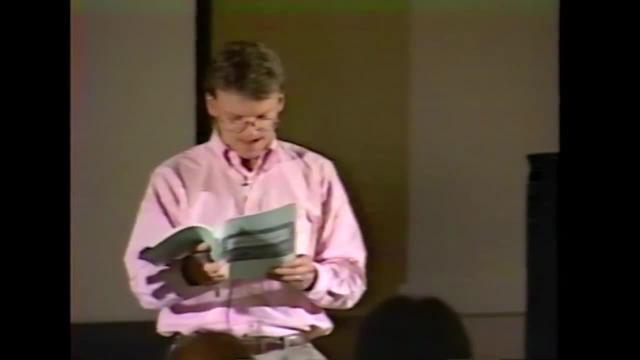 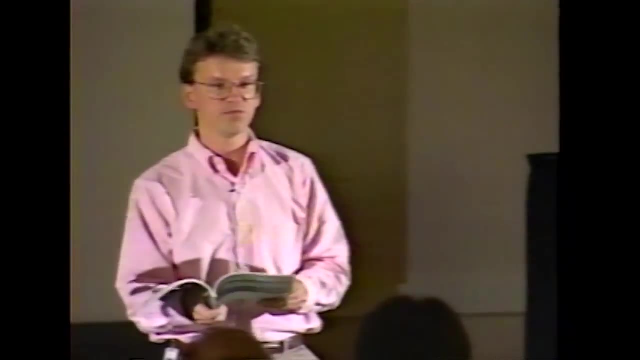 at the time he got lost. Herein follows a true anecdote which illustrates how difficult the most simple human interface issue can be and why thorough testing on real people is so important. As we tune in, It's so easy to entertain a crowd just by reading something Bruce wrote. 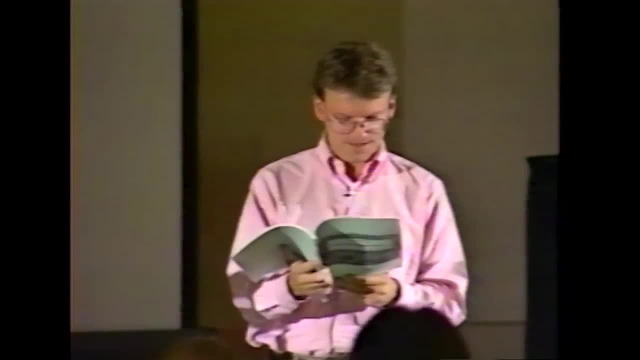 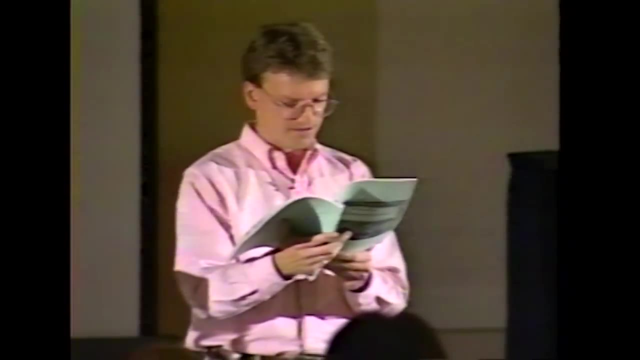 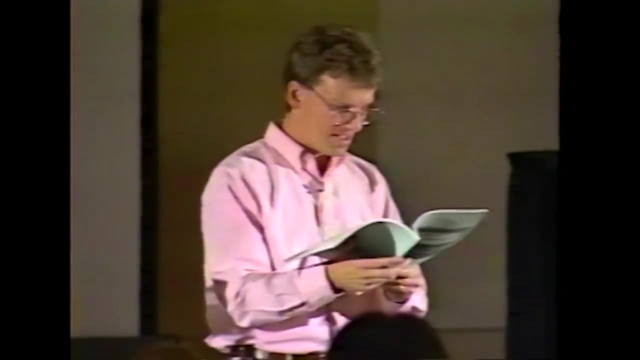 As we tune in, the authors of the software, both of whom pride themselves on clever interface design, have anguished for hours over difficult passages in their program. It was to turn out their guesses were quite accurate. in said difficult passages, It was the simplest question of all that caused the problem. 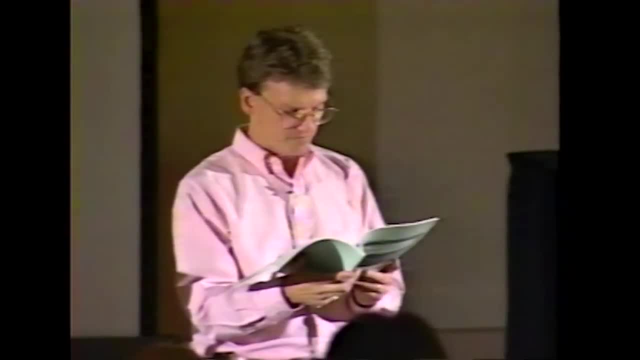 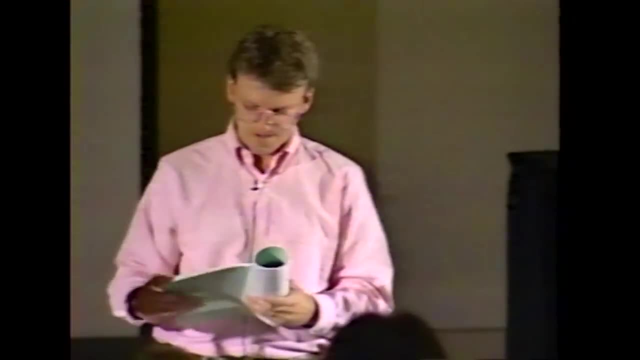 In. Apple Presents the Apple IIe, a training program for teaching fundamentals of using the new Apple IIe. find out if the user is working with a color monitor. User profile, new owner, customer in a computer store or member of a class learning how to use an Apple computer. 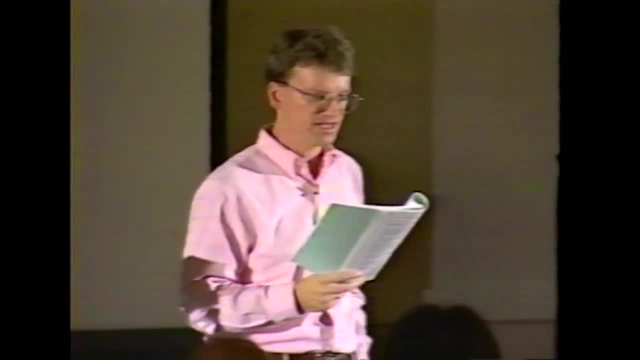 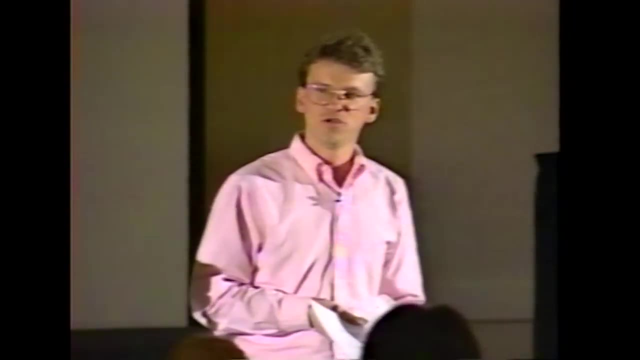 Test user profile. customers in a computer store, non-computers in a classroom environment. friends and relatives. First design: a color graphic is displayed on the screen Prompt. are you using a color TV on the Apple Anticipated problem? those who are using a Chrome monitor. 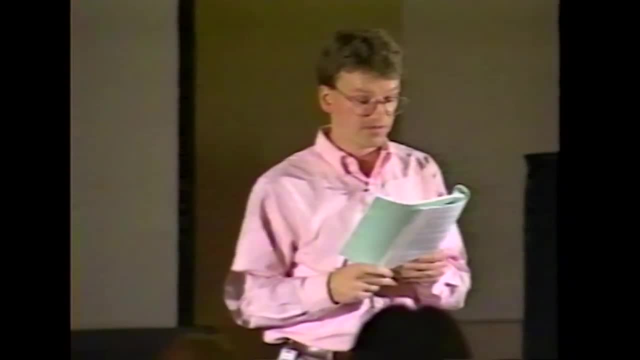 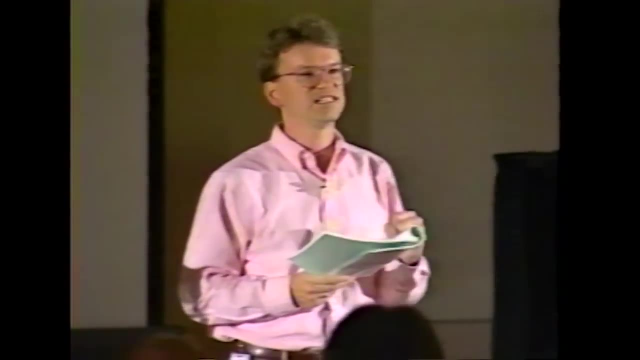 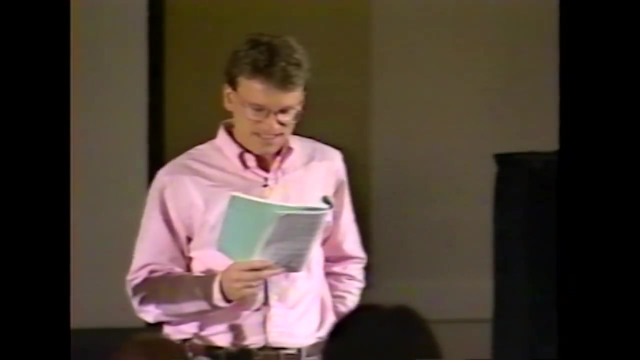 in a classroom or a computer store. situation wouldn't know whether the monitor was black and white or was colored. with the color turned off, First attempt to color graphics displayed Prompt is the picture above in color. 25% failure rate. Reason as anticipated but incorrectly overcome. 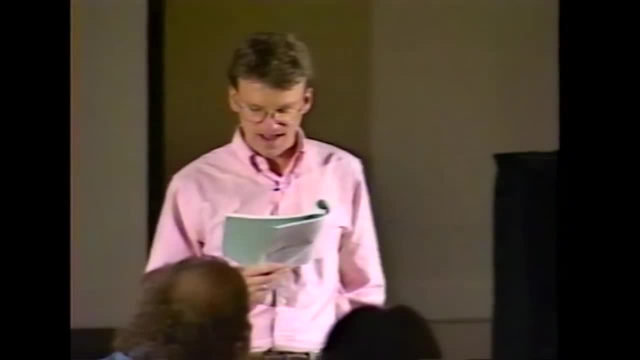 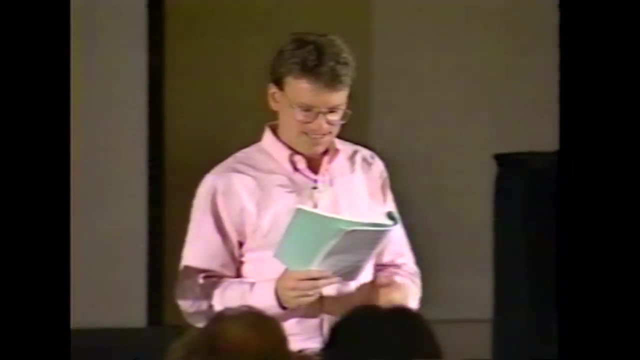 those seeing black and white thought their color might be turned down. They didn't answer the question wrong. They turned around and asked one of the authors whether the monitor in question was color or not. A decision was made. the authors could not be supplied with the disc. 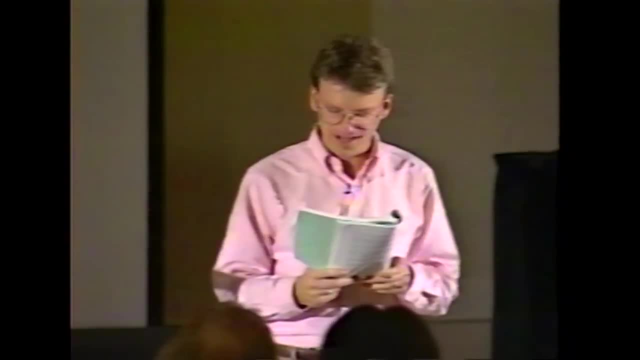 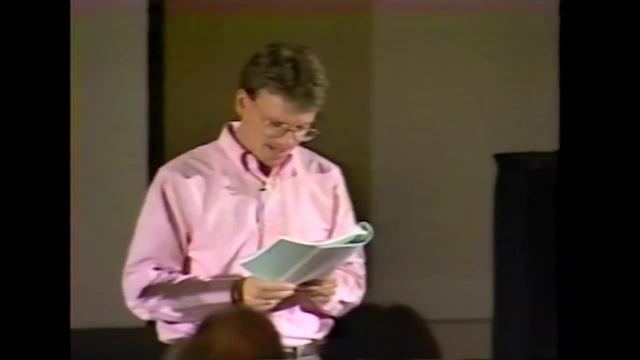 Second attempt: a smaller graphic with large letter words in their own vivid colors was substituted: green, blue, orange, magenta, which were the only colors the Apple II could display. Prompt are the words above in color: Color failure rate: color TV users: none. 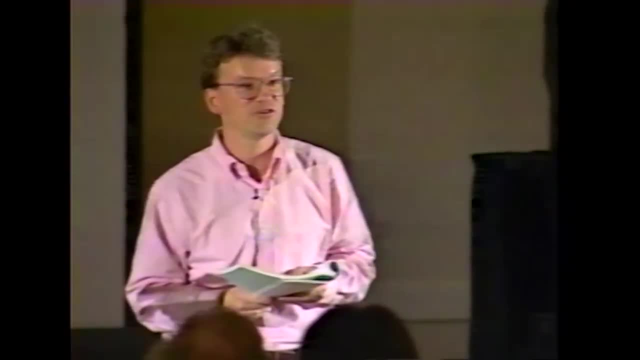 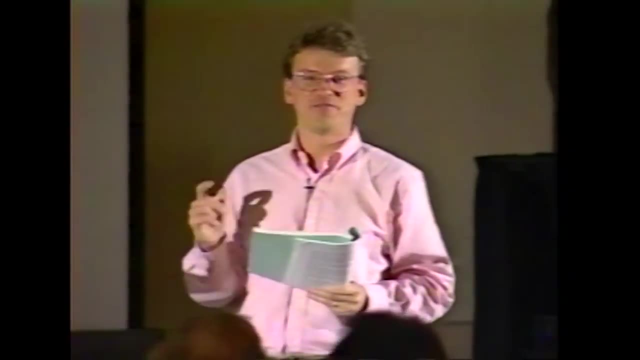 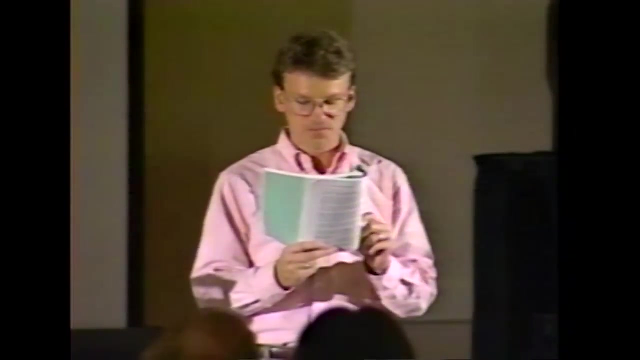 Black and white monitor users: none. Green screen monitor users: 100%. This is why it pays to have a variety of configurations in your test suite. Third attempt: the graphic remained the same. Failure rate prompt are the words above in more than one color. 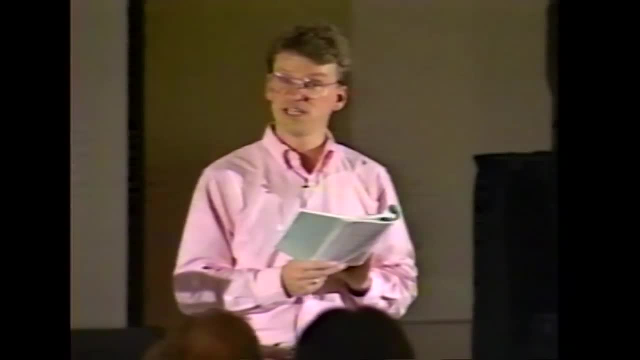 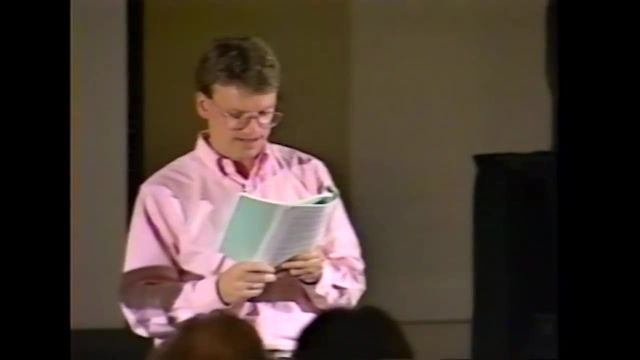 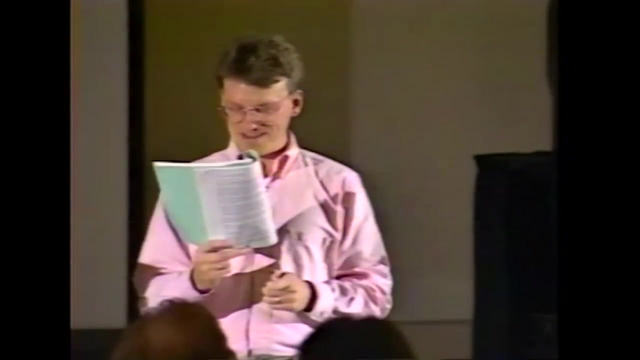 Failure rate. color TV users: none. Black and white monitor users: 16%. Green screen monitor users: 50%. Reason: the black and white monitor users who answered incorrectly admitted they did so unbrought. This is the purpose. 50% of the green screen folk considered that they were looking at both black. 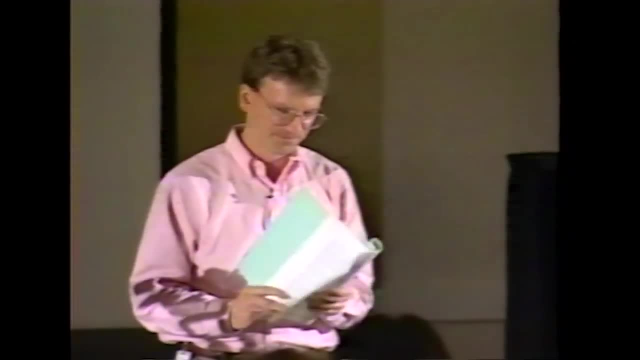 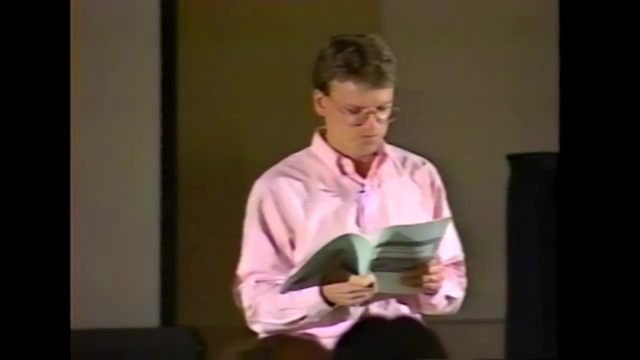 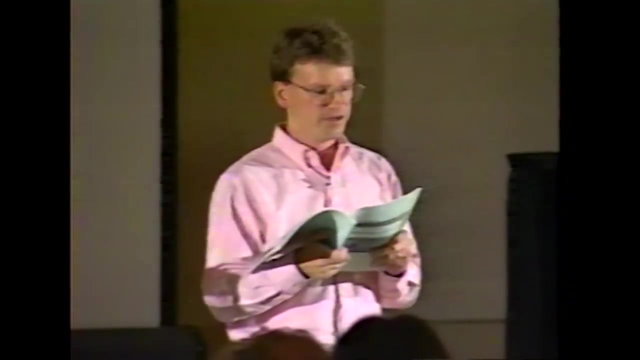 and green- two colors- and answered the question accordingly. Fourth attempt: same display of graphic and colored text. Prompt: are the words above in several different colors? Are the words above in several different colors? Failure rate: color TV users: none. 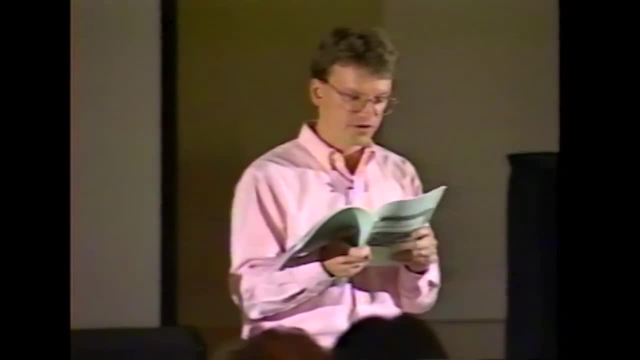 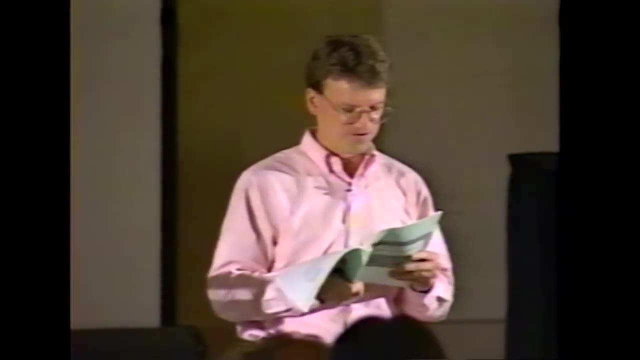 Black and white monitor users: 20%. Green screen monitor users: 23%. By this time the authors were prepared to supply everyone who bought an apple with a free color monitor, just so we would not have to ask this question. It turns out about 20% of the people were not really reading the question. 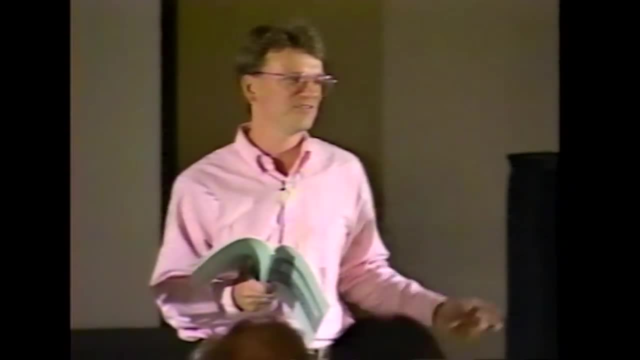 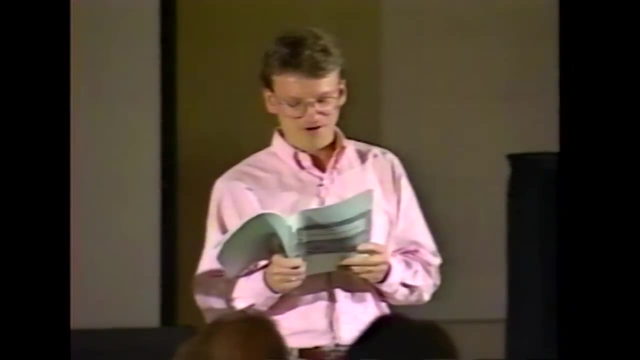 and were responding to. are the words above several different colors? Well, yes, of course. Green, violet, red, there are several different colors. Let's move on. Fifth attempt: same display of graphic and colored text Prompt: do the words above appear in several different colors? 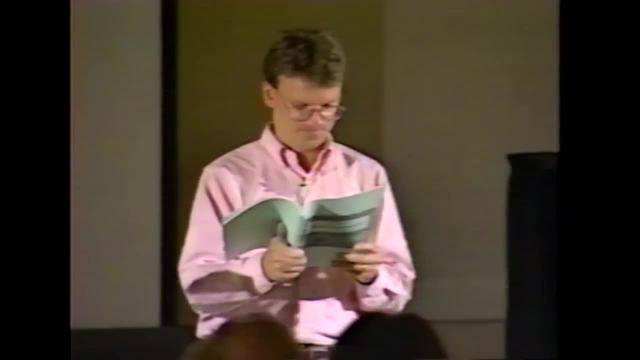 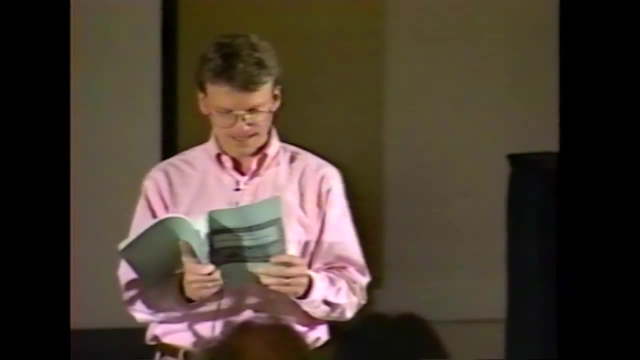 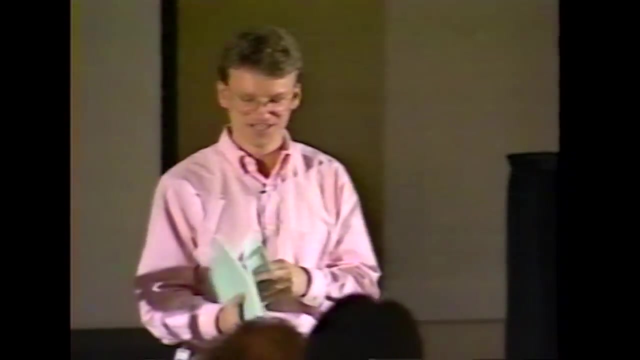 Failure rate none In case, it appears the authors were simply dull fellows. be it known that this was a fully interactive training program in excess of 100K of code. Remember, it was a 128K machine And this was the only interface issue that required more than one correction. 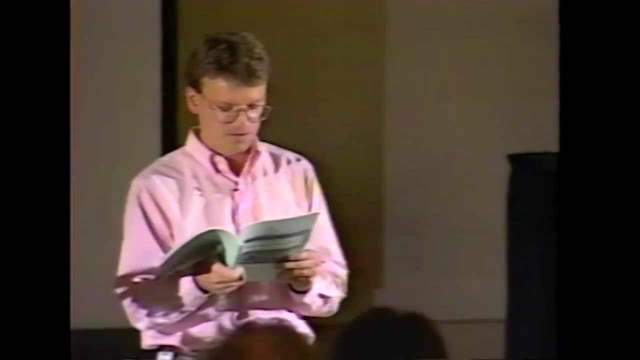 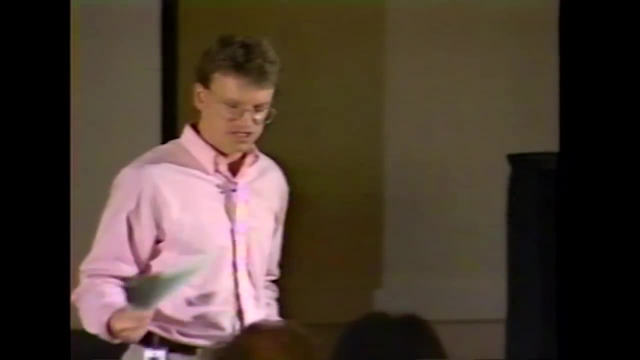 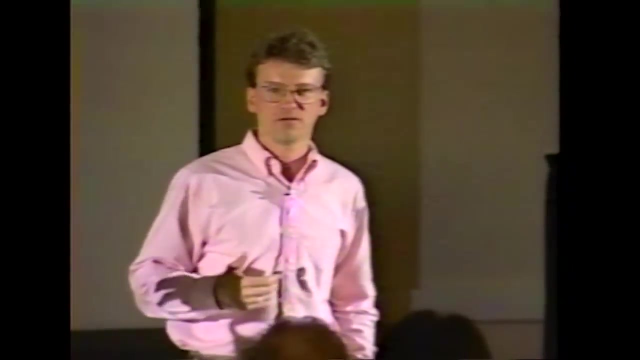 It clearly exemplifies how even the most careful designers can totally miss when guessing at how users are going to respond. So a reading from Bruce Tognosini. The Apple II project had started out well. the Apple II wasn't really a project. 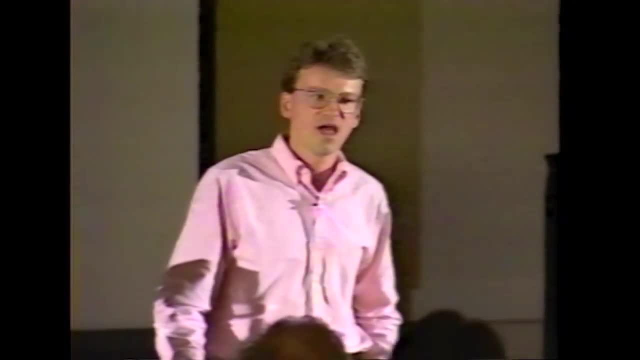 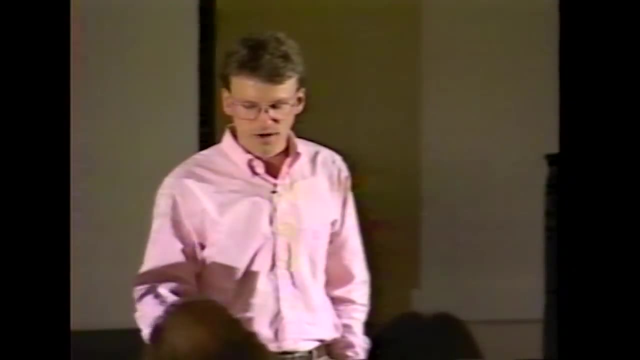 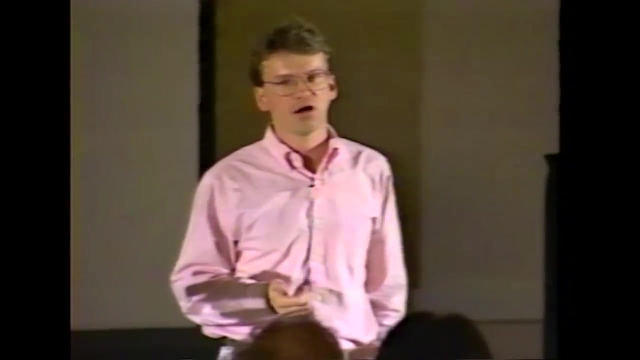 it was a collection of projects. We started out with a number of pieces of software that had our cherished angle bracket or square bracket prompts. By the time we got around to the Apple IIe and the Apple III, we developed a more or less text windowing interface called the file card metaphor. 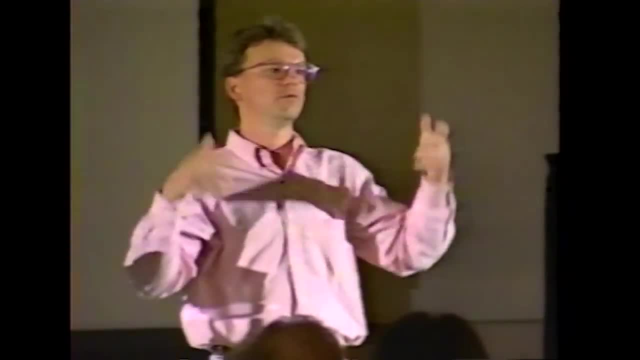 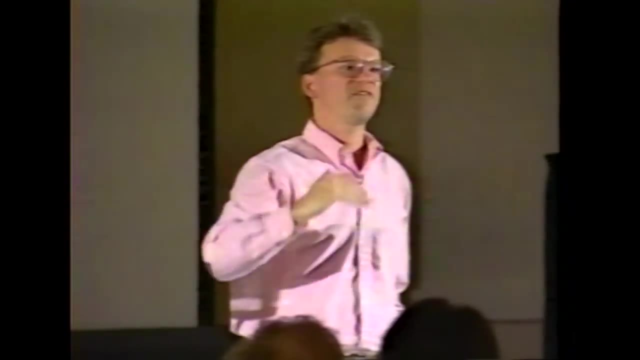 where we used special characters and the character generator ROM to do something like the file card interface in the Lisa with pick 1,, 2,, 3,, 4,, 5, 6 menus and you use the escape key to back out through a hierarchy. 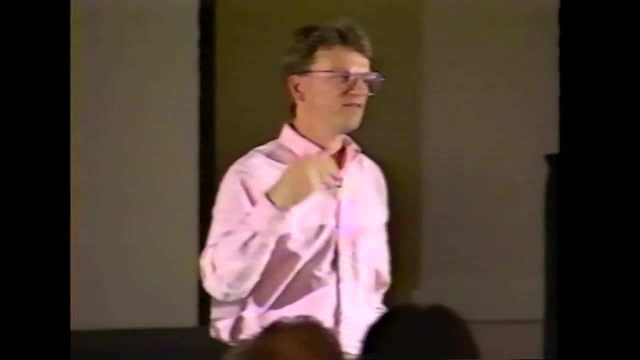 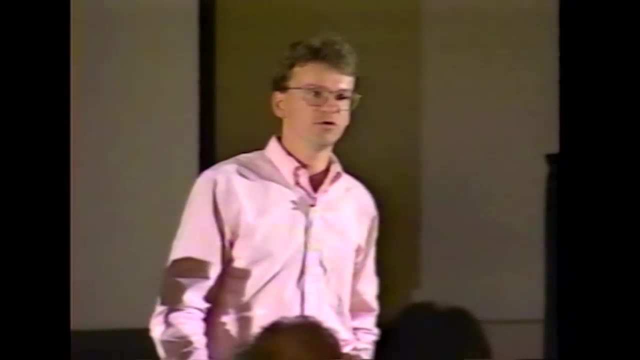 and press numbers 1,, 2,, 3,, 4,, 5, 6 to advance to the next level. It was a hierarchical, spatial, text-driven, keyboard-driven user interface. It didn't use the mouse. It was very successful for what it did. 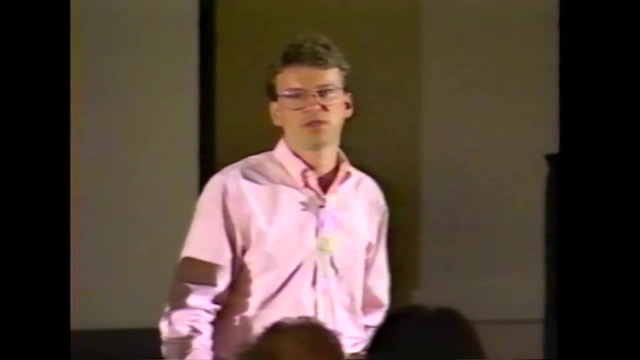 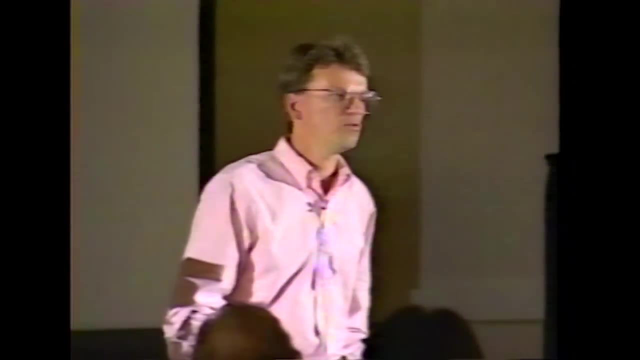 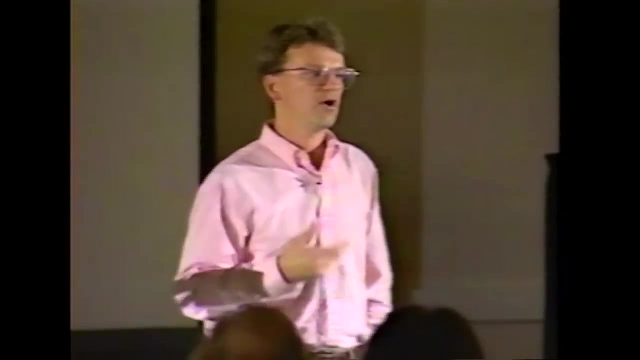 We ensured consistency across many applications: all the applications that Apple implemented, as well as third-party applications. For example, if anyone was familiar with Quark Catalyst, Quark they're the people who make Quark Express. now They made the original hard disk manager for the Apple II and the Apple III. 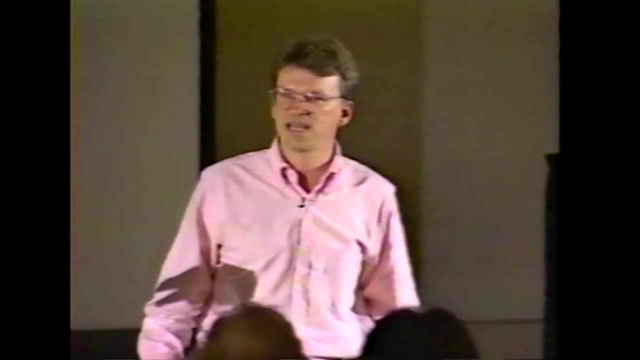 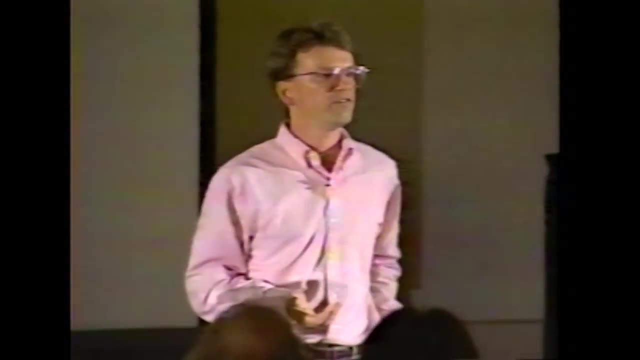 and it used the same interface. It had consistent use of the keyboard keys. The open Apple always meant the same thing in different applications and so, even though it was a text interface, it had many of the underpinnings of the consistency of the graphic user interface of the Macintosh. and it was driven by the exigencies of user training, which was my mother's group, because the less time we had to spend on user training, the cheaper and faster it was, and if the software were consistent, the training went more easily. 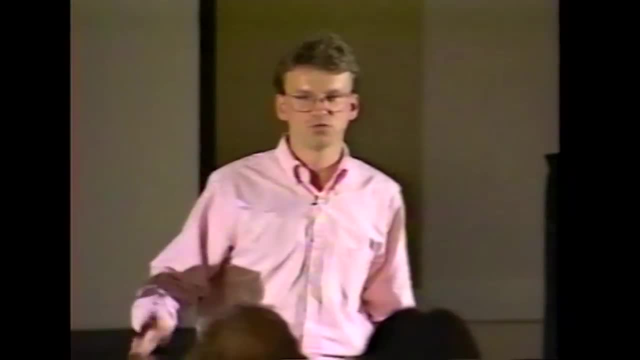 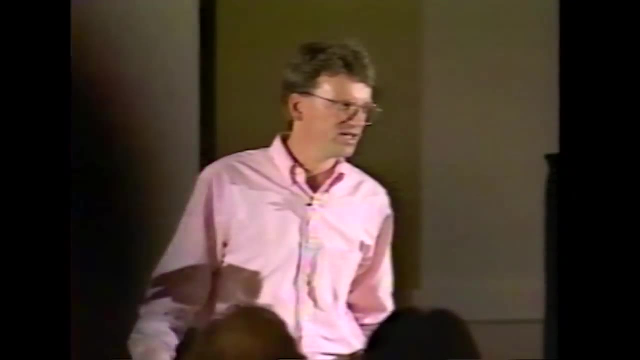 It was driven by the exigencies of publication, which was the group I was running, and one of the problems we faced in publications was that, having not invented desktop publishing yet, we had six weeks minimum from film to printers, which was usually the time that was reserved. 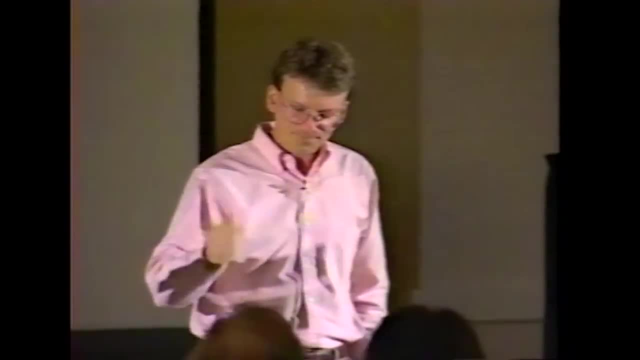 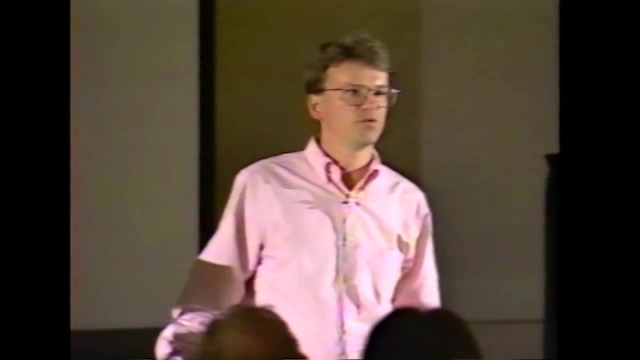 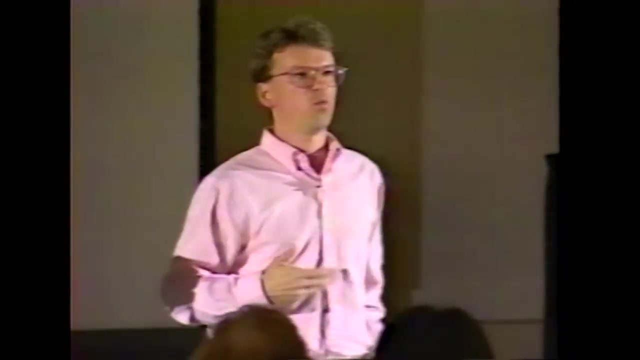 to write or finish the software, and we often had to be finished with the manuals several months before the product shipped, which, in the software, wasn't finished at that point. so, in order to have manuals that accurately reflected what the software was going to do, 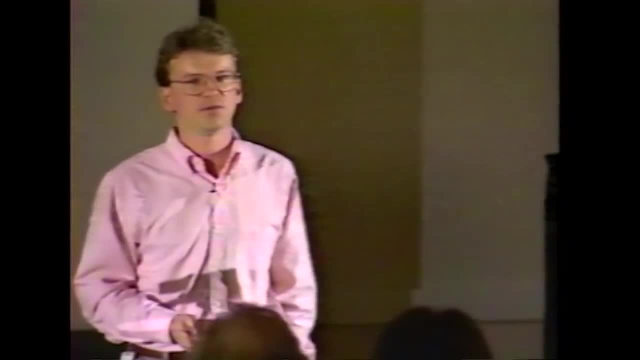 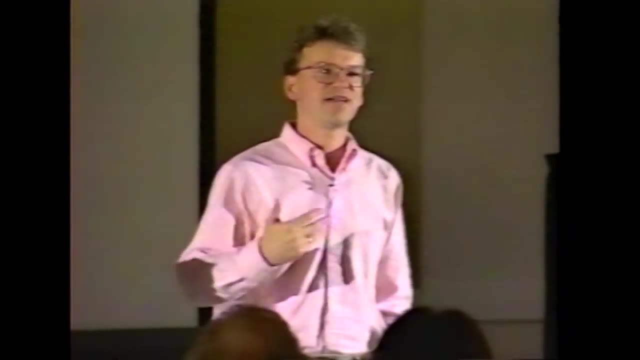 we had to have the programmers tell us what the user interface was going to be and then, in going through that with the programmers, having them do it the same way that other applications did, it gave us a more full idea. for okay, it's going to do this, it's going to do this. 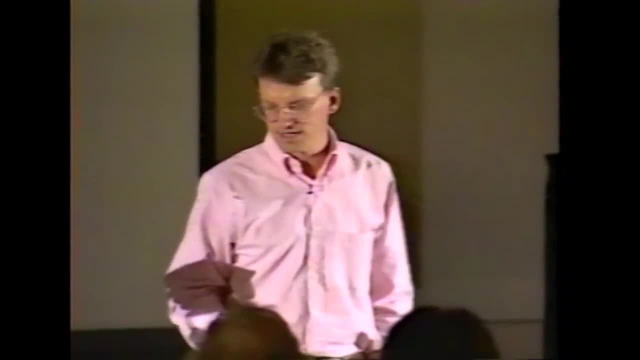 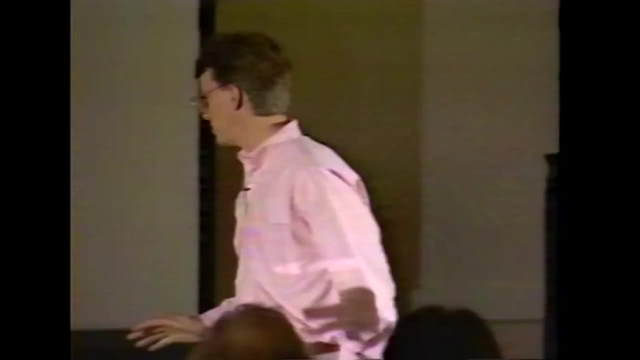 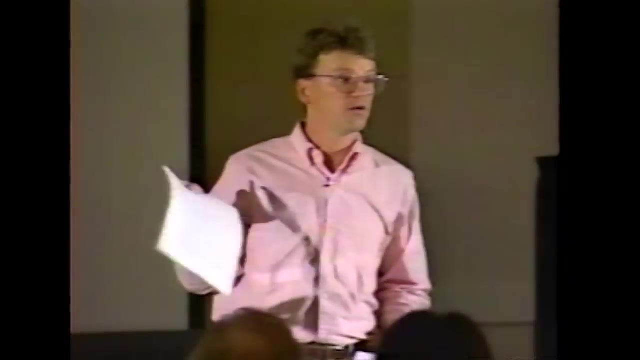 it's going to do that if they followed some standard or some guidelines. In fact, what Bruce did before writing the Apple II human interface guidelines, and what the origin of this document was, was, in fact, a publications style guide, which was how we wrote manuals. 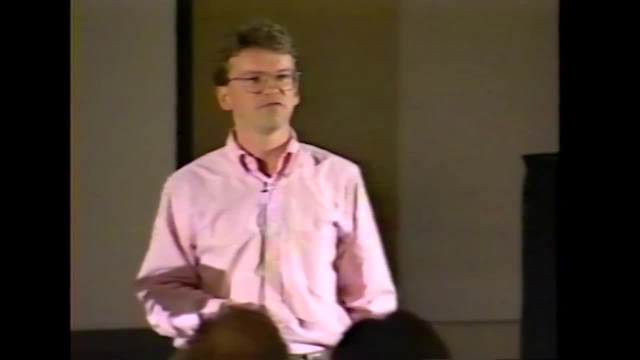 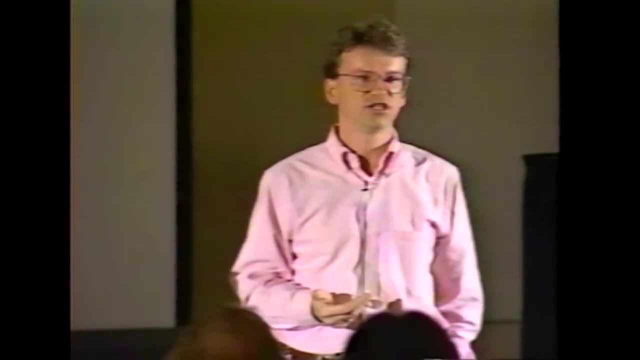 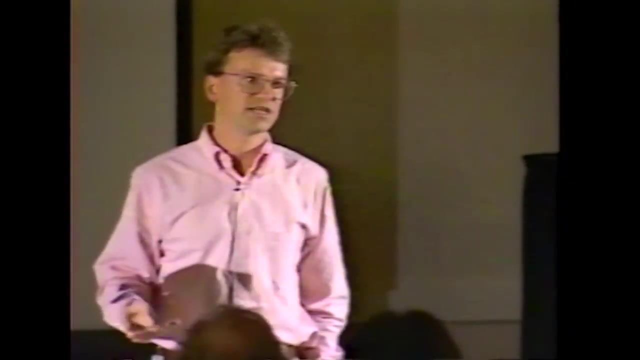 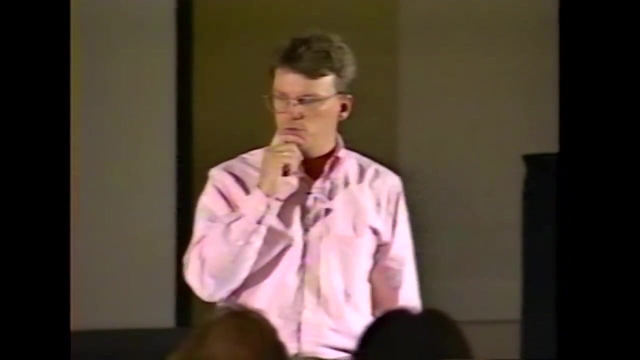 and how we explained portions of the human interface and explained portions of how you use the computer and by using consistent explanations that drove consistent design in some of the applications. So that was some of the origins of user testing and of consistency of use and user interface design in the Apple II group. 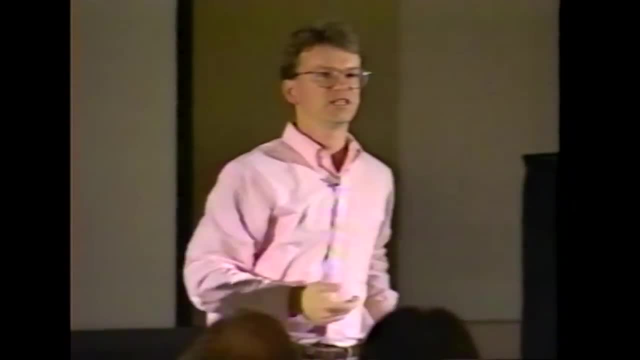 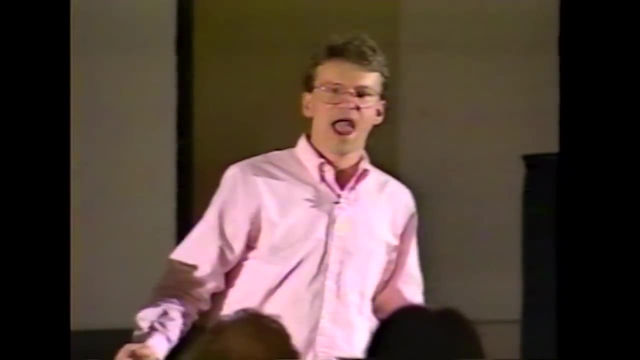 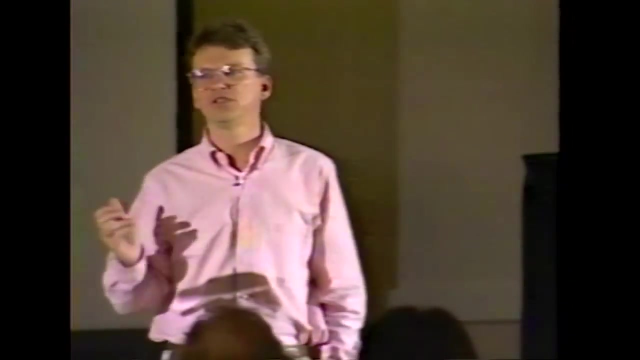 As I said, it moved into the. the LISA group started with a separate angle from which Larry talked about coming from the Xerox PARC, and the two basically fused in the Macintosh group where we had the LISA just benefits of the years of LISA user testing experience. 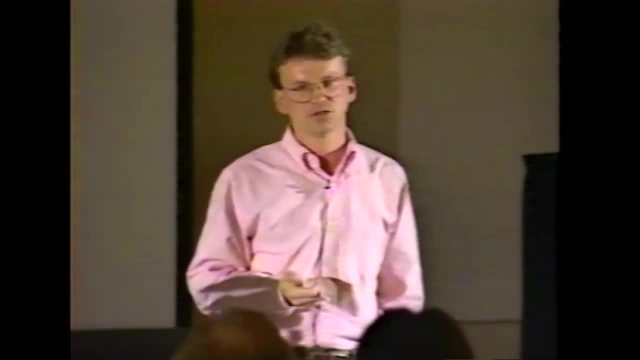 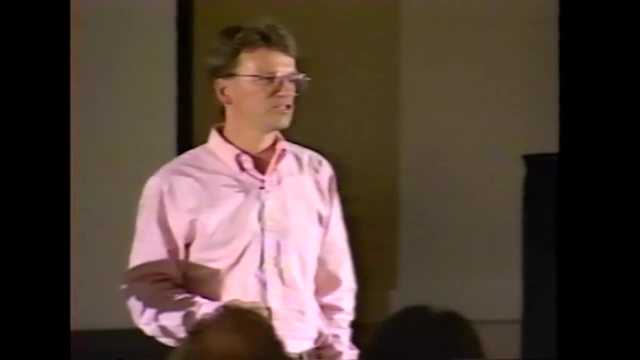 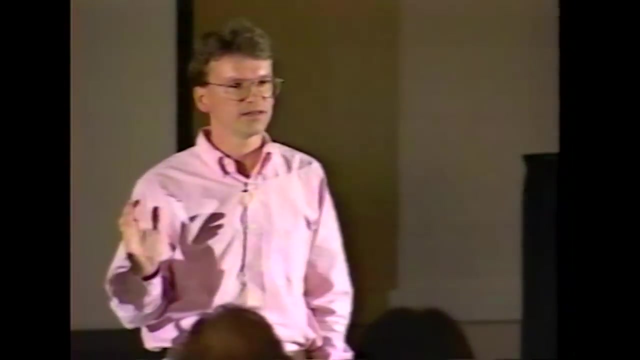 and the massive amount of design that went into their graphic user interface, plus a lot of the the democratic, grassroots issues that had come up through the Apple II. Remember, LISA was only dealing with seven applications. That was all you got on the LISA. 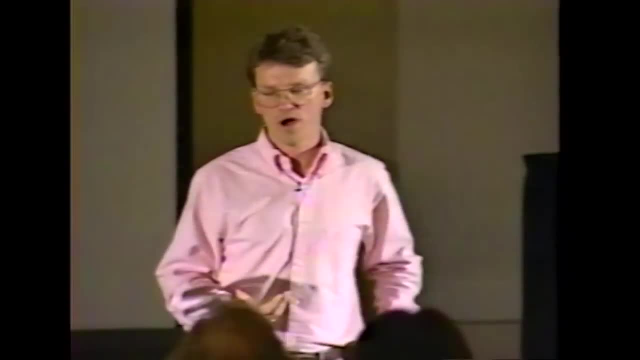 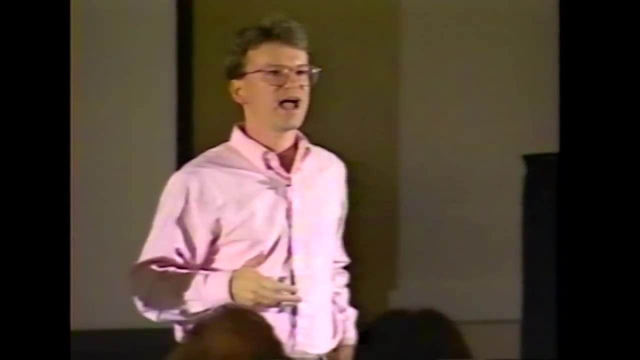 The Macintosh was designed like the Apple II, as something where you had many, many applications from third party developers, and so we took the LISA user interface, grafted it on to the guidelines that had come out of the Apple II style guide and Apple II guidelines efforts. 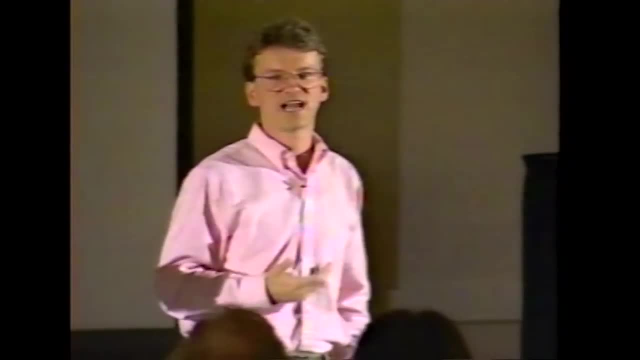 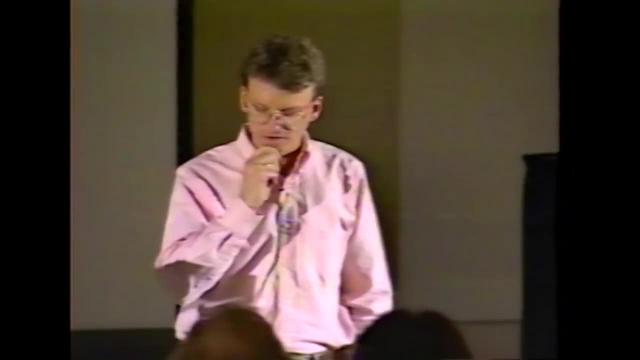 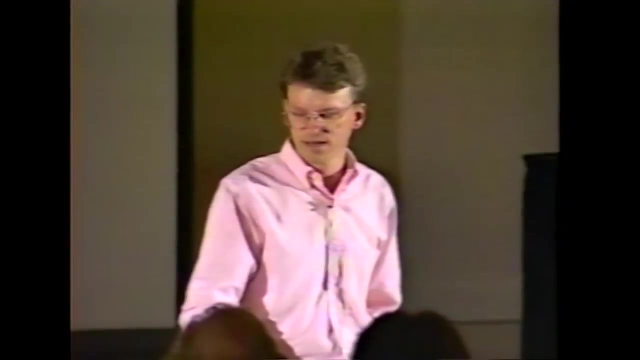 and published that for third party software developers to use as style guides for their own applications. I remember very, very, very clearly that one of the massive controversies around the development for the Macintosh circa 1982, 1983 was developers would come up to us and say: 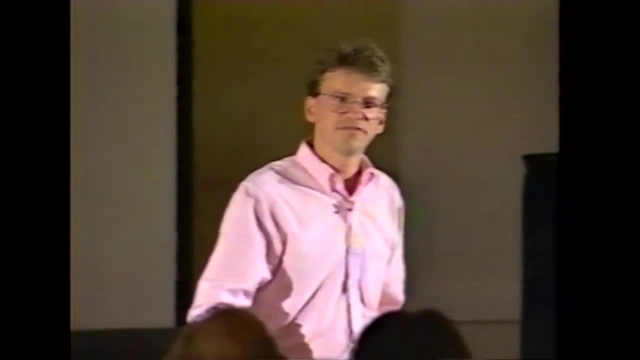 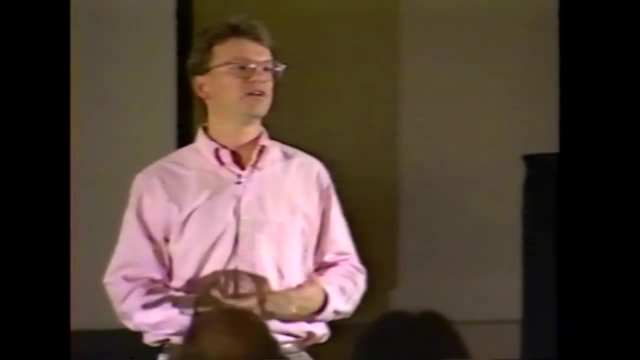 you know if you make the user interface consistent and if you put all that software in ROM that makes it. you know if you make it hard to write to the screen directly so that we have to use your user interface software to talk to the user. 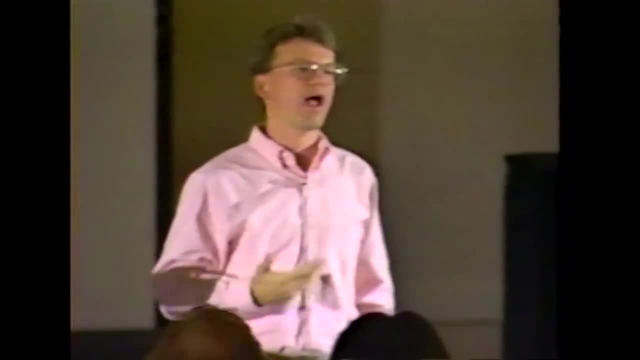 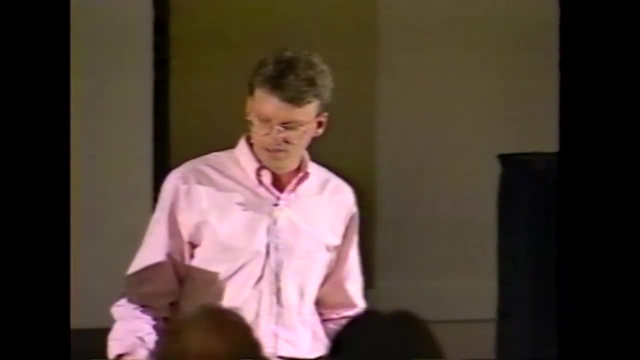 how are we ever going to make our applications unique and stand out and be different from each other in the marketplace? They found a way. I'm very happy, but the human interface and the idea of a consistent human interface, much less a graphic one. 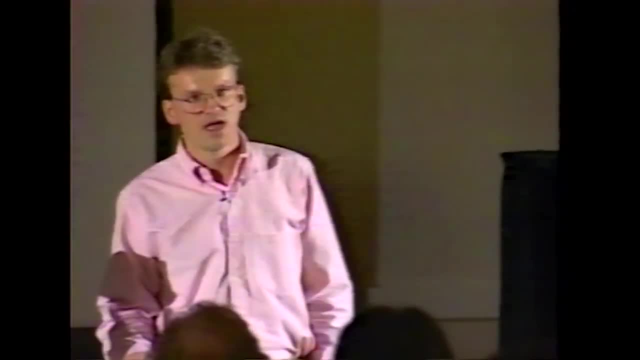 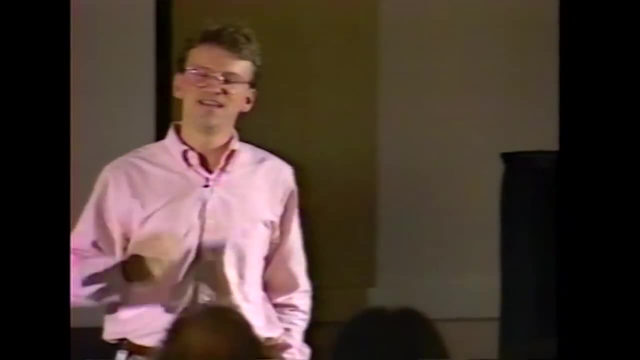 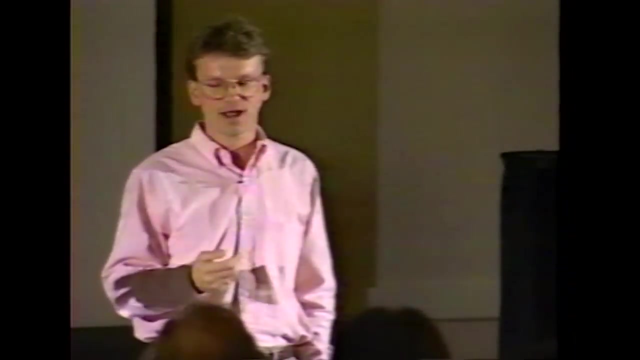 was very, very controversial among software developers, and only by having the user testing under our belt to show them that, hey, this is going to add significant value to your product by making your product easier to learn and easier to use, especially for people who already know another application. 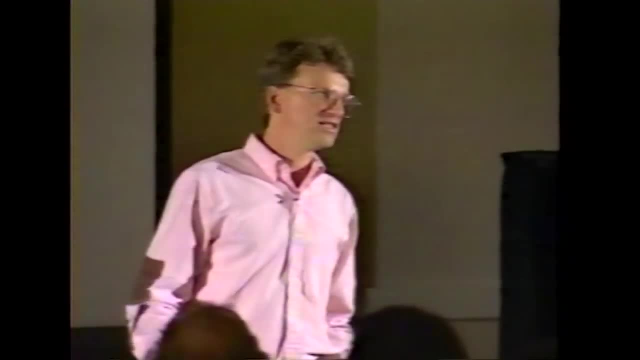 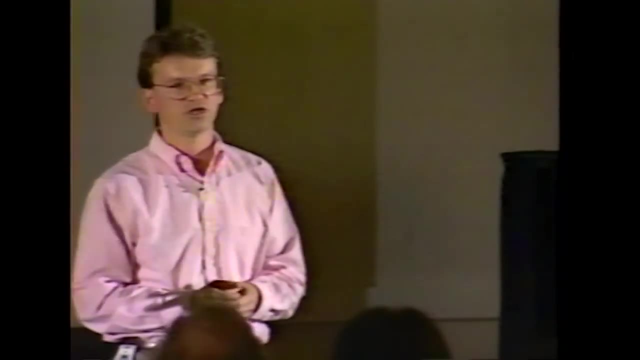 Were we able to really convince them that a consistent graphic user interface was a good thing to have. I want to fast forward a little, skip through the early years of the Macintosh and go to a tape that I dug up from the Apple library of some user interface testing. 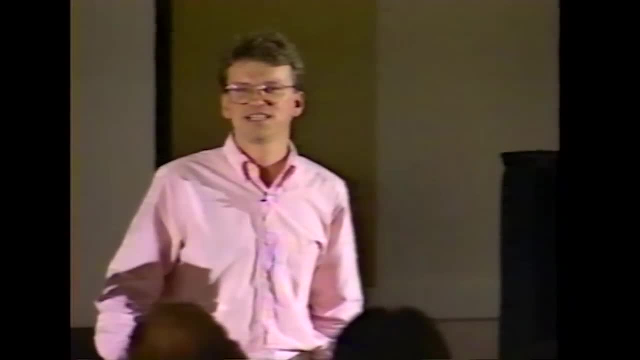 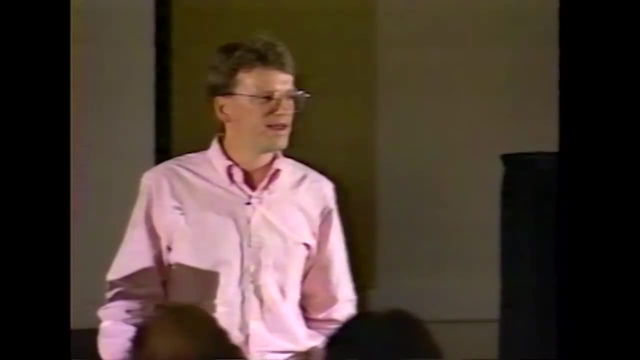 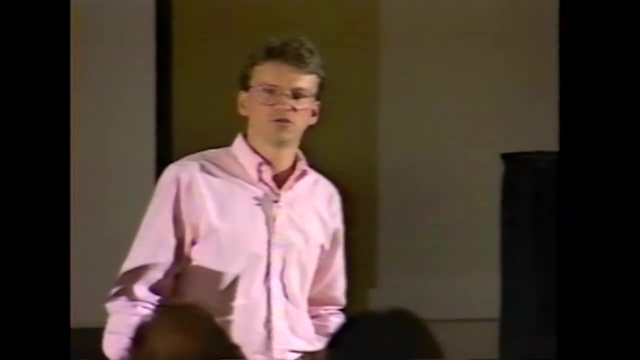 that shows how amusing user interface testing can be in the kinds of situations and far-flung places that members of our glorious human interface group went to find the truth about what real users would do. And this is a tape of a couple of our user interface designers. 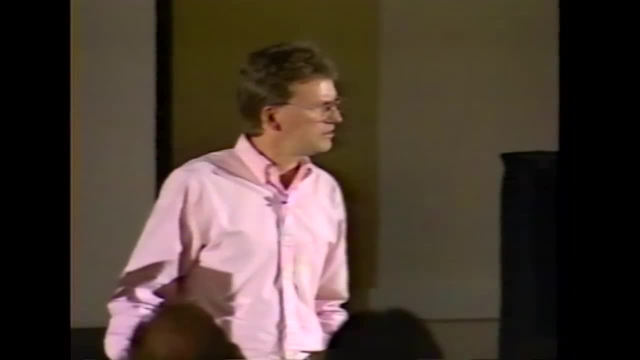 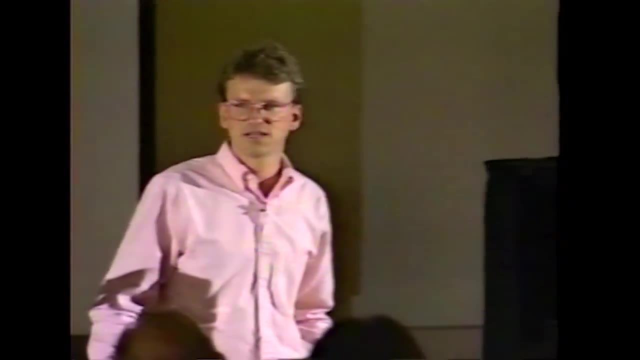 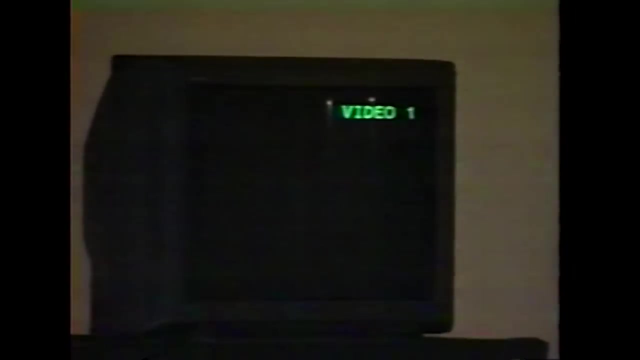 Laurie Vertelny and one other person- I may come up with her name, I don't think it was Gita- traveled to France to a parts dealership for Renault automobiles who were deploying a new automotive parts catalog based on HyperCard, and HyperCard being a. 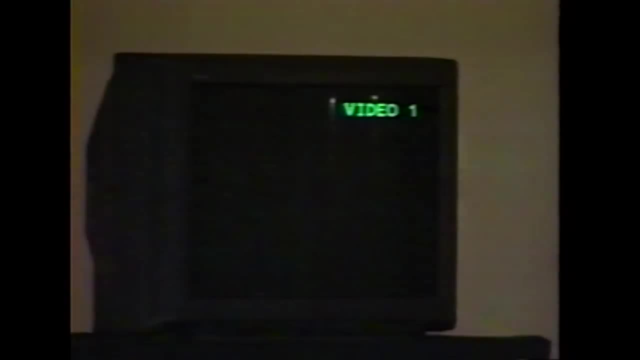 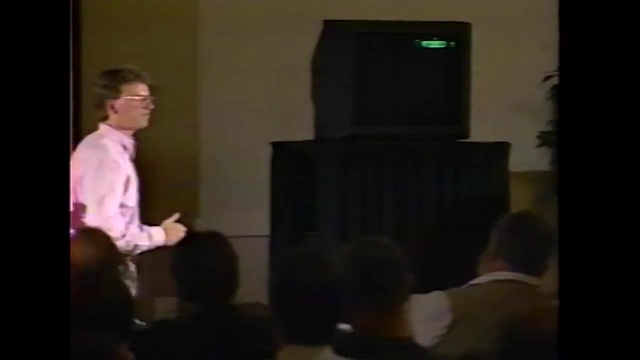 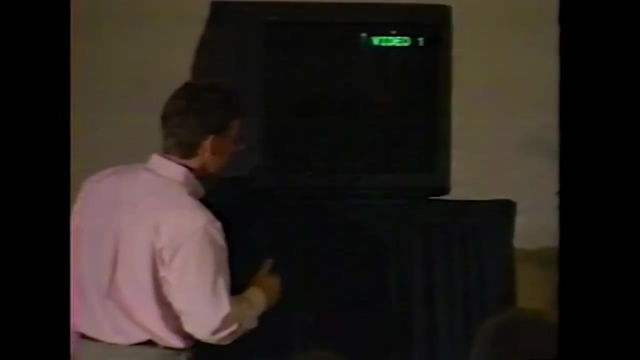 a free-form tool kit for designing new software interfaces, presented an entire raft of new problems in human interface design, and they actually went to France to test auto mechanics in their own environment. And I'm going to play that tape for you now. Yeah, I'll turn it on. 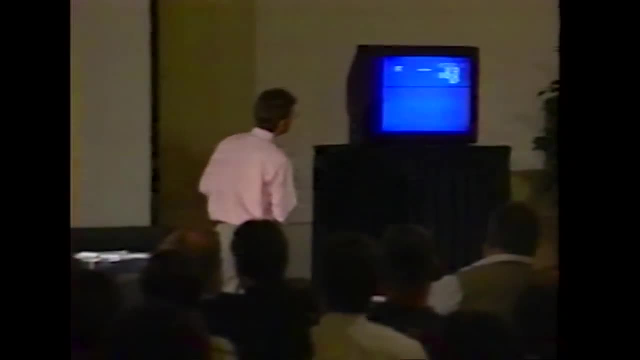 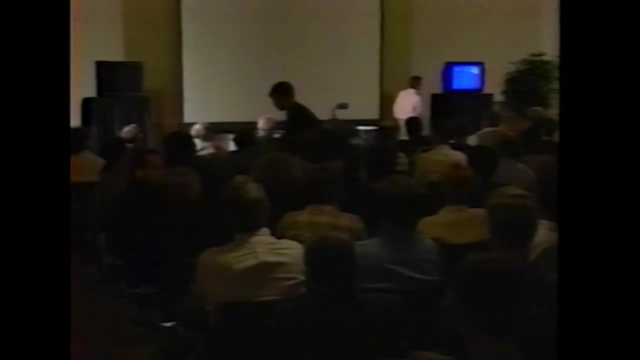 It might have been Kate Gamal. yeah, Okay, Thank you, Annette. Was that Annette? Oh, it's Joy, Hi Joy. Okay, You can see, Annette. Yeah, okay, this is the part. The first part of the user test was to test users attempting to fill out an order form. 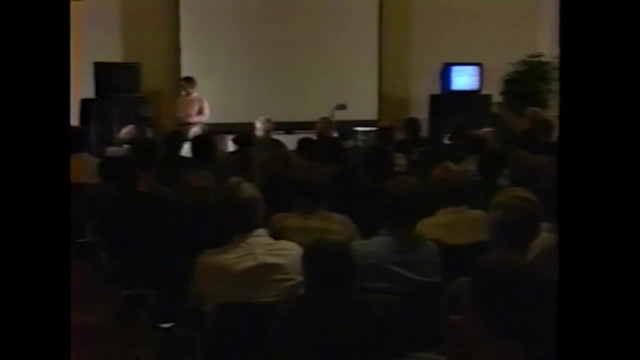 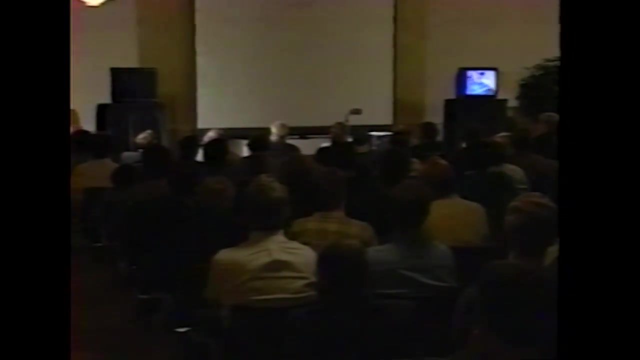 and estimate form using the current paper methods. These are the order and estimate forms that the mechanics currently use. The vehicle heart catalog is a catalog of the vehicle heart. The vehicle heart catalog is a catalog of the vehicle heart. The vehicle heart catalog is used to look at heart information. 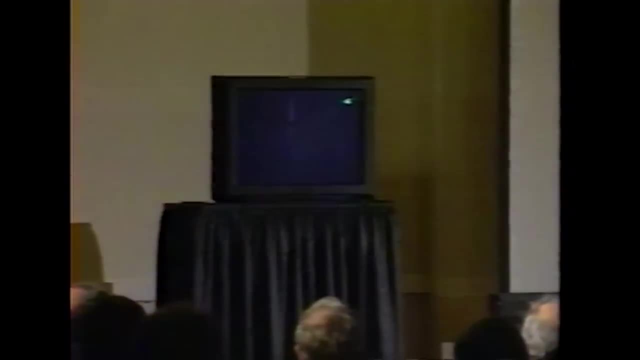 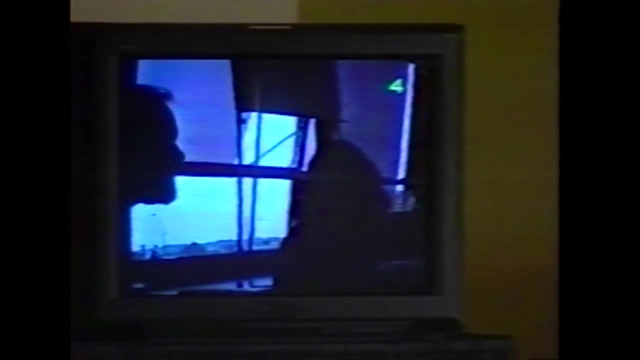 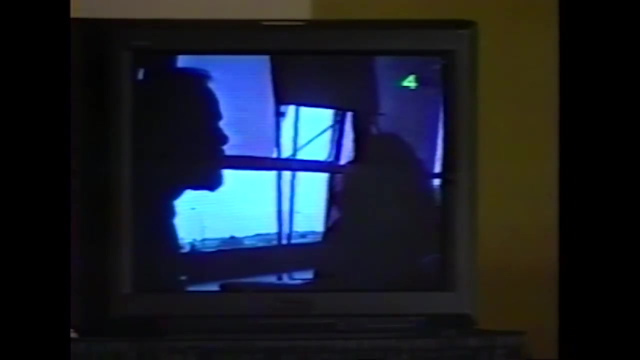 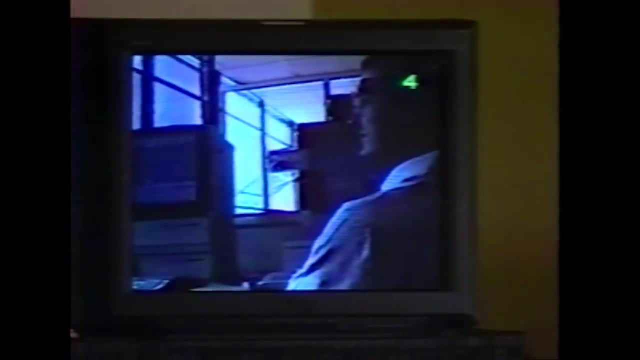 And the repair manual has instructions on how to repair the car. Kate explained the testing procedure and the task to be performed in the tent. All of her instructions were interpreted in the tent because Kate didn't speak French. If you have trouble with some of the tasks, it's the systems fault, not yours. 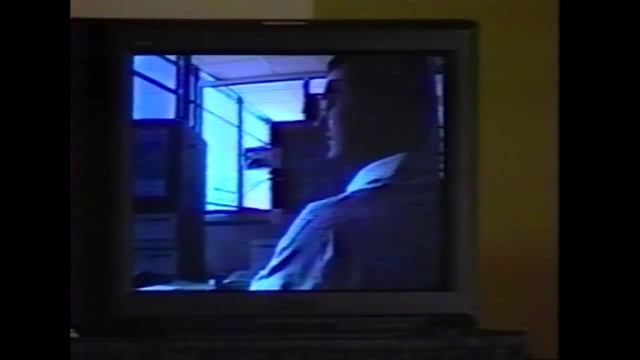 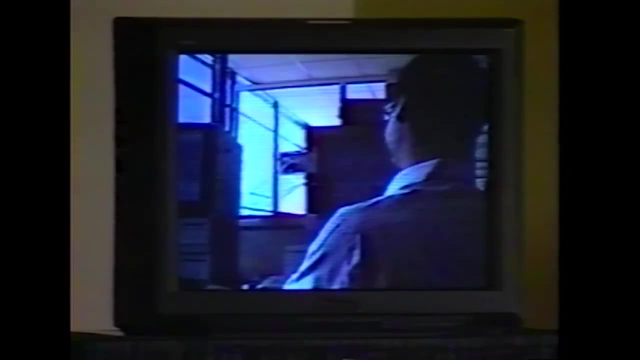 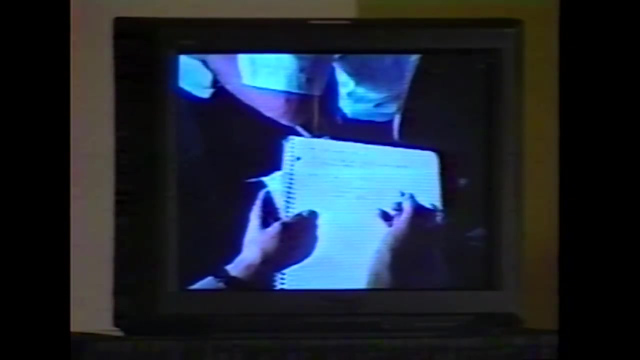 Thank you. If you happen to feel any difficulty in the system during the test, it is necessary to re-design it for the future. Congrats, the mechanic has attempted to perform the task. Kate took notes that would help us evaluate the results later. I will be out here for the test session. 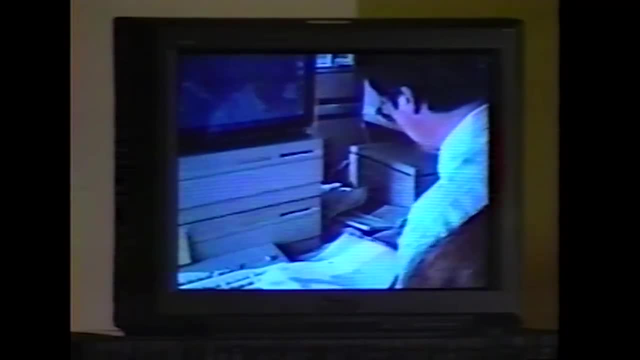 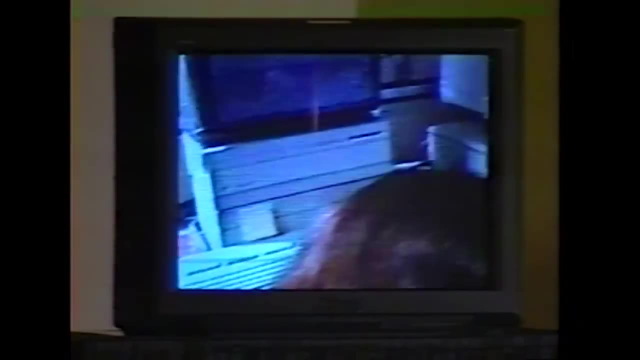 Seeing the mechanic work with the paper helped us to understand how he preferred to view the information. For example, he stacked the forms on top of the catalog and flipped through the pages while he was searching for information. These search techniques helped us to make design recommendations for searching with the electronic version of the form filling process. 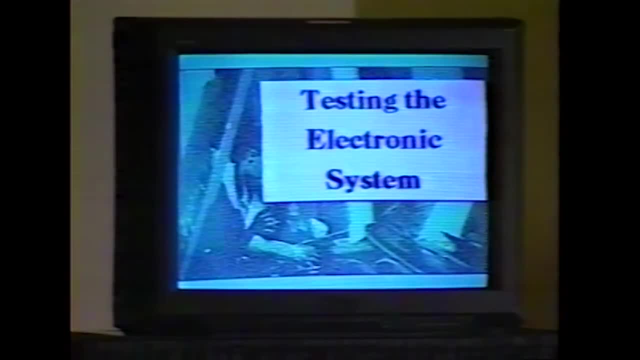 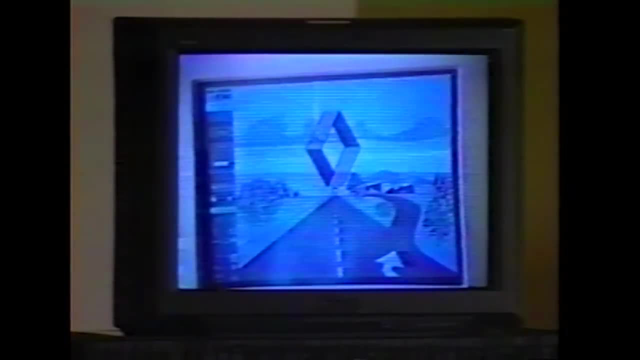 Once we had finished testing the current form filling procedure, we asked the mechanic to solve the same problem with the documentation electronic system. At this point in our test, the user has tried for almost 10 minutes simply to start the system. Kate finally did it. 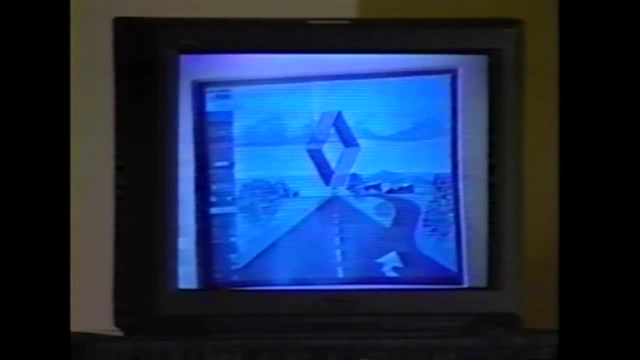 Now he instructs the user that he must click on the tiny icon below the Renault logo to start the system. The interpreter wants to know if he should explain the pop-up menu that lies below the start icon, and Kate says no. The user clicks on the icon, knowing nothing about how to use pop-up menus, and then initiates a dialog box which explains to him that he needs to hold down on the icon. 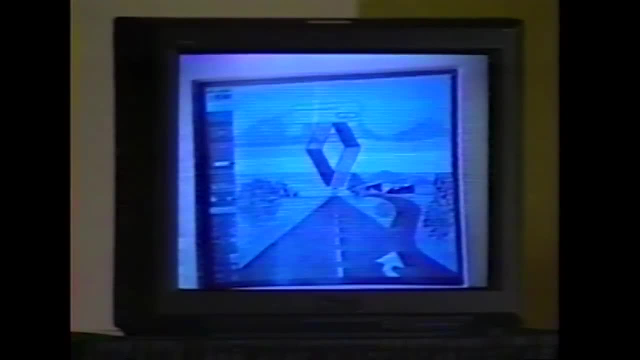 Of course, the mechanic has never seen a dialog box before and is confused not only about the message inside of it But about what to do with it. He finally realizes that he must click on OK to get rid of it. The user tries to start the application and clicks on many of the buttons in the menu to the left of the screen. 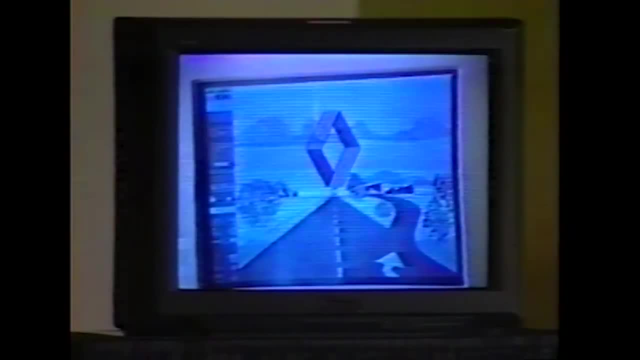 Unfortunately, none of the menu items work at this point because he has not filled out the appropriate vehicle identification. to actually start work session, He tries a small icon in the center of the screen. Apparently, once again, he breaks up the dialog box and tells him to hold down on the icon. 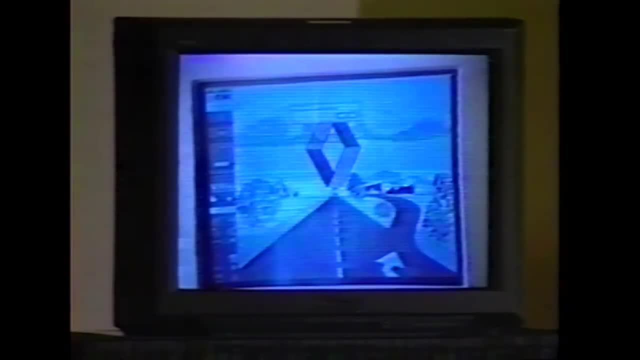 This time he doesn't see that he must click on the OK box. He starts clicking around the screen. Did you hear the system beep? Finally, Kate instructs him to kind of hold down on the button in order to start the program. He misinterprets this to you and holds down on the OK button in the dialog box. 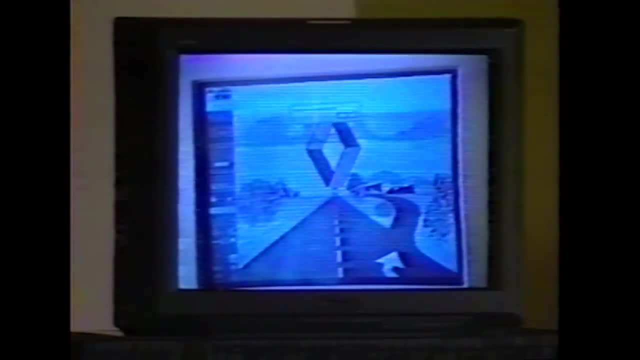 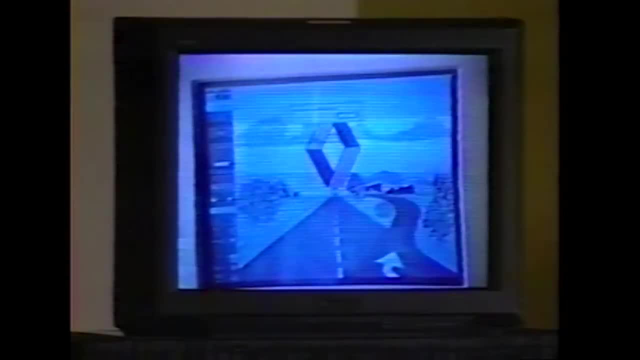 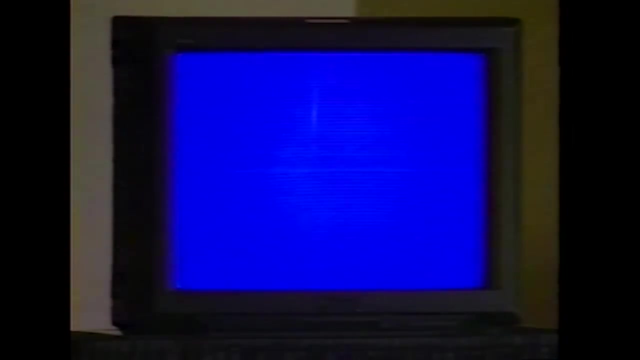 He tries to open the dialog one more time, but again it brings up the dialog box. He tries to open the dialog box. So that just, I think, is an illustration of two things. One, that bad design knows no bounds. 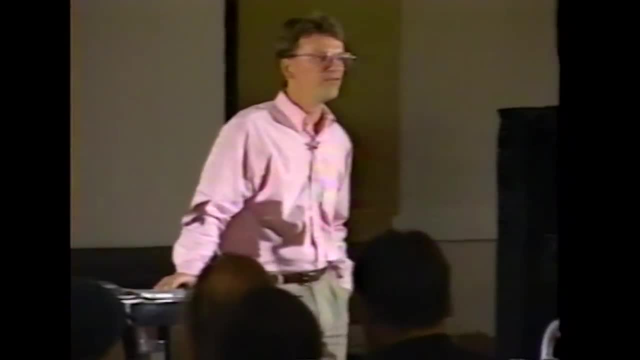 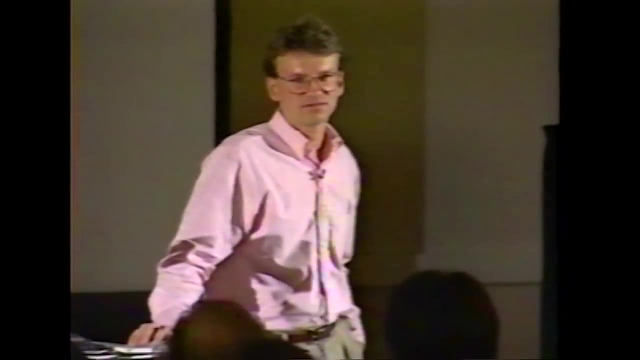 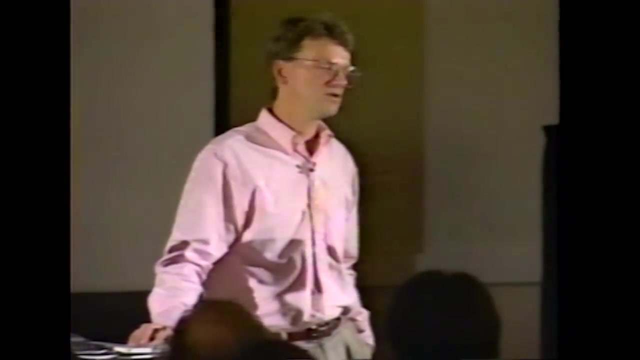 And two, that you never get a user interface right And that user testing from the earliest times, when you have a totally unsaturated market of people who've never seen personal computers before, much less mice keyboards, screens, things like that. 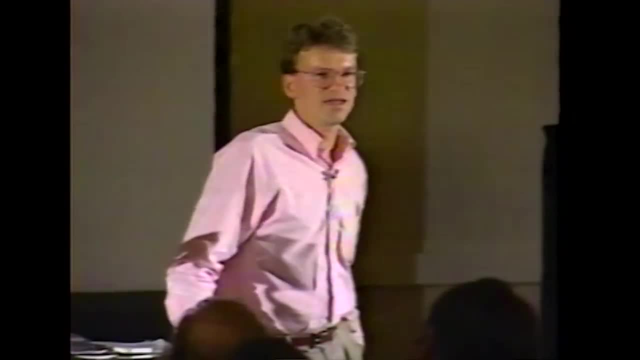 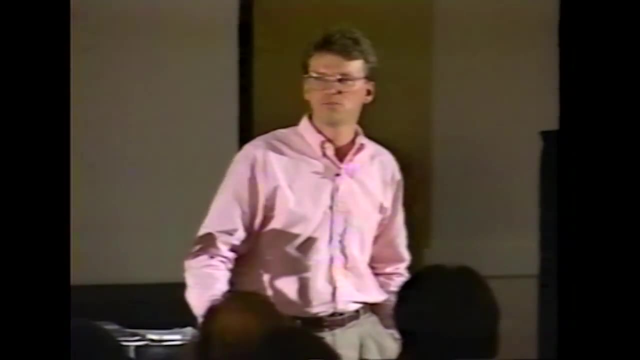 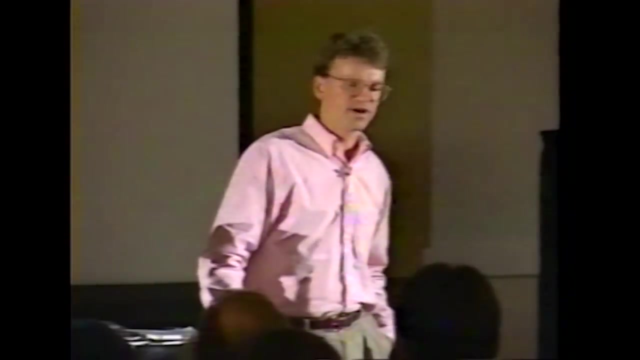 to today, when we assume that anybody who's ever been in Western society has had to have encountered a personal computer at some point And knows the basics of pointing, clicking, dragging, pressing what a file is, what a document is, how to print, why. to print what a floppy disk is. 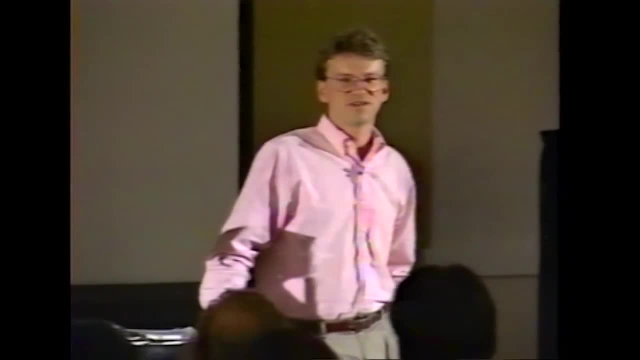 I mean, I still find it surprising that we don't talk about sectors and cylinders anymore on disks, which was one of the main things we had to explain in 1978, 1979. Because there was some reason. you needed to know that. I forget why. 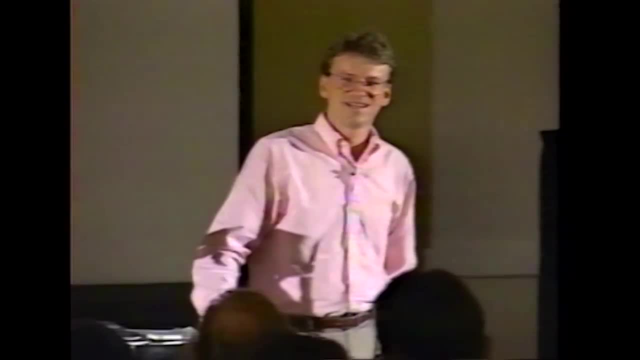 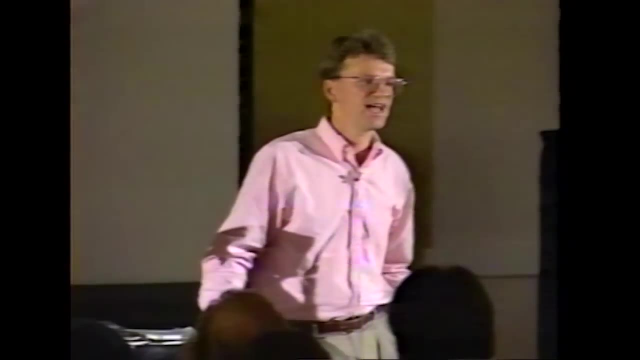 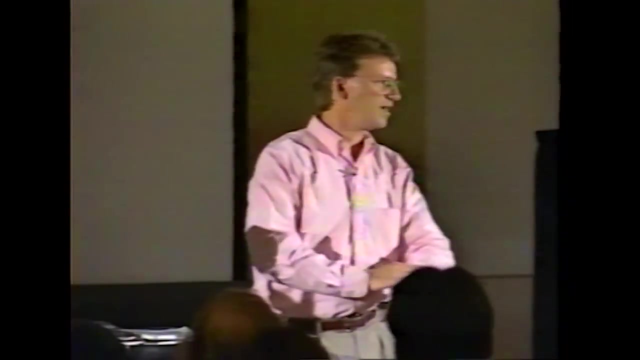 But, yes, But that some things never go away And that having to test new designs and test your assumptions of what your audience knows is pretty much eternal. So at that point, having run pretty late, I think, Larry and I will take a few questions. 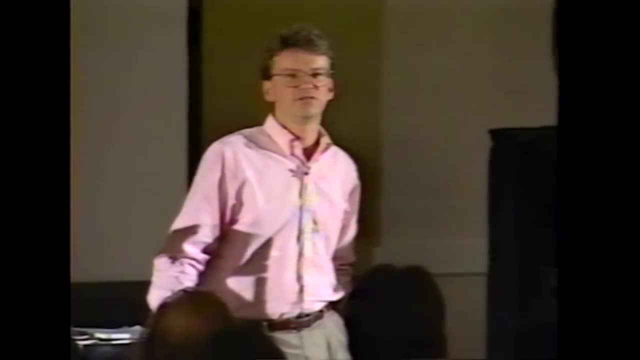 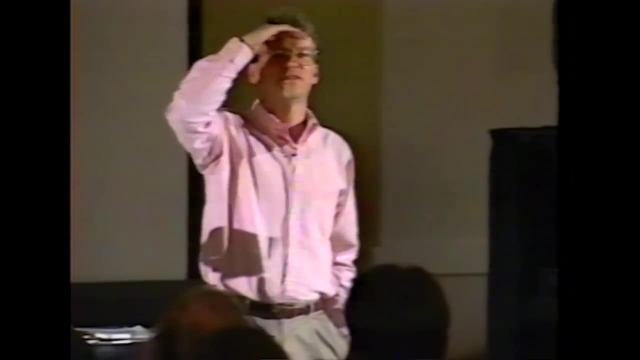 And I think that we are going to take free liberty to defer to several people in the audience who are noted in Apple Human Interface history. I see Joy Mountford and Annette Wagner back there who've been instrumental in human interface groups in the past. 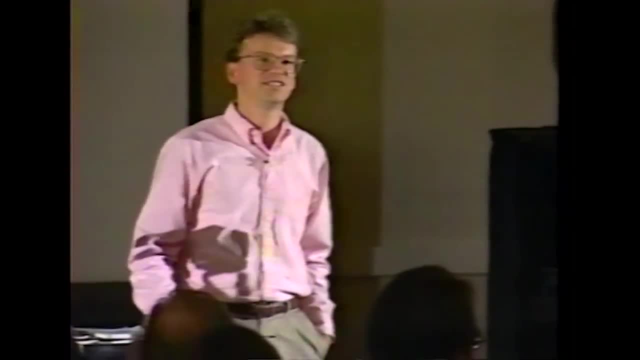 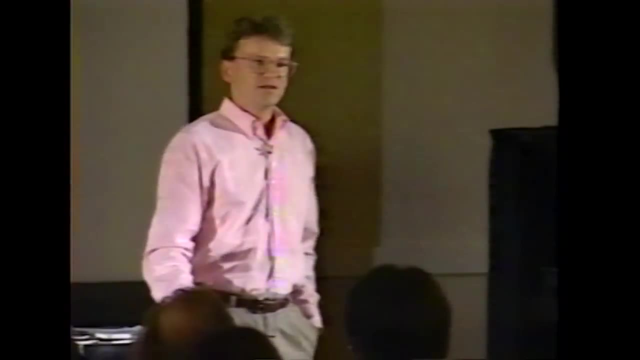 And if there are any others and if you have strong opinions, disagree with us. have more information than we're able to supply. please chime in. And, Larry, do you want to pass the mic around so people can ask questions in the mic? 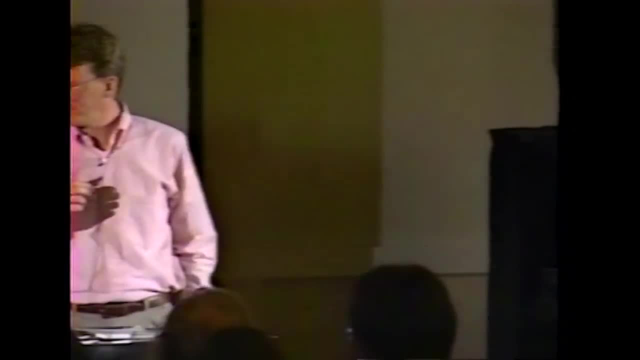 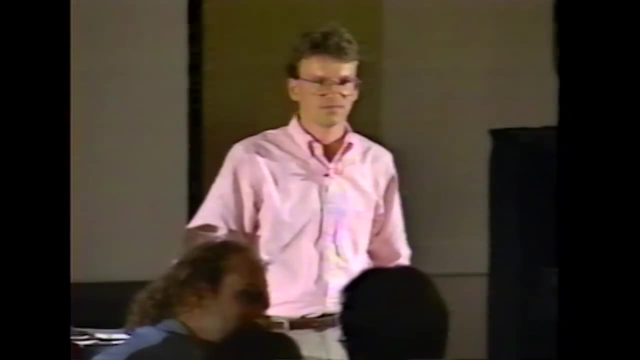 I think we'll just repeat the question. Okay, Hello, Hello, Okay, that works. Well, you're close enough Here, Larry. I wonder if you could comment on on the story that's often told that Apple ripped off the Xerox PARC work. 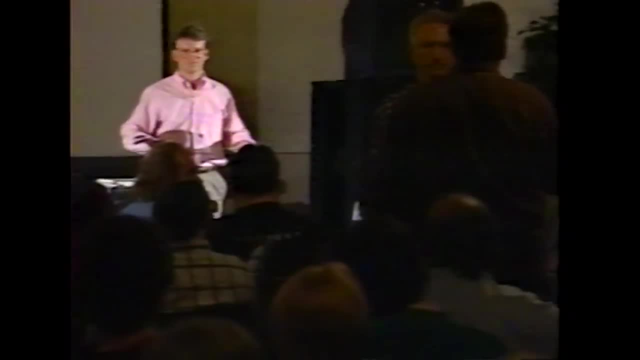 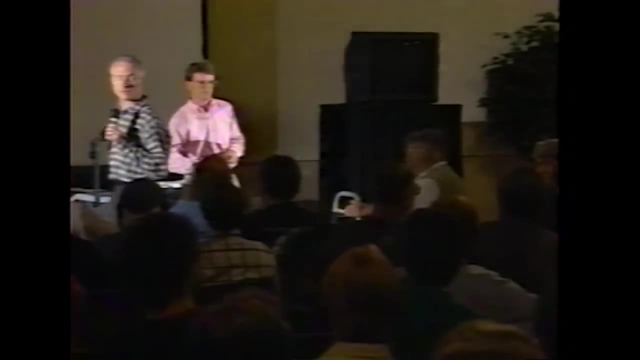 I know Jeff Raskin has refuted or denied that, but it's such a popular story. Could you go on record as giving your perspective? Yeah well, I actually showed at the beginning of the talk a picture of the Smalltalk interface to see that in fact. 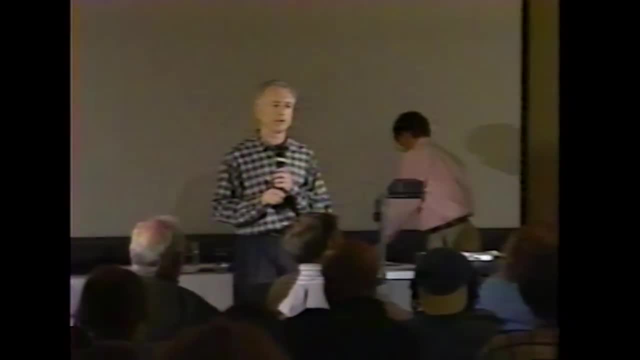 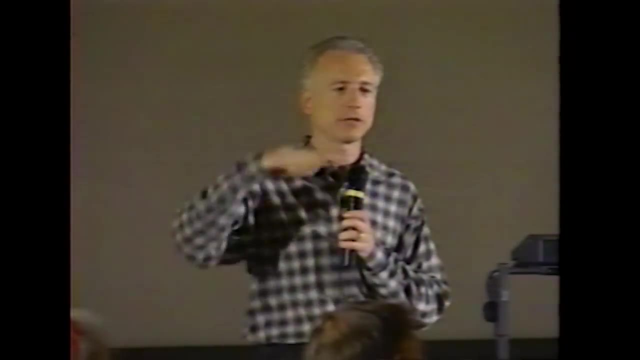 the early user interface designs were very close to that- The look of the windows in particular and the icons in the desktop. But it evolved over time and you know, the menu moved to the top, The screen and so on. 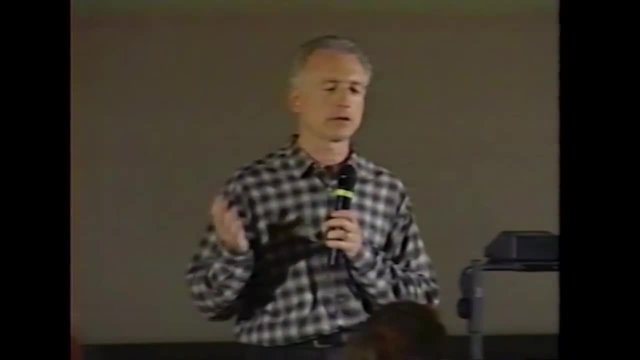 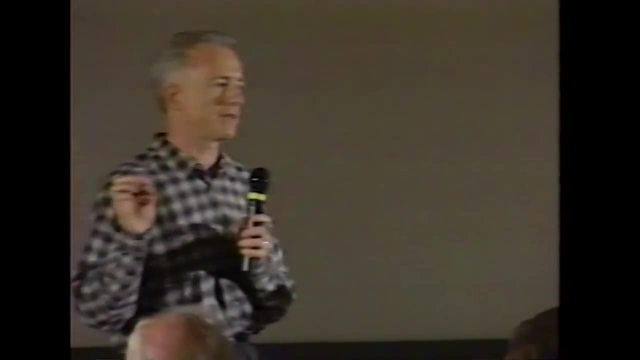 If you actually look at either a Xerox STAR or a Smalltalk screen and then look at a Lisa or a Mac, I think you'll see a lot of differences. What was taken was the concepts, The concepts that there ought to be overlapping windows. 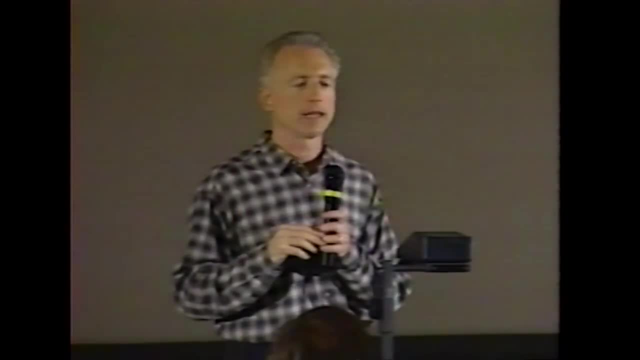 that there ought to be direct manipulation and so on. But the Xerox STAR, for example, didn't have the concept of dragging things And it had two-button mouse. You'd click one place and then click another place. It didn't have a menu bar. 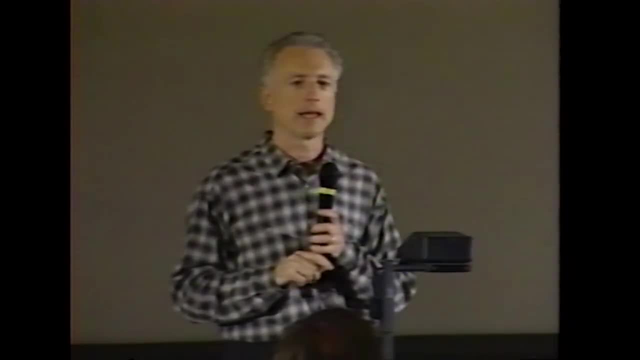 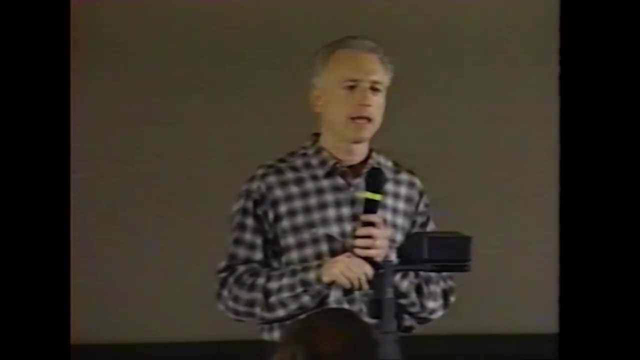 In fact there was only one menu that was added late in the development And it you know. but some things were similar. There was a horizontal and a vertical scroll bar, So certainly the concepts came largely from there, But, as you see, some of the concepts came from other things. from HP systems, UCSD, from Apple II, from some work that was done at IBM that I didn't talk about today. that was published around the late 70s, So there were a lot of origins for it. I think Xerox work had a lot to do with it. 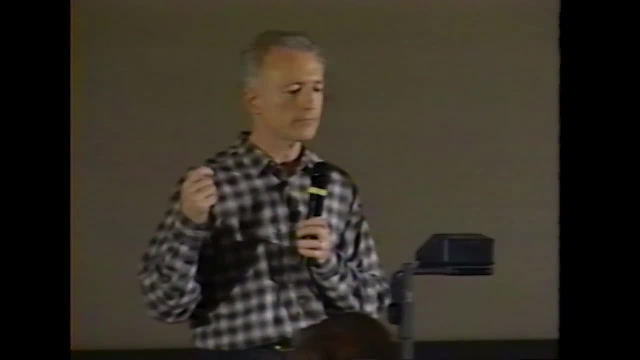 But usually when you're working with a computer, you're going to have a lot of problems. You're going to have a lot of problems. You're going to have a lot of problems When the if you sat down to try to use a star or a small talk. 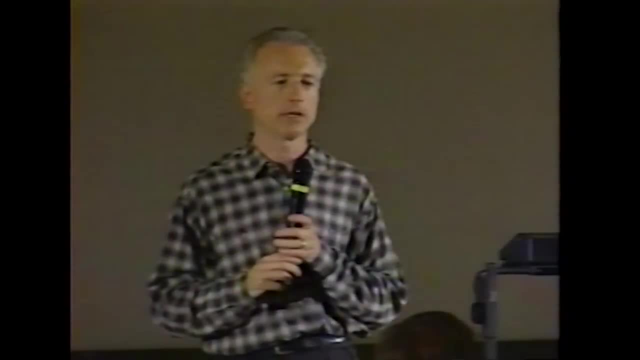 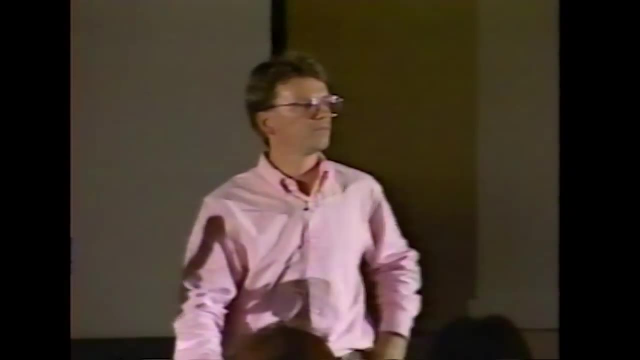 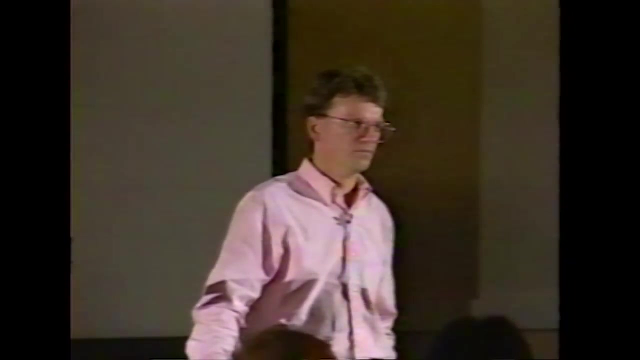 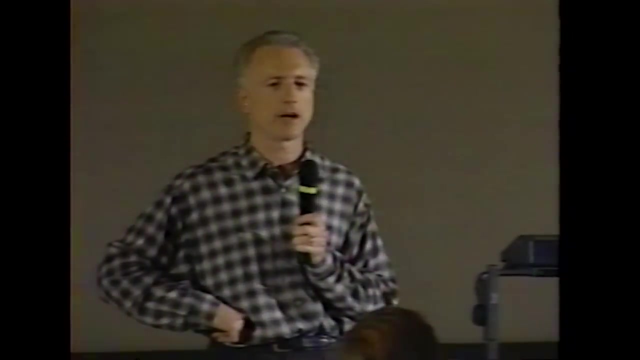 you would find that there were, I think, more differences than similarities in what you would actually see and do. Yeah, go ahead. The question is: the user testing we showed for the Lisa had to do with novice users And the question was whether we tested for how people acculturated. 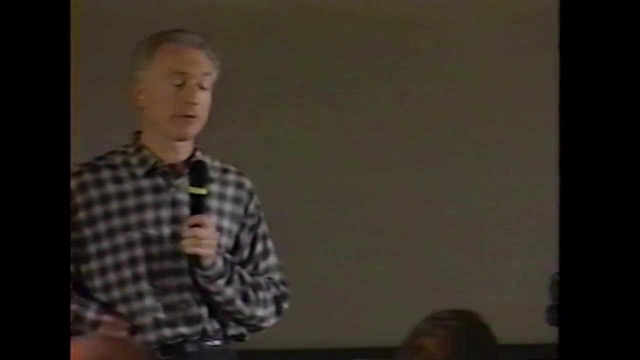 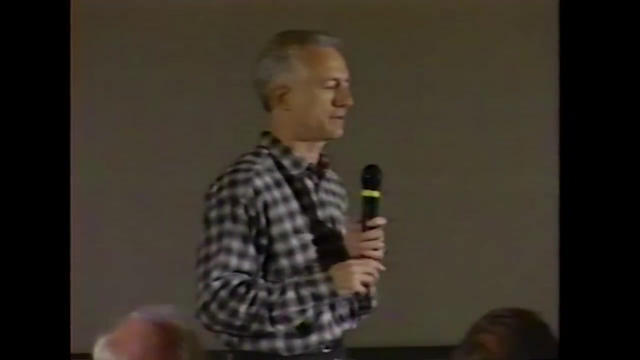 over time. Well, the system, remember from the very first page of the User Interface Guidelines, Bill wrote- was targeted at novice users. That was the target, which was about everybody in those days, And we did have some theories about how people would you know? 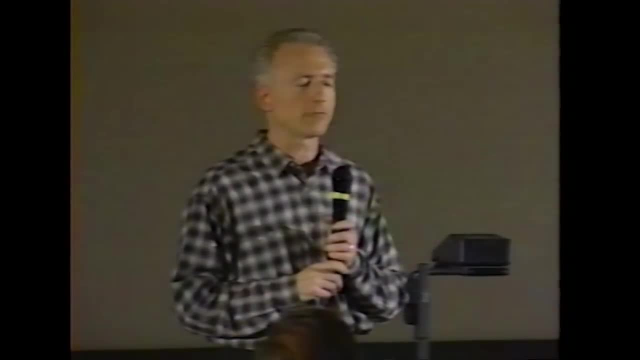 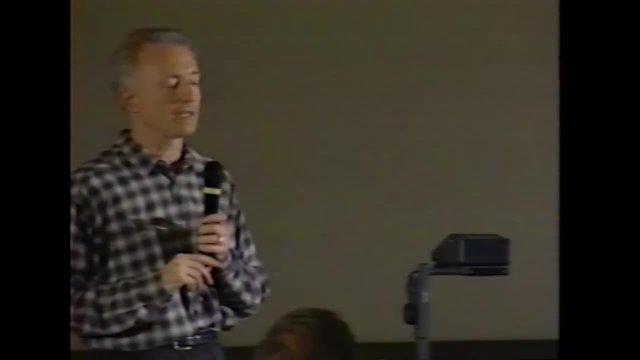 use command keys as they got more expert and so on, But we didn't run user tests. One reason we didn't was because it would have taken a long time to get people up to speed. So what we did was we just used kind of ourselves. I don't mean anybody. I don't mean anybody. I don't mean any engineers, But people who worked in the Lisa division, who had Lisas like people in product marketing. they became expert after a while And they would start telling us that things were too slow or too hard or whatever. 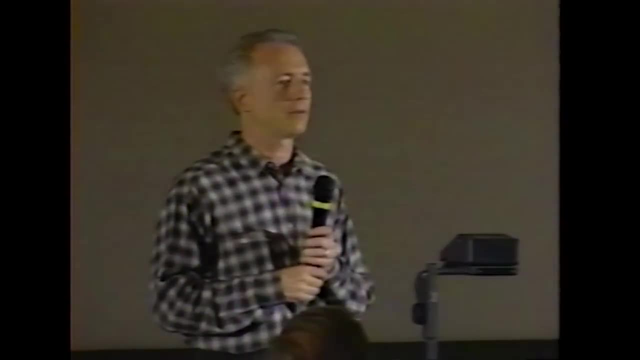 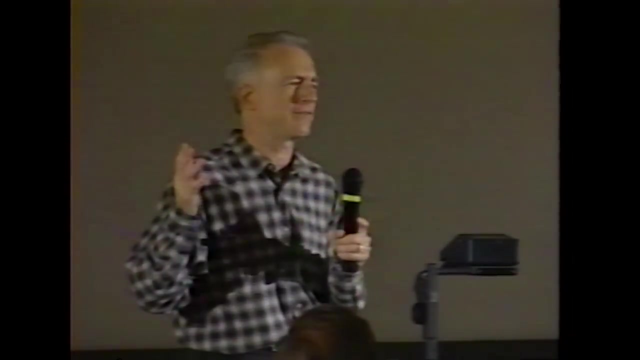 And that's how we got that kind of feedback- just from people inside, And I think it's more relevant today to check for those sort of things than it was back then when everybody was, you know, 95% of the people were novices. 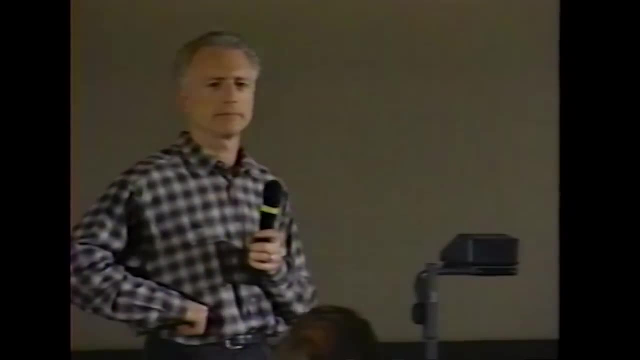 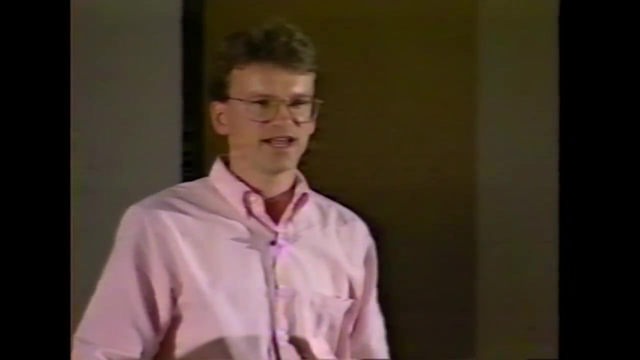 One of the constant tensions- and this was true on the Macintosh as well, especially because we had the benefit of the Lisa Lisa worked before us and some of the Lisa machines- was the constant tension is that the people who are designing are almost always by definition. 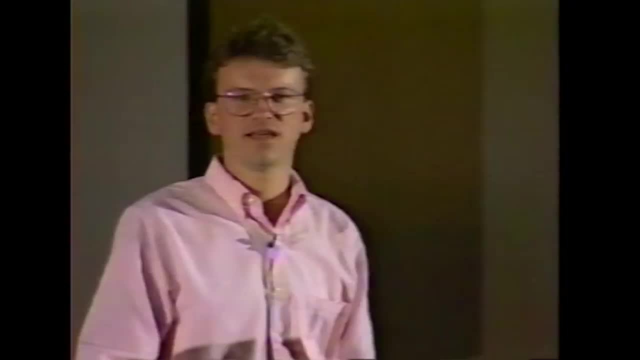 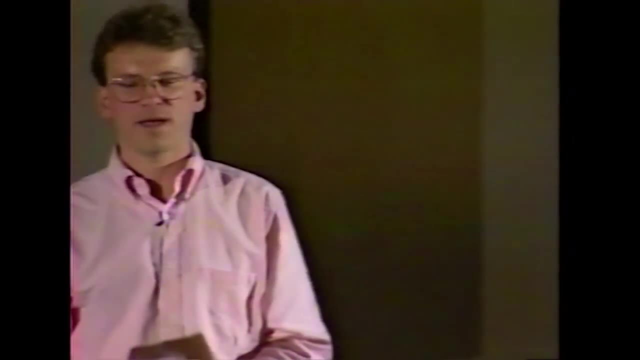 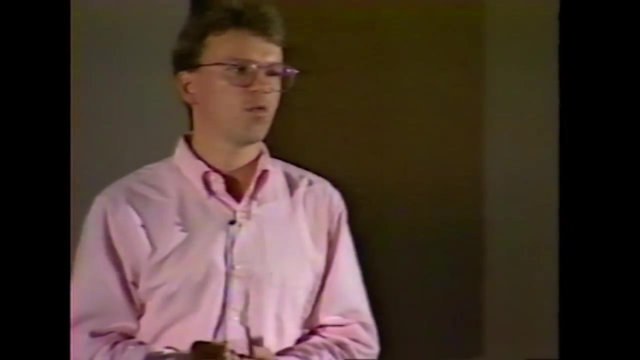 expert users and will often overlook that what they think is obvious is not at all obvious to a novice user. And so there's constantly the dilemma- which you've seen historically in Mac system software- that the expert users want to put in the features they want to use. 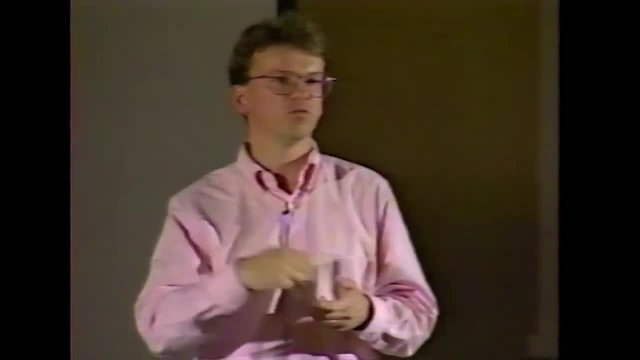 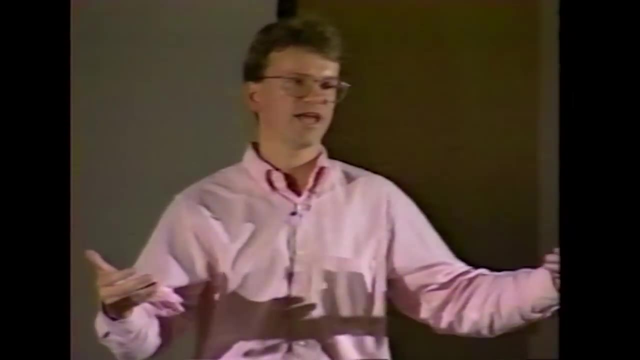 but the people who want to keep the system pure for the novices want to resist those. And if you're lucky, you get a system that is easy to approach for the novice and gradually unfolds itself for the expert, And if you're unlucky, you get a lukewarm mediocrity between the two. 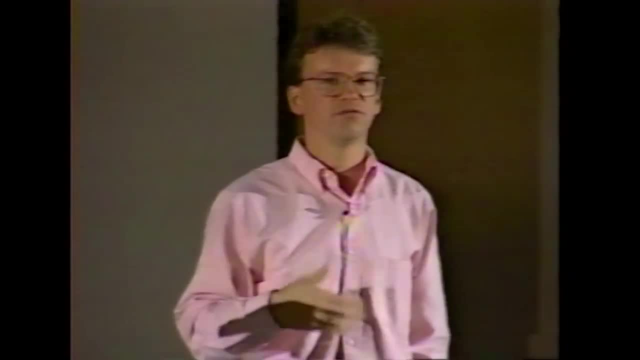 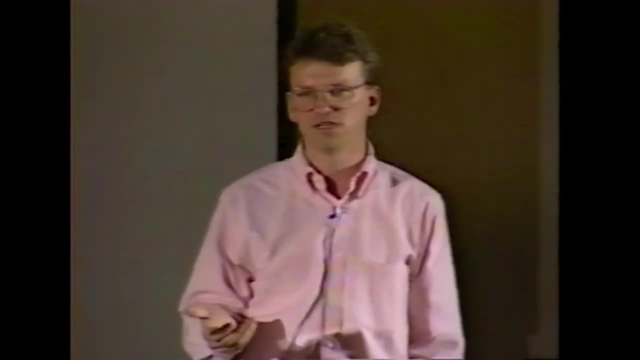 where it's a little too complex for the beginning user to understand but still not nearly powerful enough for the expert user, And some of our designs and some of the industry designs have been one gradually unfolding and others have been just plain mediocre. Awesome. 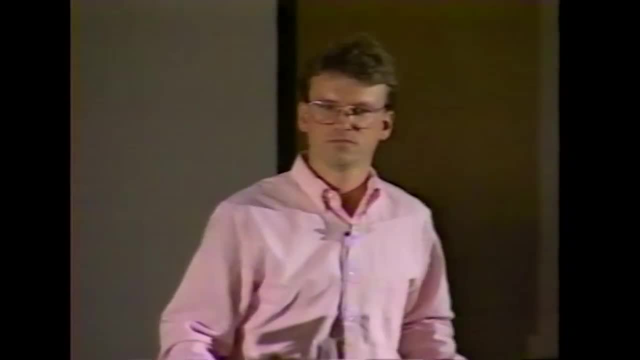 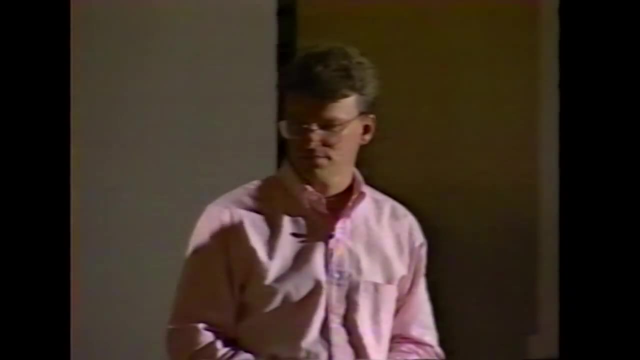 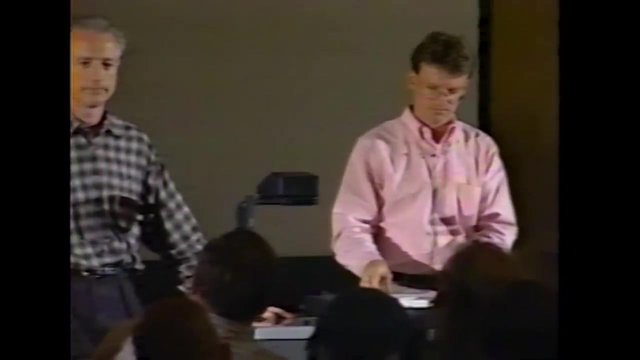 I have an observation and then a question. Larry and I have known each other for years And it's interesting to me that, for one thing, you folks weren't aware of the similarity to the WordStar commands that already existed in the WordStar editor for copy, cut paste kind of things. 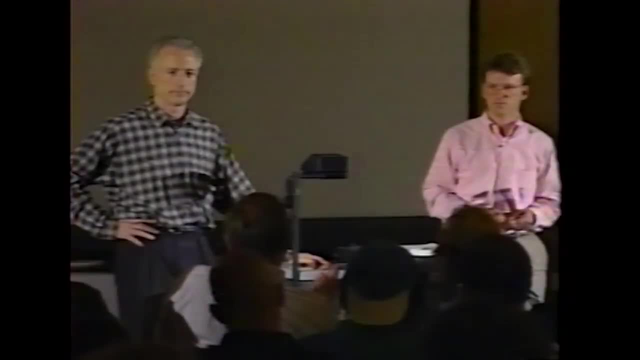 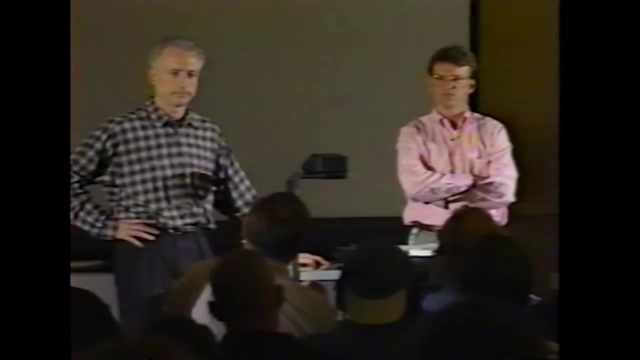 But also I think the word assumption is key And what you just said is very correct. People assume that, as they're developing something, that they know the best way to develop it, rather than go outside and get other information. You know one of the things that I've seen as a software person in the past. 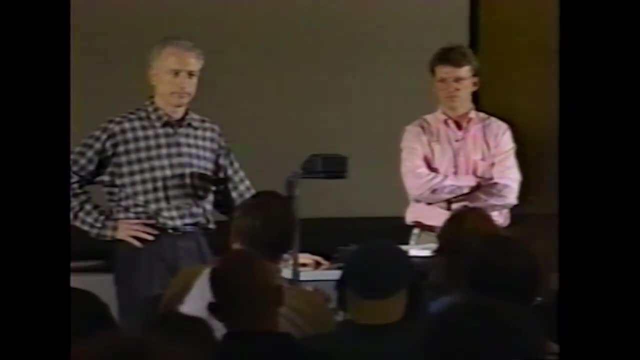 having to do work for people for money, so that they expect us to have something done by a certain time- not for a company that I'm working for, but for as a consultant- is that they really do expect the thing to work the way their people want it to work? 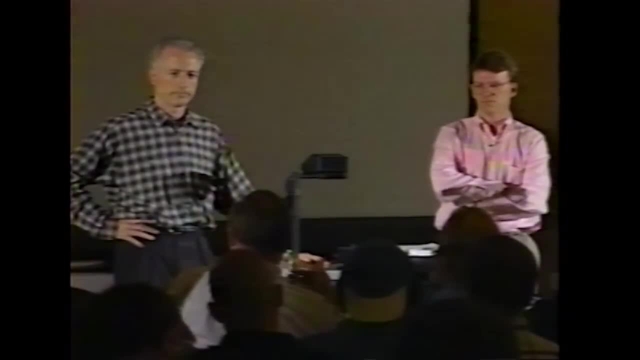 And there you have to really do a design review And all sorts of things with those people first before you get to the right setup, before you can actually start actually writing code. And one observation about the Lisa. that was very interesting when I first saw it. 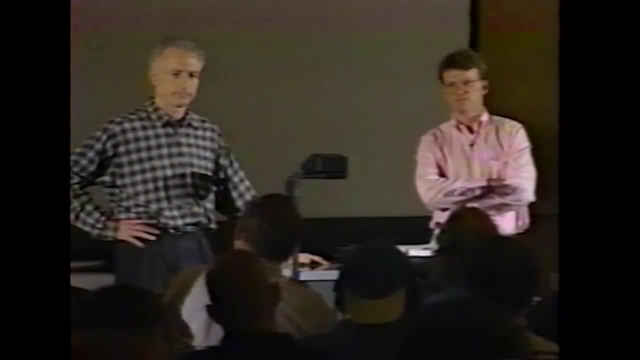 I first saw it, I think, at the West Coast Computer Fair in San Francisco. Steve Jobs was there. I don't know who else from Apple was there other than marketing staff, But I had gone there with a friend from Xerox And we looked at the star system. 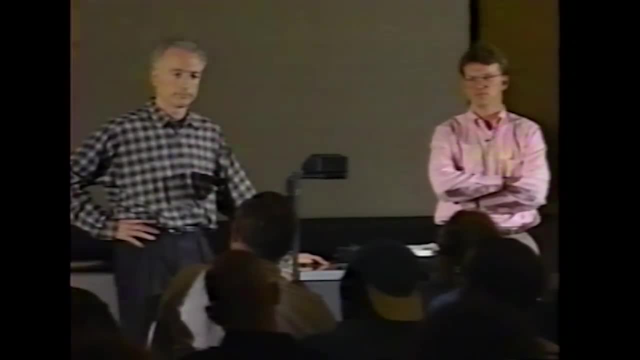 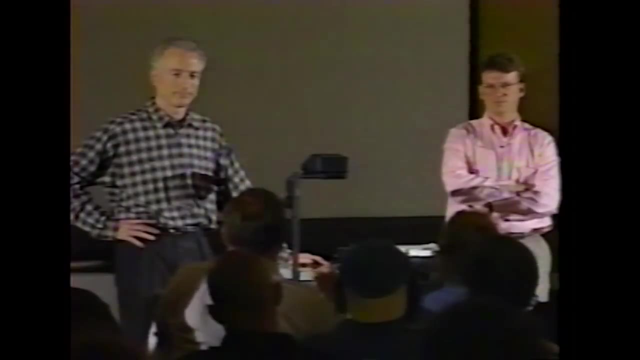 And we'd actually looked at the Fortune, which was the system, which was the first 16-bit personal computer that was available, And they had a very fancy, you know, display and so forth And everybody was looking at it And it was beautifully designed and everything else that it ran CPM. 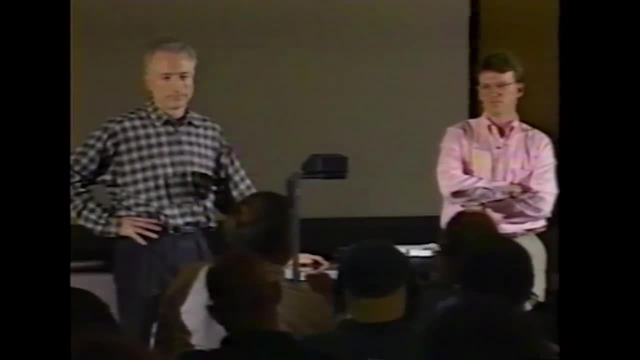 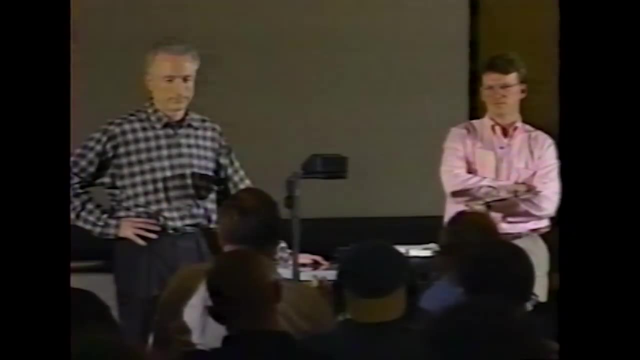 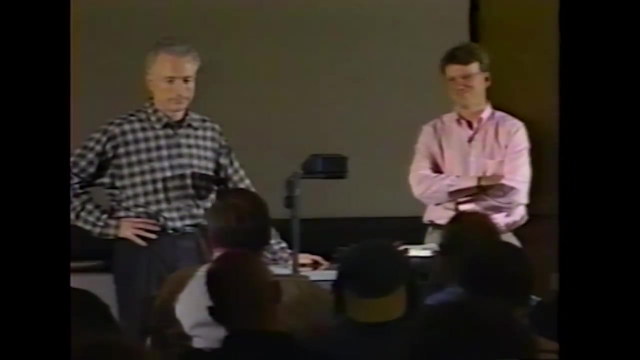 and Unix, a version of sort of Unix. There was one test in the software work that we had done for real customers- you know who really wanted reliable software- that we'd accidentally come upon, Which was called the keyboard mush. You take your hand and you run it across the keyboard a few times. 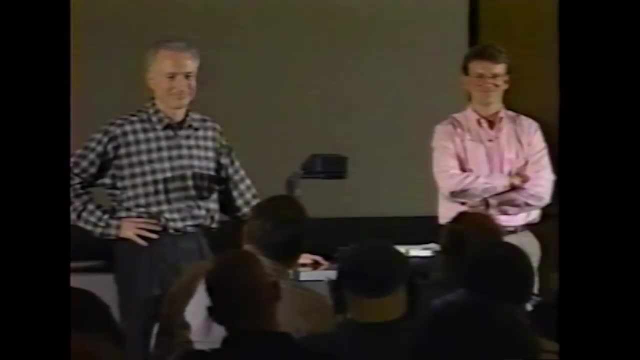 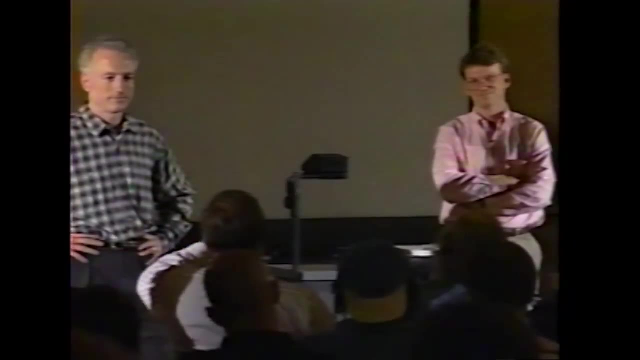 And you see if your software is still running, And I told this friend of mine from Xerox about it. So he walks over to the Fortune system on the big podium up there with the pretty girl standing by it And he tries it And the thing dies. 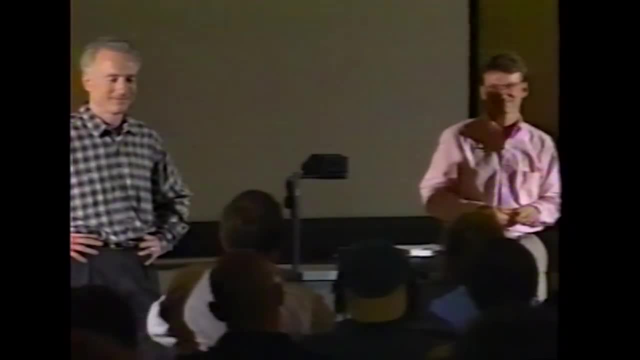 So we kind of sneak away And we go over to the Apple booth And there's Steve and the other folks there And we decided we weren't going to try it on the Lisa. So in reaching for a brochure, though, I accidentally touched the upper right portion of the Lisa keyboard. 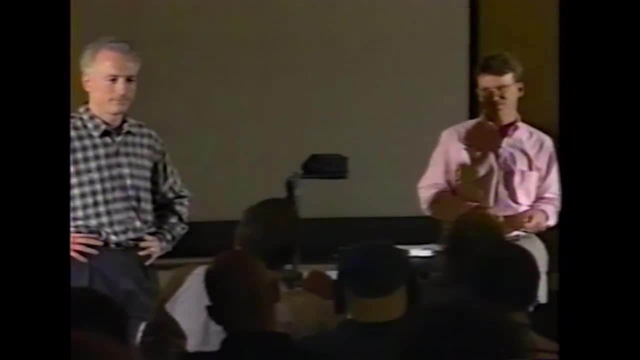 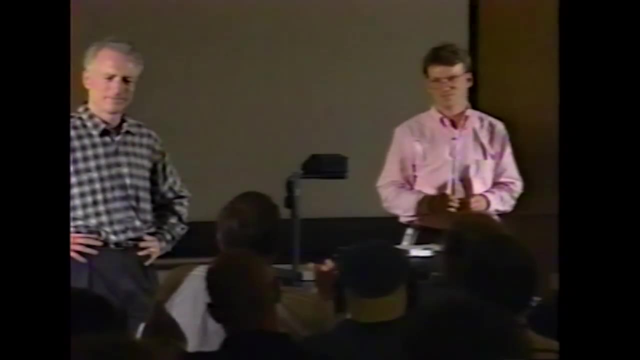 They were networked at the show for demonstration of networking. It brought down that Lisa. The guy helped me try to reboot it. It wouldn't come back. It also brought down all the other machines at the booth on the network And the only thing you finally could do was to power cycle the whole system. 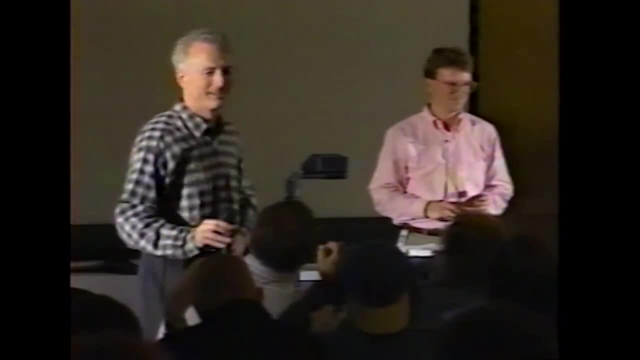 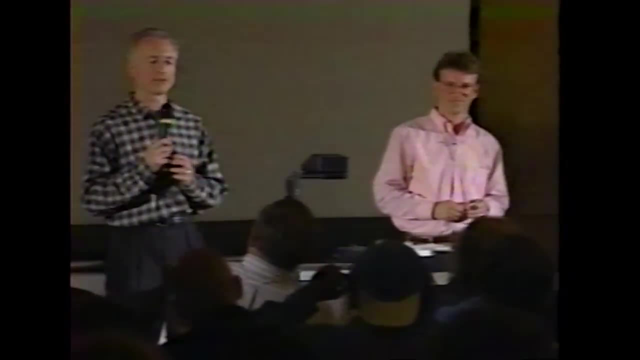 So I just wanted to bring that out. Well, no, I just wanted to bring out the power cycle. I wanted to bring out the basic nature of testing, which involves looking for the unforeseen. Looking for the unforeseen, Okay Right. 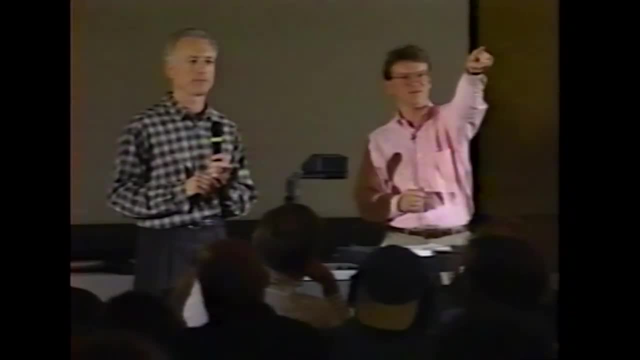 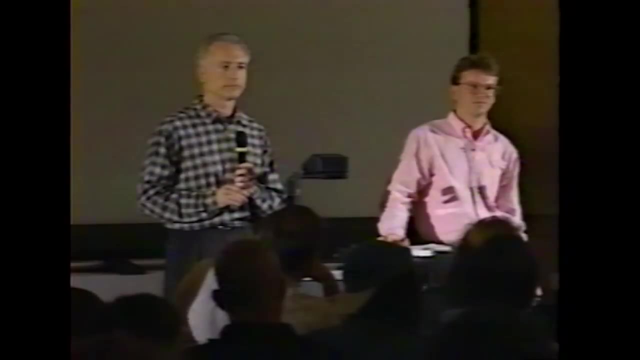 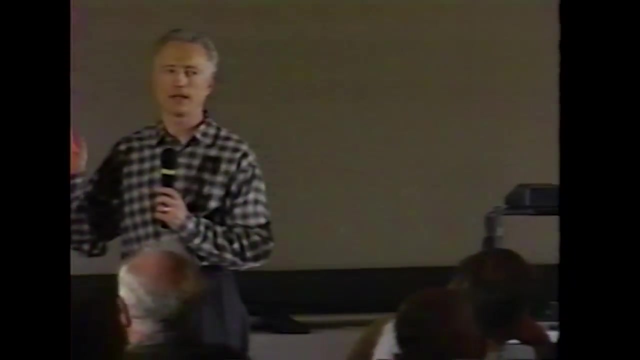 Good point. Just in the interest of time, we're going to try to keep the comments shorter though. Yeah, Yeah, Yeah, Do you see any relationship between the object-oriented programming metaphor and the three F's? Yes, The question is whether there's some correspondence between the object-oriented programming metaphor. 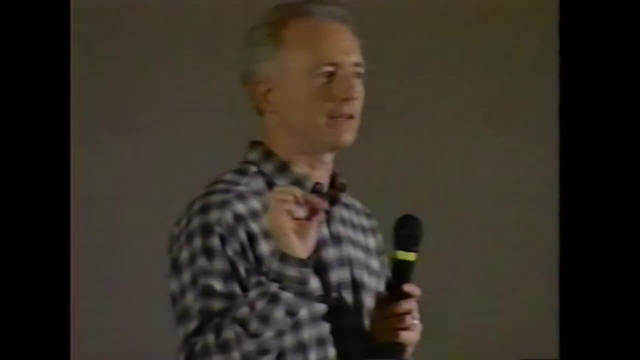 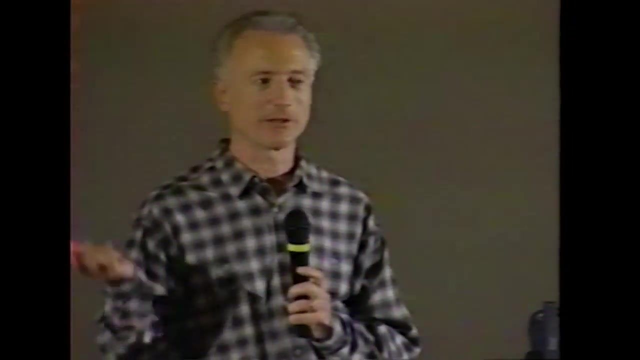 and the user interface metaphor. and yes, there is In fact in the Smalltalk user interface, which was one of the first of this type in the Smalltalk language, which was one of the first of the object-oriented type. the connection was very. 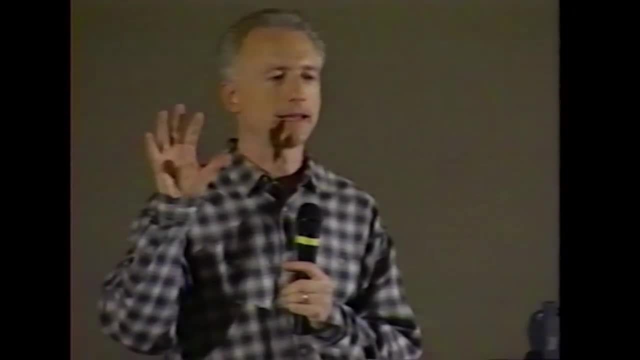 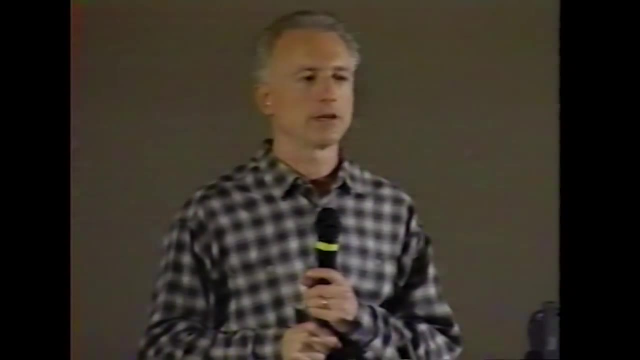 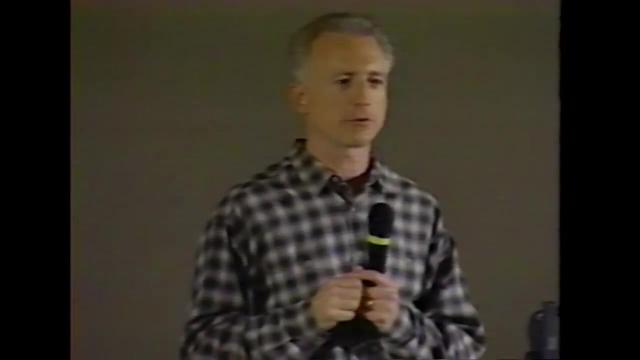 explicit that you had objects that had generic commands that could operate upon them, and that was something that existed both in the language and in the user interface, which was done even more so in the star. But we- definitely the programmers who were doing these user interfaces- definitely had. 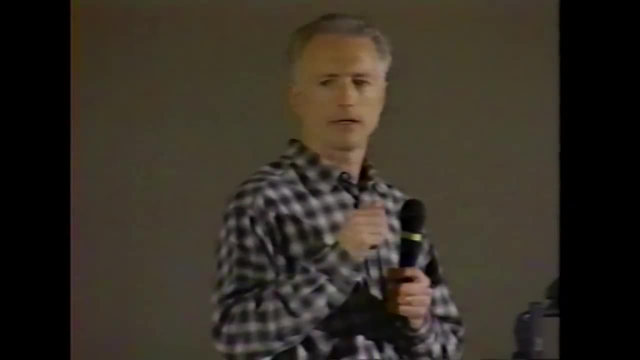 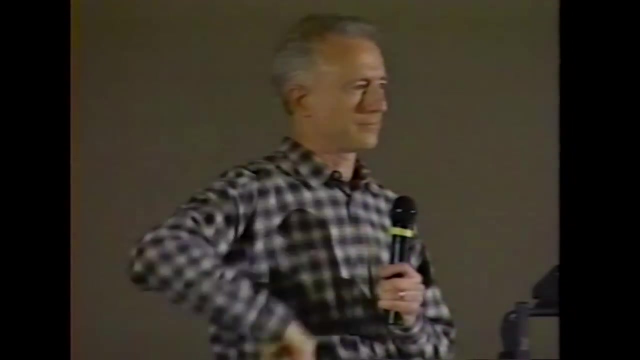 that in mind as a correspondence. Sure, John, John, John. I think there's some counter-examples on that, including NLS and Grail, which had great user interfaces for their time- graphed user interfaces that had nothing to do with object-oriented. 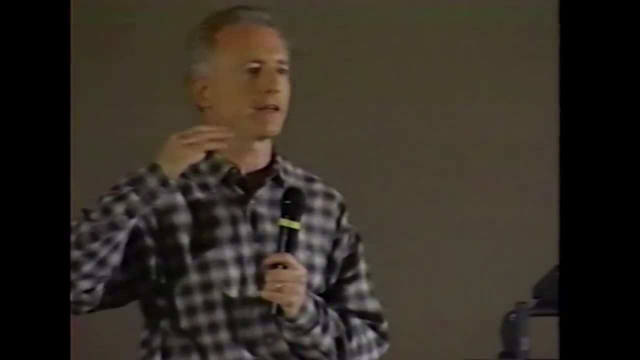 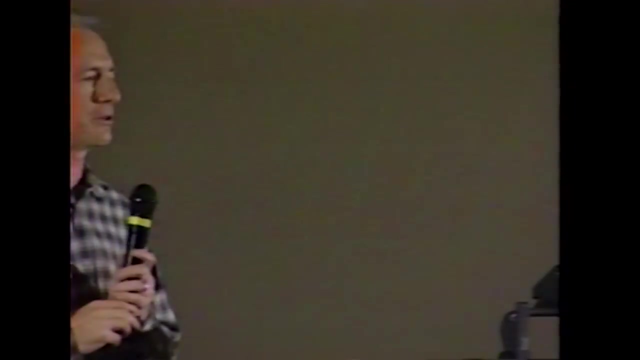 programming. Oh yeah, Good user interfaces don't have to. I'm just saying that the user interfaces that we were developing, we had that in mind. But the question is: But that doesn't mean that a good user interface has to be object-oriented. 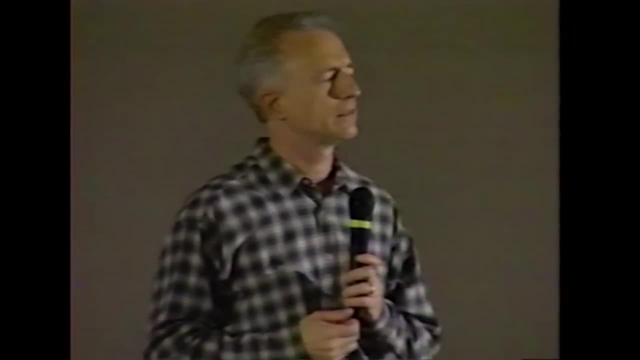 No, You showed two years of memos that you had written and received. Yeah, Having come from an environment with the Alto Bravo, Jitsi and Ears, what did you write all those on? What did I use to write the memos? 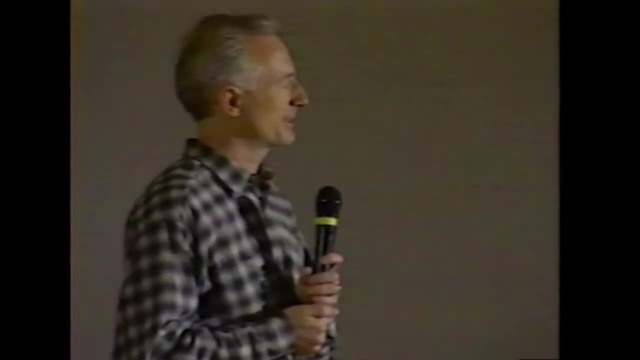 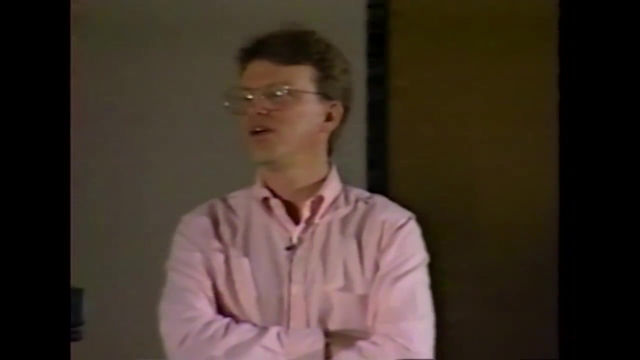 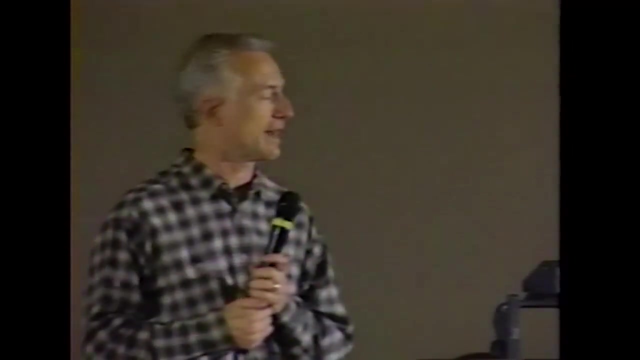 Okay, question: Probably Apple Writer. Let's see, Early on we were using Maybe Apple Writer on the Apple II or maybe UCSD Pascal Program Editor On an Apple III Being abused on an Apple II. I never had an Apple III. 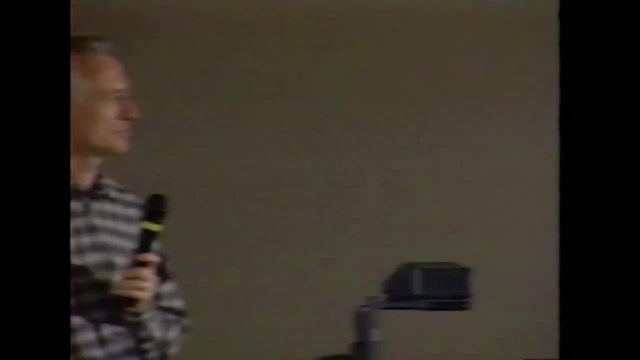 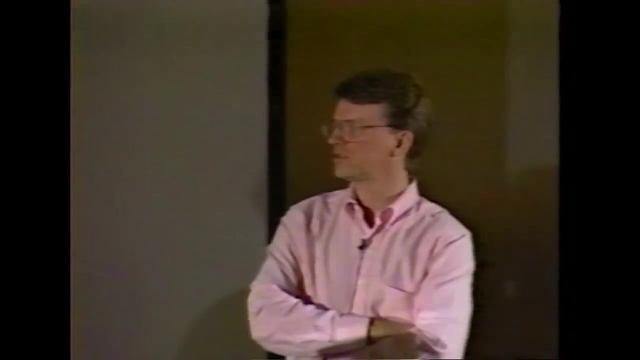 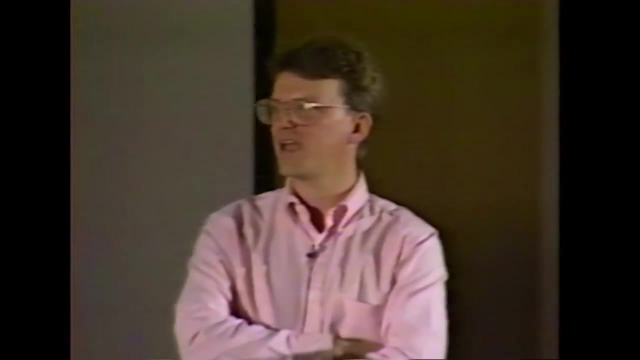 You're right. You were probably using either Apple Writer on an Apple II or sophisticated people used the UCSD Pascal Editor and output it using an NROF-like program called Apple Script Right. We output it to QM printers when we could afford the time and noise and to dot matrix. 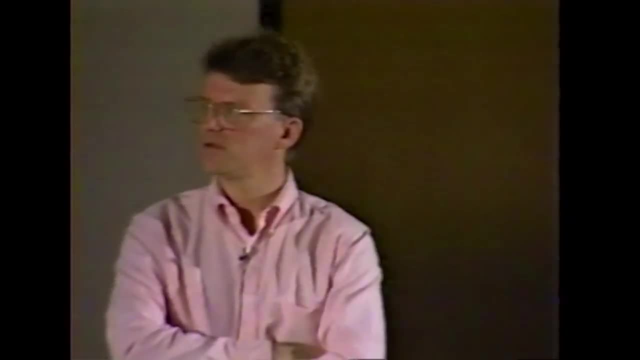 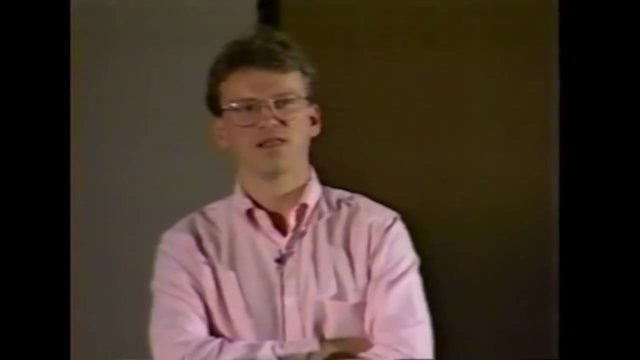 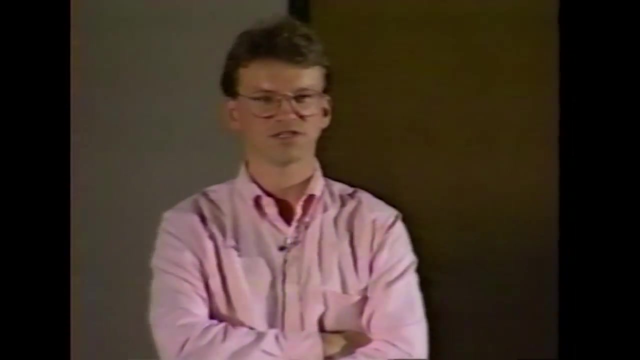 printers, 80-column dot matrix printers, and you had a mix of those two. Before we got the Apple II and Apple III's up, Jeff Raskin had imbued us with polymorphic poly-88s using their editing system and we did all of our editing on poly-88s- SOAROC terminals. 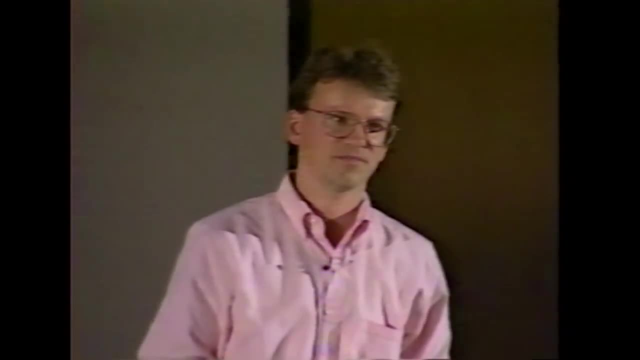 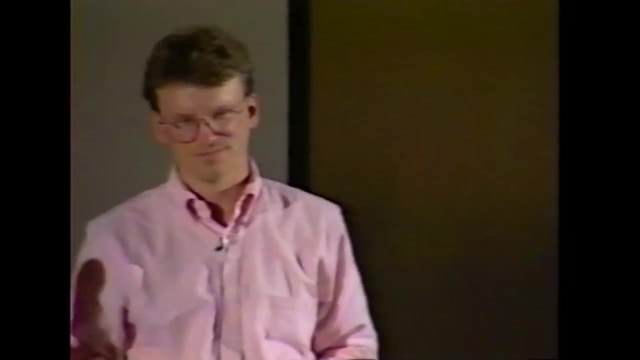 Back there, Back in the- I think it was probably 1983, 1984- time frame, digital research had a graphic interface called GEM Right- Different name. That's sort of got varying litigation of some sort, Mm-hmm. 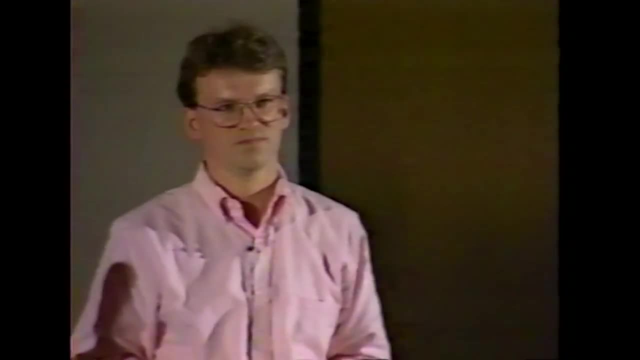 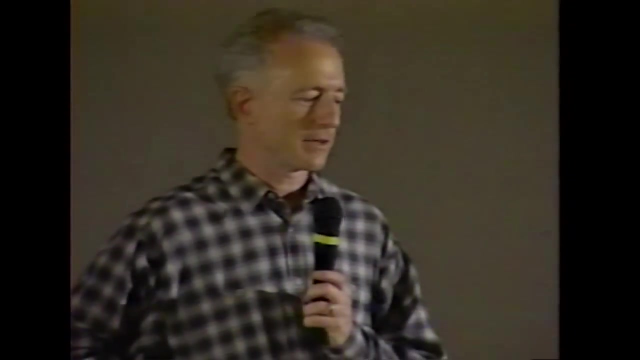 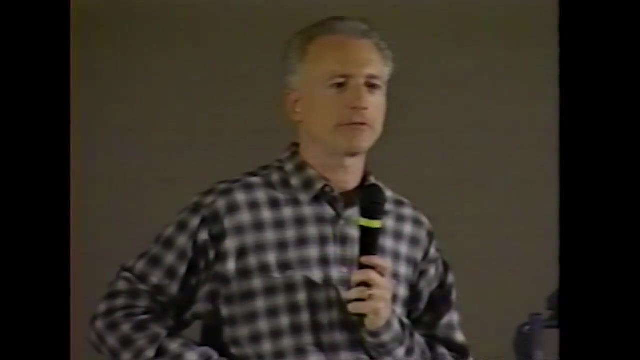 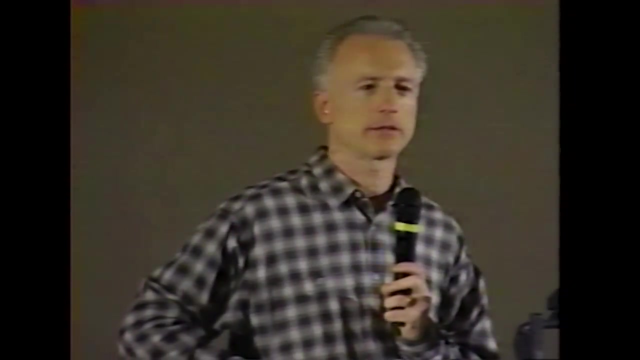 Can you comment on that whole story from Apple? Well, I don't know about successfully competing in that part, but yeah, definitely it was extremely close to the Mac user interface, the GEM user interface, by digital research, and Apple sent some kind of complaint letter and there were some discussions between the. 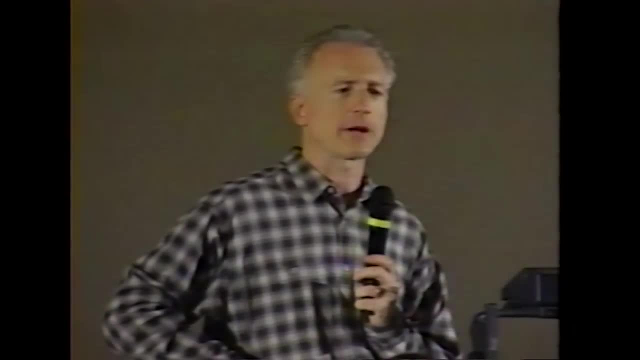 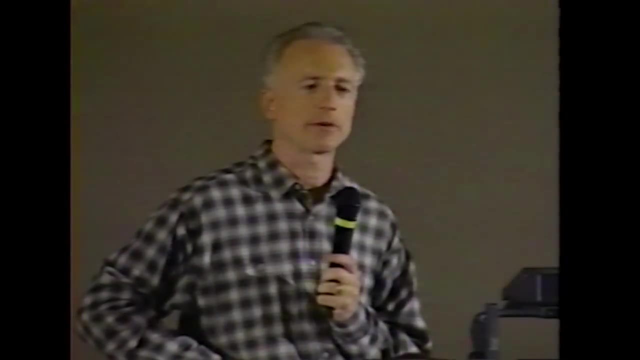 companies, but then Microsoft and Hewlett-Packard started to talk about it and they said: well, we're going to start doing Windows and New Wave, and that was a much bigger issue. so Apple kind of stopped bothering digital research and instead got involved in a big lawsuit. 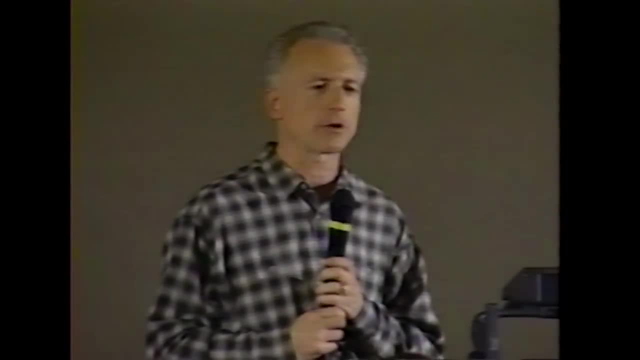 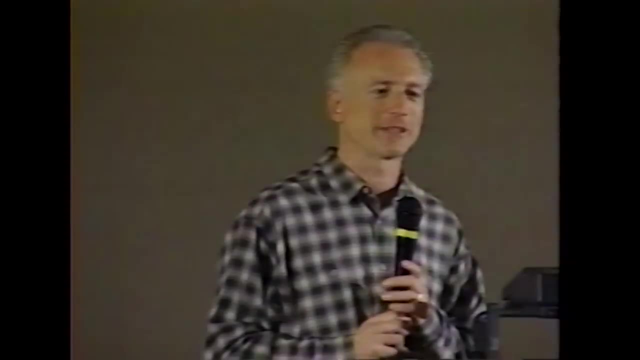 with HP and Microsoft. Digital research at the time was kind of a struggling company and Apple didn't want to. you know, basically pick on a little company. so instead we picked on two companies that were too big instead of picking on one that was too little. 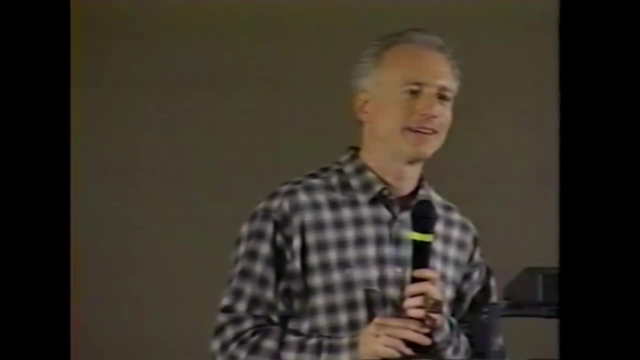 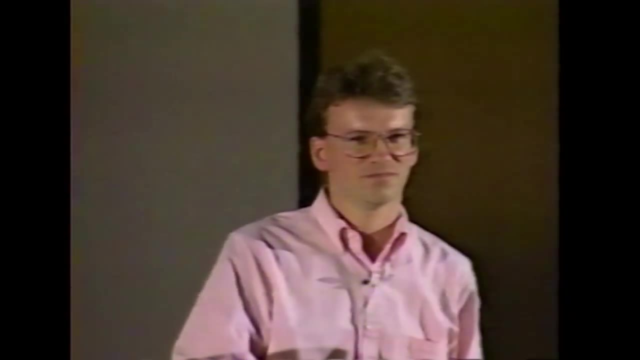 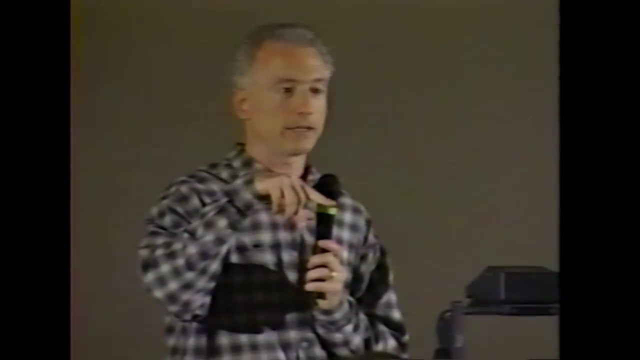 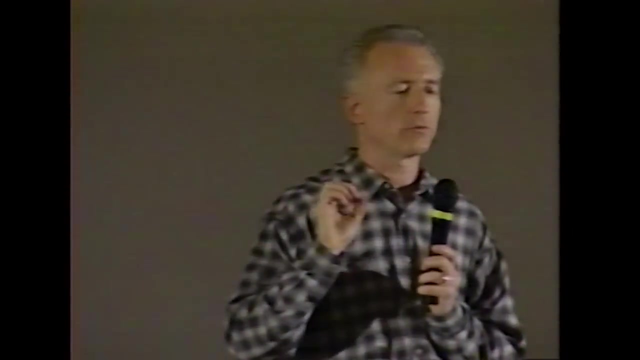 Bernard. Bernard, Would you like to comment on the fact that both Lisa- Yeah, the like- the Xerox Star and the Lisa were, the idea was that in both groups was that people would only use a few applications. It's kind of true. 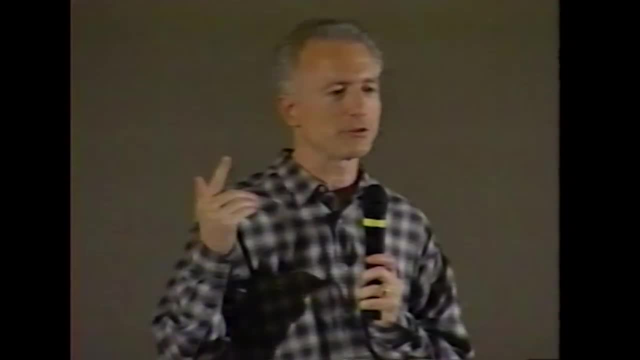 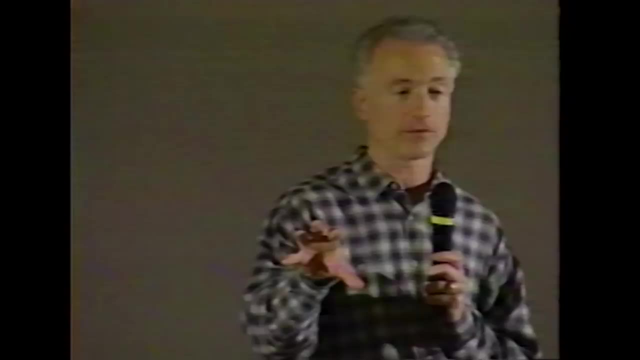 Most people only do use a few applications, but the conclusion that therefore it wasn't necessary to have third-party applications was kind of ridiculous. Actually, in the Lisa it turned out, we did have a place for third-party applications. We thought for certain vertical markets there would be third-party applications and we'd 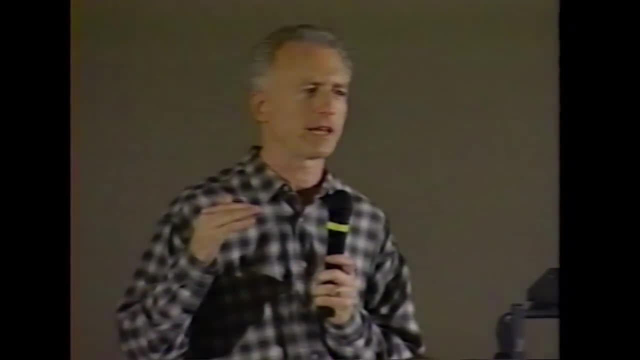 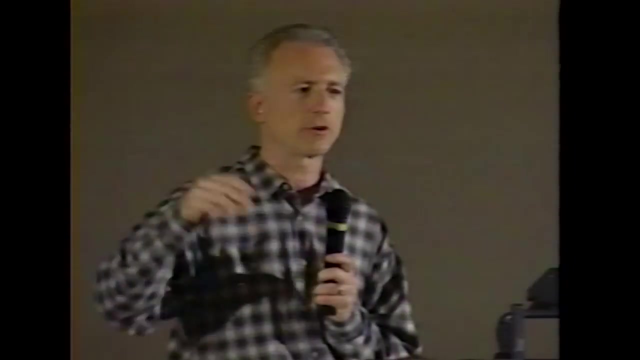 have accounting software and so on. but even then we were thinking very small scale, like there would be one page layout application and there would be one accounting application and you know, a couple of vertical market things. If we ever had 20 applications or 30, that would have been a very large number, very different from the Mac which, from the very beginning, was going to try to do the same thing. It was going to do the same thing as the Apple II and what the IBM PC did, which was go for lots of third-party applications. 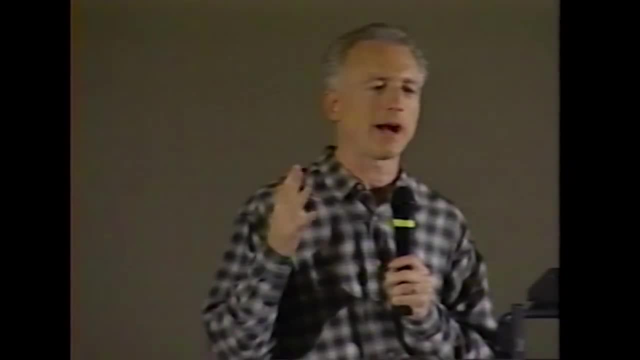 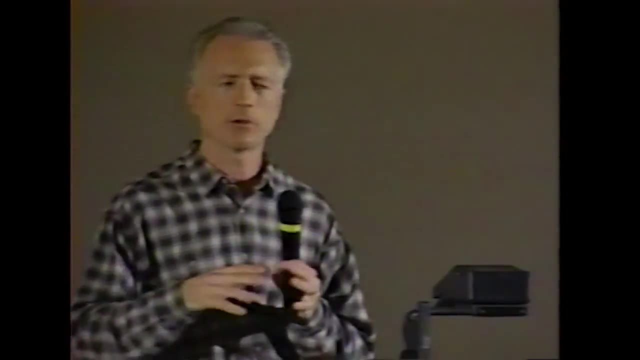 I think one reason the Lisa was designed as it was was to try to justify why there was this project going on in the company and we already had an Apple II and an Apple III. Why do we need this other thing? And well, the Apple II and the Apple III, you know, are going to have all this third-party. 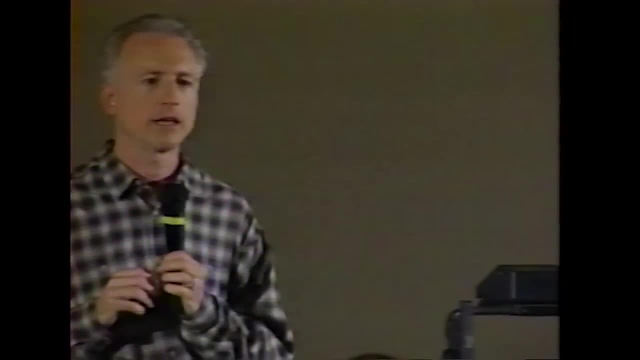 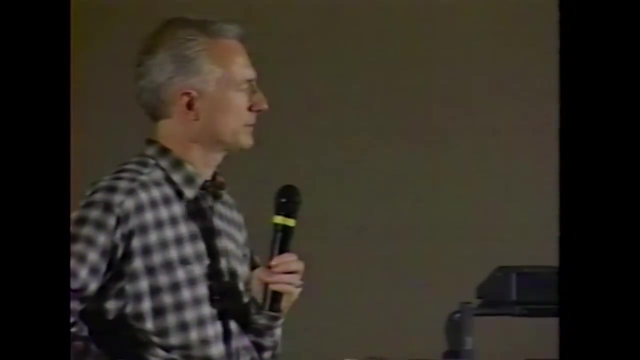 software, but the Lisa won't. It was kind of a differentiator, It was a kind of a closed system. that was supposedly a plus. It turned out to be a major minus, of course. Yeah, well it was. that was not necessarily unique to Apple at that point. 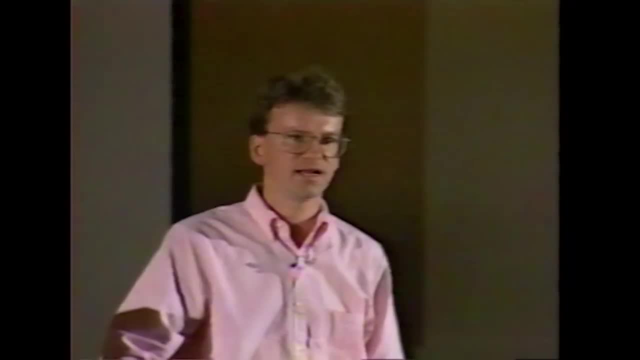 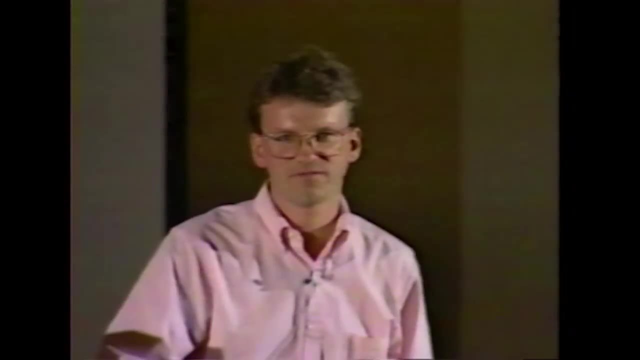 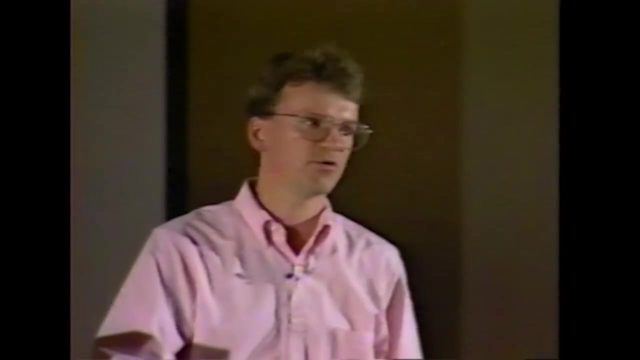 Remember, one of the leading software companies of 1979, 1980 was Personal Software, which became VisiCorp, and their flagship product line at that point was a failed product line called Vizion, which was an attempt to expand VisiCalc into a comprehensive suite of interacting. 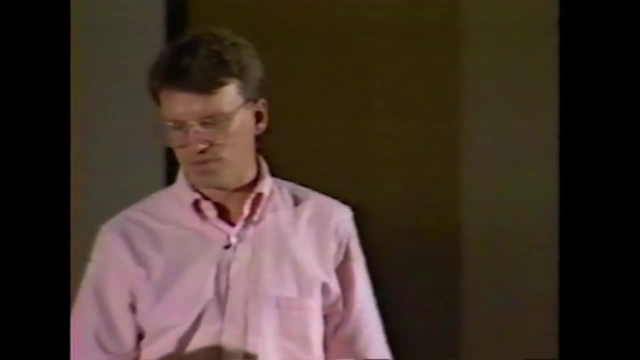 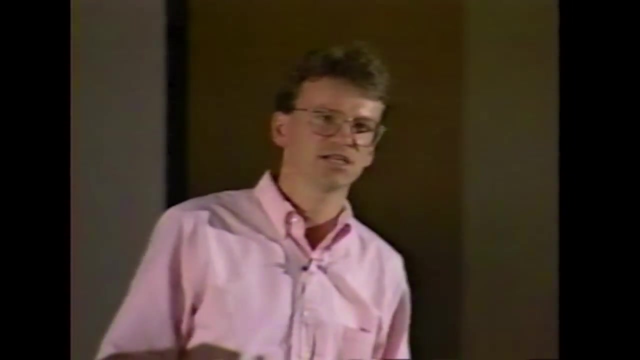 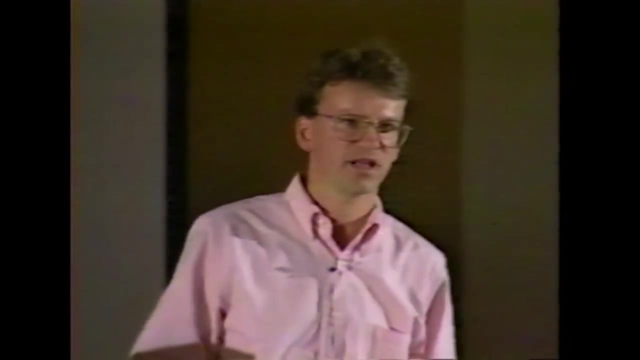 applications, a word processor, a database. WordStar at that point was also trying to expand and everybody was trying to do what Microsoft has successfully done with Microsoft Office, Which is turn the thin end of the wedge of getting one successful application which 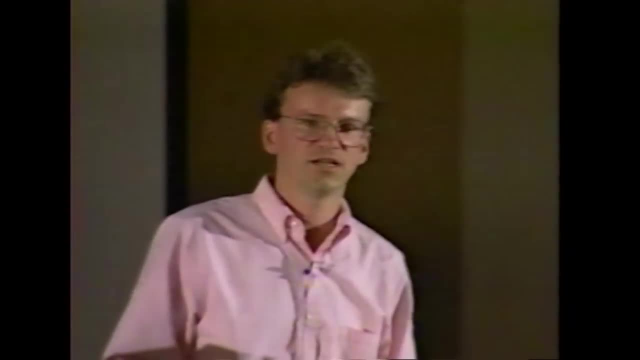 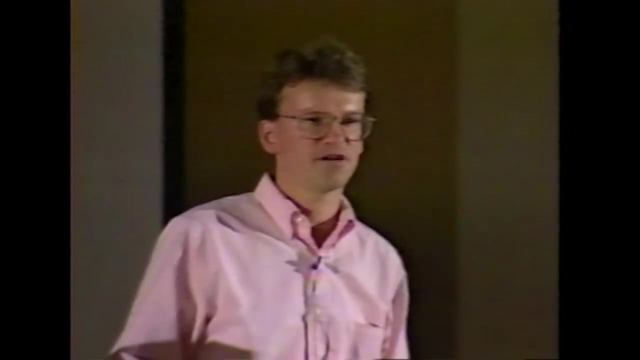 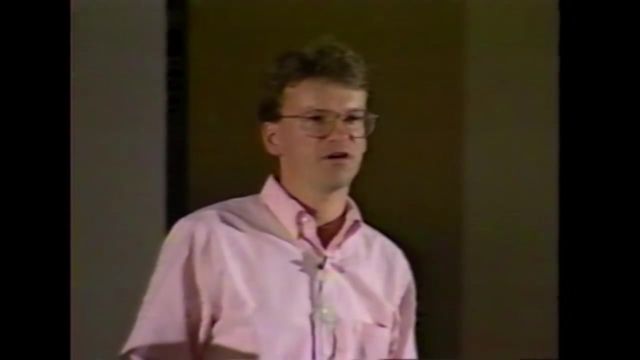 Microsoft had with Excel on the Macintosh and turn that into a major suite that delivers all of the application computing needs of a given set of users. Microsoft has done it successfully and one could argue that the default computing platform right now is Windows with Microsoft Office and not very much else. So I don't think that that necessarily was a bad idea. It may have been many years ahead of its time, but Microsoft was selling the Microsoft Office for Macintosh in 1985.. I still have a box on my shelf where they supplied the word processor, the spreadsheet. 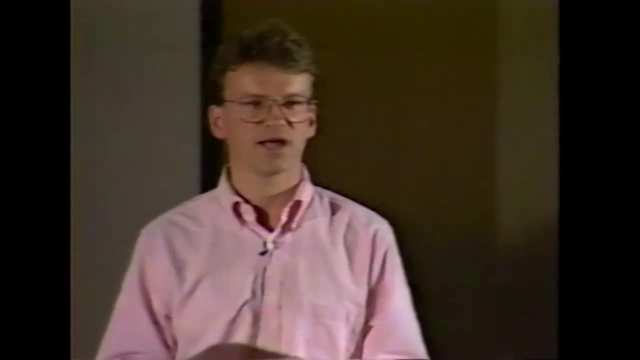 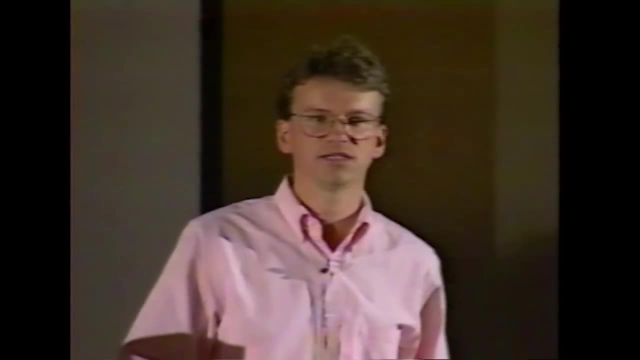 the filing program, the terminal program, in one box for one price for the Macintosh. So Office Suites are certainly, they certainly were not a dumb idea of 1981. It's something that has really monopolized the industry. Yeah, I think that part's true. 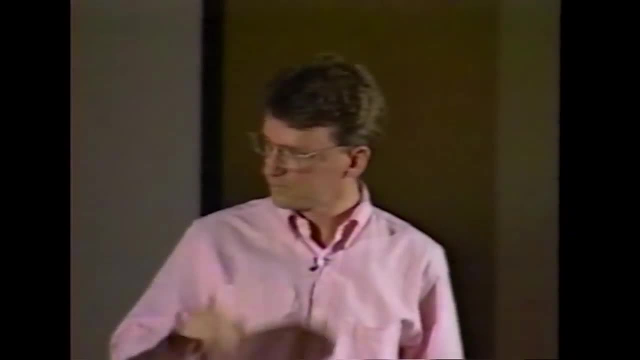 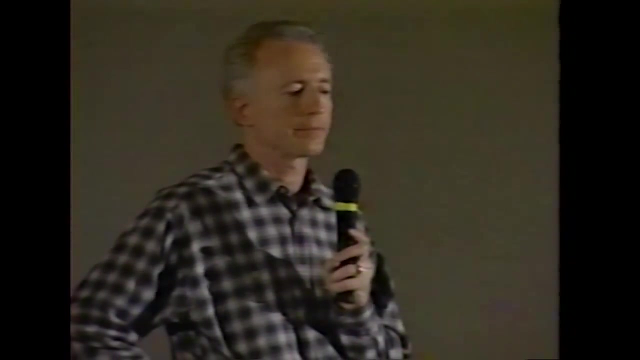 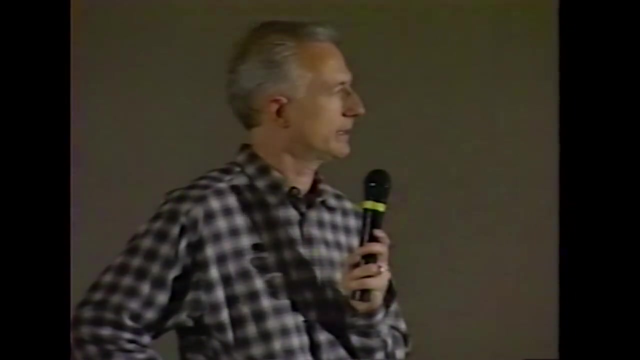 Is this on? Yeah, It was really one of the first Suites, in addition to the ones that Personal Software did, And it was also one of the. it was the first, probably multi-tasking personal computer, But basically ahead of its time and missing the main point, which was you needed a low. 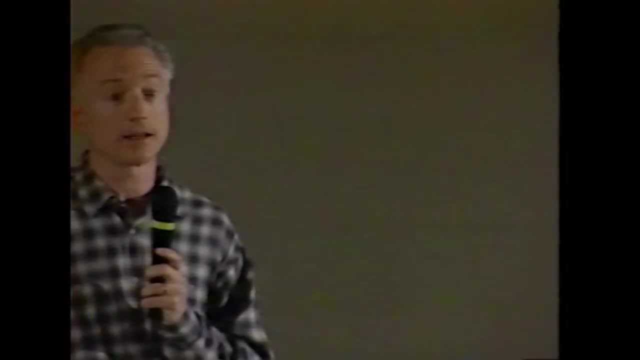 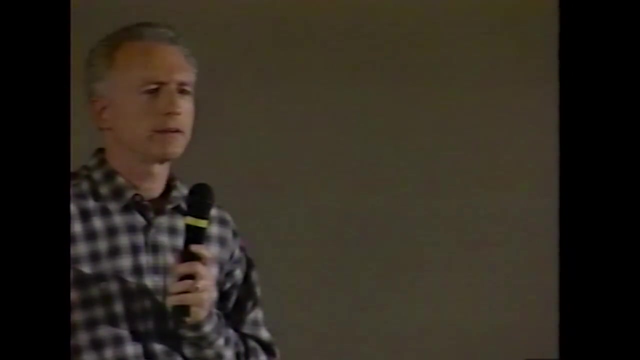 cost platform that had reasonable performance and that had lots of third-party applications. Back there in the aisle, You were passionate about Microsoft. Yeah, You were testing for totally naive users, without any instructions by and large, and yet in the intervening years, acculturation had taken place. 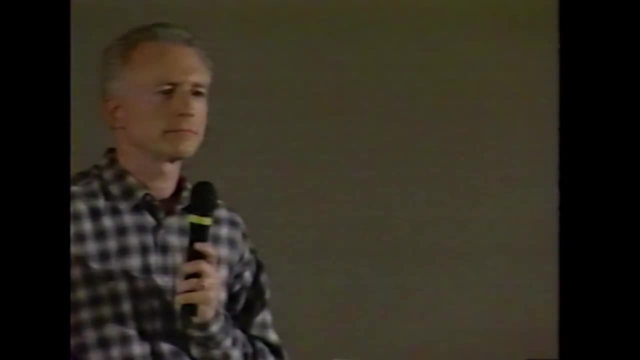 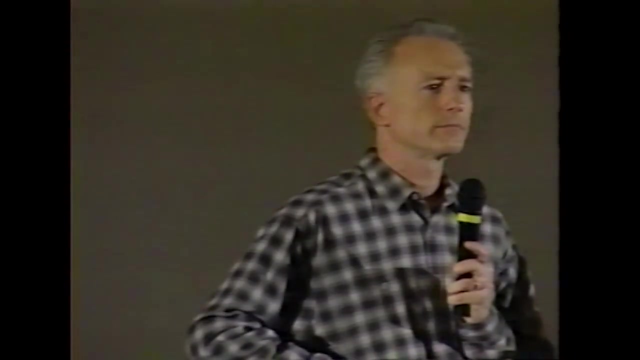 I wonder if that really tells us that, in fact, your testing was not done as possible. Acculturation probably had to take place. The point is that we were testing in the early years for totally naive users and that oh. 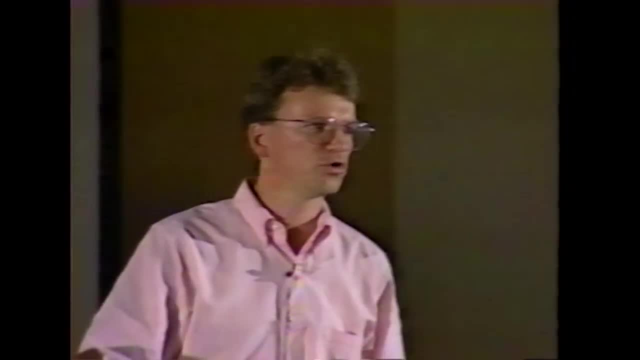 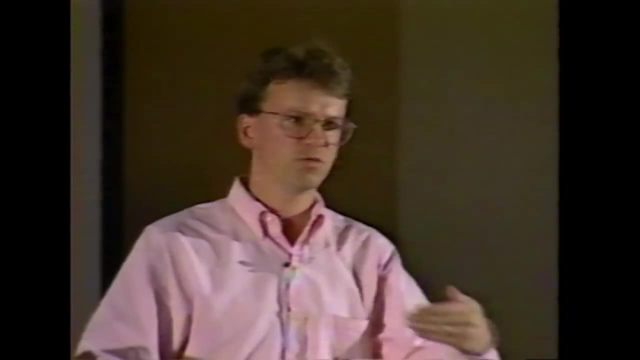 we were testing in the early years for totally naive users, and that, oh, we were testing for totally naive users, And over the years, acculturation has taken place. as I talked about, More people approach computers with less fear and with more pre-knowledge of what they're. 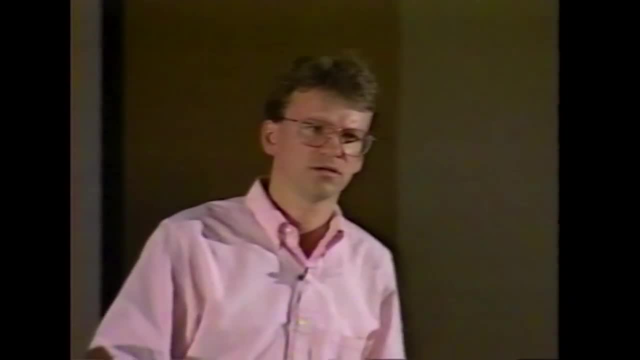 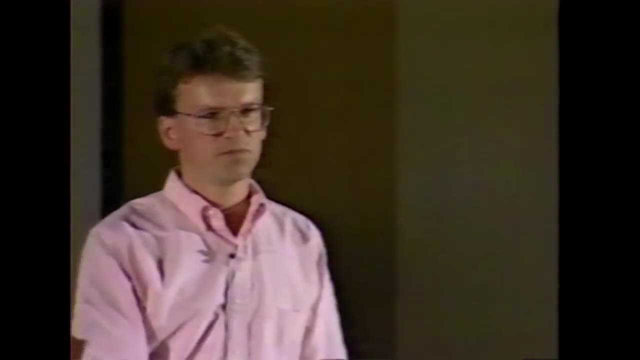 doing. Is that your general point? Yes, And that pre-knowledge came from a process of a decade or more of experimentation, And the process came from a decade or more of experimentation. Well, I'll tell you about an interesting user experiment that I did. 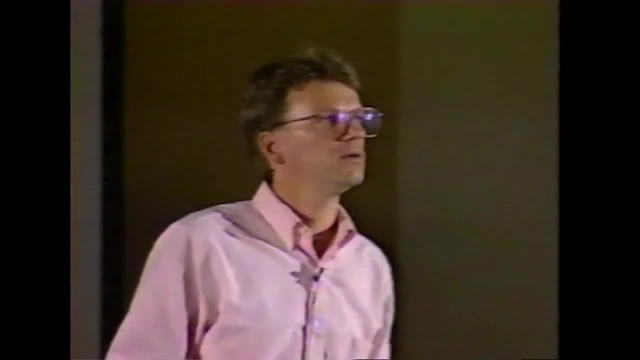 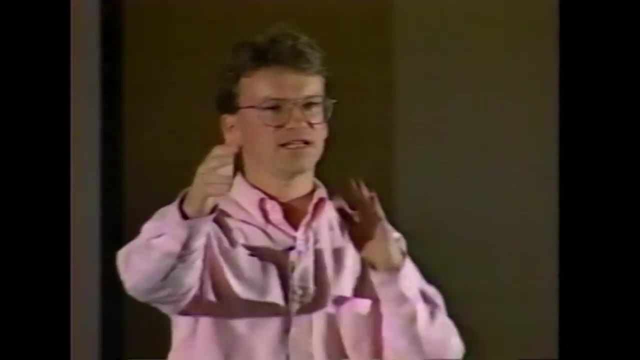 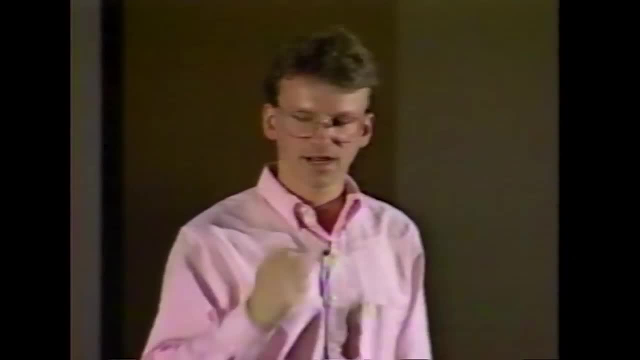 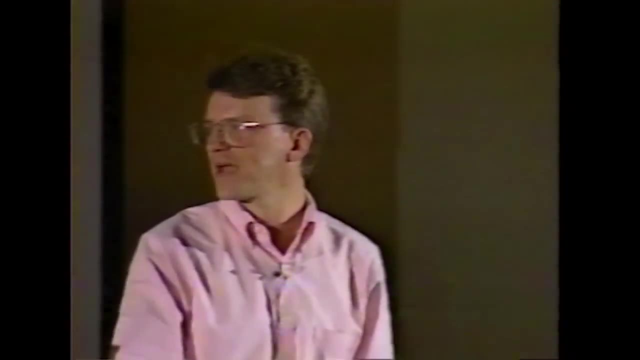 We didn't have any of the injection molded cases yet With the guts. inside. it was running an early version of Mac paint, which was called Mac Sketch at that point, And it was a turnkey application. You put the disk in and you booted it up and it went straight to that application because 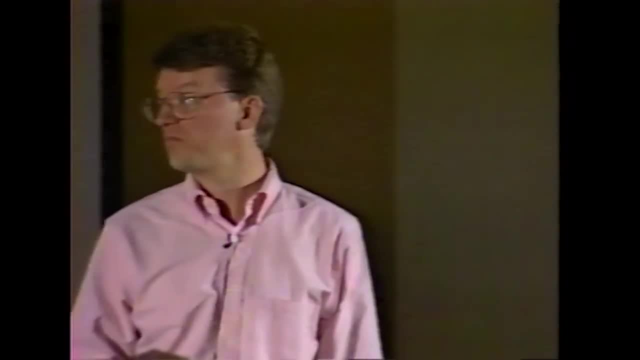 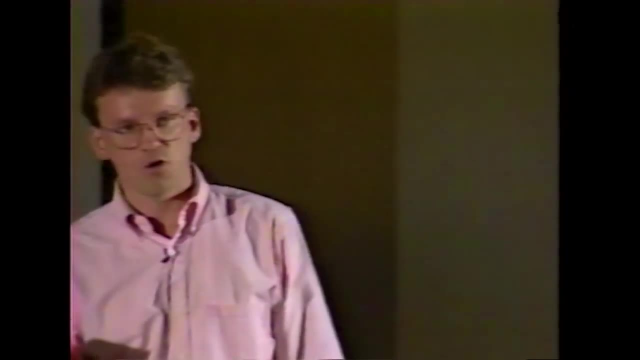 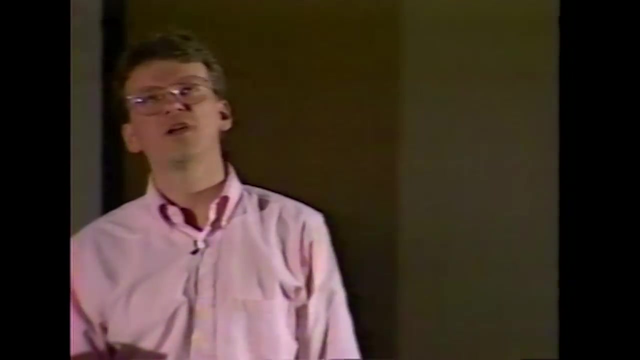 there was no finder at that point, which was actually the paradigm of most other machines, which was turnkey boot. you put the floppy in and you booted it and you got into that one application and i took it over to my girlfriend's parents house for thanksgiving where she had a three-year-old 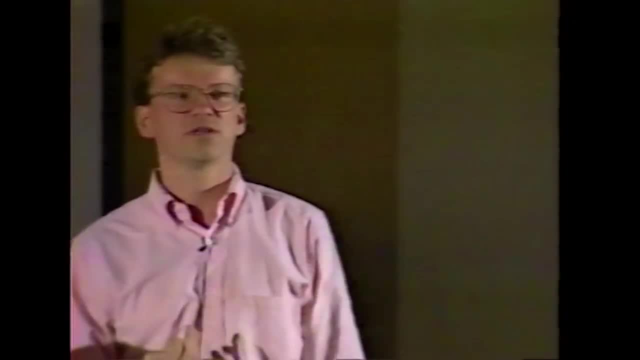 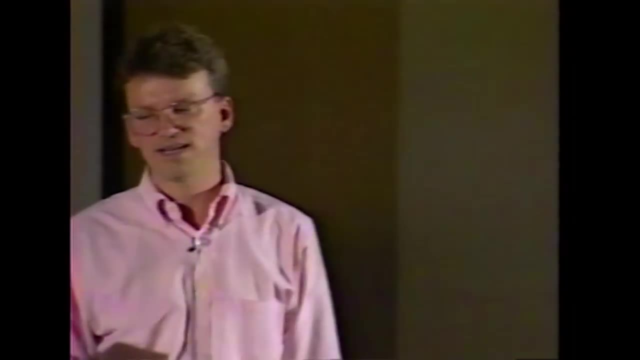 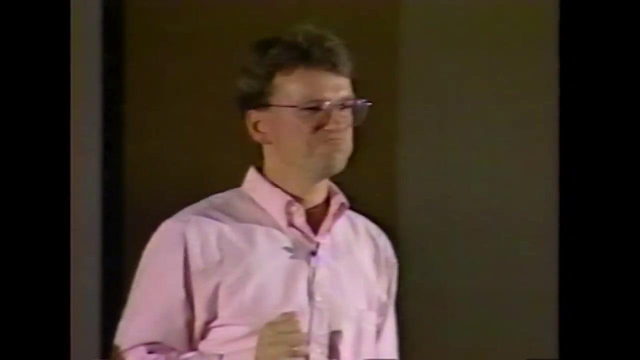 nephew, three-year-old nephew, and this was in 1981. video games weren't even that, hadn't even gotten down to three-year-olds by 1981. that boy spent four hours drawing with mac sketch. he learned it in no more than 15 or 20 seconds, just you know. you press the button and draw things on the screen. 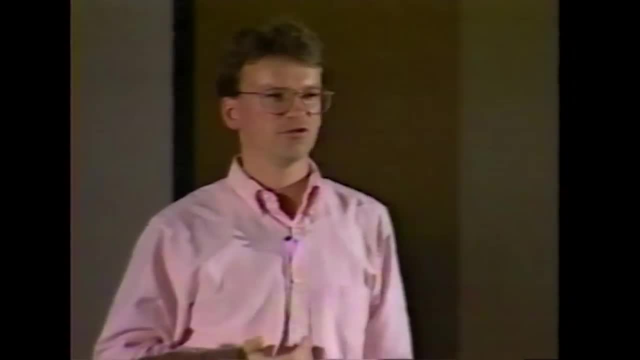 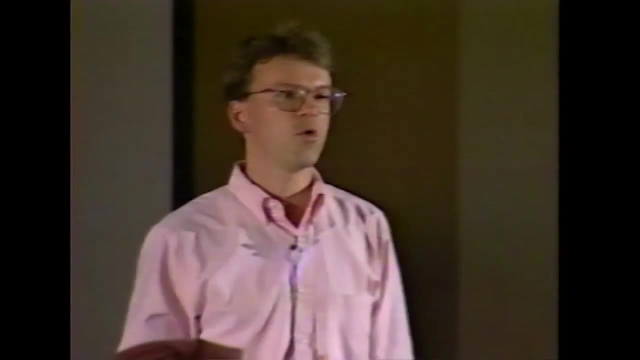 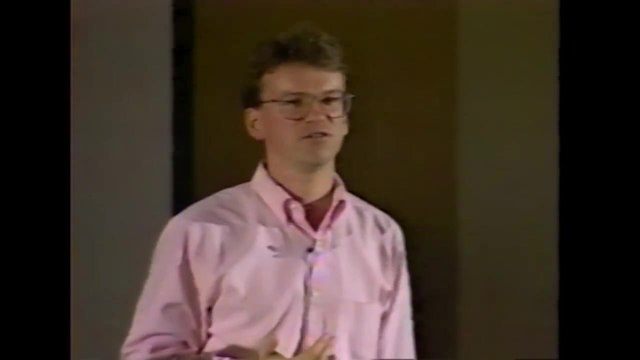 and he was drawing things with with an early version of mac paint, with virtually no tutoring and almost no language at all, with no cult, with no acculturation at all. so there were some things that we got basically right about you, human, human factors: if you can appeal to a three-year-old and get a three-year-old, with no 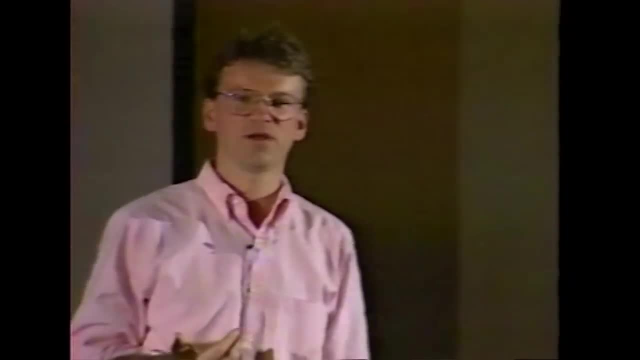 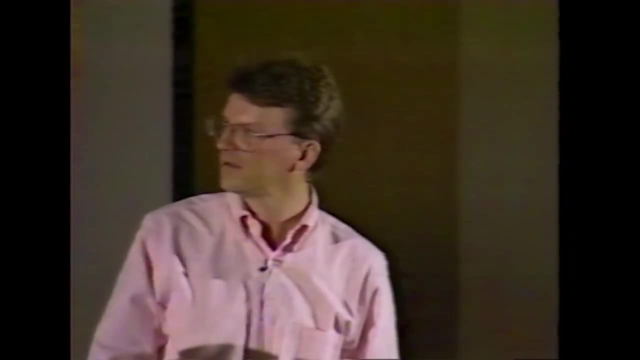 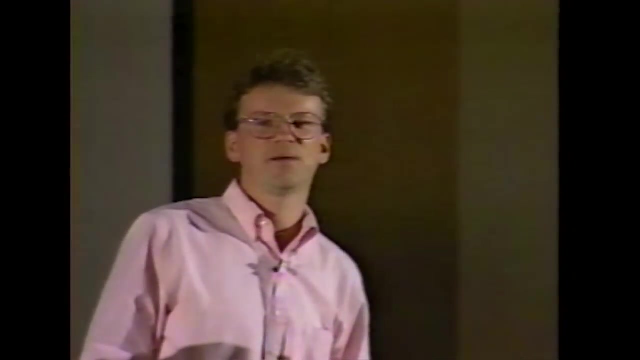 language skills to understand how to do something productive in no time at all. that's not a cultural statement. you've done something right in design, and that's when i knew we were really onto something. i don't think it's had no effect. i think what acculturation has done is it's um, it's got it's.